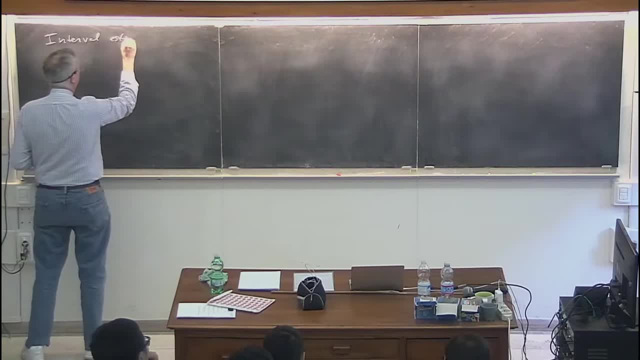 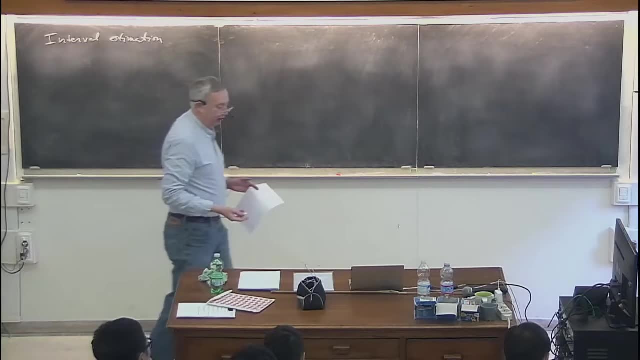 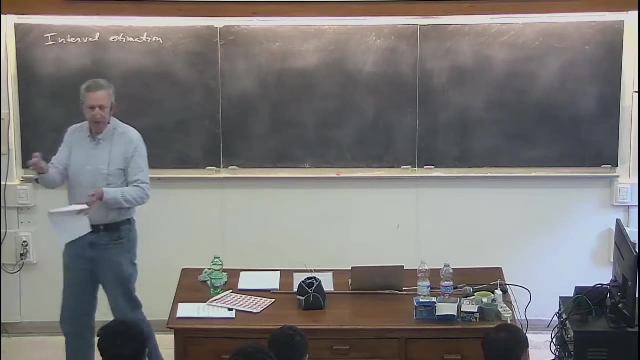 so interval estimation. This is as opposed to point estimation. so if I construct an estimator like the maximum likelihood estimator, I'm getting a single number out that I used to estimate the value of a parameter. But what I would like to do now is to construct an interval, And I want to make 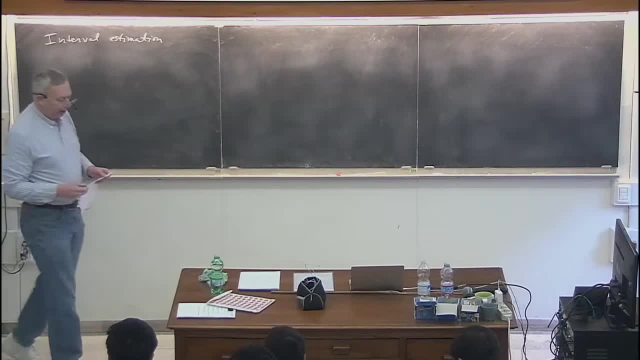 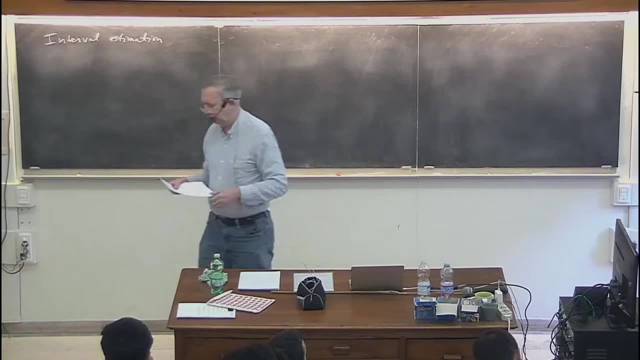 some kind of a statement that says that the probability that this interval will contain the true value of a parameter is at least a certain amount, And this is going to lead to the well-known things like confidence limits on parameters. So I should say interval as opposed to point. 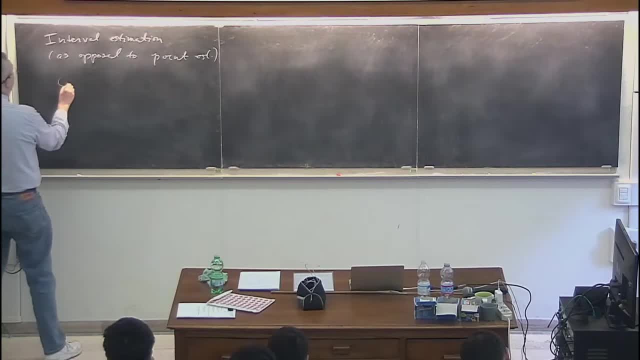 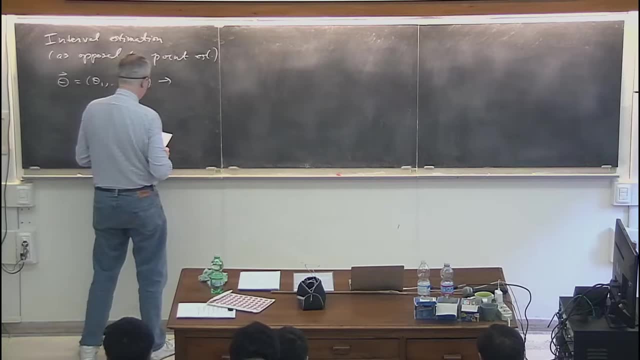 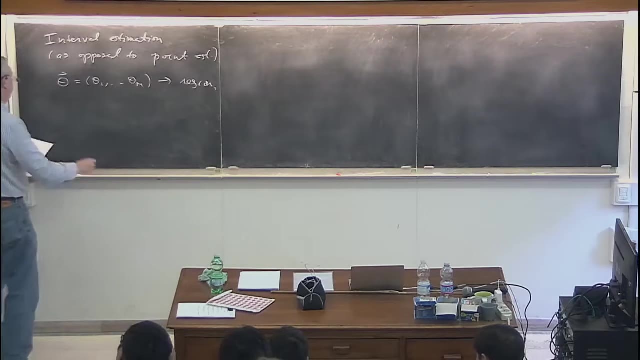 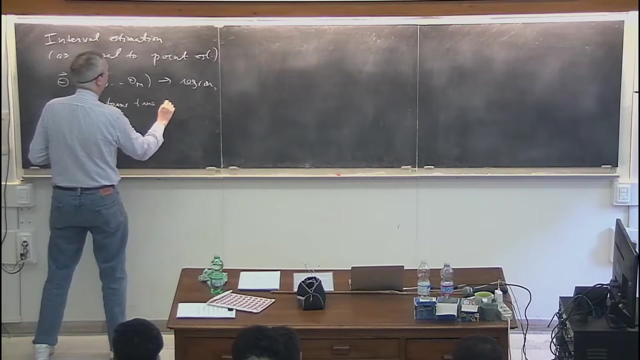 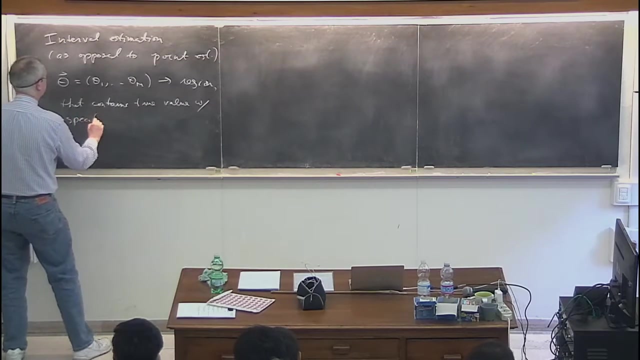 And in the case if we have a multi parameter problem, so some some vector of parameters in some higher dimensional space, what I'm going to find is a region that contains the true parameter value with a specified probability, And so what I'm going to do is I'm going to take a set of parameters and I'm going to 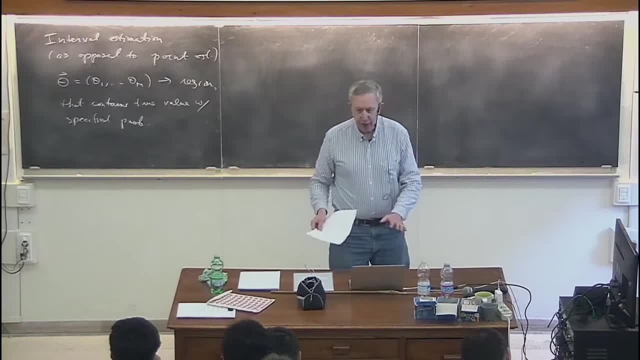 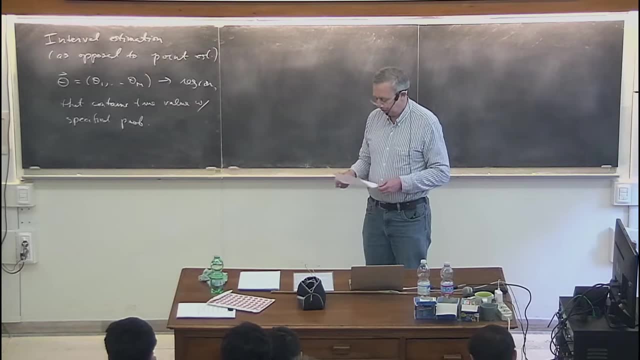 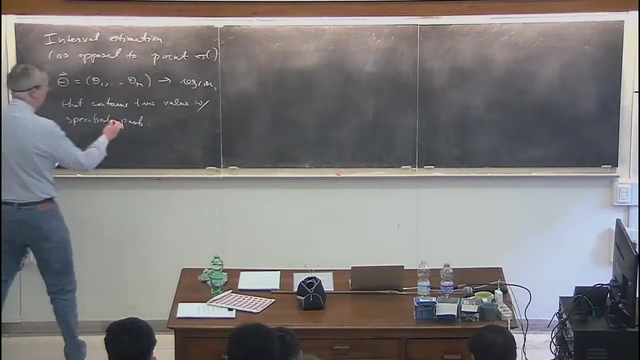 describe is the is the frequentist approach to this, and if we have time- I think it might get pushed into the discussion session- we can go over the the corresponding Bayesian procedure as well, and it's conceptually in fact much, much easier. All right, so well, I can say: actually both of these in both the 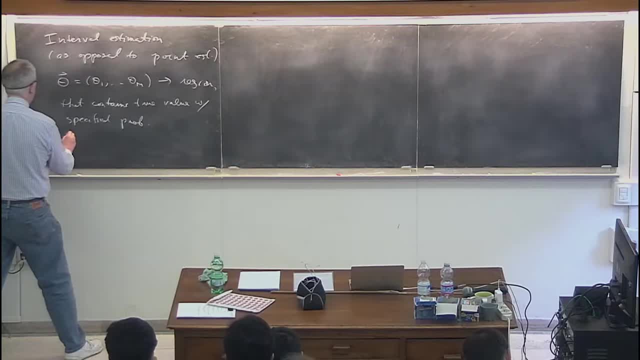 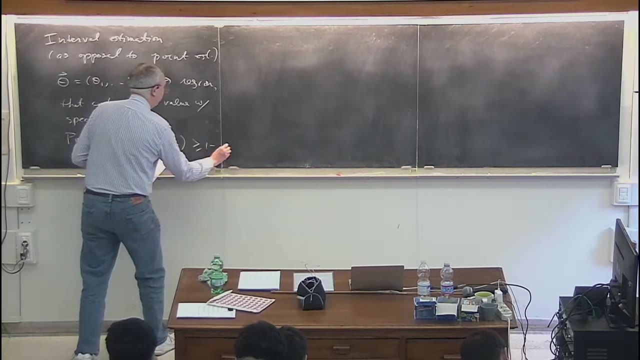 Bayesian and frequentist approach. what we're trying to do is is to say something like the following: probability- theta true- is contained in this region that I will try to construct greater than or equal to some value that I'm going to call 1 minus alpha. I'll call it 1 minus alpha. 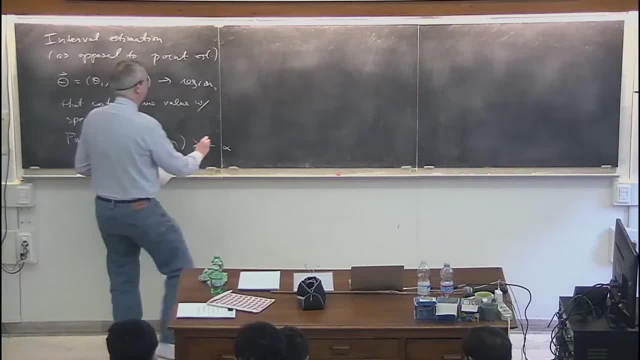 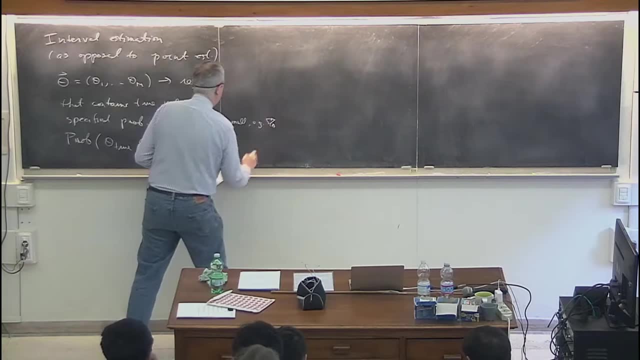 with this usual idea that alpha is some something small, Something like 5% and 1 minus alpha, I will usually call the confidence level. At least that's what we call it in the in the frequentist case, In the Bayesian case. maybe we also call 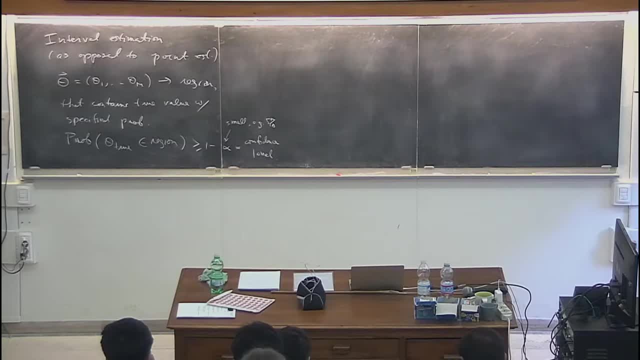 it that, or sometimes it's called the credibility level. But the point is that if I want to make a statement of the form, the probability that a true value of the theta is contained in a certain region, that means I have to have some notion of how I interpret my probability, and so you can see already that this is. 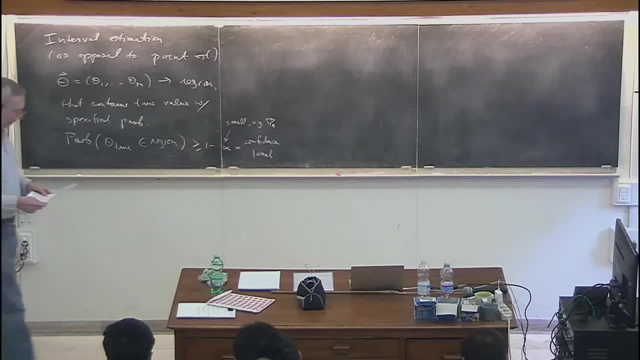 going to lead to it to different down different paths in the frequentist approach and the Bayesian approach. So let's talk about the frequentist approach, Frequentist. The idea now is, if I have a problem with a parameter, theta is I'm going to. 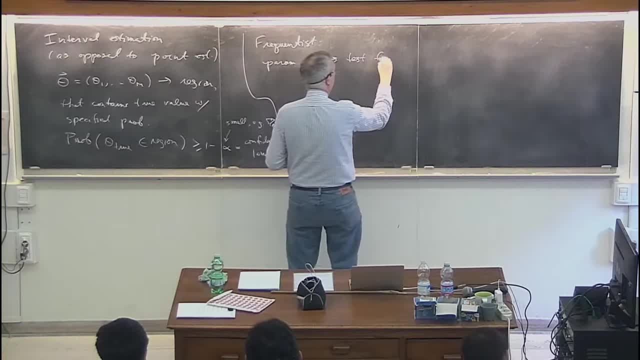 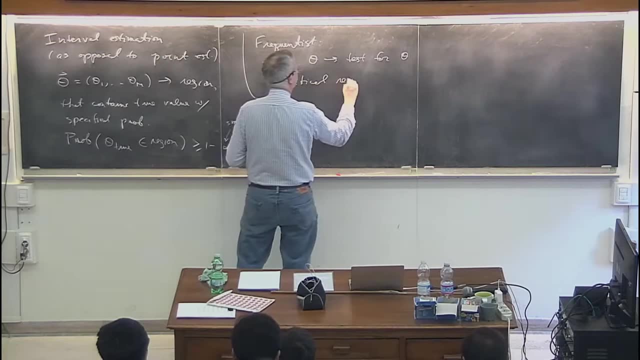 construct a test for a specific theta, and what does that mean? That means that I need to have a critical region W, and since this is going to be a test specifically for a value of theta, I will label that critical region with a subscript. Okay, so that's W theta, Alright. and once I've found that critical region, I do the. 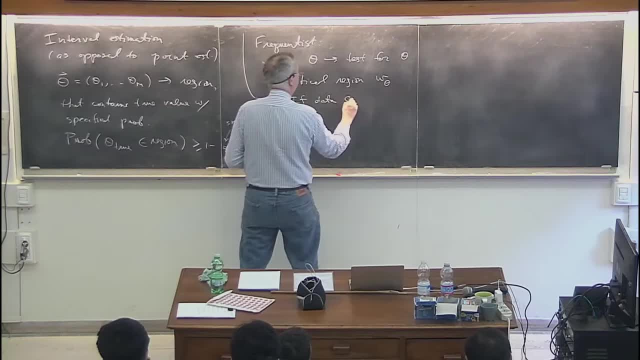 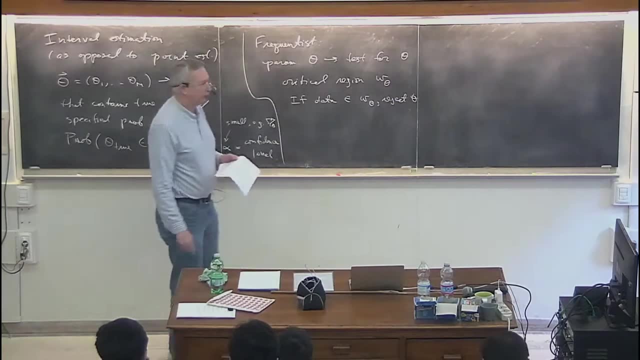 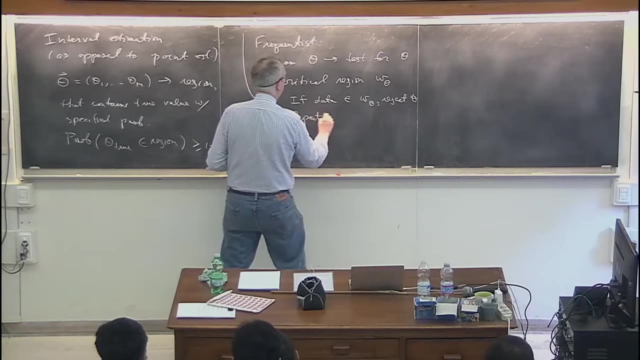 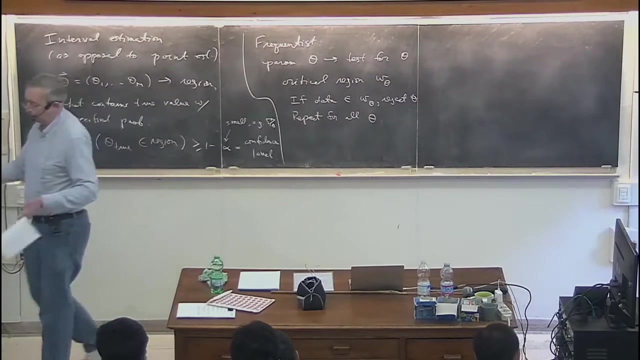 experiment, and I say that if the data are contained in the critical region, you reject that value of theta. Alright, and once I've done that for one value of theta, I can repeat the procedure for all values of the parameter Right, and in doing so, some of the values will be rejected and others will. 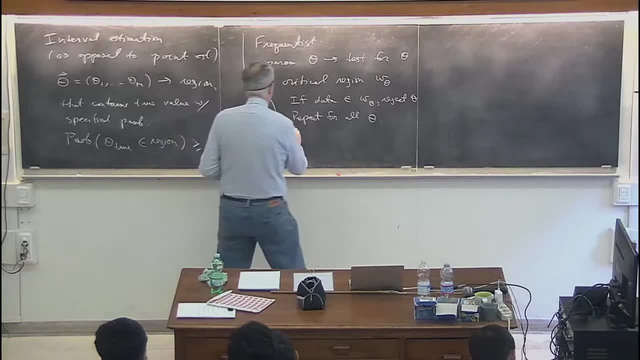 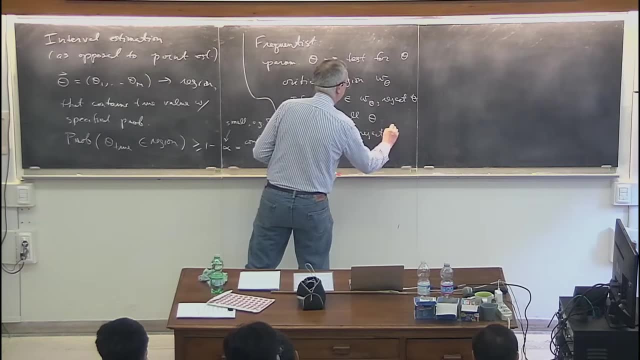 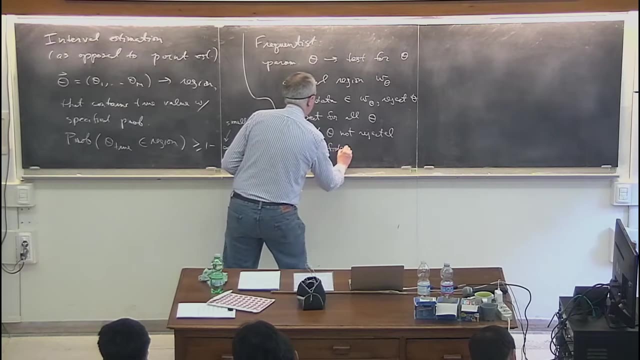 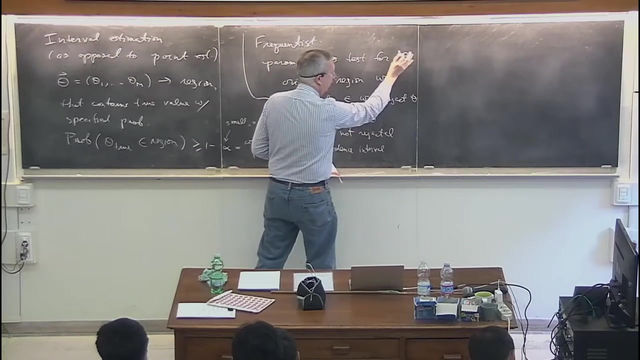 not be rejected. And now I simply say that the set of values not rejected constitute what I call a confidence interval, Confidence interval for theta, or if what I mean by theta here is a vector of parameters, then Okay. Then of course I'm testing all points in a multidimensional space. 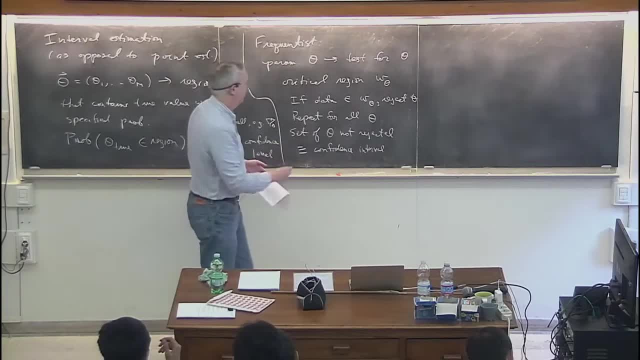 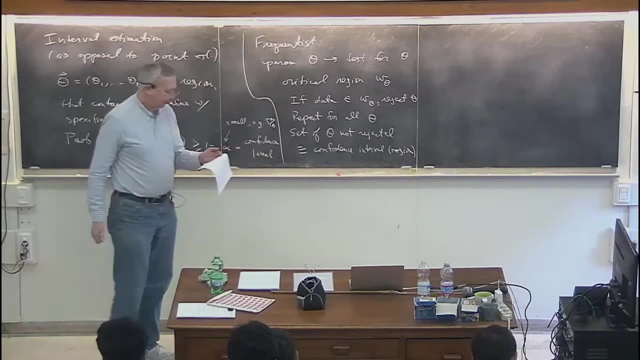 and I'll have some region of that parameter space which is not rejected, and so then I would call it a confidence region. but that's just a matter of vocabulary. It's the same basic idea, And we always specify then to specify the test. 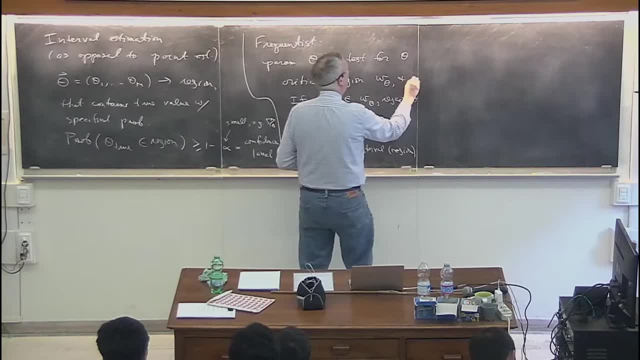 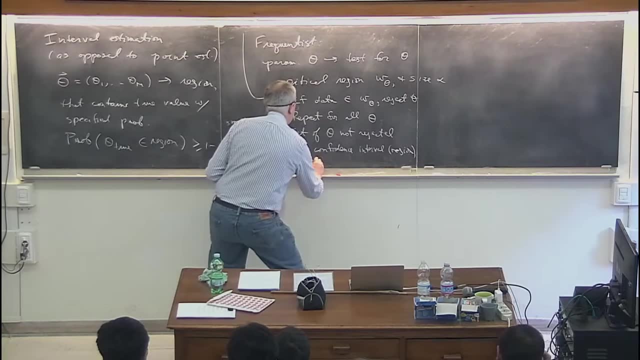 I need to have the critical region and I need to choose a size of the test, And so the confidence interval is then said to have confidence level, or I'll say CL 1 minus alpha. Sorry, that's getting small. It's legible. 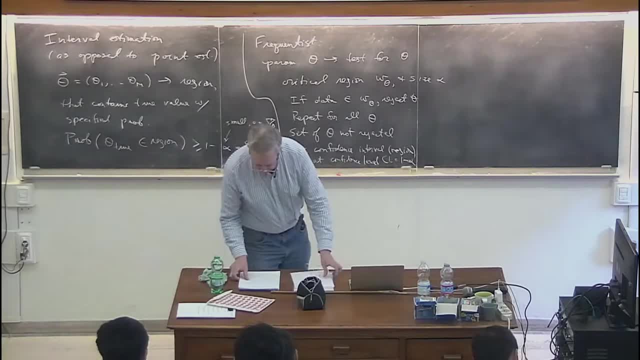 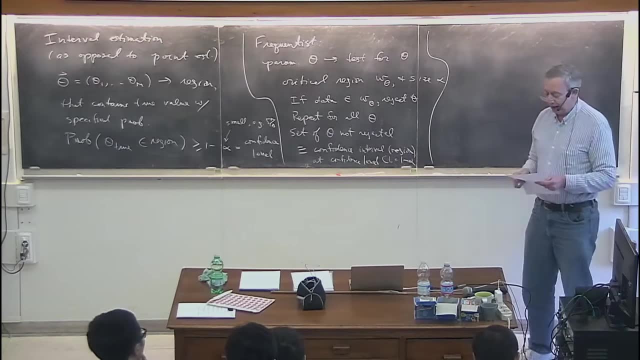 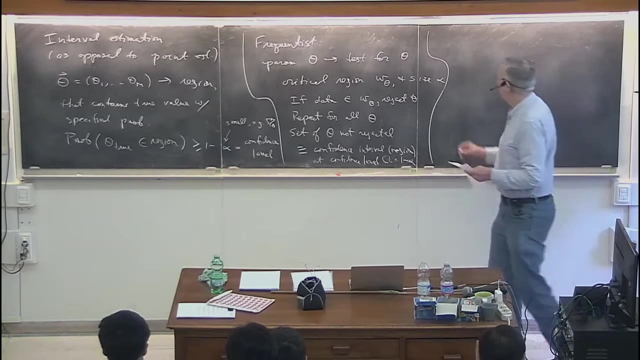 Right Now there's an equivalent formulation of this. We saw that there's an equivalent formulation of the tests with P1 and P2. And it's easy to recast this game with the construction of confidence intervals with P values. What I could do is I could simply say: 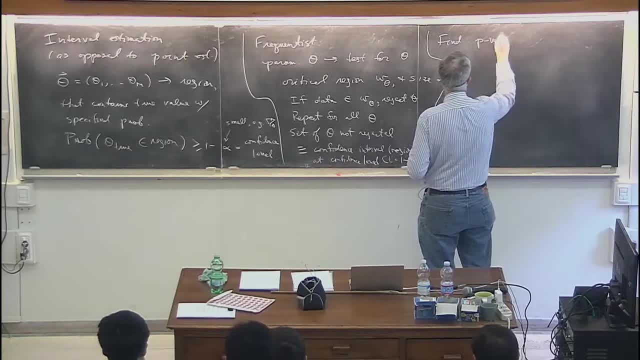 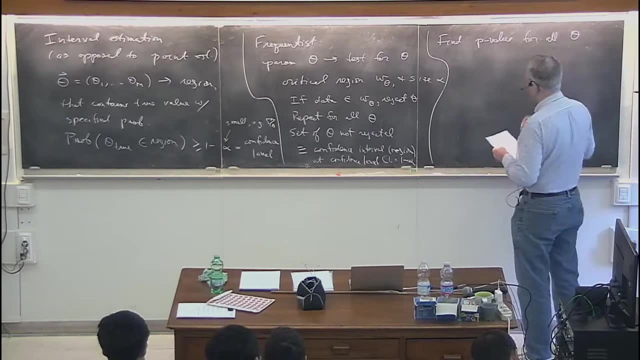 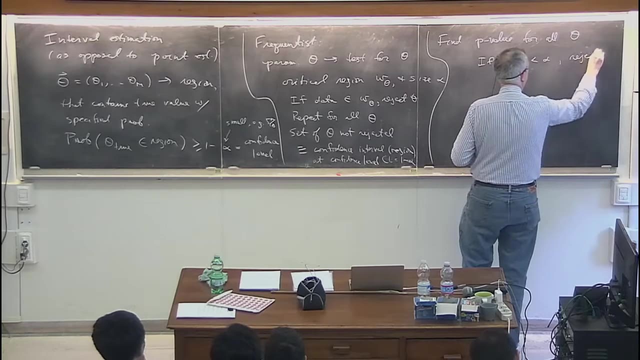 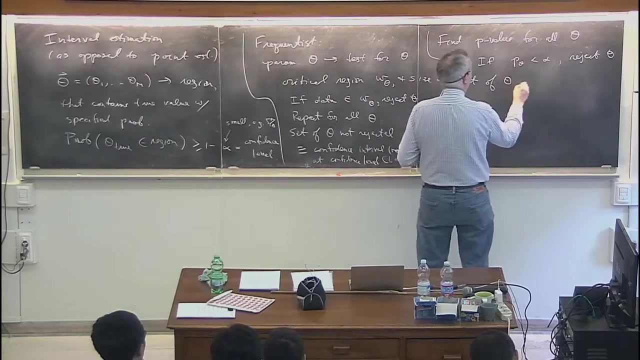 find a P value for the hypothesized value of theta, and I do that for all values of theta, And then I simply say that if the P value is less than alpha, I reject the corresponding value of theta. Okay, And so that means that the set of theta with a P value greater 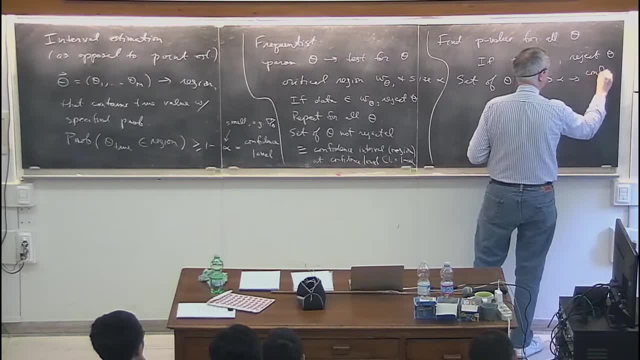 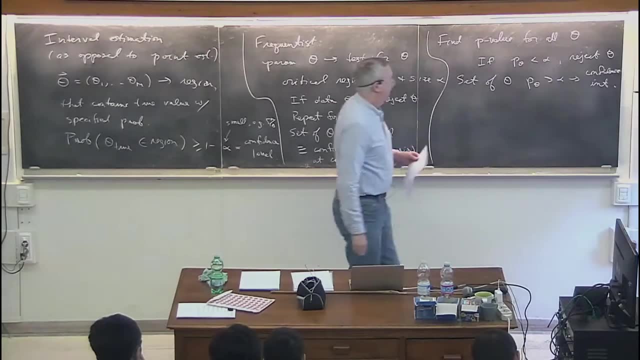 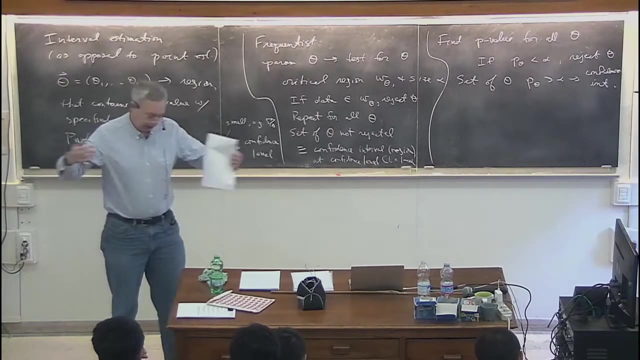 than alpha. that's my confidence interval, Confidence interval, And so that means that everywhere inside the confidence interval, those theta values have P values greater than alpha, And everywhere outside, the rejected ones of course have P value less than alpha. 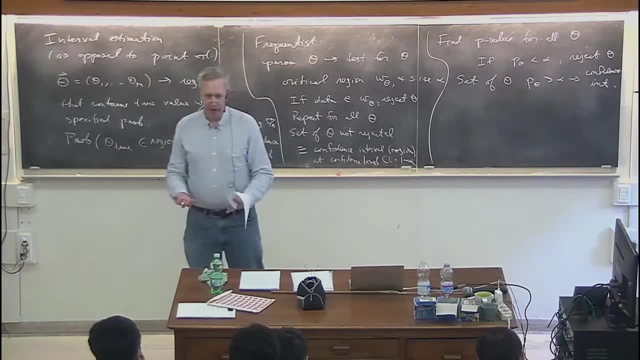 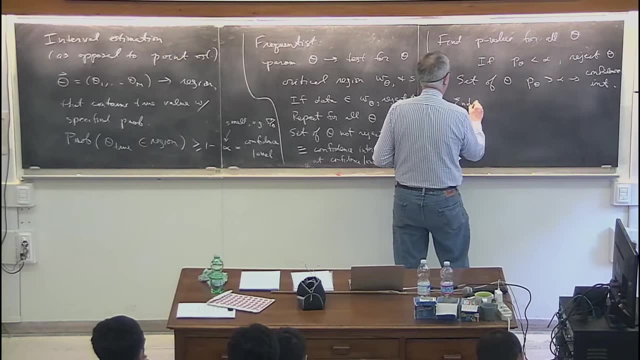 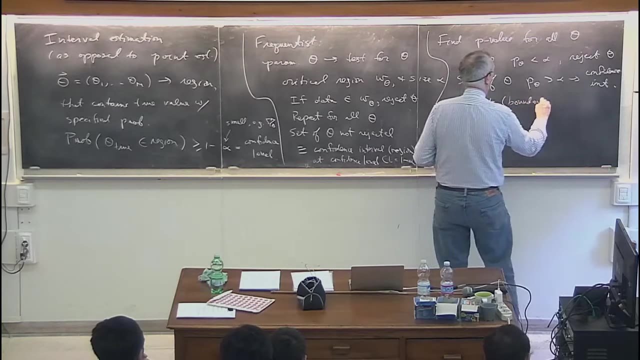 And what you typically want, of course, is to know the boundary of the confidence region or the endpoints of the confidence interval, And so those are the points where the P value is exactly equal. Where should I write this? Endpoints, boundary of the interval. 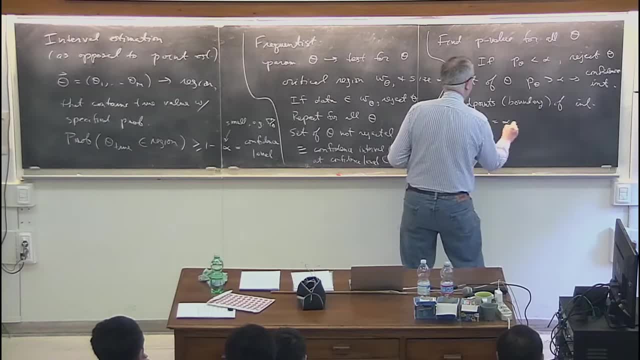 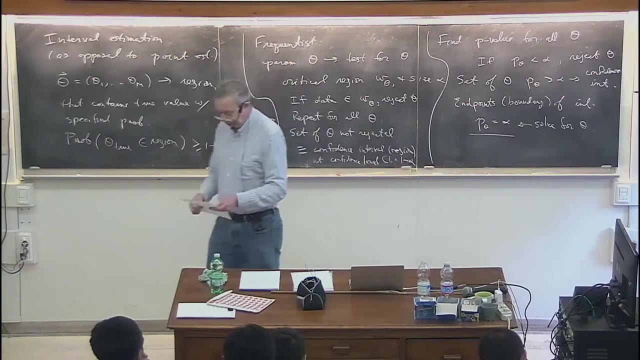 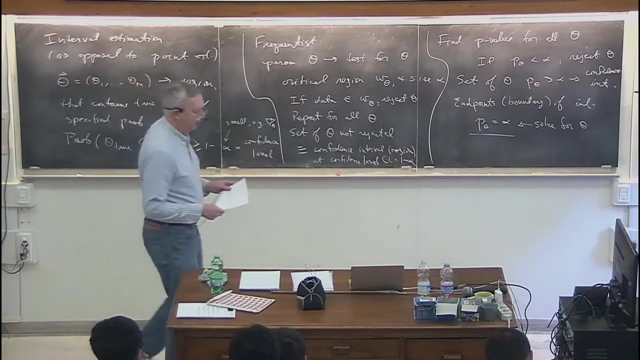 are the points where the P value is exactly equal to alpha, And so what you need to do to find those endpoints is simply to set up this equation and then solve for the corresponding parameter values. So I'm focusing now on the continuous case. 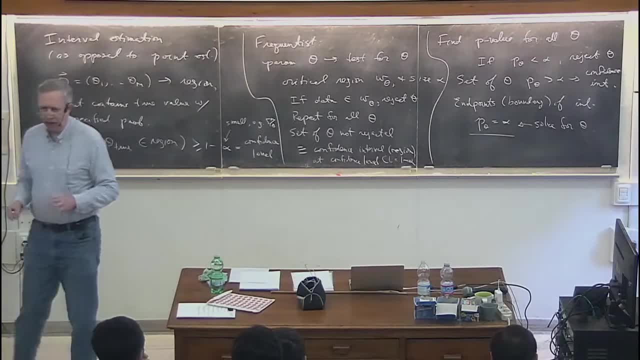 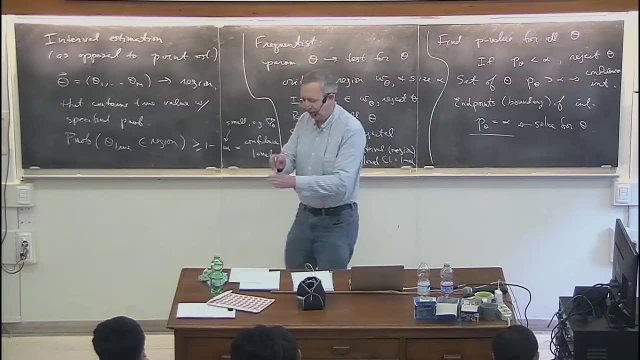 regardless of whether the data are discrete or continuous. Okay So, but if I have a continuous- sorry, if I have a discrete parameter, then what I'm talking about in principle, yes, you could do the same thing, Yeah. 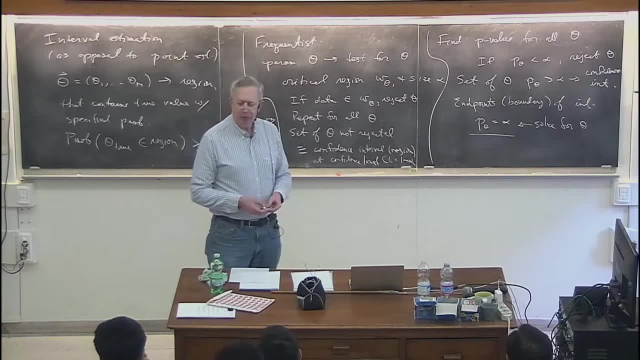 I'm trying to think of an example that comes up in practice, and there are a few. I mean, normally, if you have discrete hypotheses, then of course you can test them and you can either reject them or not, But usually those are not labeled with discrete parameters. 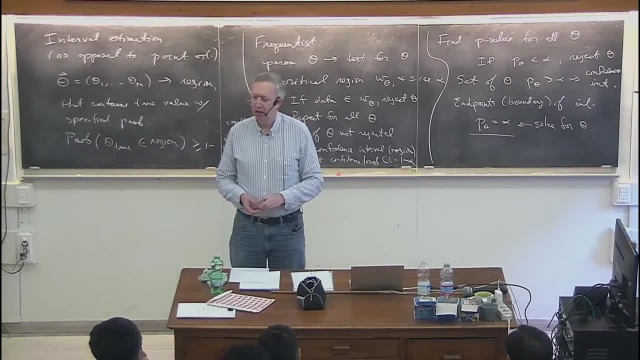 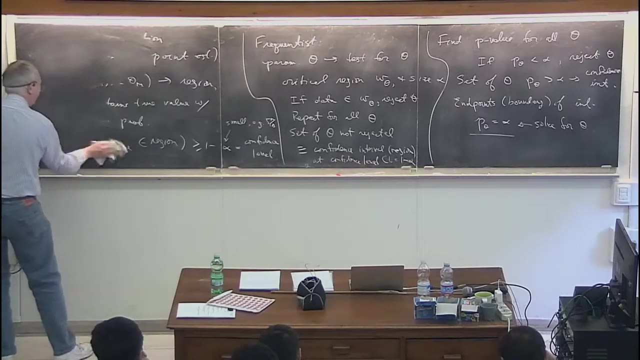 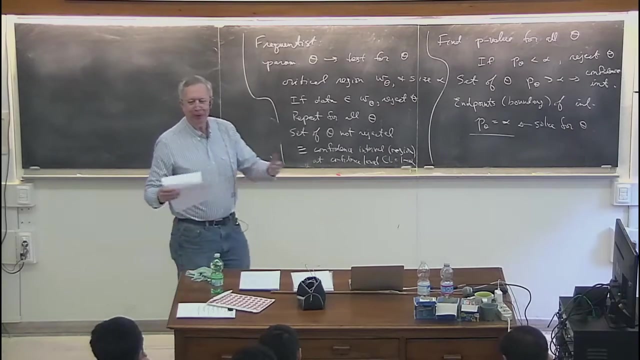 Rather, That's not the situation I'm focusing on now. Yeah Right, So now here's a simple or subtle, difficult point, depending on how you look at it. The way that I've described this interval here is just sort of the generalization of our discussion of a test. 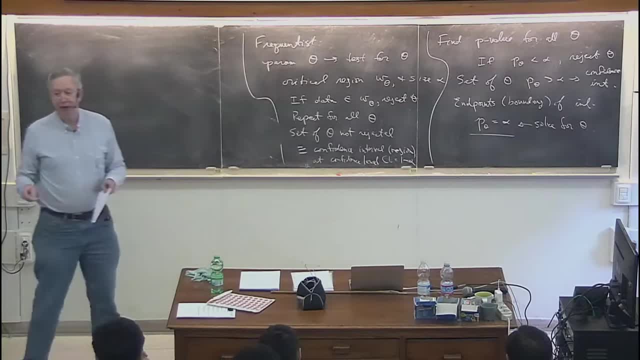 And I want to now assert that the interval that we construct has this property that I alluded to at the beginning, namely that it will bracket the true value of the property: Right, Right, Right, Right, Right, Right, Right. 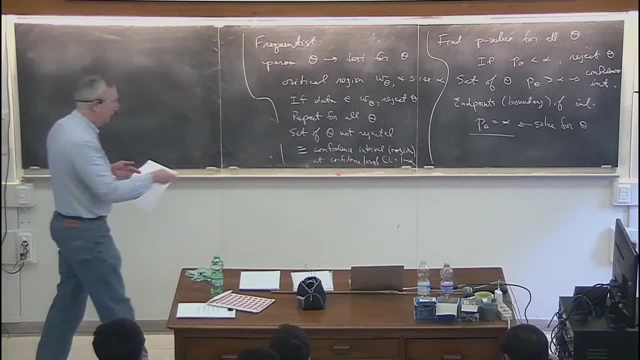 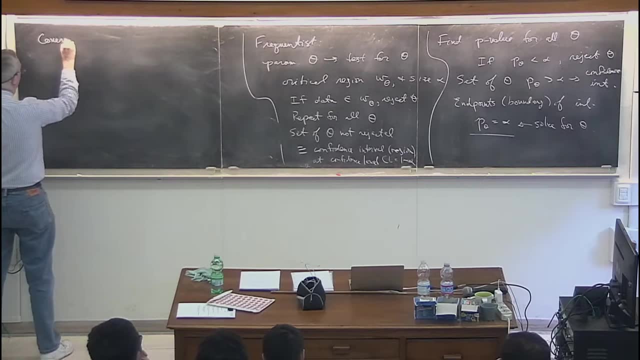 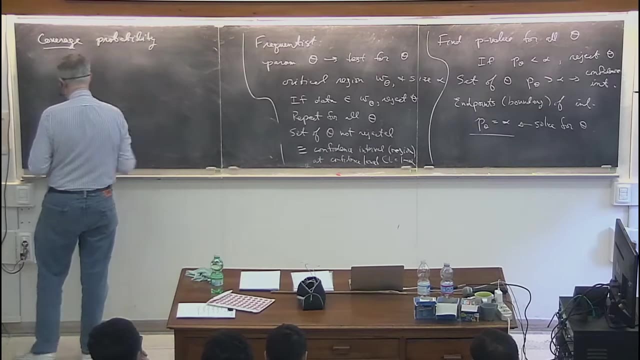 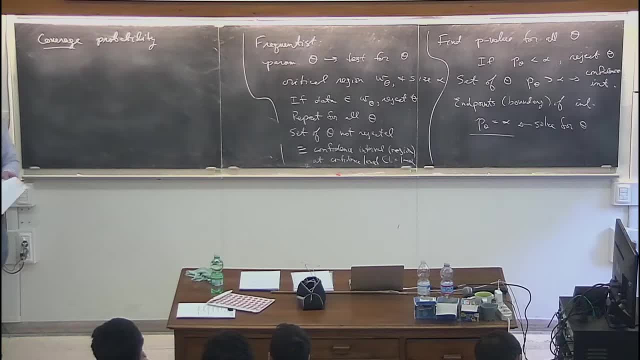 Is that if the true theta is rejected, then it's definitely not in the interval, Right? So let me just write that This is obvious: If theta true rejected, the interval does not bracket or contain the true value. That seems like a silly statement. 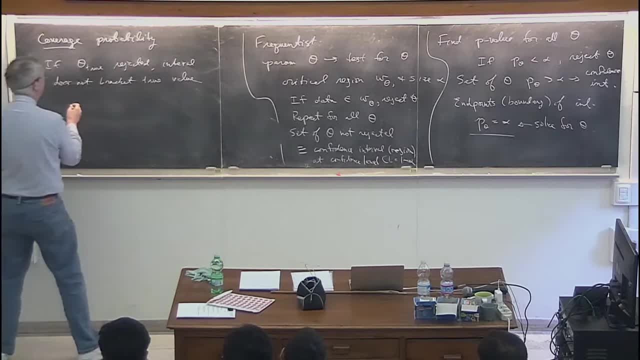 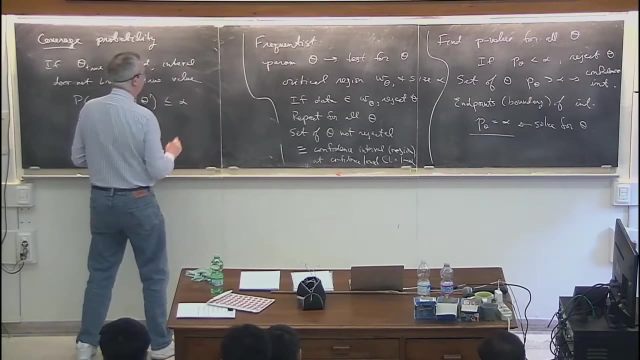 It's just obvious. But what is the probability for this to happen? So the probability that we reject a value of theta- given that it is true by construction- that is less than or equal to alpha, because that was the criterion that we used to establish the critical region of a test. 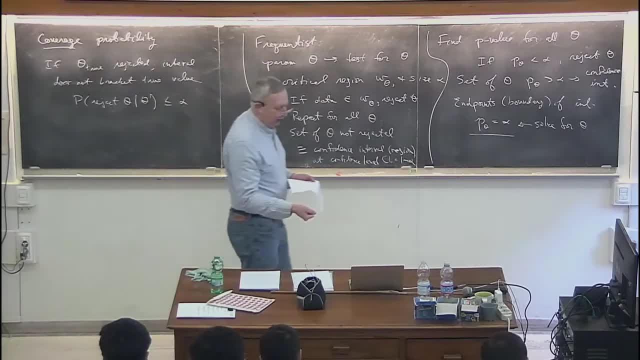 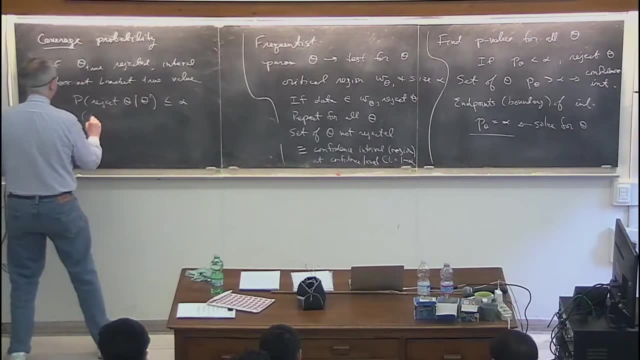 We said that the probability for the data to land in the critical region had to be less than or equal to alpha. That was its defining property. So this is by construction, And so therefore we can say that the probability that the confidence interval contains theta true. 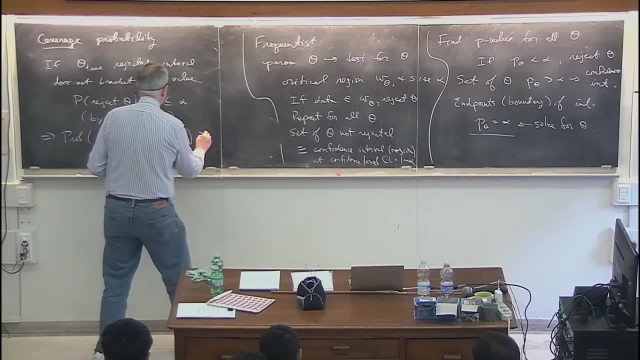 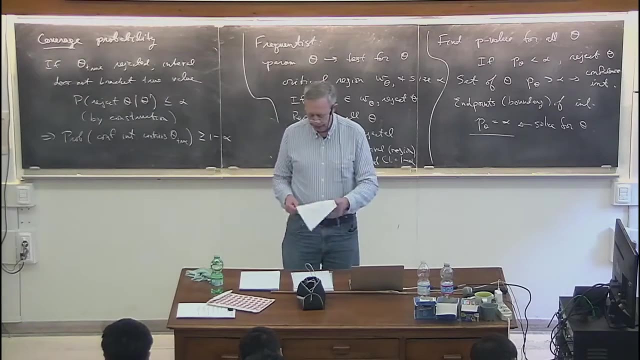 is greater than or equal to 1 minus alpha, And that's usually what is cited as the quintessential property of a confidence interval. It brackets the true value of the parameter With a probability at least equal to this confidence interval. And remember that if the data are continuous. 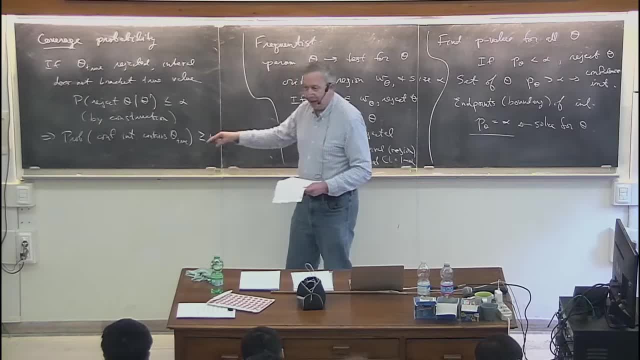 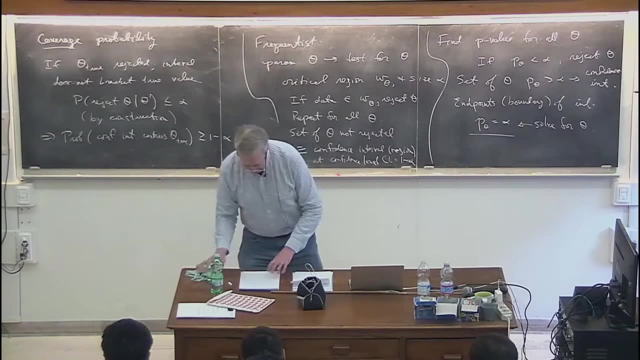 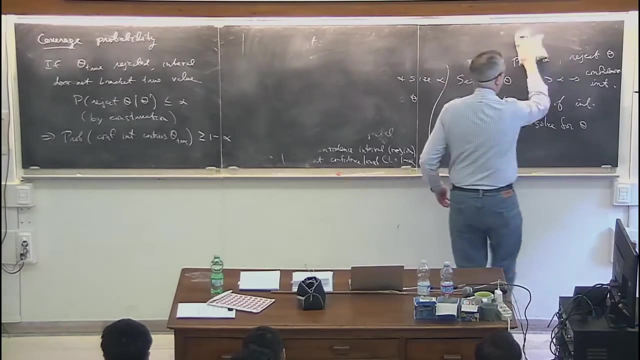 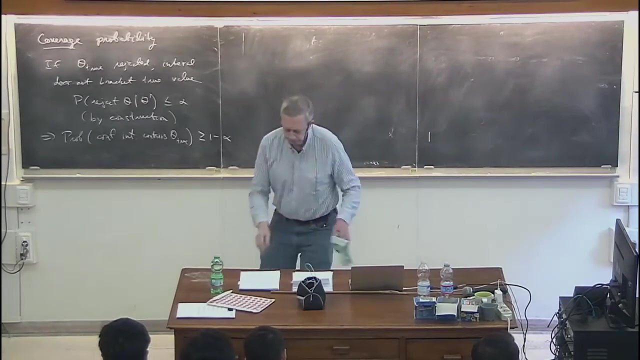 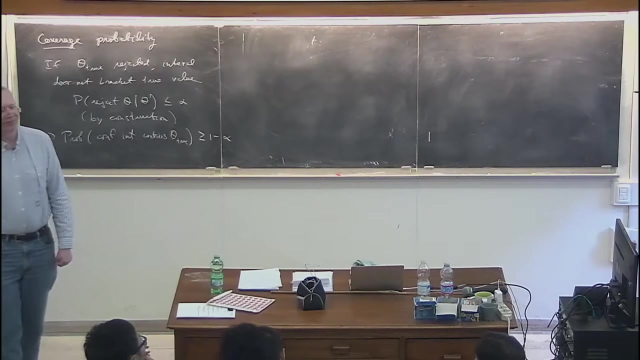 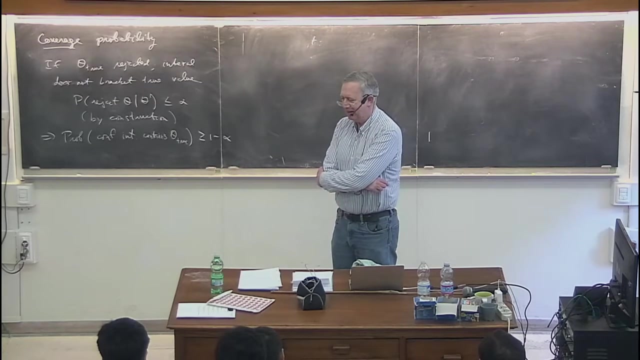 then this greater than or equals is just equals. The greater than comes about in the case when we have discrete data. Okay, so let's do an example Right? So the way that you phrased the question is very good That I should refine this. 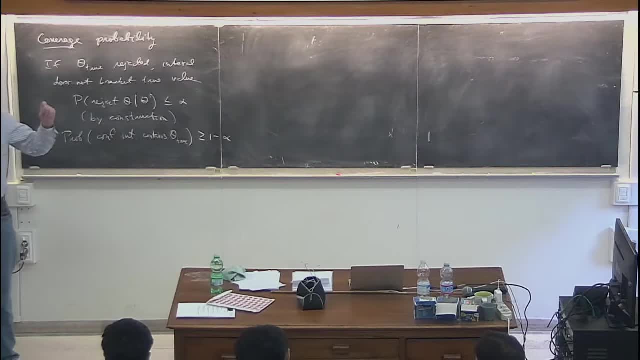 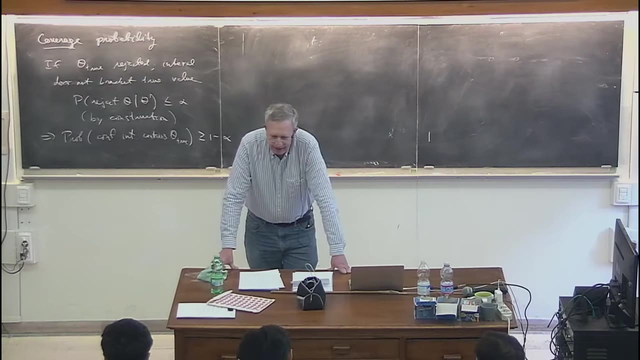 The problem, The probability, that I will assume that, within the considered values of theta, that one of them is true. That is to say, I assume that, amongst the hypotheses that I Consider This is a very well-posed question- What we can say, for example, 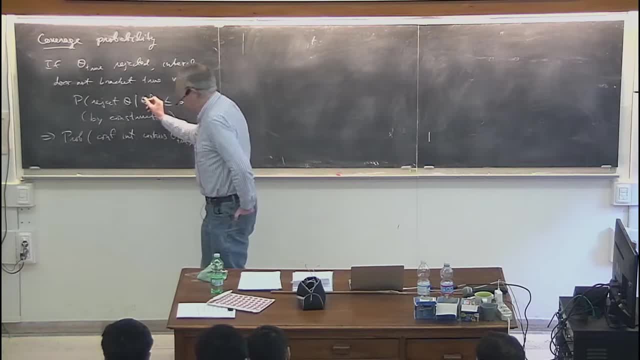 is that, Under assumption that the Higgs does exist and that its mass is a certain value, the probability that we reject it has to be less than alpha. So that means that if we assume that the Higgs mass takes on some true value, 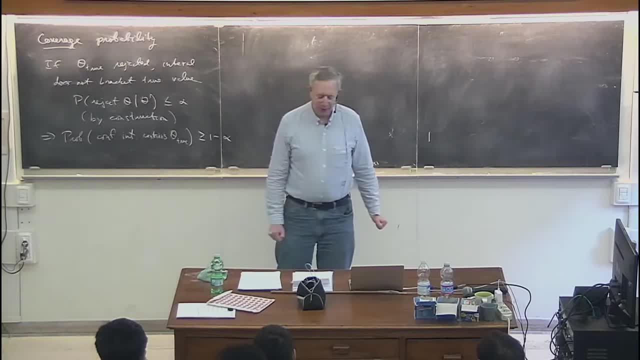 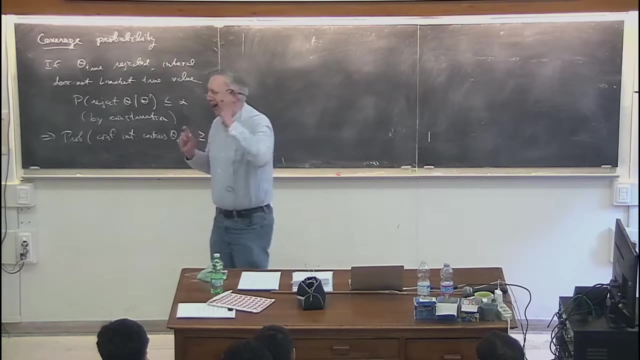 then the interval has to cover it with a probability equal to the confidence level. So I guess I have to qualify that with that caveat. That's correct. Yeah, good point, But we are going to see. The reason I hesitate there is that we're actually going to see situations. 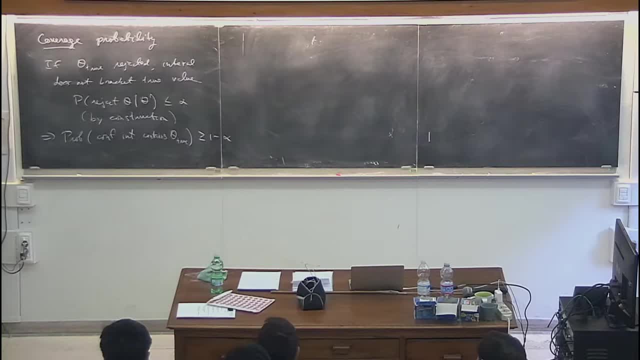 where you can consider a set of parameters And for certain values of the data you will in fact get a p-value less than alpha for all hypothesized values of the parameters. So there will be situations where we can say that the interval didn't bracket the true value. 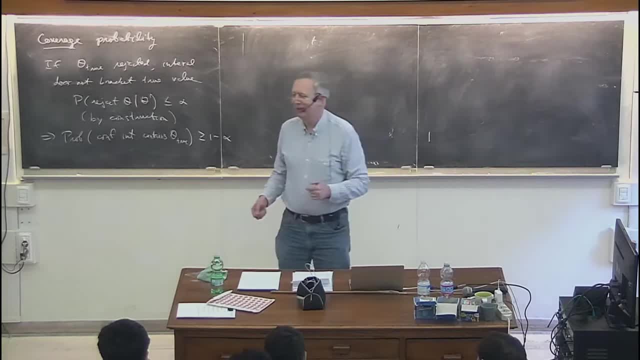 But that's a different situation from what you're saying. You're saying: suppose that the entire theory is wrong. So no, that's not true. No, I'm assuming that the form of the theory is correct and that there's a true value somewhere in the space. 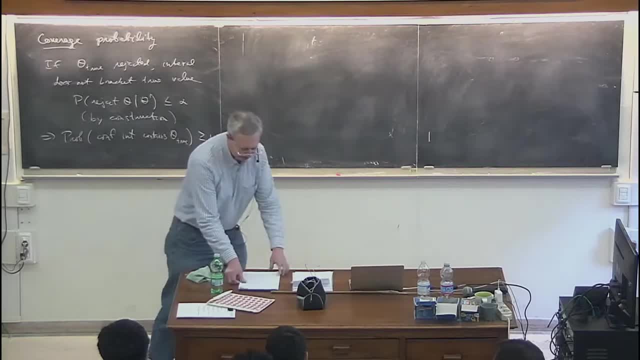 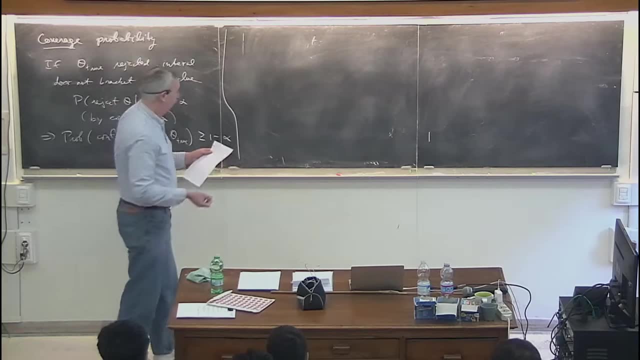 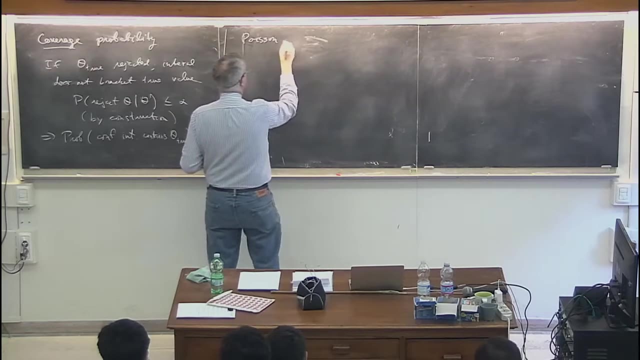 Okay, yeah, Right, Let's do an example now. So one of the most important ones in particle physics is this Poisson counting experiment, So the Poisson counting which we've already seen. I assume that the data value that I get in my experiment 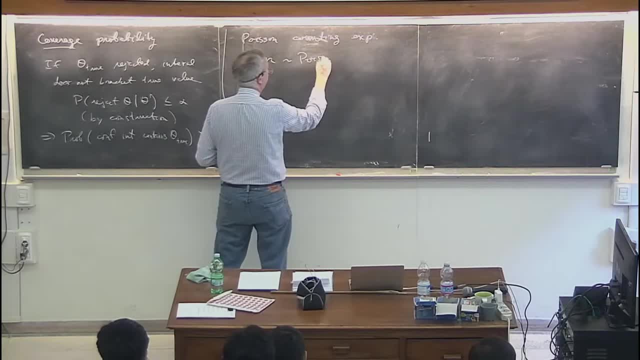 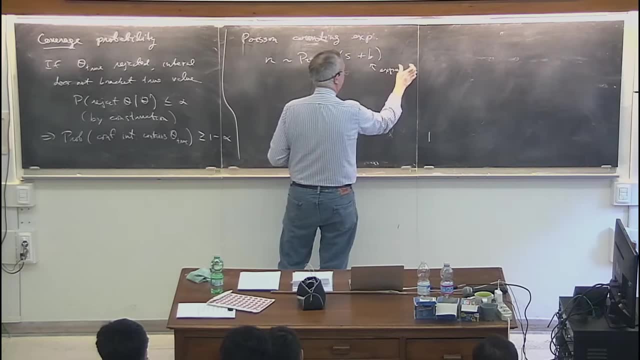 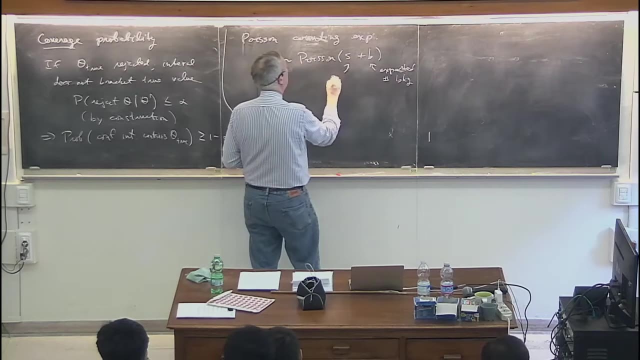 is a number n and that follows a Poisson distribution with a mean of s plus b, where that's the expected number of background events and that's the expected number of signal events, And I'm going to assume that b is known. 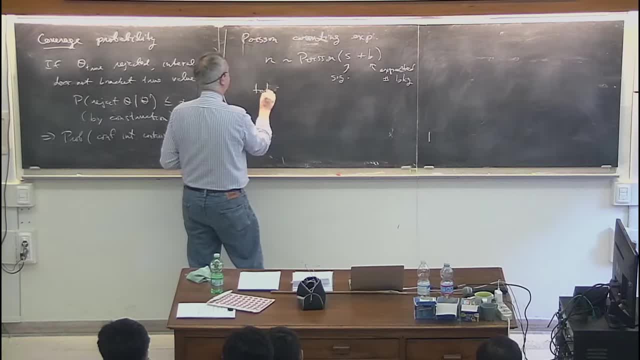 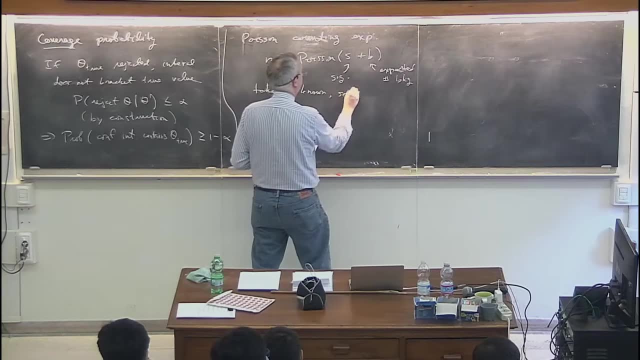 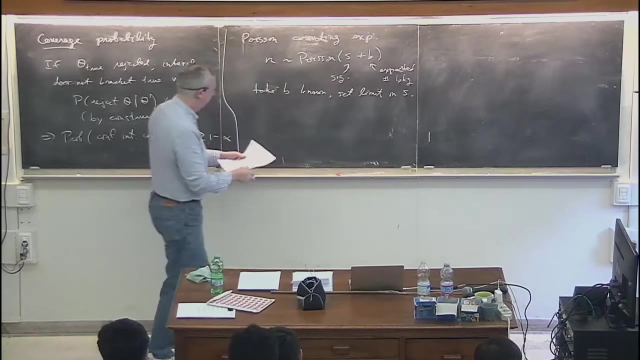 and I want to set a limit on s. And so let's see, In this example I actually have some numbers. Let's suppose that b is equal to 4.5, and let's suppose that n observed is equal to 5.. 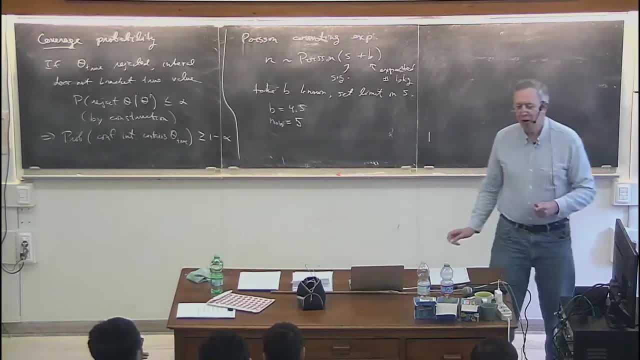 Now these are almost the same numbers that we saw in the example yesterday, when I said: suppose that b was 0.5 and n was 5.. And then the immediate thought was, ah, it looks like we've discovered a new signal process. 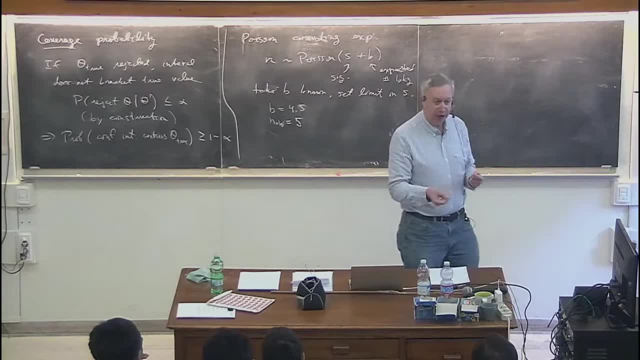 and what we did is we tested the hypothesis that s is equal to 0, and we gave the p value for that. But now suppose the expected background is not 0.5,, it's 4.5, and you observe five events. 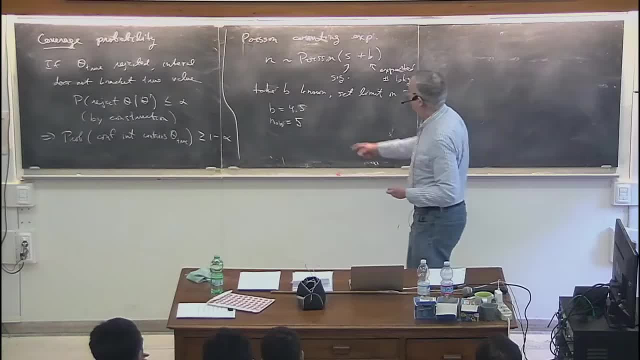 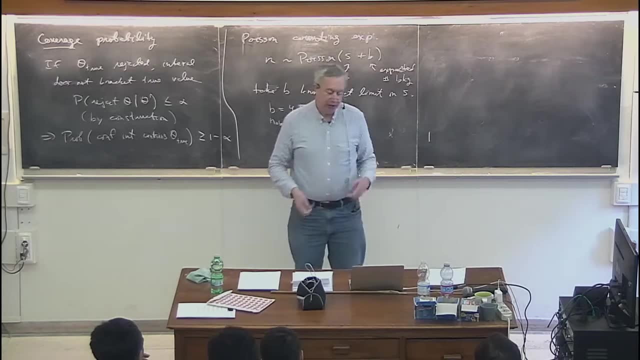 Well, that seems perfectly compatible with the hypothesis that s is equal to 0, so it's clear that we're not going to be able to establish a discovery. If you were to compute the p value, the probability say, assuming s is equal to 0,. 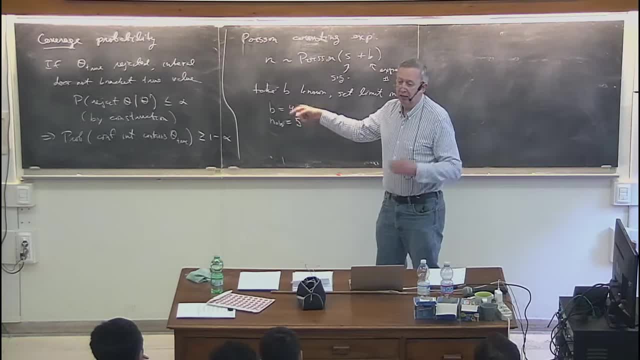 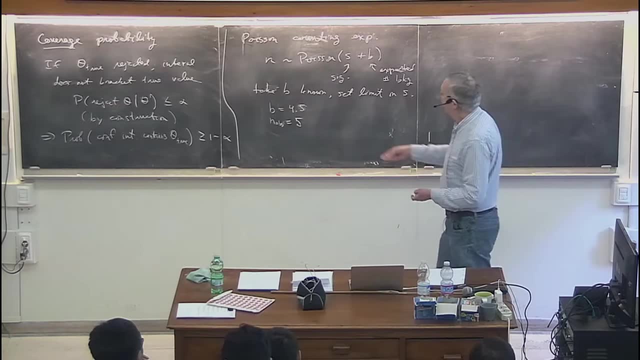 to see 5 or more. given a mean of 4.5,, that's going to be something like a little less than 50%, And so you wouldn't reject that hypothesis. On the other hand, how about very high values of s? 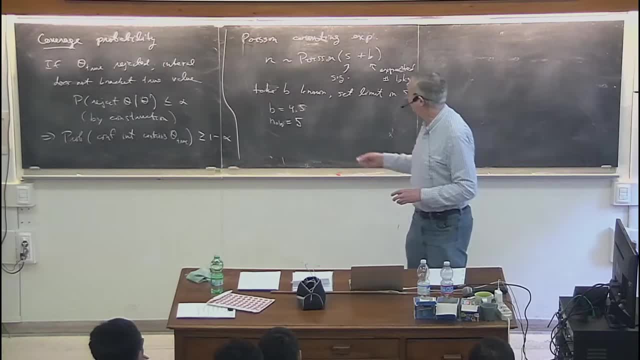 Are they compatible with this outcome? All right, how about? s is equal to 30?? All right, so that s plus b would be 34.5.. And we saw five events. Well, no, that's clearly too high. That is to say, the predicted rate is very high compared to what we've observed. 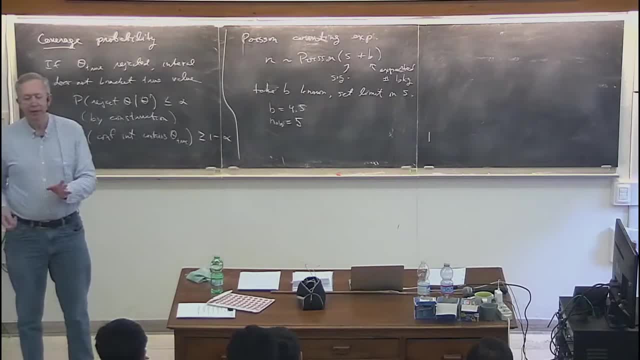 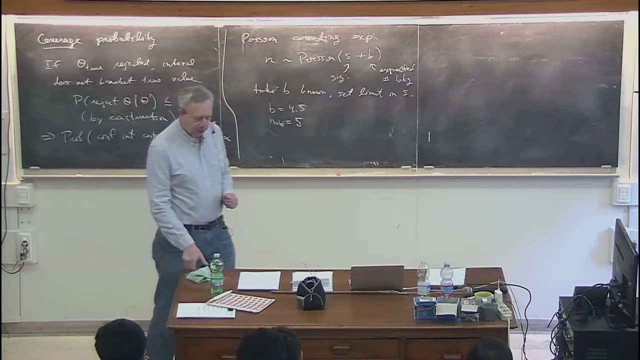 And so that's the idea. now We want to test different values of s to see that, if we can exclude them on the basis that they were too high, So try to test high values of s. What's the alternative to a high value of s? 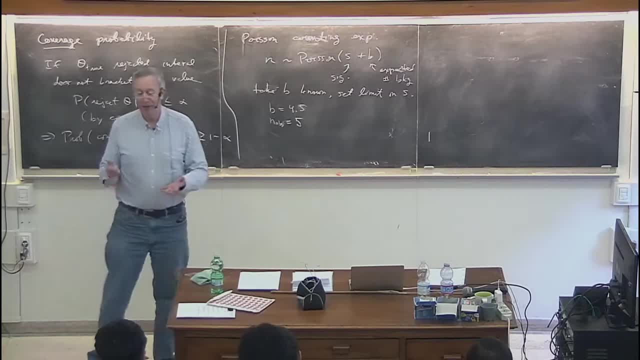 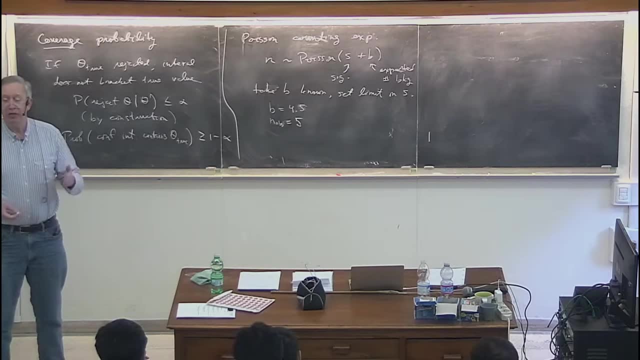 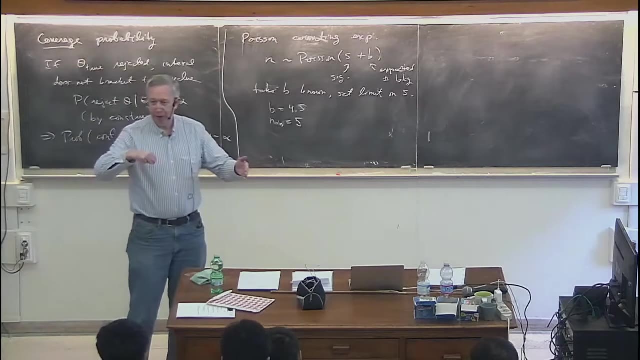 A low value of s. All right, so the relevant alternative hypothesis in this case would be low s, or say s is equal to 0. And so that means that the region of data space that constitutes lesser compatibility compared to the hypothesis that I'm testing. 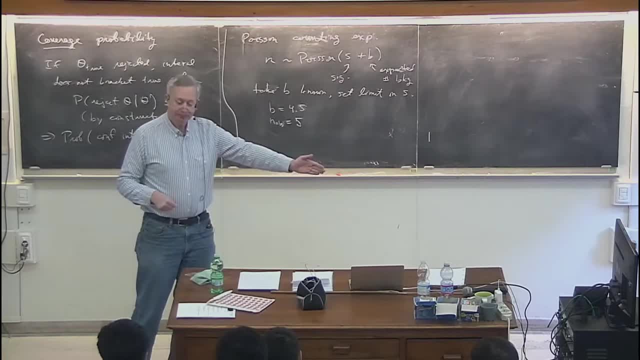 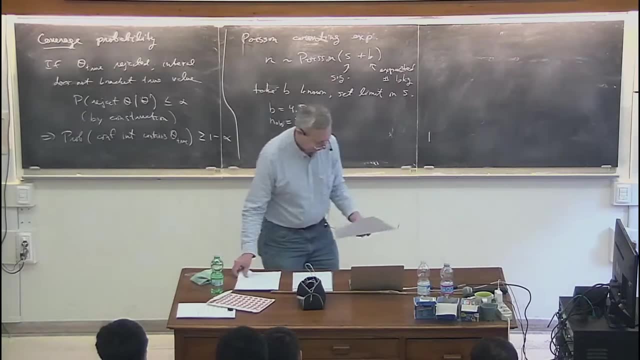 that's going to be the region of data values that are low. All right, so I just have my sheet of paper, Right, sorry. So that means we're going to do the following: We're going to say that the p-value of a hypothesized value of s 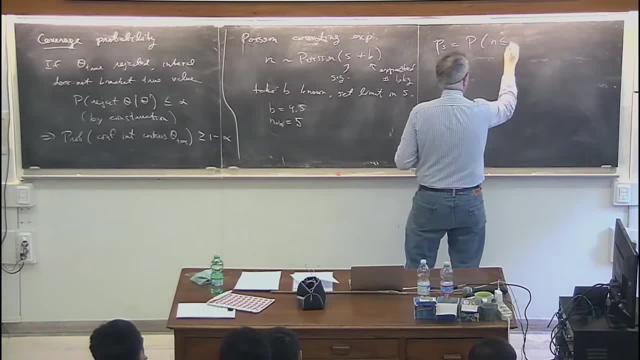 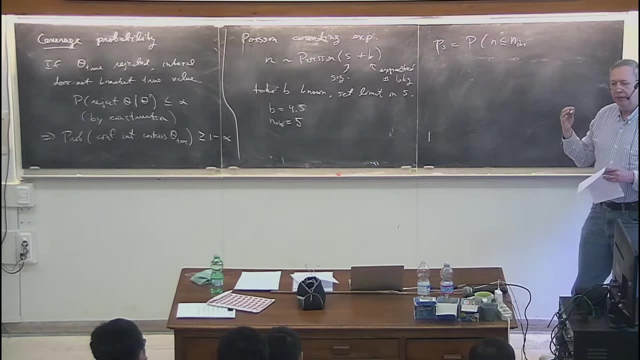 that's going to be the probability to see n less than or equal to the number of events that I observed. I take the low values as the values that now constitute lesser compatibility. Equivalently, I can say that I will put the critical region of the test. 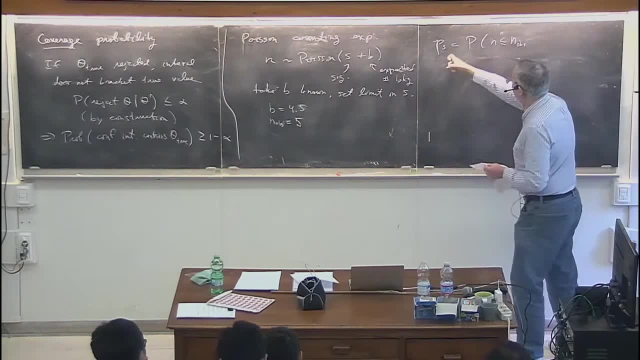 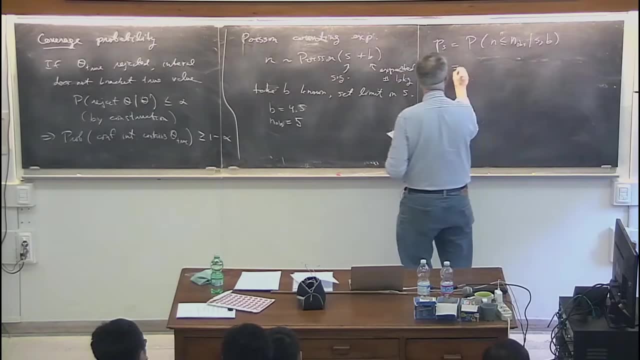 at the low values of n. All right, and so I'm going to test a value of s. That's why I have that subscript, And so this is the probability for s and b, And so, of course, this is just the sum from n equals 0. 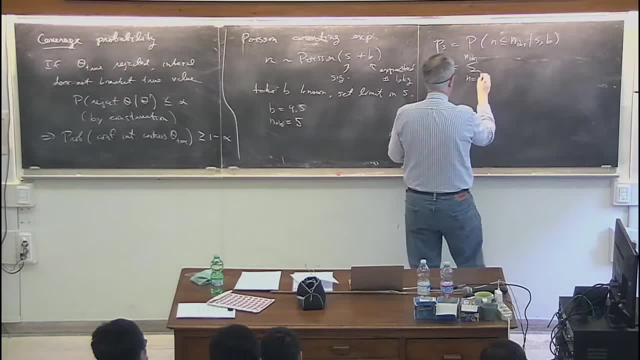 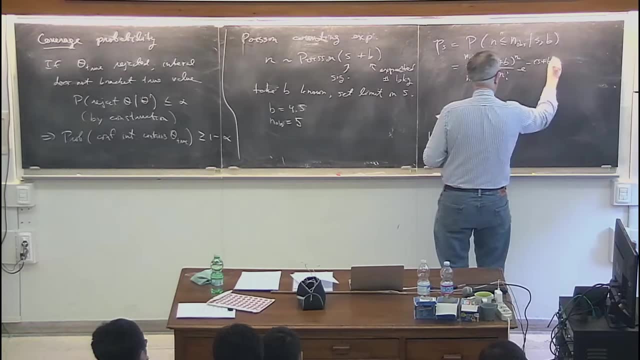 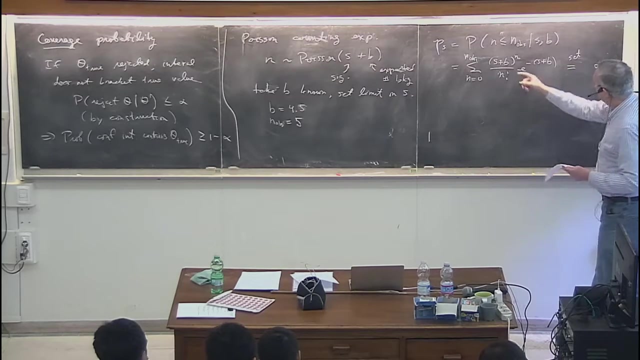 up to the observed number of the Poisson probability. All right, and so now all we have to do is to set this p-value equal to alpha and solve for s. So we want to set this to alpha- All right To alpha- and solve it for s. 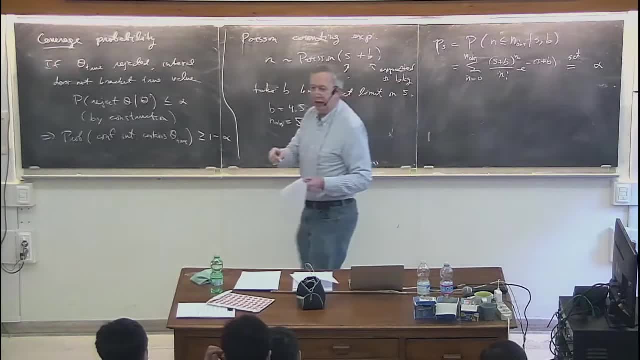 And here there's a trick which, if you look- I don't know if you've had a chance to look at the I think it's in problem sheet number 2, that's on the web page- There's a trick for summing these Poisson probabilities. 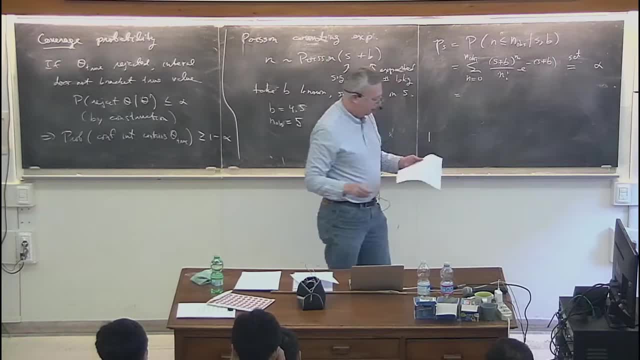 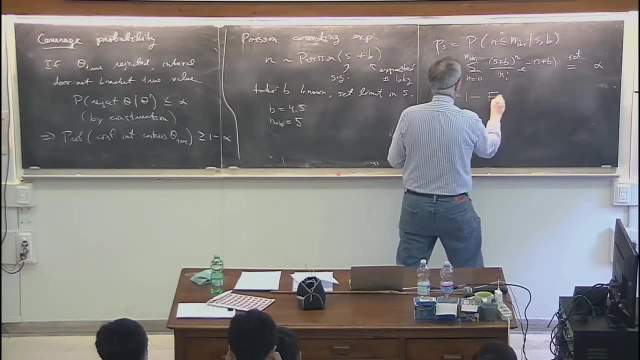 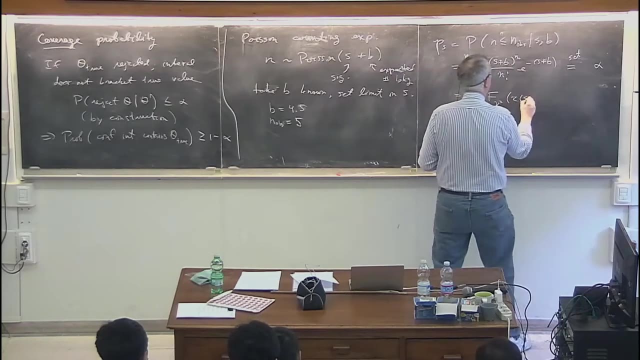 in which you can relate them to the cumulative distribution of a chi-squared distributed variable. You can show that this sum is equal to 1 minus the cumulative distribution for the chi-squared distribution of 2 times. whatever the mean is here, Which is s plus b? 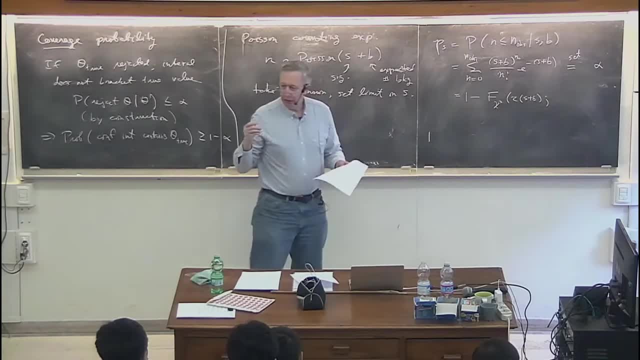 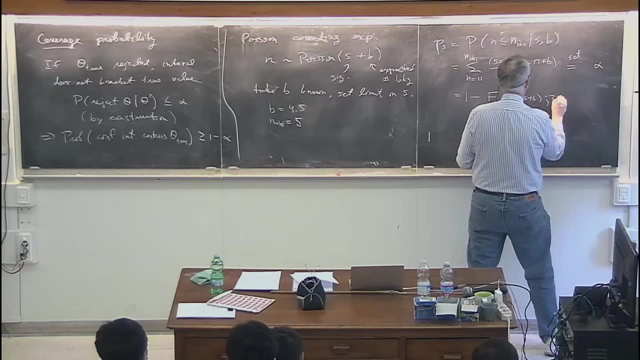 And then the chi-squared distribution has a discrete parameter, which is the number of degrees of freedom, And the number of degrees of freedom you need to use is equal to 2 times the upper limit of the sum here plus 1.. That's just a mathematical identity. 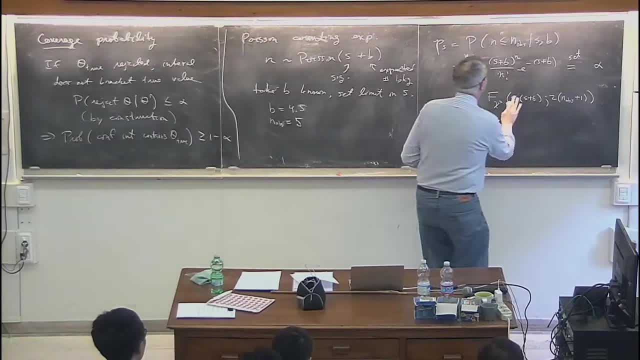 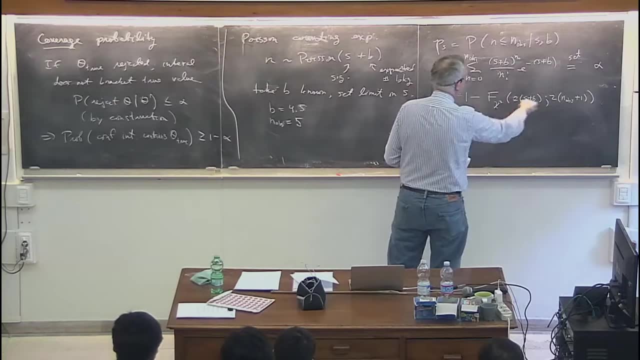 And so I'm not going to. I don't know how to derive that. We have to think very carefully about how to do so. It's quite obscure, But it's just a mathematical identity that allows you to do this sum and express it in terms of a function. 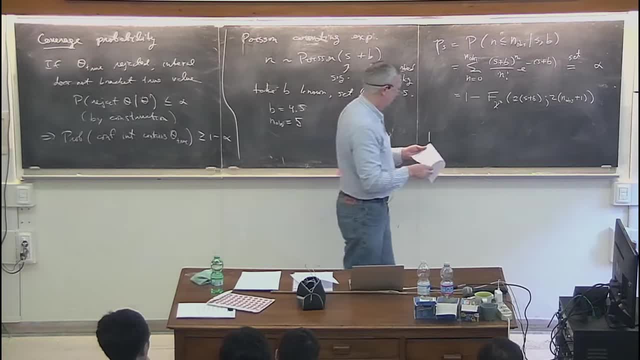 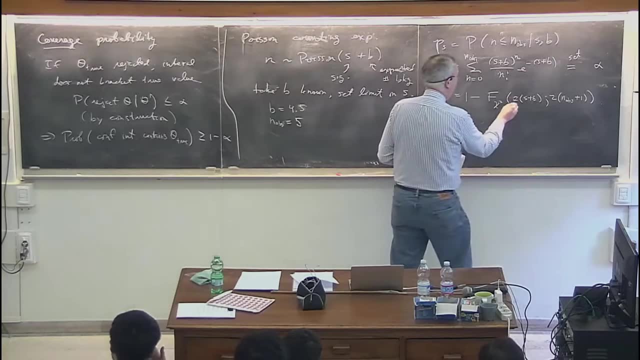 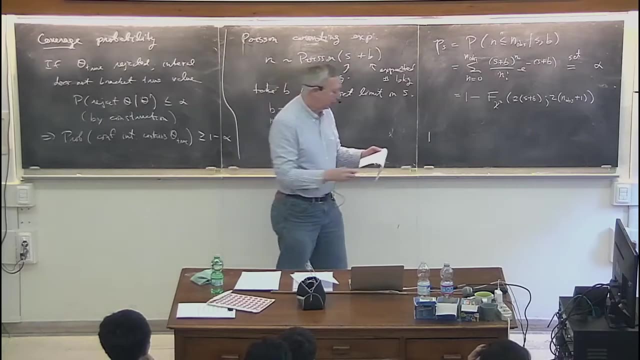 that we can access through some computer library. No, no, it's identical, It's exact. And so if you set that equal to alpha and solve for the cumulative distribution, I can then just take the inverse of the cumulative distribution on both sides, and so that allows me to solve for s. 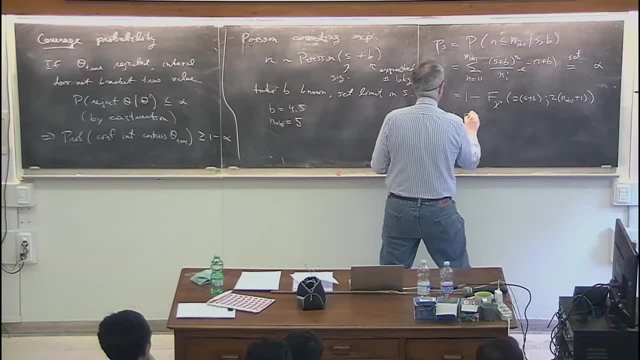 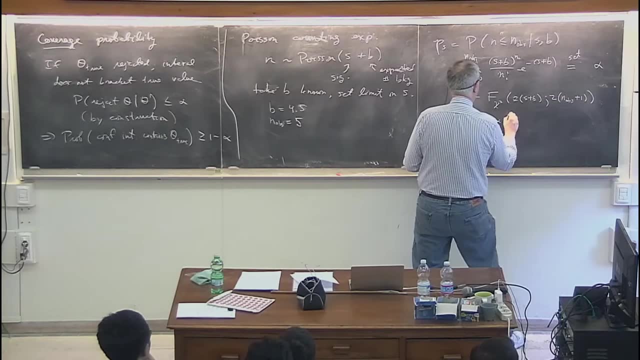 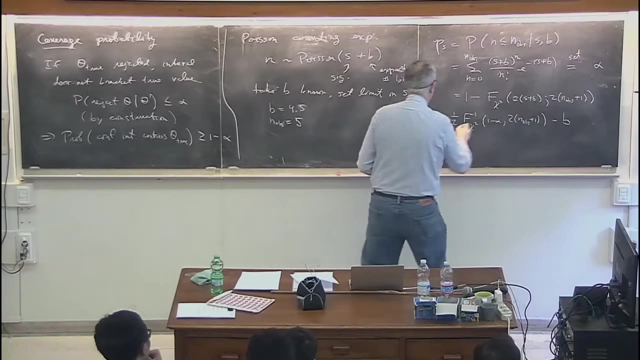 And I get 1, half times the inverse of the cumulative distribution. So that's called the quantile right: 1 minus alpha, Same number of degrees of freedom, obviously Minus b. And so once you solve for s, that's the value of s, that gives you the p-value just equal to alpha. 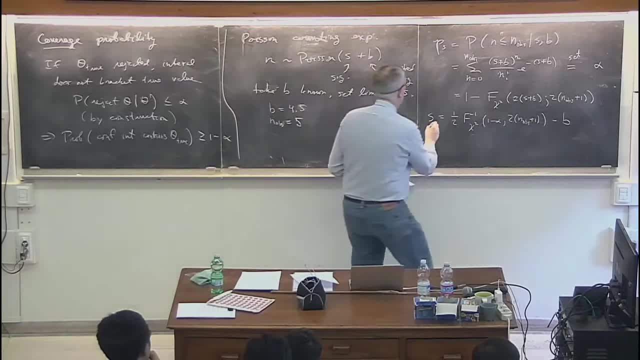 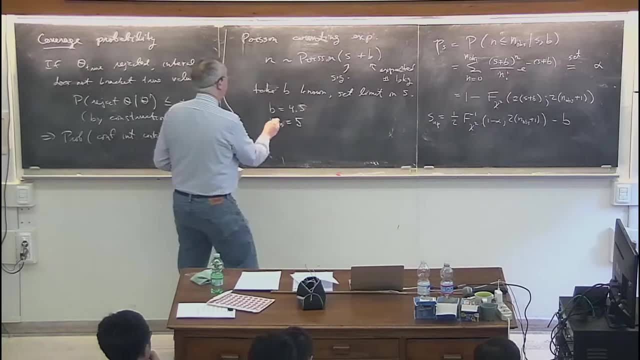 And so that's the limit, That's the boundary of the interval, And so I'll call that s sub up. That's the upper limit, Alright, And if you put in the numbers that I put in here, b is equal to 4.5. 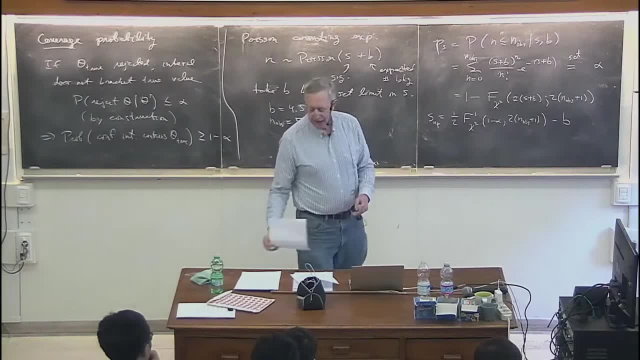 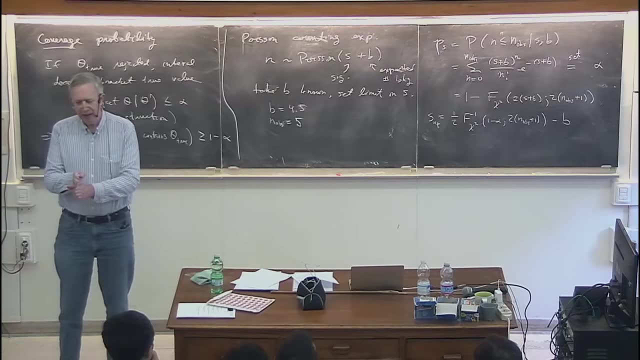 and n observed equals 5.. Before I put in the numbers, let's just take a guess. What do you think is the hypothetical value of s such that I would get only a 5% probability to see 5 events or fewer? So remember that b is 4.5. 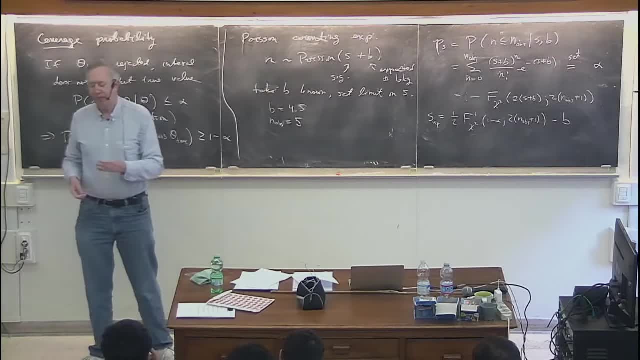 and I have to add s and b. So you can imagine what's a Poisson variable, mean value such that I would only get, say, 5 events or fewer, Maybe a dozen or so, If the mean of a Poisson variable was a dozen. 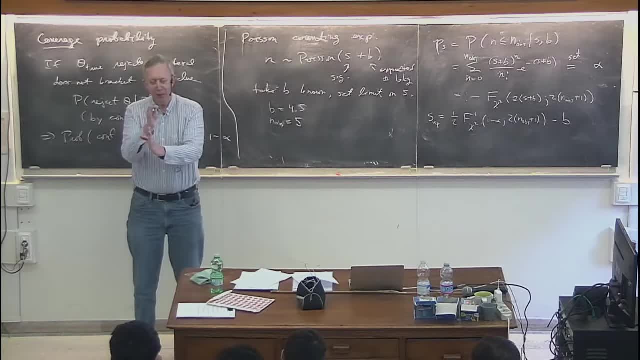 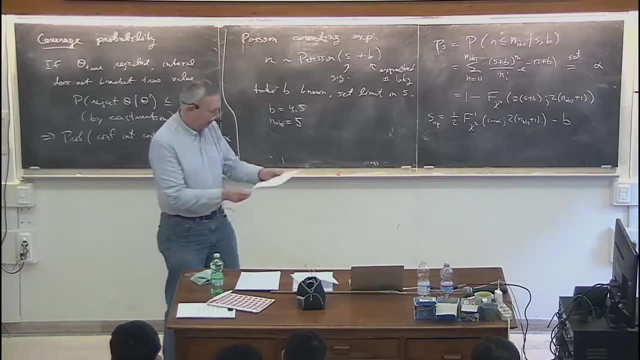 then you can imagine it would be distributed about 12 and maybe very rarely it would get down to 5 or below, And that's actually very similar to what I get when I do this calculation. This turns out to be 6.0.. 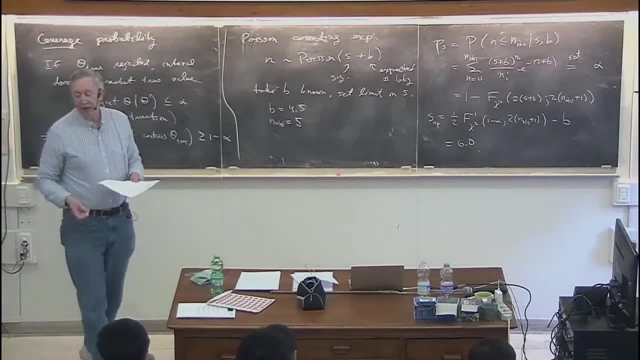 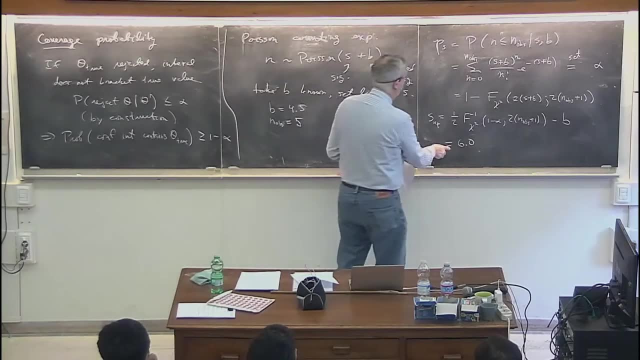 So it would correspond to a mean of the Poisson variable of 10.5.. So that's the way that you interpret the upper limit. The upper limit is the hypothetical value of the parameter, such that there is a probability alpha 5%. 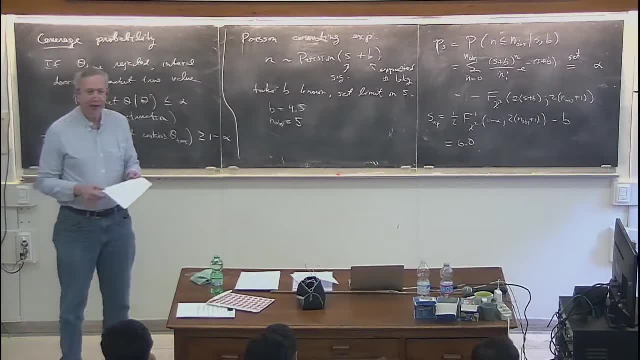 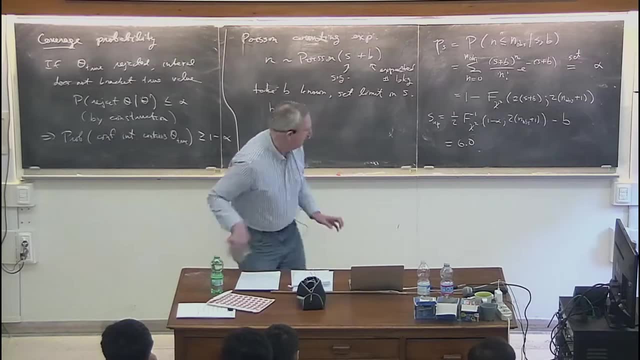 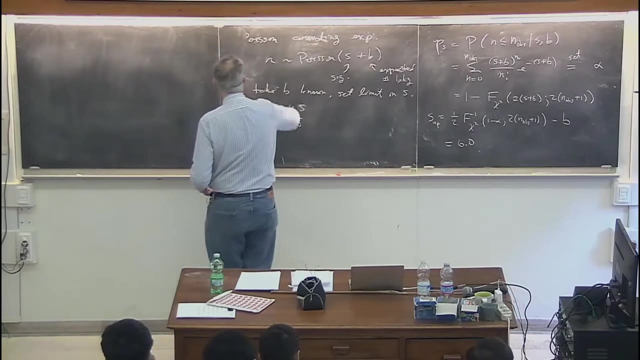 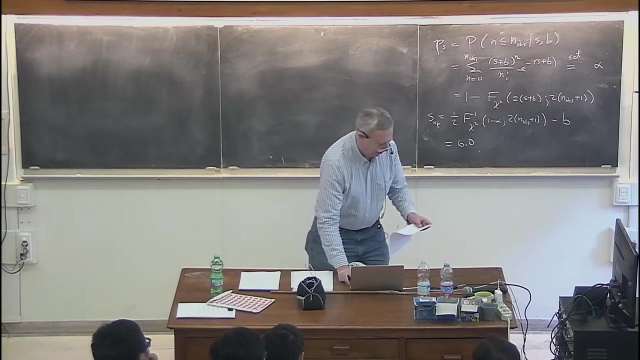 to get as few events as you found, or fewer. That's the way you need to think about a frequentist upper limit. So I have a. Is this the right page? I'm just going to sketch it. It's easier that way. 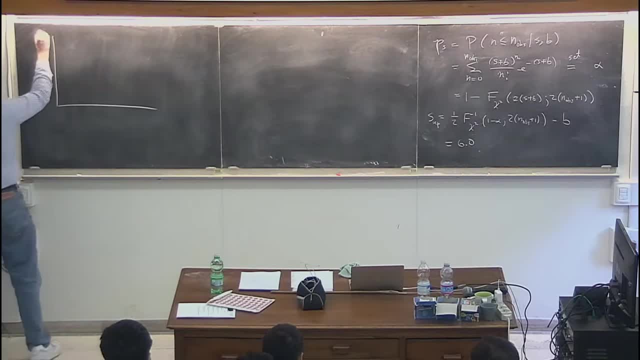 In the notes. there somewhere there's a sketch of the upper limit at a confidence level of 95%. So alpha equals 0.05.. And what I've sketched is the upper limit as a function of b for different numbers of the n. 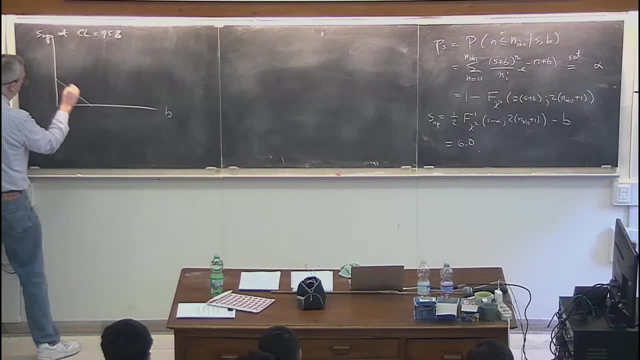 different numbers of the observed number of events, And it's a family of curves that looks kind of like this, And so this would correspond to n equals 0,, 1,, 2, and so forth, And there's a famous number here. 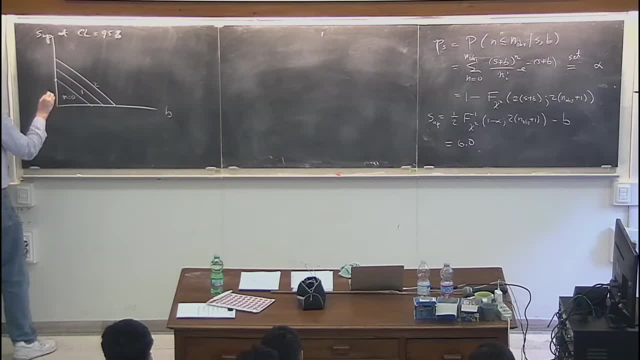 which is that if b is equal to 0 and you observe 0 events, what's the upper limit? at 95% confidence level, And it's about 3.. It's 2.99 something, but let's say 3.00.. 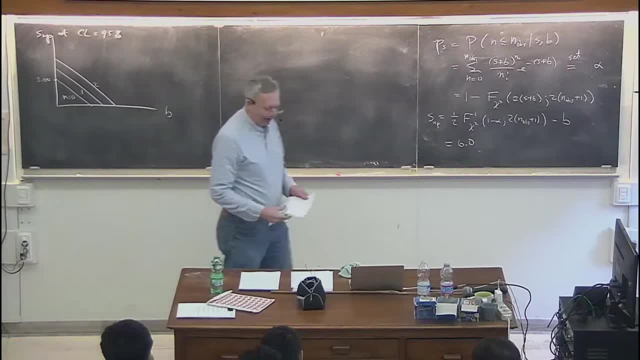 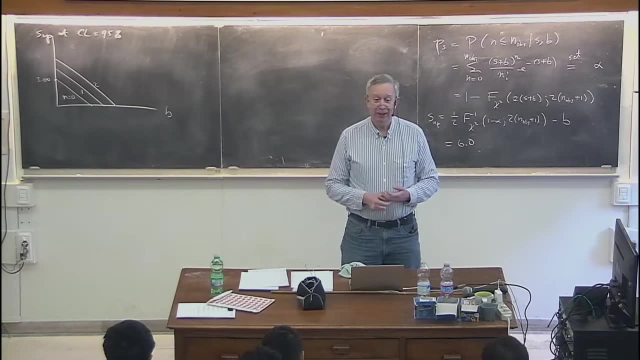 I think it rounds to 3.00.. And that's kind of a famous number that almost everybody who deals with these things has in memory, And so a classic example would be something like proton decay. And so in a proton decay experiment like Super-Kamiokande, you've got your humongous tank of protons water and you stare at it for a year and you see if any of them are going to decay And the expected number of background events is very low. It's not identically 0, but it's much less than 1, say. 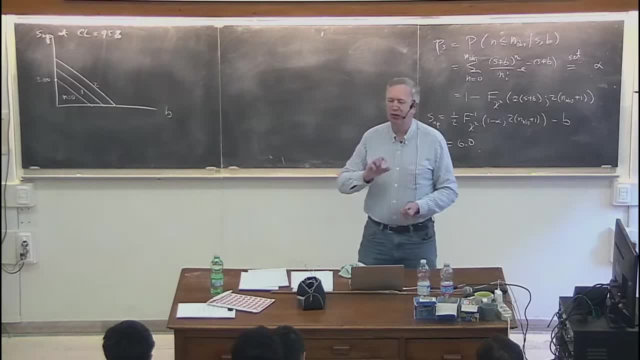 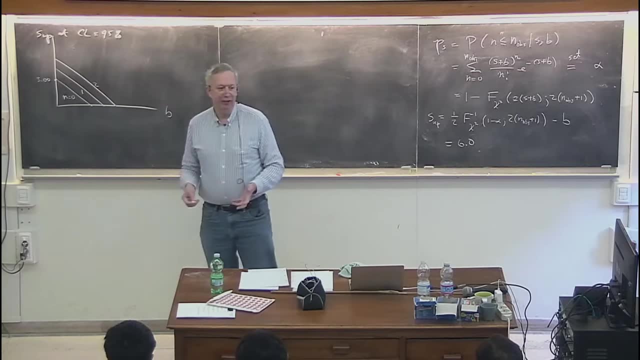 And so you look at this tank of water for a year and you don't see anything. You see 0 proton decays. So the question is then: does that mean the proton decay definitely doesn't exist? No, Maybe you got unlucky. 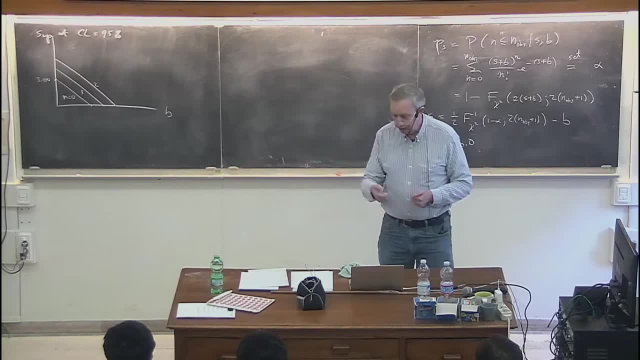 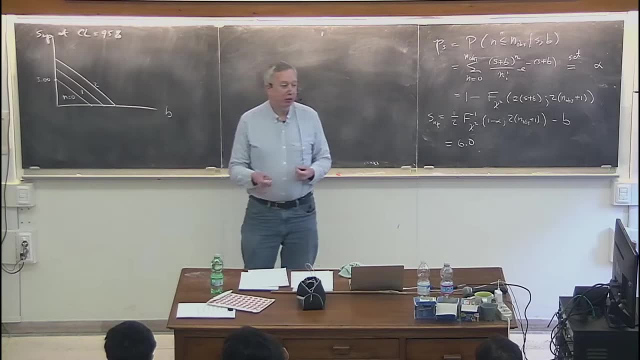 Maybe your proton decays once every 5 years and during the year that you looked, you just happened to see none. So you need to set an upper limit. Set an upper limit on the expected number of proton decays in a year. 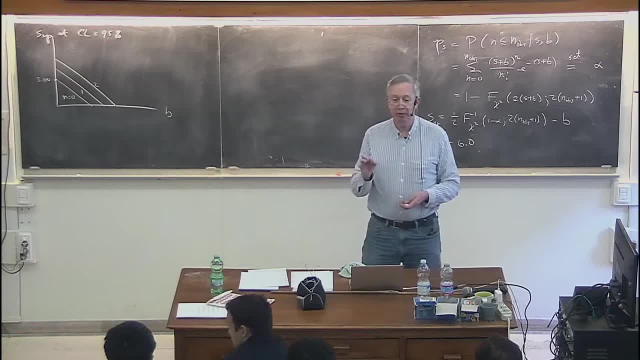 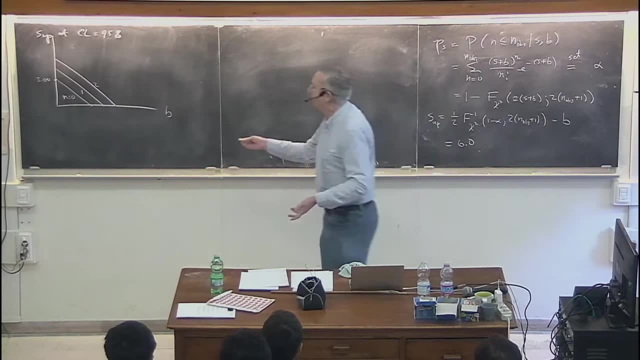 And the way that you would do that is you would say what's the hypothetical number of proton decays, such that I have a 5% probability of seeing 0? And that number turns out to be 3.. So that would be the upper limit. 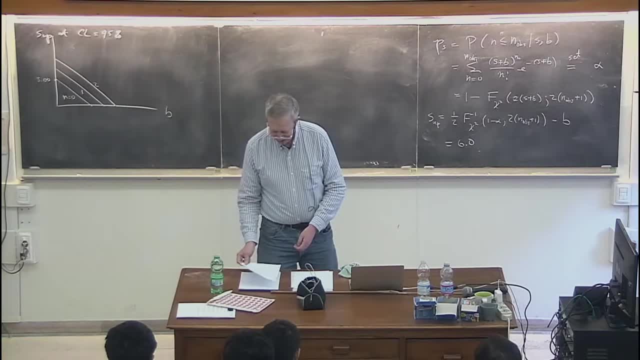 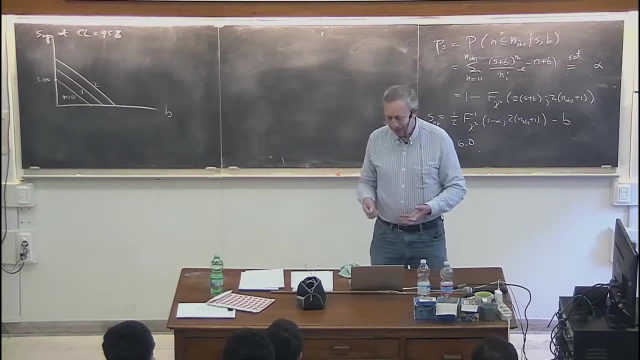 That's a number worth keeping in mind. What's kind of interesting is that that doesn't depend on the size of the water tank. Suppose you have a little tiny proton decay detector and you look at it and you see nothing. What's the upper limit? 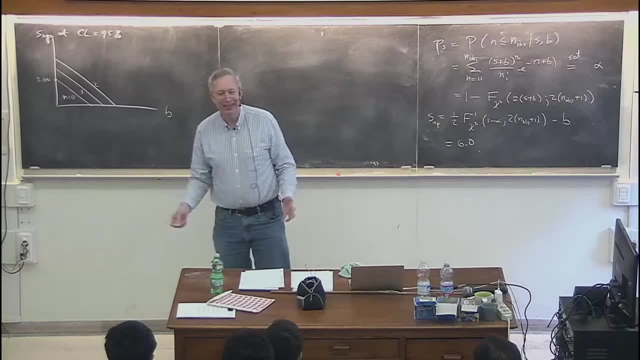 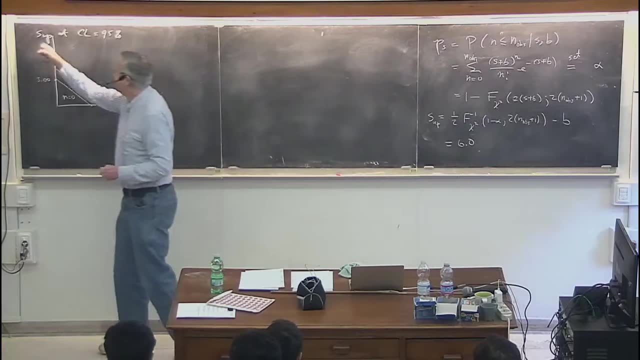 3. Suppose you upgrade with a huge budget a big proton decay detector. Still, if you see nothing, your upper limit is 3.. But obviously what you do is, once you have the upper limit on the expected number of proton decays, 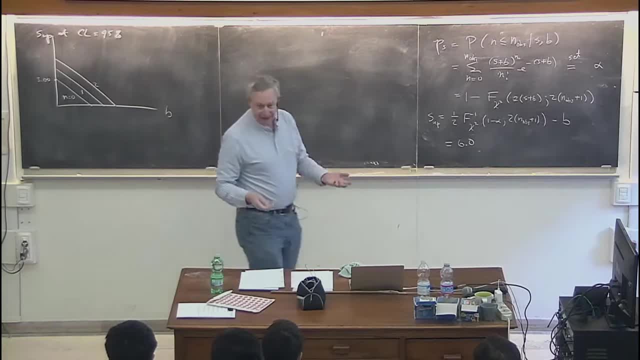 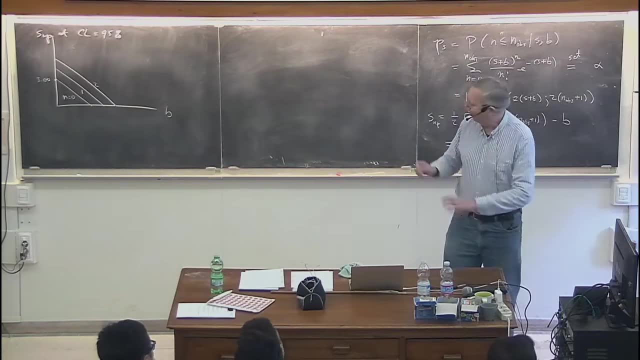 you convert that into an upper limit on the rate, the expected rate, And that of course, scales with the size of the detector? Yes, it will, obviously, But I'm assuming that I can neglect the background for purposes of just this discussion. 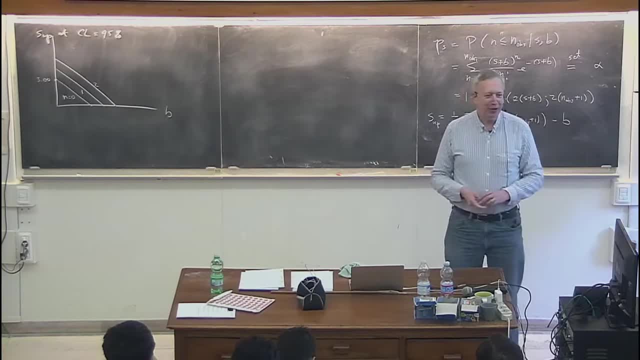 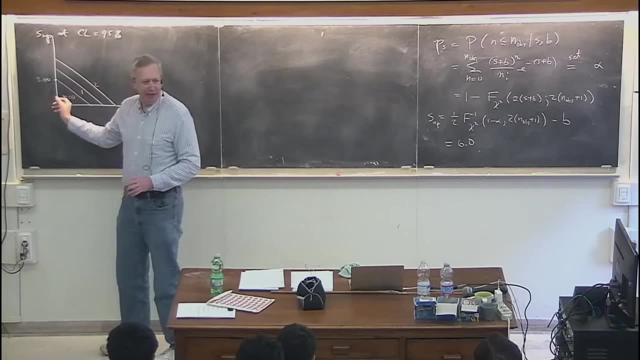 And even in something as big as super K, I forget. we can look up the paper, but the expected number of background events was 0.1 or something And they would take that into account. They don't actually report the 3.. 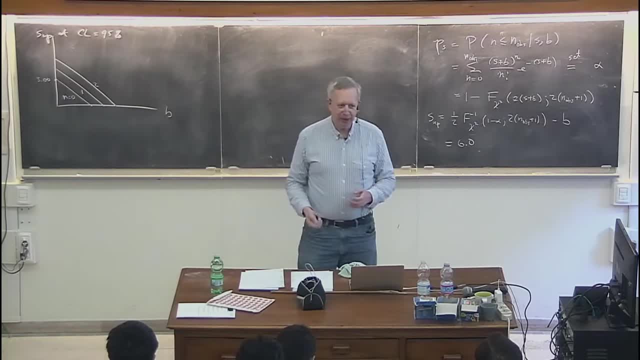 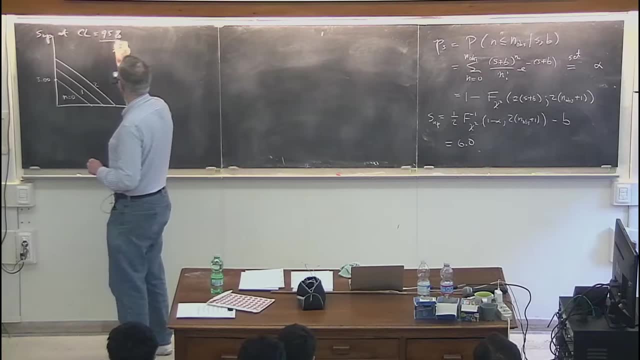 I mean they make the appropriate correction. But just to get a rough idea of what the limit is going to be if the background is very small, the upper limit is 3.. But this is the upper limit at 95% confidence level. 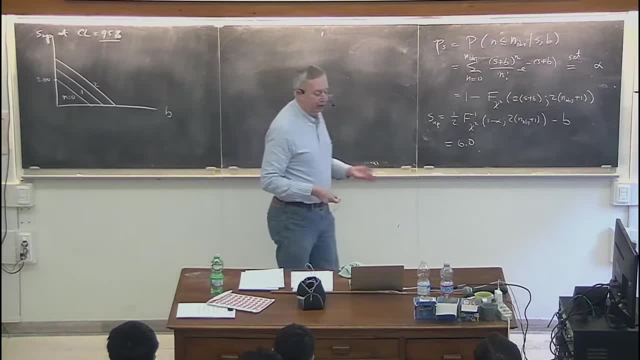 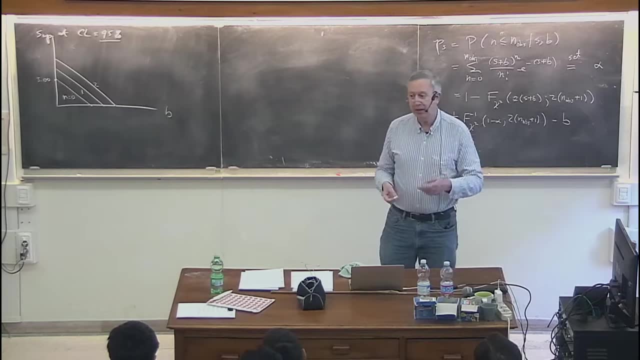 And that's a convention. That is to say, using a test size of 5%. that's just a convention, And in other fields you might use a different conventional number. In fact, in neutrino physics they may have switched. 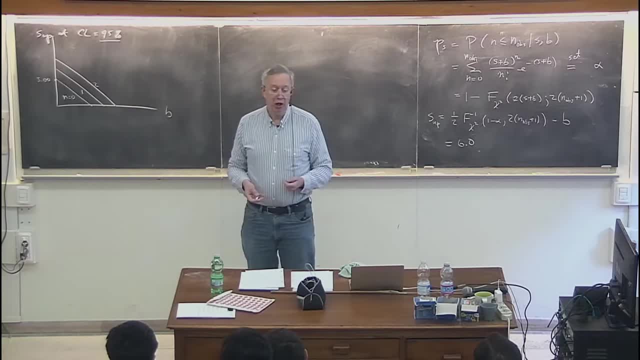 But for many years in neutrino physics 90% was more commonly used than 95%, So you can imagine what happens to this family of curves. if you were to choose 90% for the confidence level instead, Then you'd want to know the hypothetical value of the parameter. 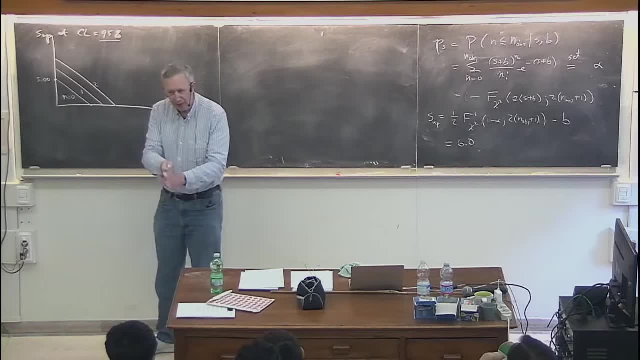 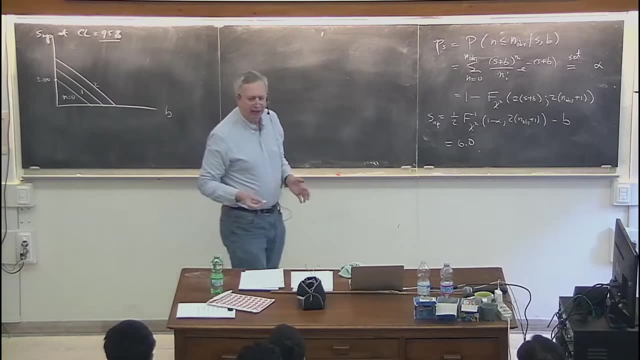 such that there's a 10% probability of seeing 0 decays or less. So the entire family of curves would just shift down. Instead of 3, it's something like 2.3,, I think, Because then you'd have a 10% probability of seeing 0.. 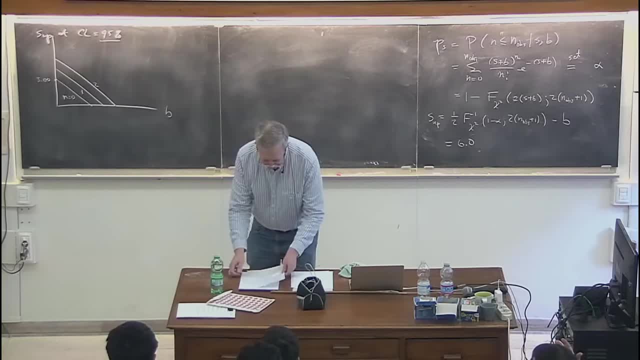 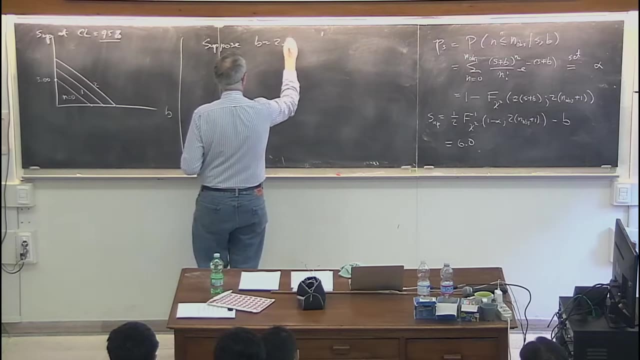 So that's just a convention. So now here's an interesting case that I'm kind of making up the numbers, but they're very similar actually to an actual case that happened. Let's suppose that b is equal to 2.5. 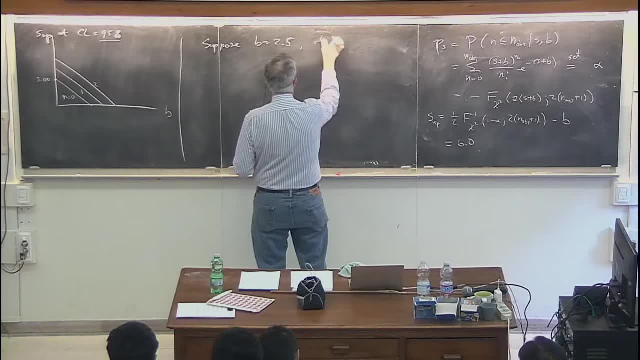 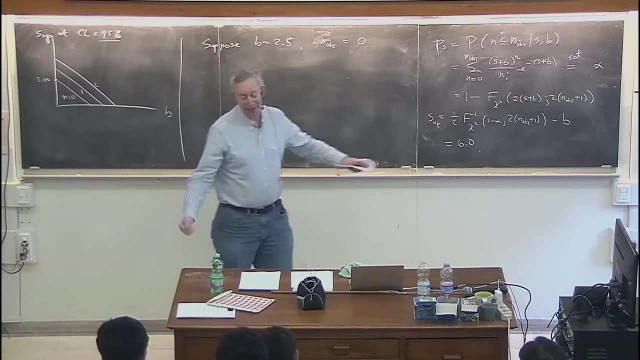 All right, You see, Should I write this: N observed equals 0.. That can happen even if you have an expected number of background events of 2.5.. You could observe 0.. And let's suppose that you're a neutrino physicist. 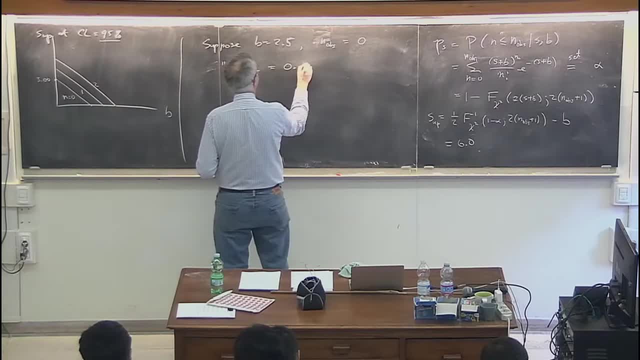 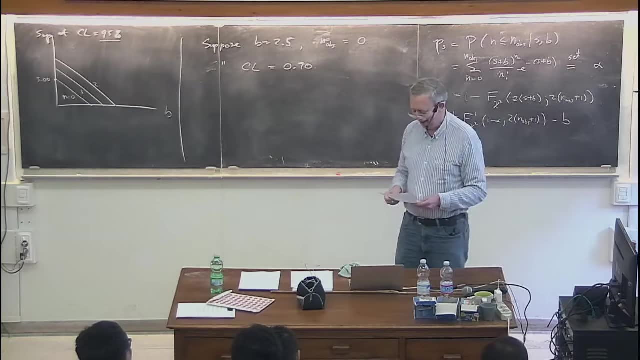 and so we take the confidence level to be 90%. I hope I get this right. I believe this was from the Karman experiment. It was a neutrino experiment And so if you take these numbers with 90% and you plug them into this formula, 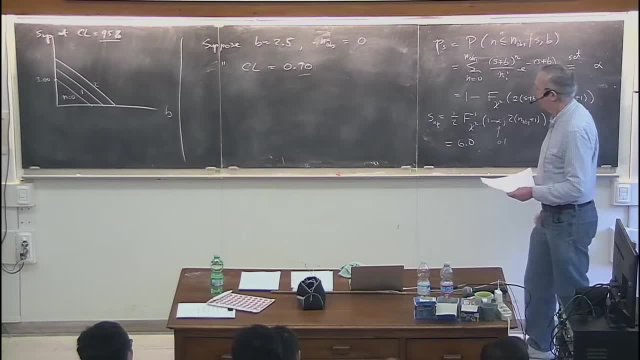 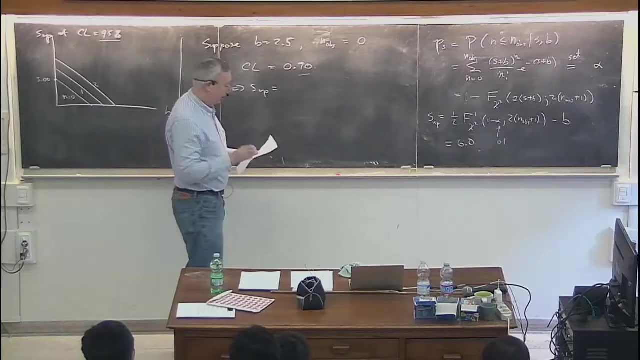 And so there I've got a 0.1 for alpha. in this case, That formula will give you the following result: It will say that the upper limit for x is equal to negative 0.197.. The question is: can I publish that number? 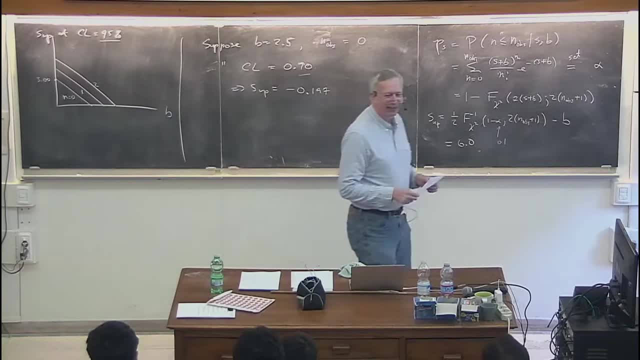 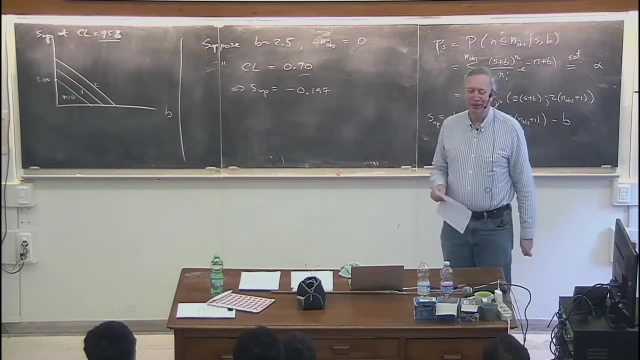 Can I use that number to summarize the outcome of my expensive experiment? I mean, obviously, before I started, before I spent anything, I knew that s was greater than or equal to 0. Maybe it is 0. But I'm not considering negative values as relevant. 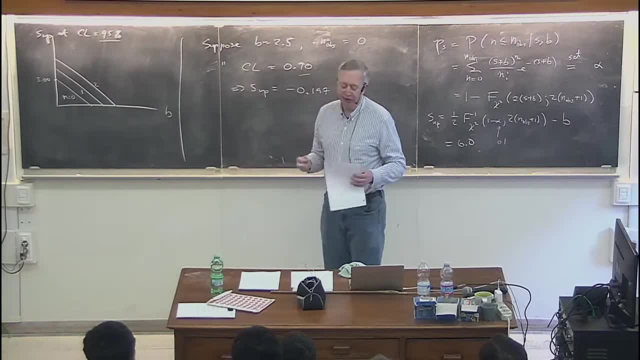 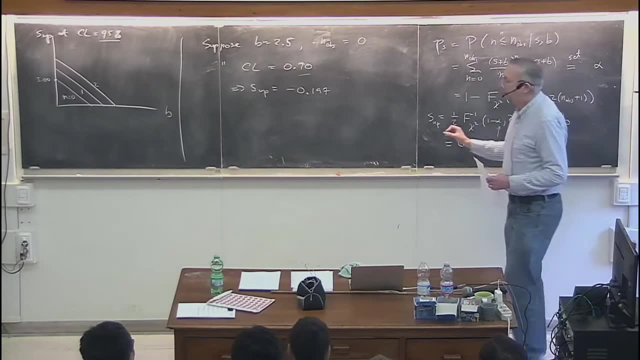 By the way, I should just say that it doesn't mean that the procedure is somehow giving you a negative limit. It means that this formula is giving you a negative number. What you're doing here, of course, is you're testing all values of s. 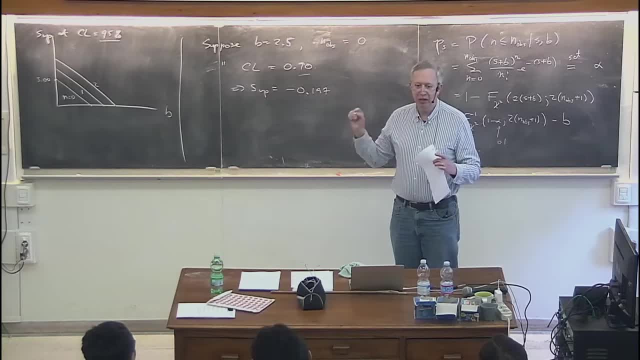 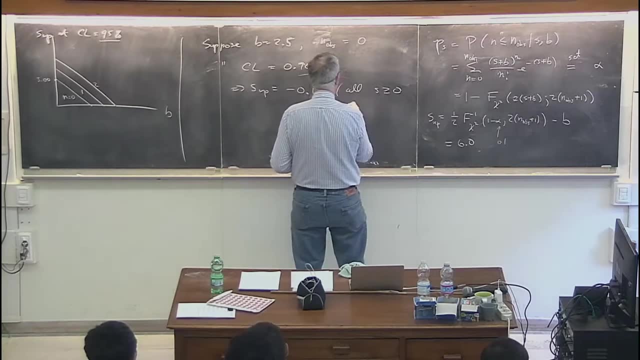 from 0 to infinity, And all of those are coming back with a p-value less than 10%. So what this really means is all s greater than or equal to, 0 have a p-value less than 0.1, less than the alpha that we chose. 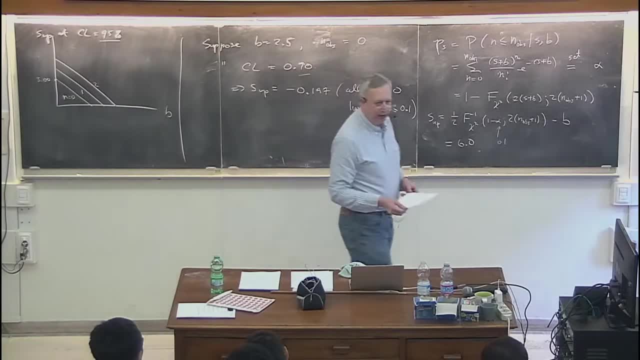 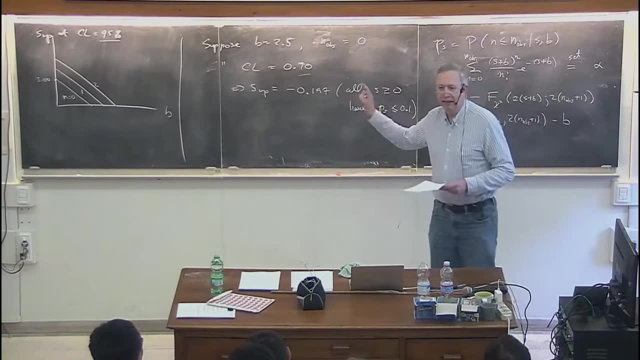 And so the physicist is all frustrated and says: this is impossible, I can't publish this. That would be laughed out of the community. But the statistician would then come back and say: look, this is working correctly. The procedure is working correctly. 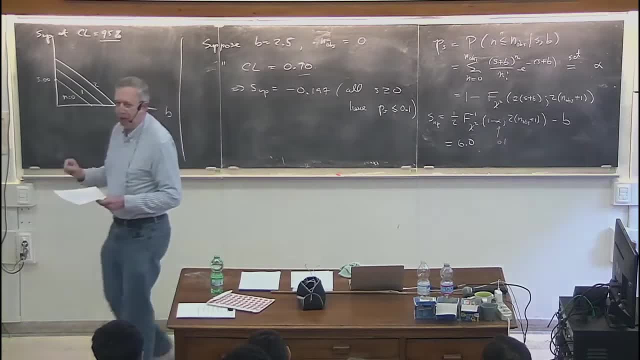 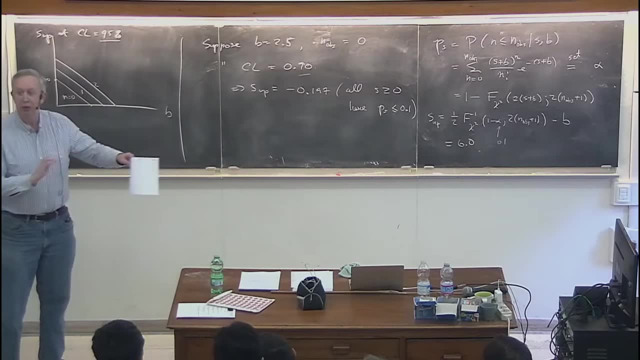 It was designed to bracket the true value of the parameter with a probability of 90%. That means that in 10% of the cases the interval has to exclude the true value of the parameter. And here your interval, which goes from minus infinity. 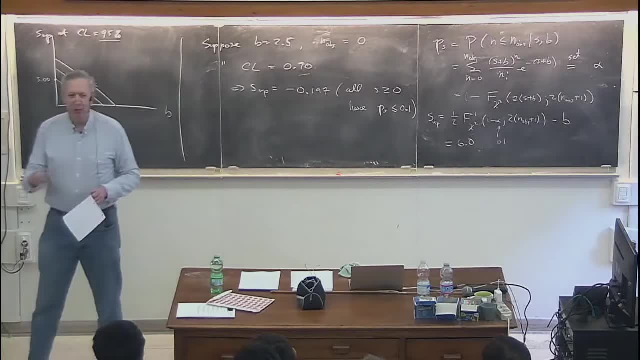 to negative 0.2, obviously missed. So you're one of the 10% that makes the whole thing work, And that's kind of interesting that sometimes, after having seen the data, you can know whether or not your interval includes the true parameter or not. 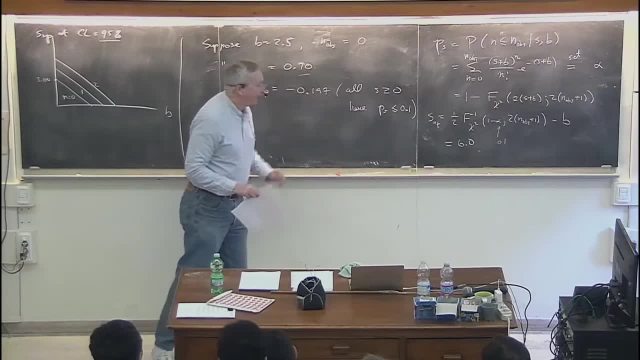 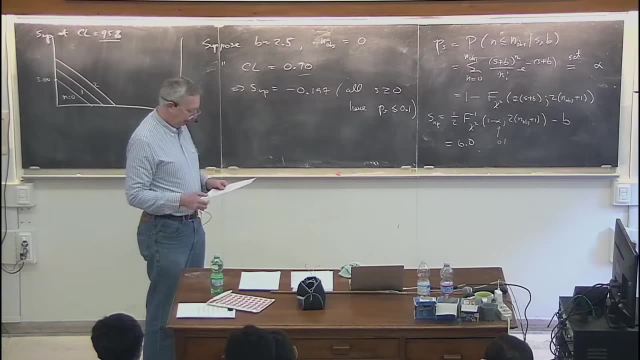 You can't always know that, but in this particular case, where you've excluded all values of s, then what you can know is that your interval certainly doesn't include the true value. You get a so-called null interval. And so then the tricky physicist might come back and say: 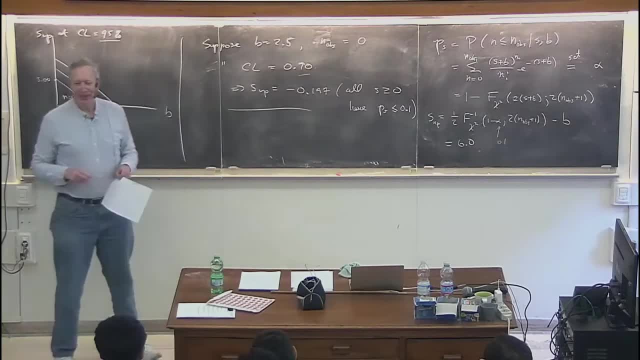 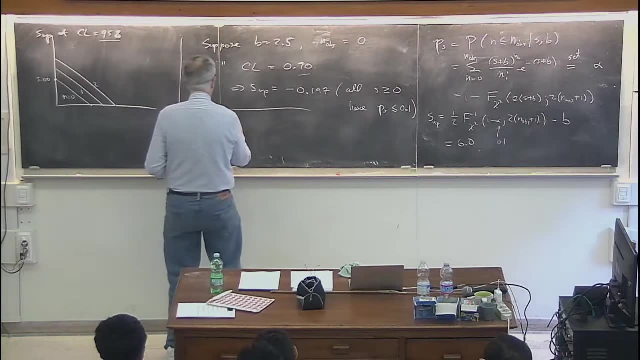 ah, these machinery physicists, They use 90%, But the guys across the hall in Atlas and CMS they use 95%. So maybe I should just do that. So if I try, cl equals 0.95, then of course what happens? 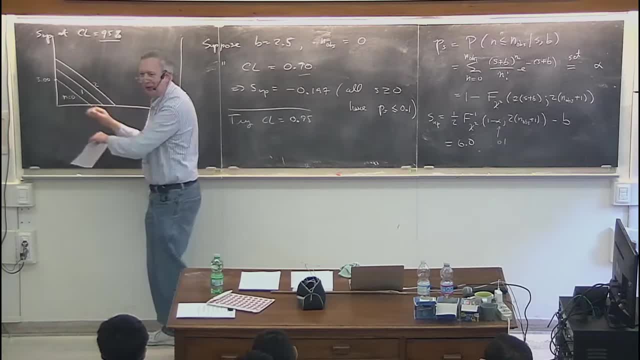 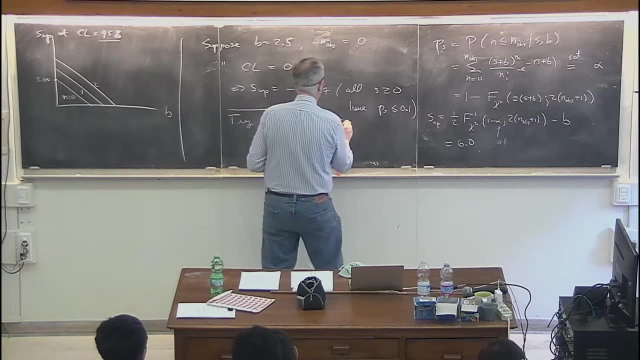 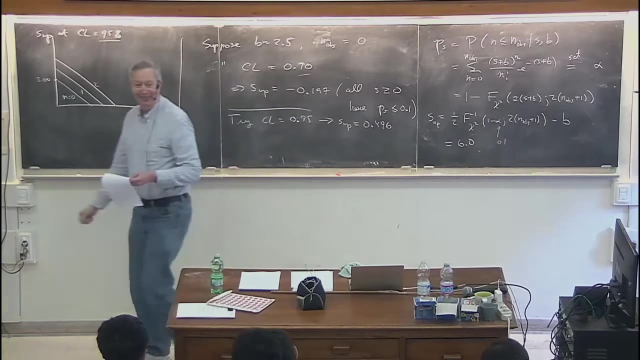 is that the entire series of curves shifts, And in fact it would shift in the direction that helps this guy. You get then the following number: an upper limit of 0.496.. It becomes positive. So now the physicist is very happy. 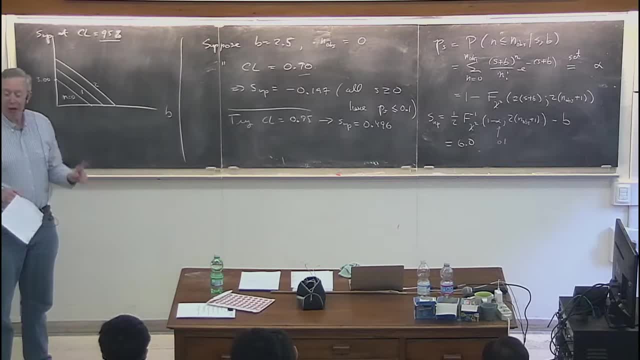 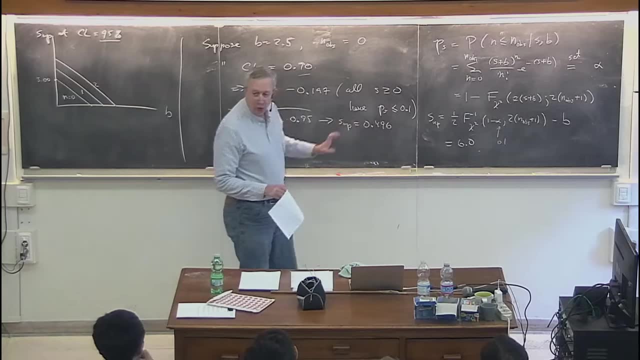 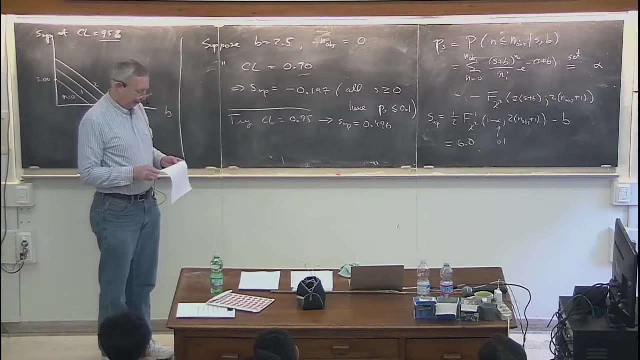 They can publish their paper. And not only are they happy that they quote a positive upper limit, but it's a pretty good upper limit, sort of 0.5, 0.496.. That's a very stringent upper limit. You've excluded a lot of positive values of s. 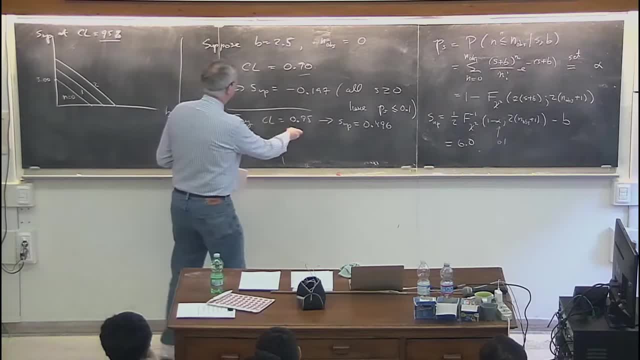 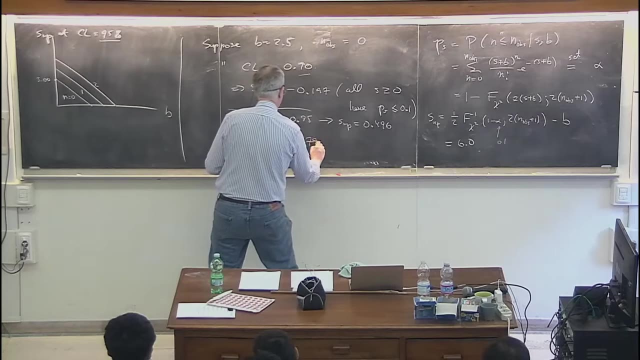 But why stop there? I mean, if you found, if you discovered that you can alter the confidence level and get a more satisfying upper limit, then you could try the following: Try here. I worked this one out: 0.917923.. 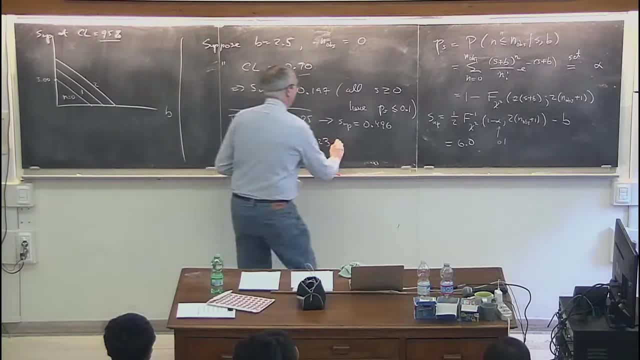 Why not? It's good at any other number, And this leads to an upper limit of 10 to the minus 4.. You want 10 to the minus 6? I'll get you 10 to the minus 6.. So what's going on here? 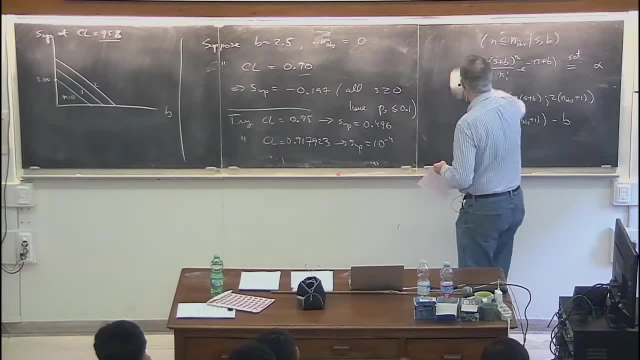 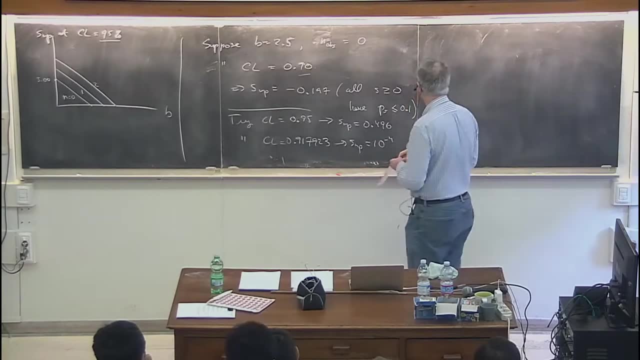 You can't actually believe this procedure is meaningful- and it's not. But where is the problem? How can we argue that this is not a meaningful way to proceed? And one of the ways to argue that it's not meaningful to quote such a low upper limit is to say: 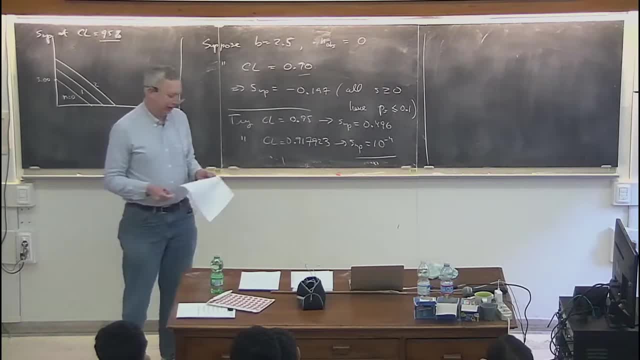 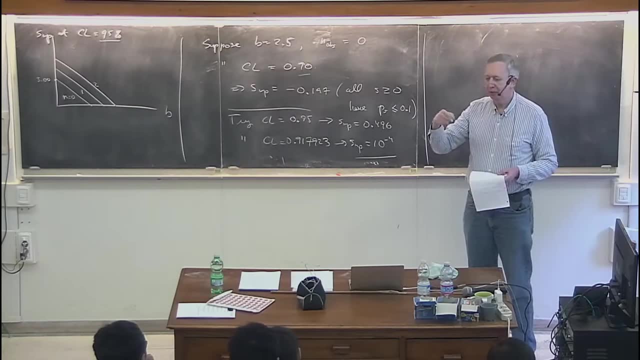 well, what's the intrinsic experimental sensitivity of this measurement? And so you'll recall that we're measuring a certain number of events, n, And that's equal to the number of signal events plus the number of background events. And the idea is, whatever we see is at least as big. 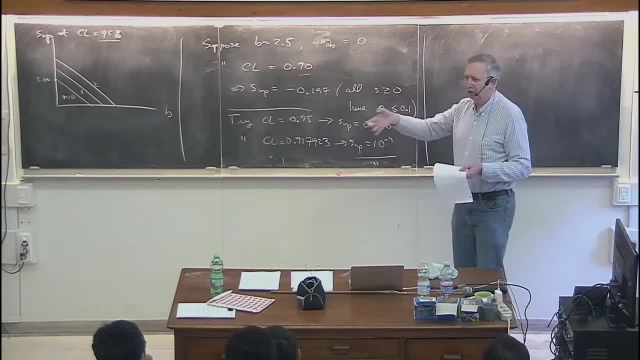 as the number of background events. The signal could be 0, or it could be something positive, And so the expected number of background I said was 2.5. And so that means that the standard deviation of the number of background events 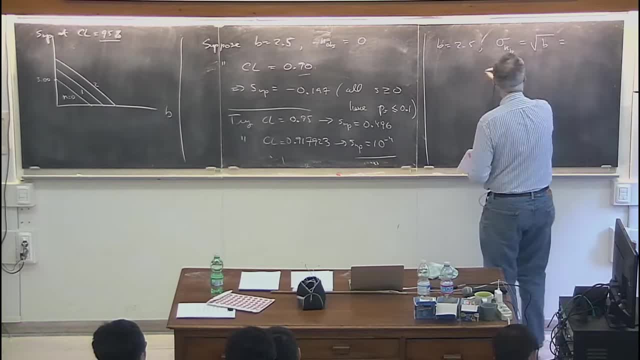 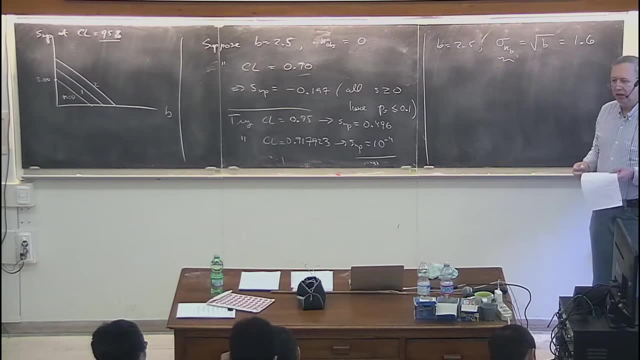 that's going to be equal to the square root of b. So that's square root of 2.5, which is 1.6.. So that sort of sets the intrinsic sensitivity of the measurement. It doesn't make sense to be quoting limits. 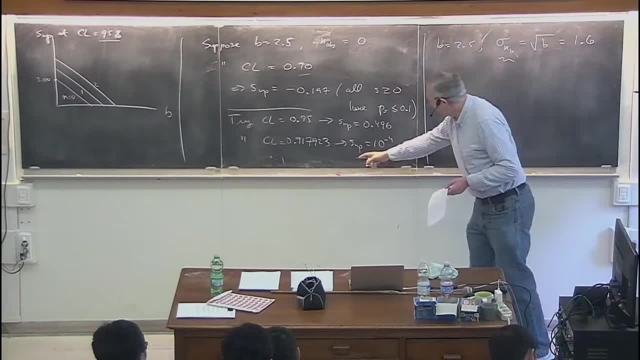 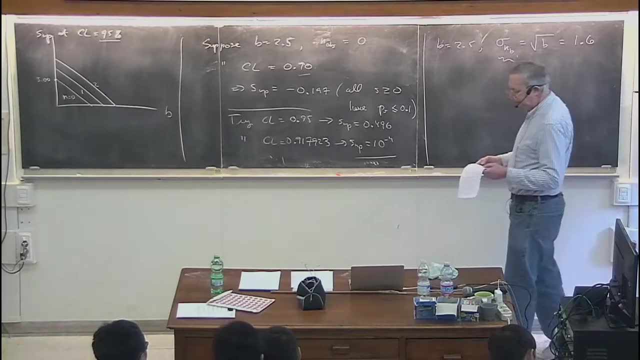 that are much smaller than that, And so clearly that tells you that this 10 to the minus 4 number is not meaningful, And it even should tell you that this 0.5 number is not very meaningful. Now how do we actually deal with this? 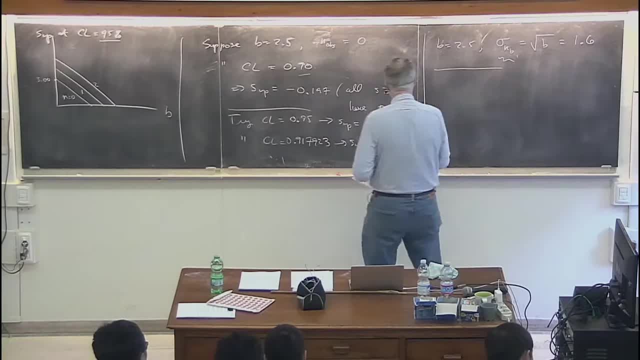 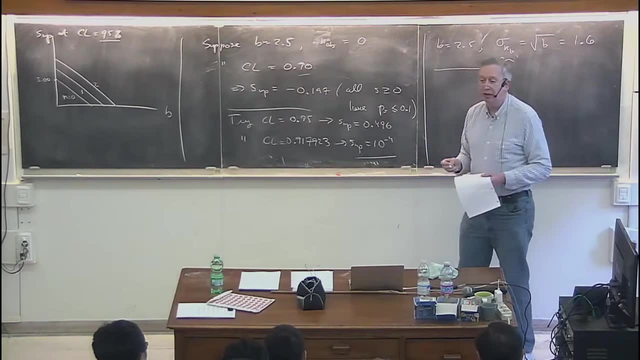 What we do is the following in practice is that whatever limit you get, first of all you don't go changing the confidence level a posteriori. All right, But suppose it were to come out that you got a very small limit. What people always do is they quote the observed limit. 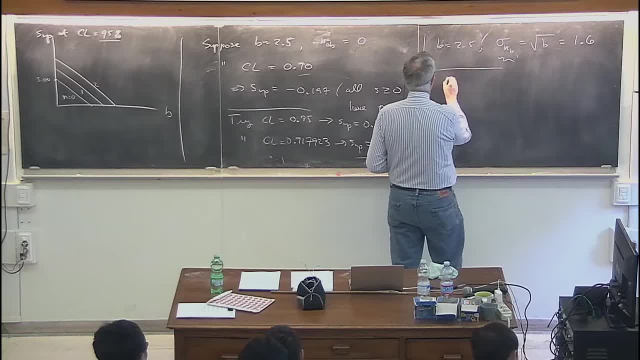 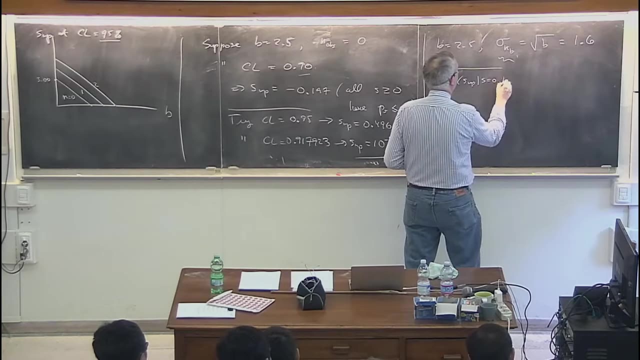 and then they do the following exercise: We work out the distribution of limits, say probability of getting a certain limit, under the assumption that there is only background. So under the assumption of s equals 0 and b, And if you make a histogram, say, of that, 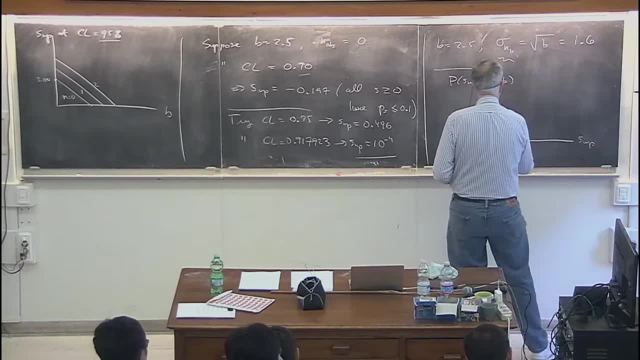 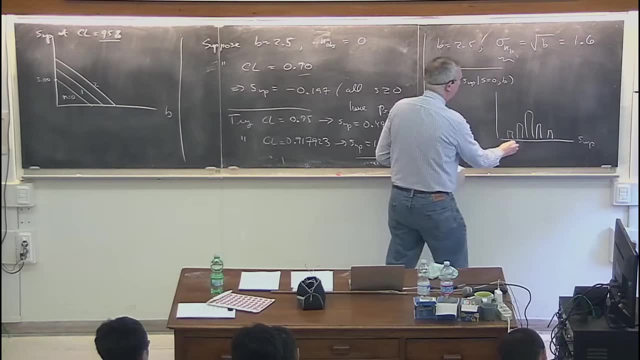 so, versus the upper limit, what you'll find is it's discrete data, So it's going to give you some distribution like that And the left-hand ones are going to correspond to the case where you found n equals 0.. So actually, here this guy, there. 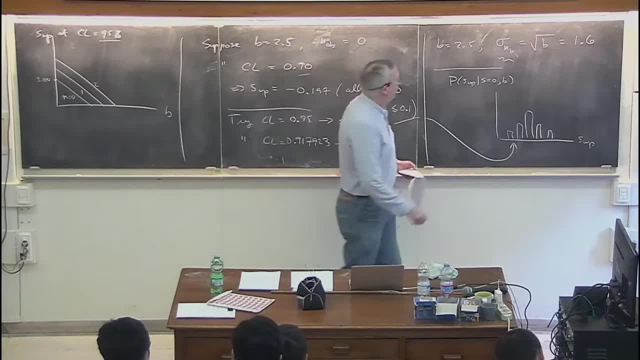 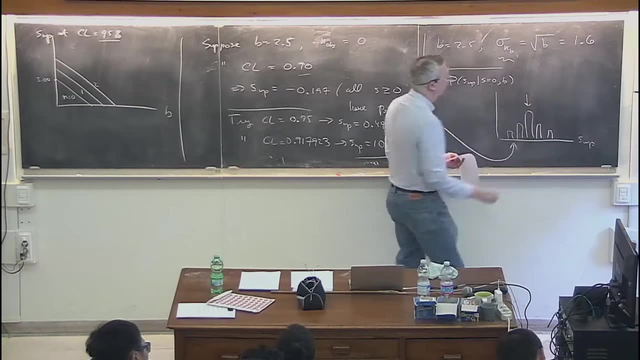 would correspond to that lower one. But, on the other hand, even if s is equal to 0 and you have a certain non-zero background, on average you're going to get a certain non-zero limit, And I worked out the numbers for this case. 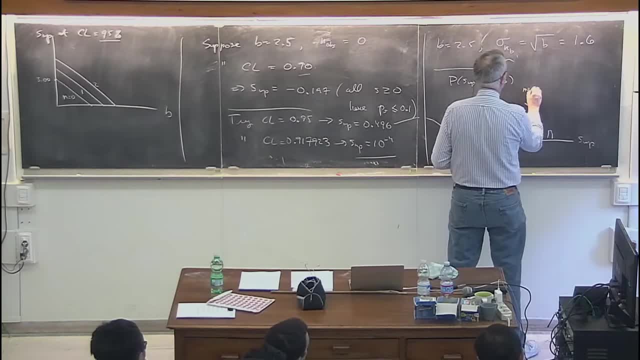 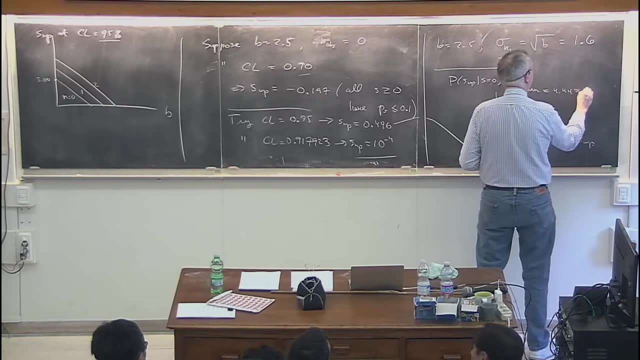 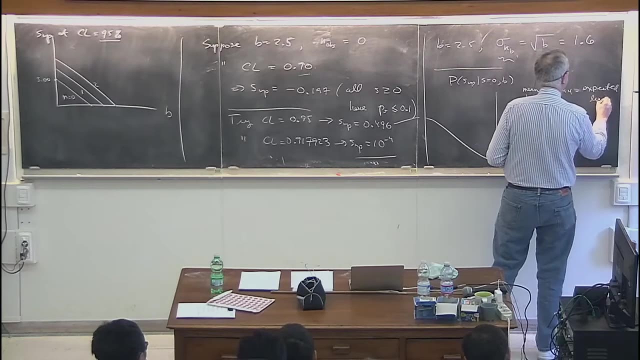 and it turns out to be the mean is equal to 4.44 in this case, And so you would give that what you would report, that is the expected limit. So people always report the observed limit and the expected limit, But you always have to then make sure. 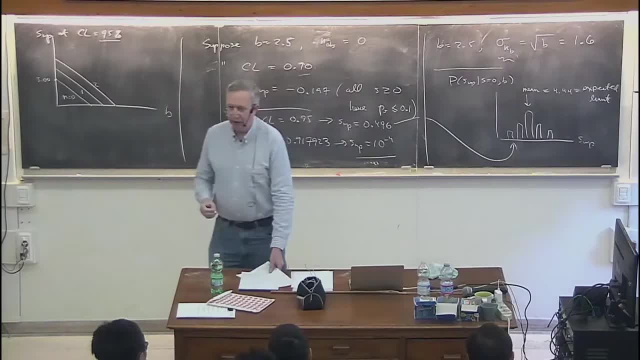 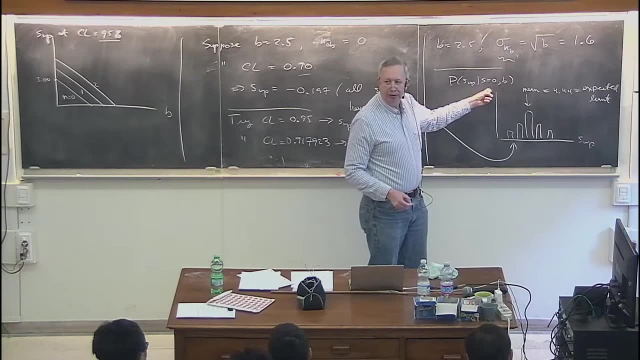 that you get them to define expected appropriately. What is the relevant expectation? in this case? I want to know what limit to expect if the signal is actually absent. So when I'm in the design phase of the experiment and I want to know how good of a limit, 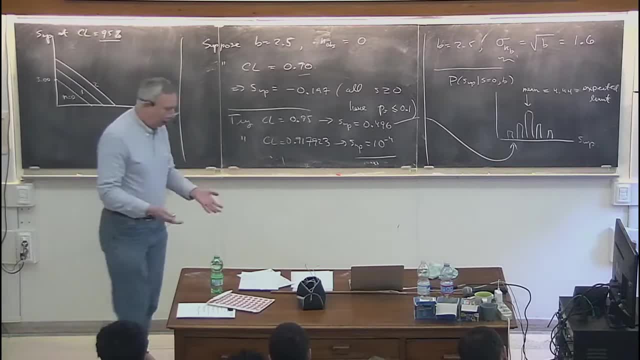 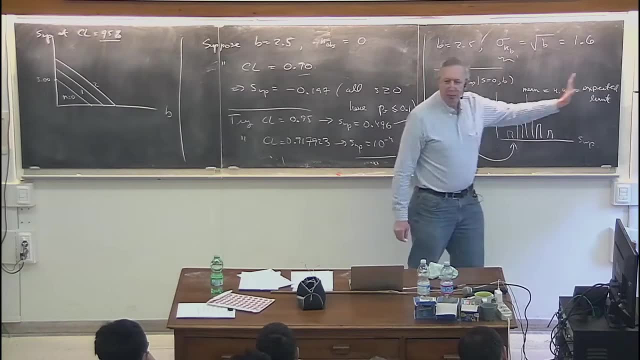 do I really expect to be setting Under assumption of what? Well, I want to know how good of a limit I'm going to set if the signal is actually absent. Obviously, if the signal is present, then my upper limit is going to be much higher. 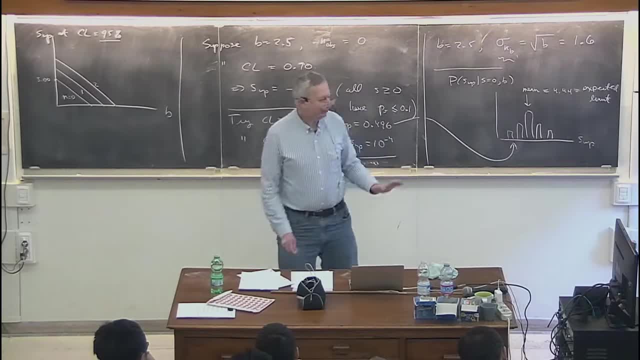 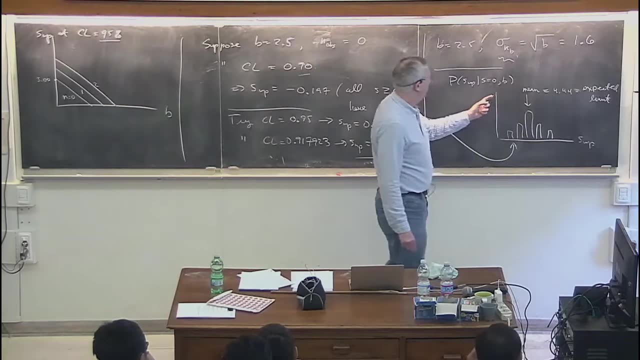 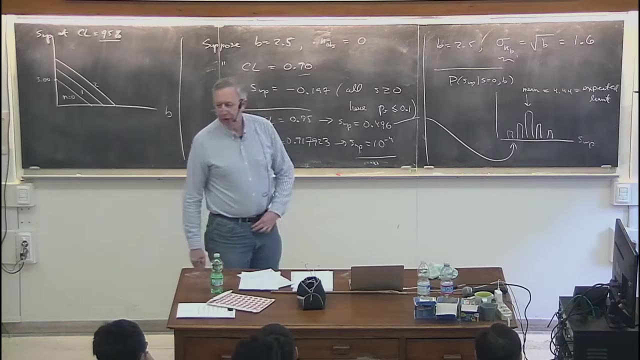 But then I don't worry about the upper limit. I'll make the discovery In terms of quantifying the experimental sensitivity. in terms of an upper limit, we want to know what the limit would be if s is actually 0.. Well, so there are various approximations. 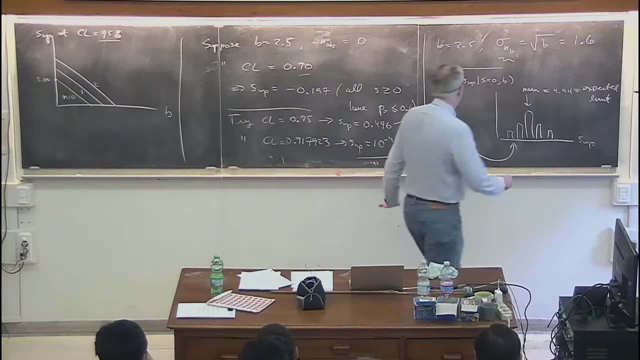 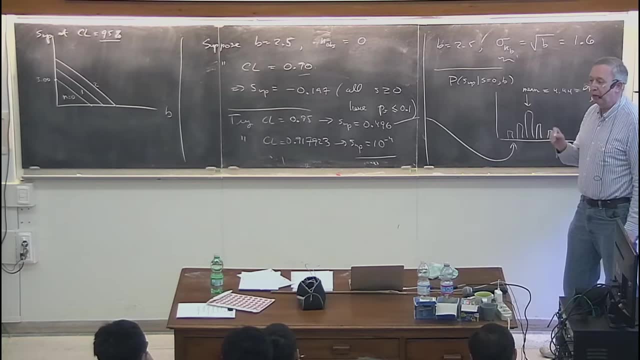 that we can go into, but the brute force way would be the following is that you would set s is equal to 0 and b is equal to 4.5, and I would generate a Poisson distributed value with a mean of 4.5. 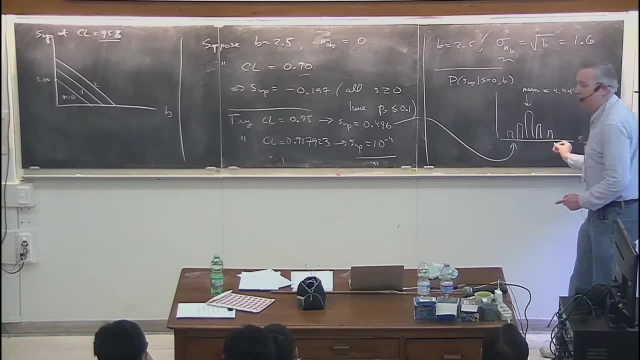 And from that value I would get a certain limit, which would be one of these values, and I would plunk that into the histogram And you simply repeat, And so that's the distribution that you would get and you compute its mean value. 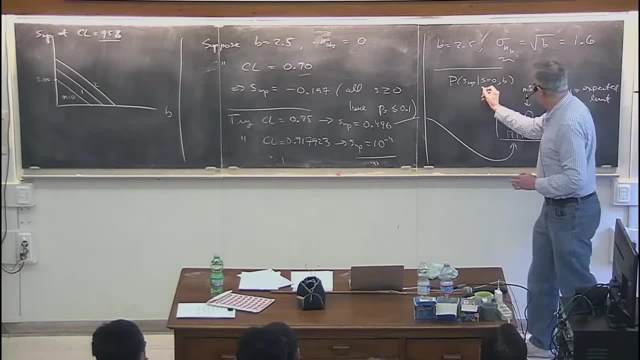 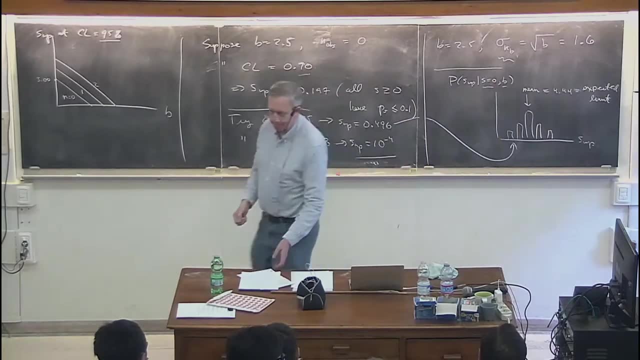 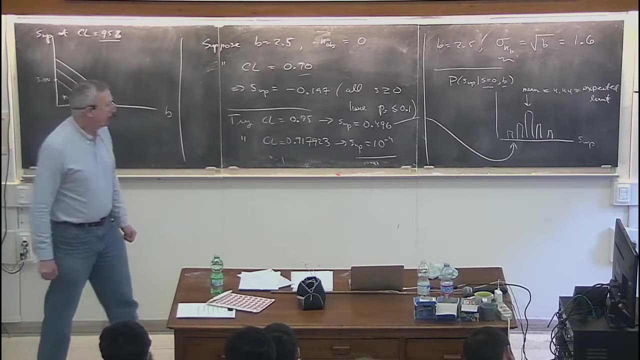 Yes, because that is the model that corresponds to this hypothesis: s is equal to 0, b is equal to something. So here the point is that I've drawn this kind of as a histogram, because that's the way I had it in the slides. 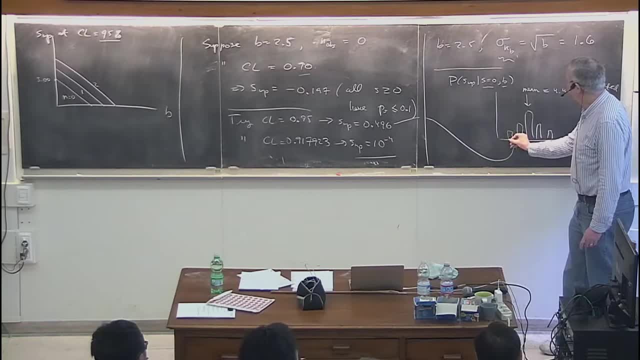 but really I should draw this just as a. It's not bins, because the data outcome is a distribution of the data and the data outcome is a discrete number. n equals 0, 1,, 2,, 3, 4.. 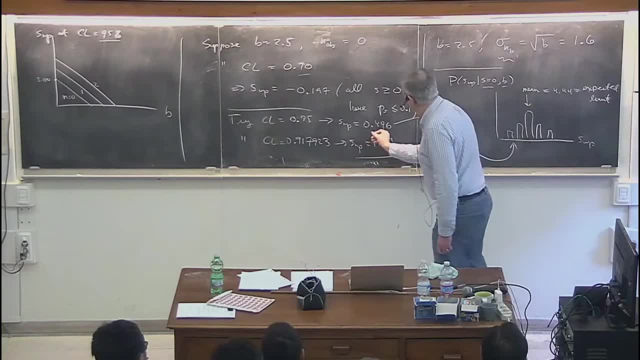 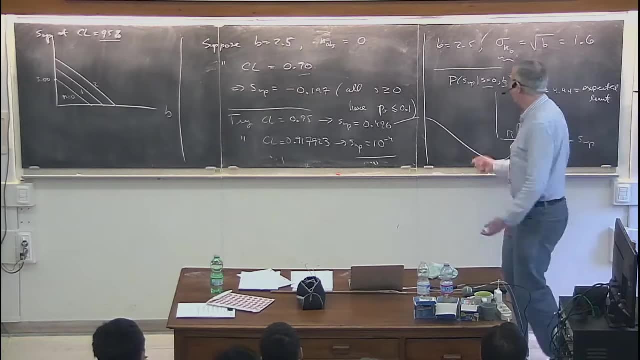 But if n is equal to 0, that gives me s up equals 0.496.. So this is not a histogram, It's a bar graph, But the point is that the distribution still has a well-defined mean value. I should comment right away. 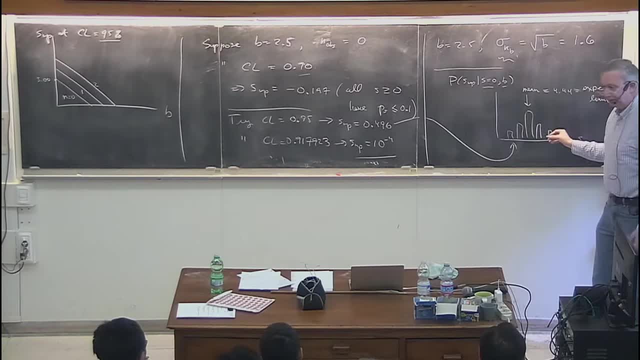 that sometimes, when we say expected limit, we mean the mean. Sometimes, for technical reasons that I'll maybe touch on later, we use the median. For a case like this, it wouldn't really matter much. You can see that the mean and the median. 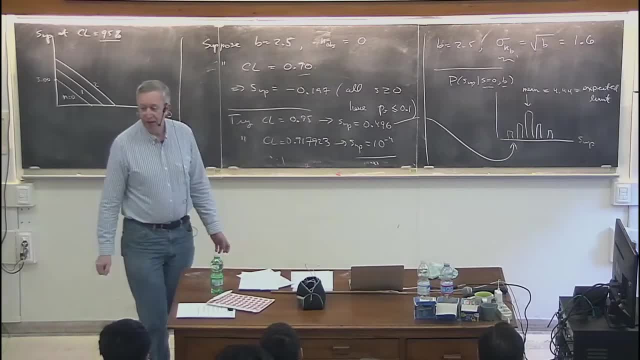 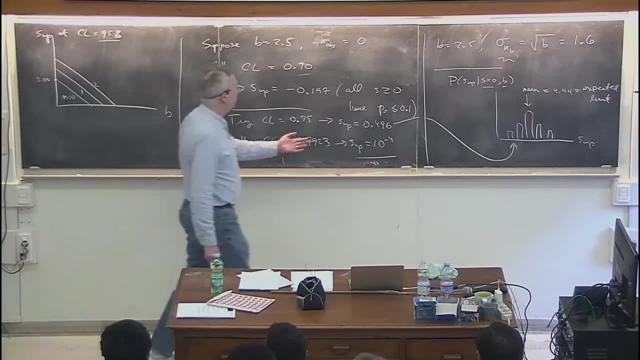 would be about the same thing For the upper limit. you report two numbers, You say our observed limit was whatever it came out to be, and then, if it was really low like this, you would probably make some comment of the form. 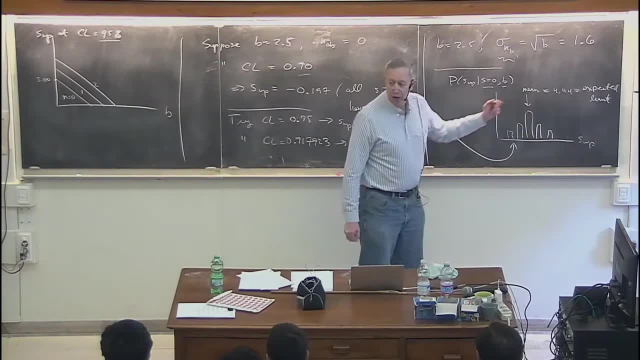 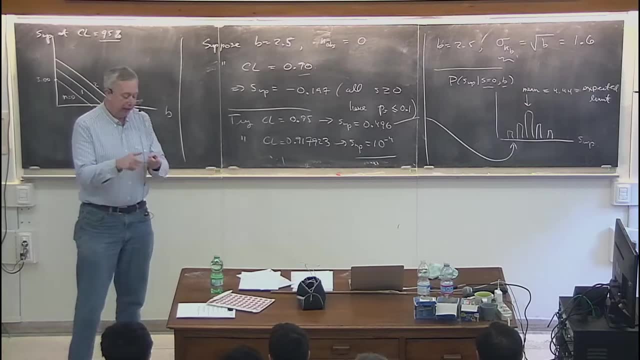 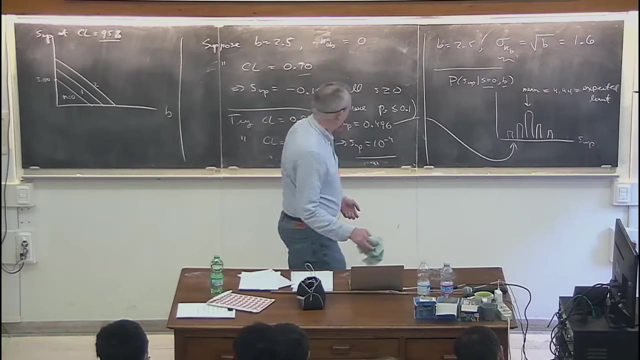 this is substantially lower than the expected limit of 4.44.. Those two numbers would go into the abstract. usually Those are the main numbers that you use to report the limit, the observed limit and the expected limit. So very often do I have a plot in the slides. 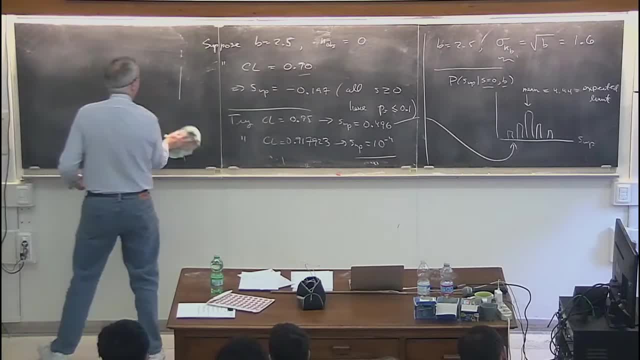 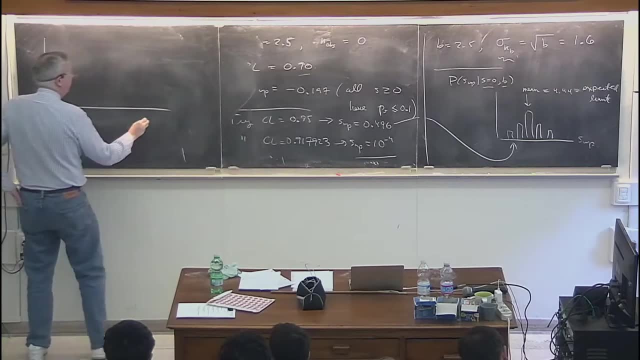 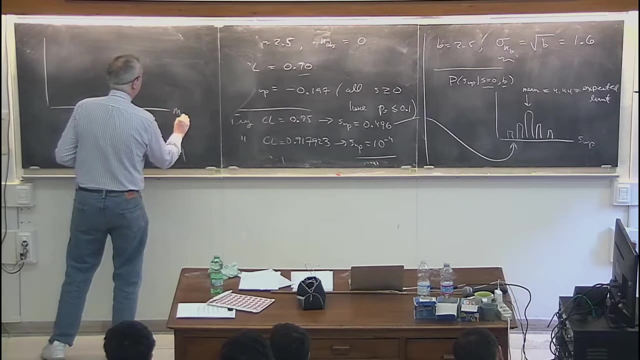 I'm sure you've seen these plots that usually have a traditional color coding- that if you have a situation where you're going to set a limit on a rate, but that's going to be a function of something like the Higgs mass, so what you'd do is you'd say: 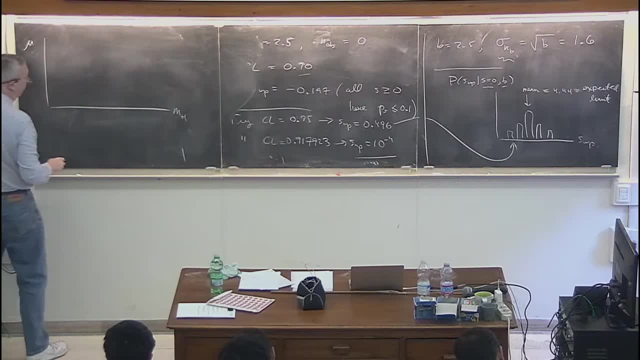 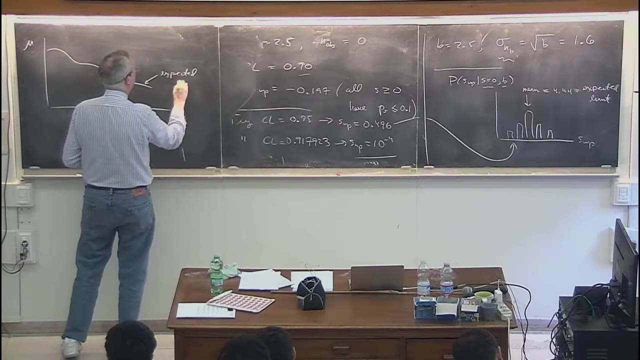 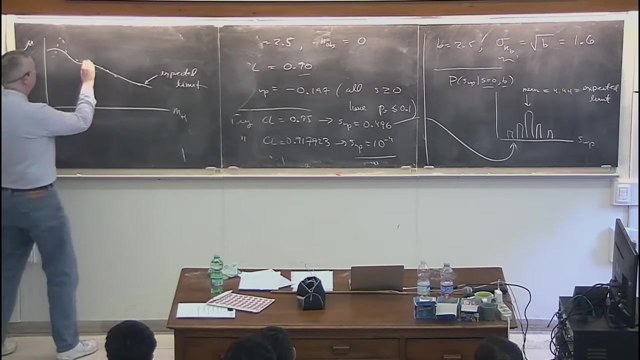 that this is the signal strength of the Higgs or the expected number of Higgs events. What you would do is you would have some curve that corresponds to the expected limit and then some other curve that corresponds to the observed limit. All right, 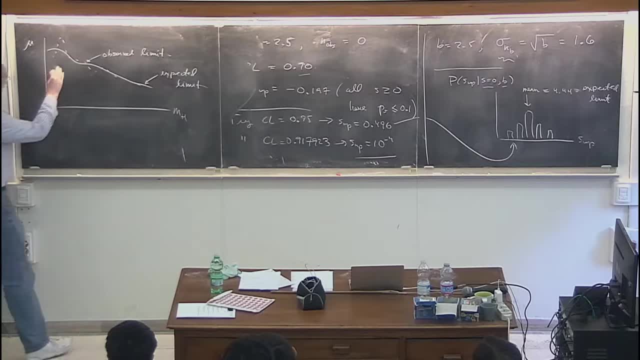 And then, if you think about how this worked with the Higgs, that in fact the observed limit was usually very close to the expected limit, except at 125 GeV, And the reason we had a high observed limit there is because there was actually a Higgs there. 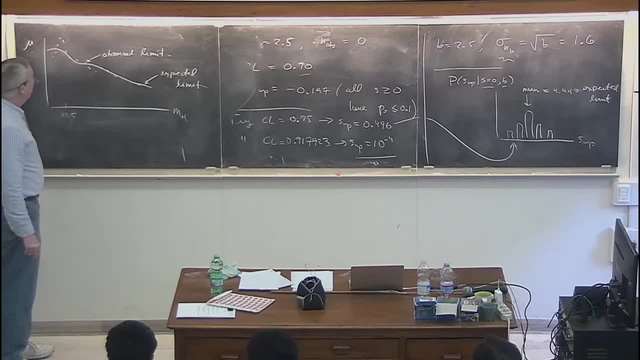 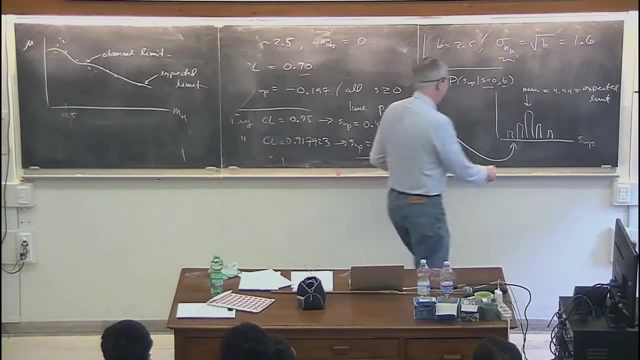 Okay, I should comment. one other thing that you've surely seen with these plots is the color coding. Ah, I have yellow chalk, This is great. So let's suppose that this expected limit is what you report to your funding agency to get the money to do the experiment. 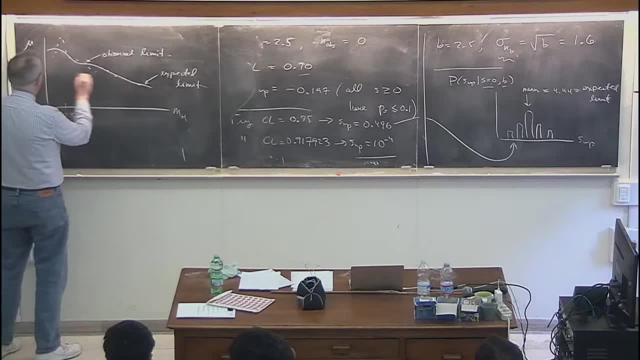 You say, if you give me the money I will be able to set a limit on the Higgs rate of such and such. Then you go do the experiment. Let's suppose this were a particle that you didn't actually discover And for this value of the Higgs mass. 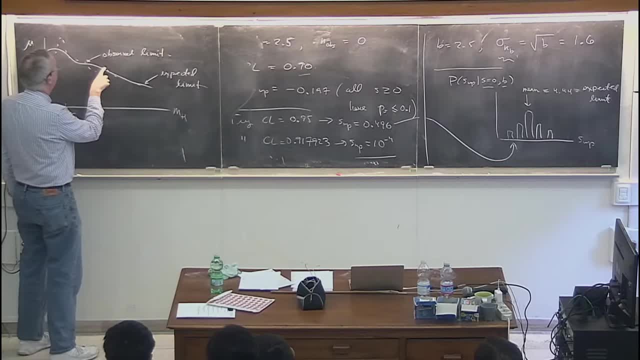 you see that actually, the limit that you observe, that you actually set, is not as stringent as the expected limit. You know, sometimes it's less stringent, sometimes it's more stringent. And so what you do is, if you look back at this distribution, 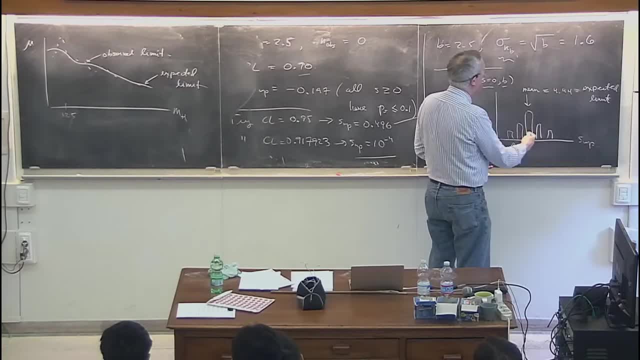 you say: well, of course the thing's going to fluctuate around, You're not always going to get a limit which is, you know, close to the mean. Sometimes it's high, sometimes it's low, And so you want to give the funding agency. 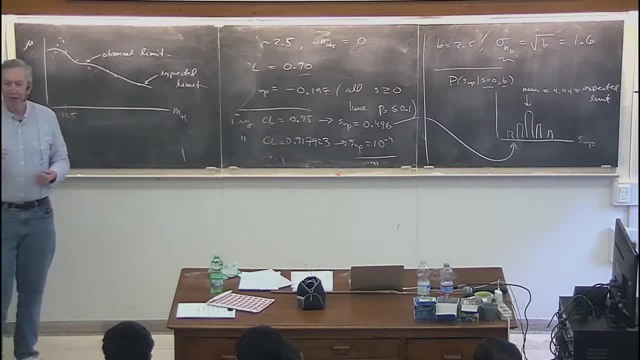 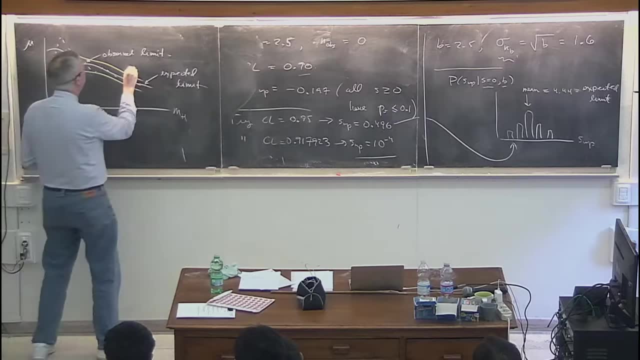 some sense of how much of a fluctuation to expect, And so what you do is you make a yellow band that corresponds to plus or minus one sigma. All right, So this is something like plus or minus one standard deviation of the distribution of limits. 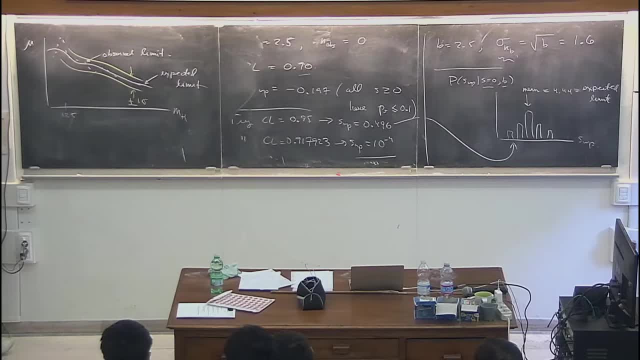 assuming s is equal to zero, And then you color that. Is it yellow or green? I forget. If it's yellow in the middle, then what you do is you make the plus or minus two sigma band green, And so it ends up looking like a Brazilian flag. 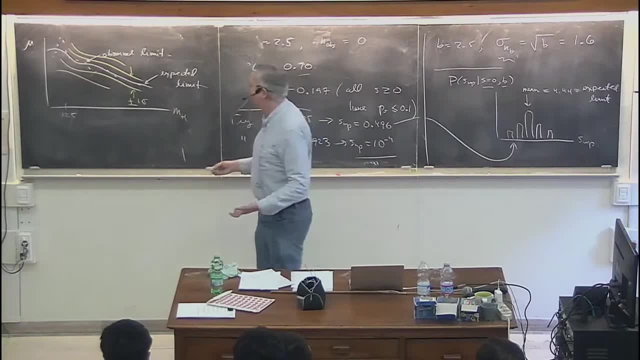 And so we refer to that as the Brazil plot. So the Brazil plot is the plot of the bands, of the plus or minus one sigma around the expected limit and plus or minus two sigma. So I'm sure you've seen these plots. That's what's going on there. 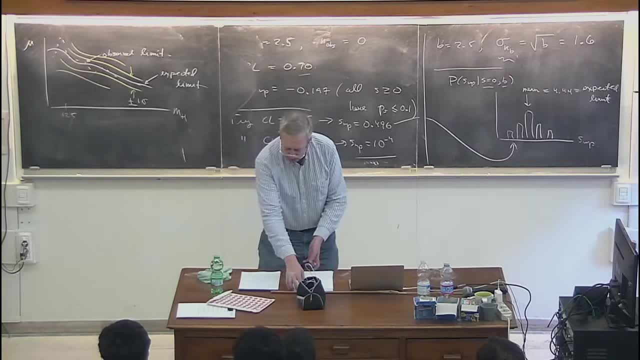 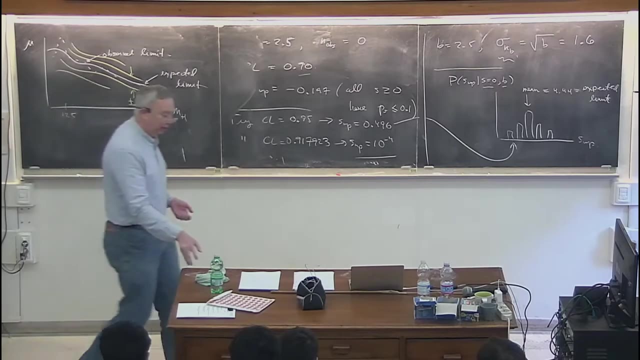 Okay, Okay, good, That's about all I wanted to say now for this particular problem, And I want to go on to a more generic analysis, which is more general than the case when we simply count one number, And we've touched on this already. 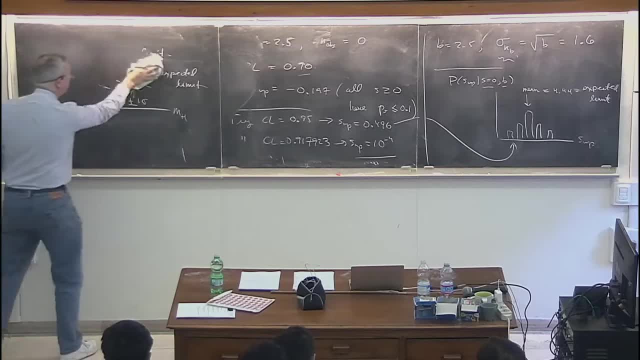 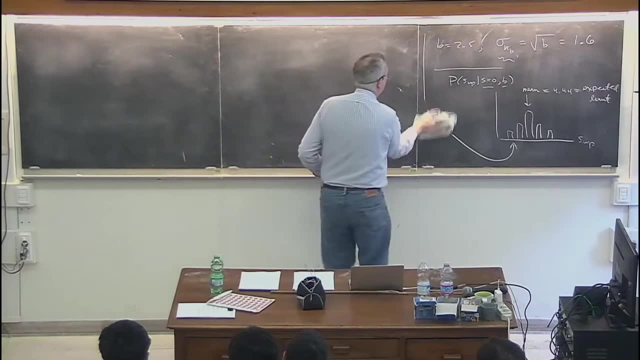 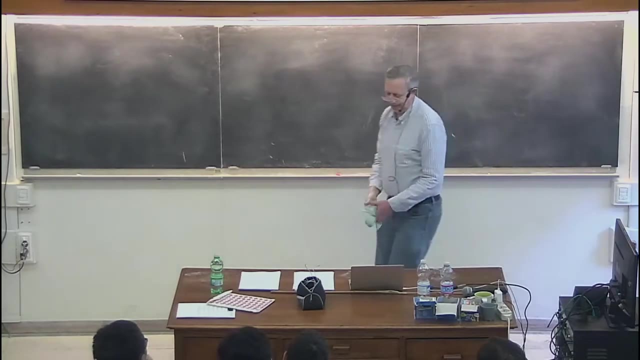 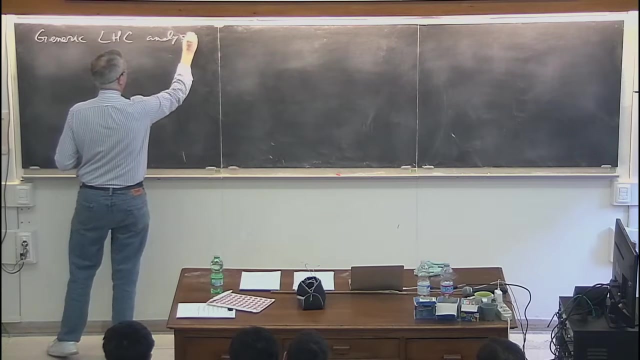 in the discussion session, but let me put it up on the board so that it's perfectly defined. So this is a more generic LHC analysis. Let's call it that. Not every LHC analysis will be in this framework, but an awful lot of them are. 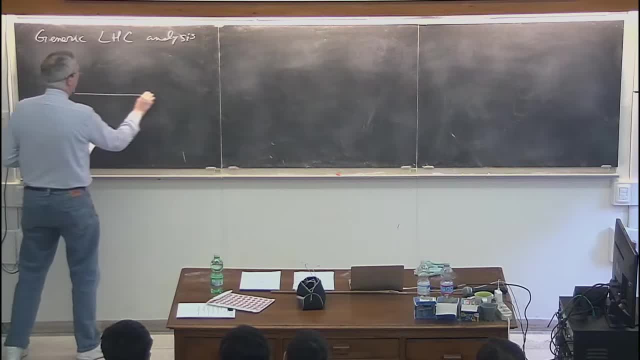 So it's worth considering this case. So let's suppose that we're looking for some new phenomenon, And the way that we do that is, for each event that we find we measure some kinematic variable. I'll call it x In the case of searching for a Higgs. 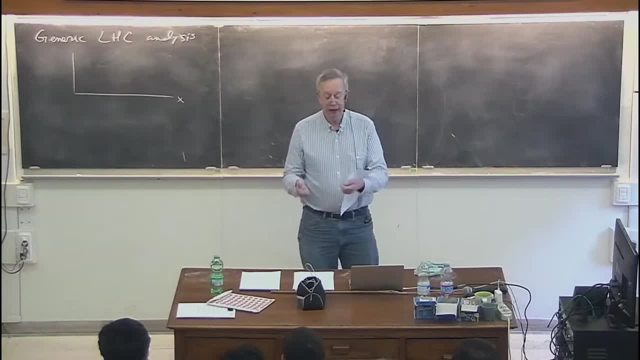 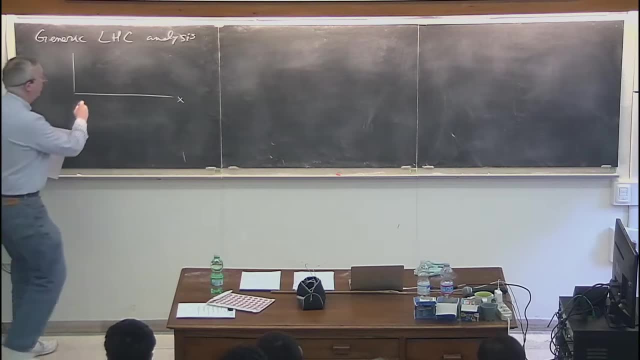 x would be the invariant mass of the Higgs candidate. right, You form photon pairs, You make their invariant mass, But in other cases it could be some other variable. But the point is that somewhere in the distribution of this variable I expect the signal to be present. 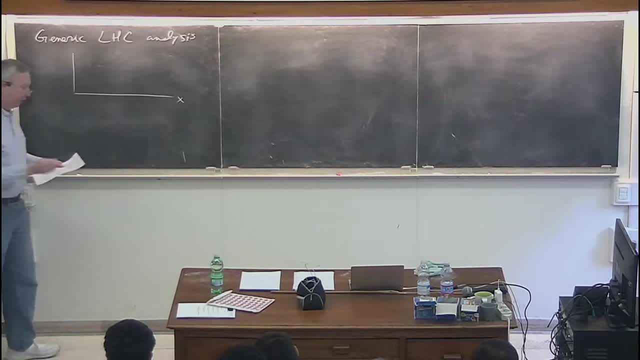 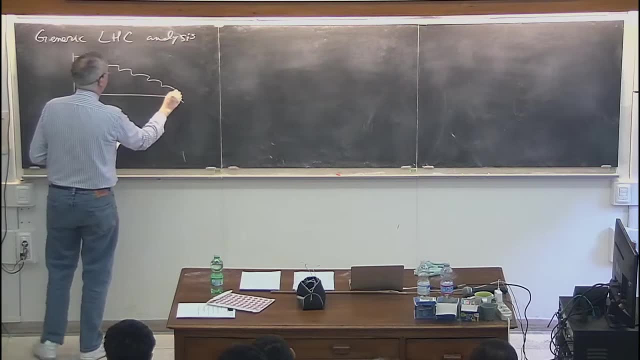 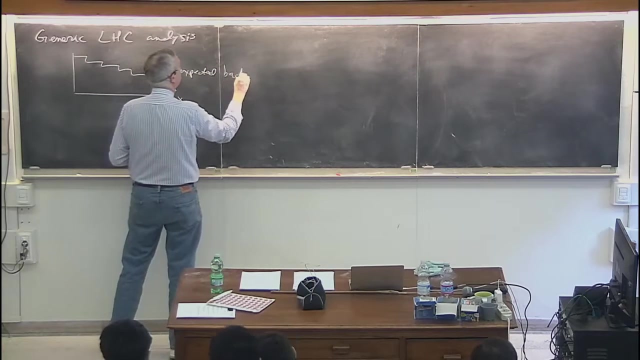 perhaps as a peak, perhaps as just a deviation from the background-only hypothesis. So let me suppose that I'm going to do this as a histogram now. So I'll have some histogram here that represents the expected background. So background is context-dependent. 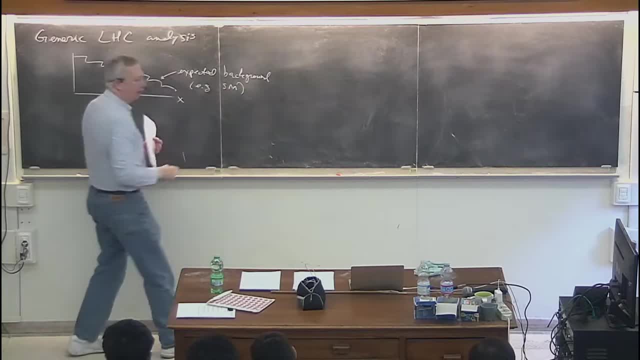 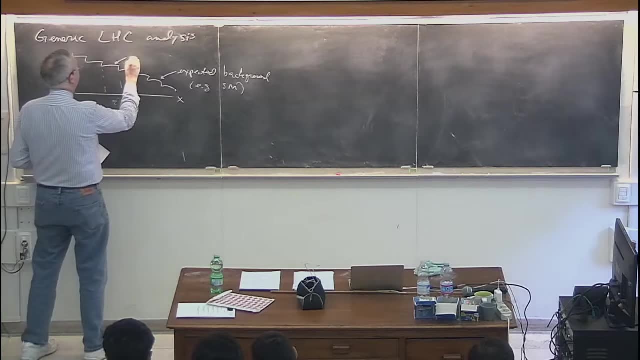 but let's suppose that that means it's a standard model, It's whatever model doesn't include the signal that I'm looking for, And so here in bin i I would have some expected number bi And then, if I then consider some signal model, 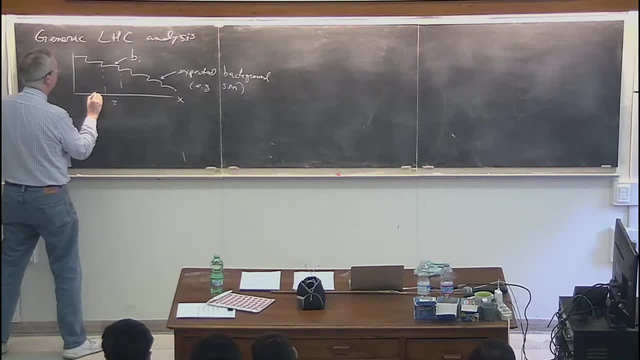 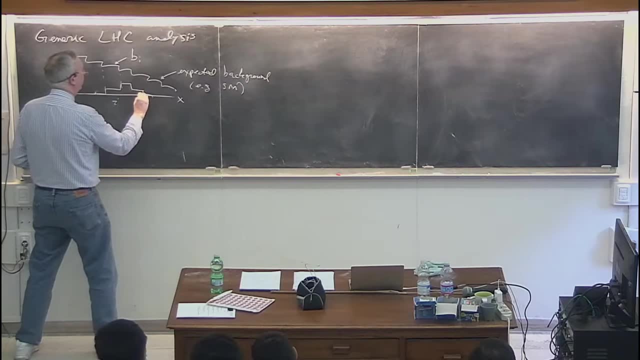 then maybe it predicts. I better make the bins line up So that histogram there represents the expected signal from some signal model, And so in that bin there I have some expected number of events s sub i, And you'd run your Monte Carlo. 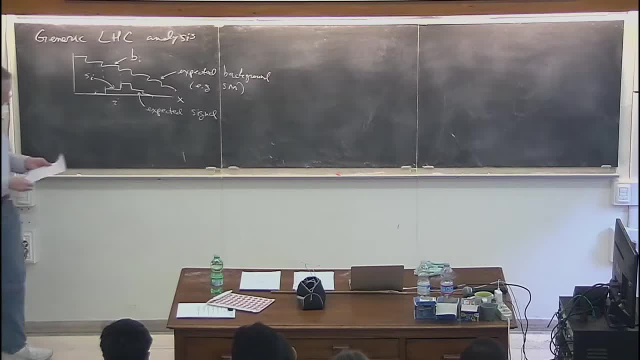 in order to determine the s? i's and the b? i's. And so now the goal, the main theme that I've been trying to emphasize for the last two and a half days, is the way to do a statistical analysis, is to decide what is going to be. 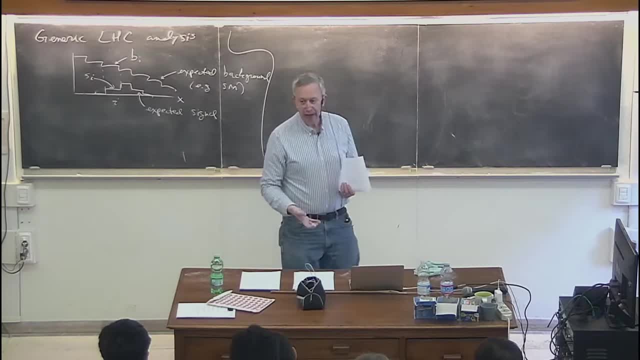 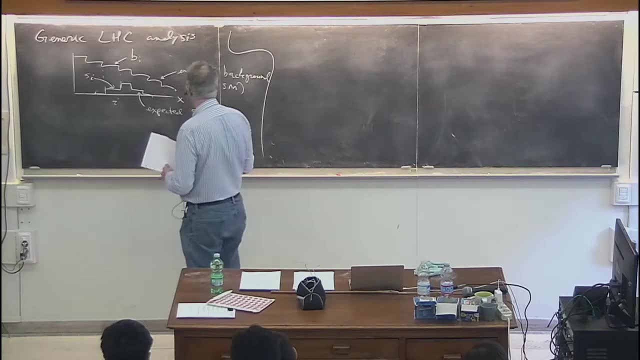 regarded as data and to write down the probability of those data. And in this case, what I'm going to say is that when I do the experiment, I'll find a certain number of events in each bin. So the measurement is to find n. i. 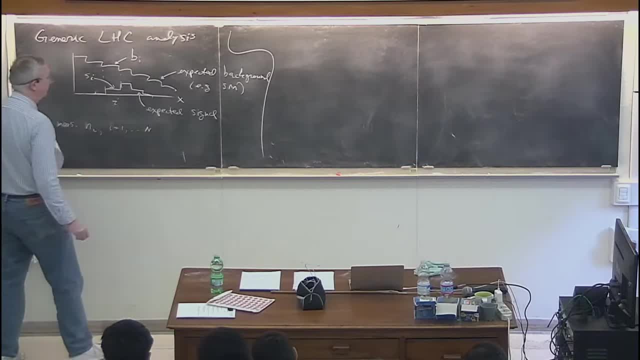 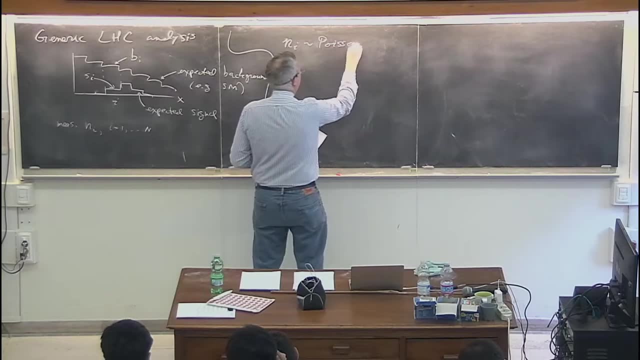 i equals one up to say some number of bins, And the probability model that is most often appropriate is that those values are independent and they all follow a Poisson distribution, And if the signal is absent, the mean is bi. if the signal is present, 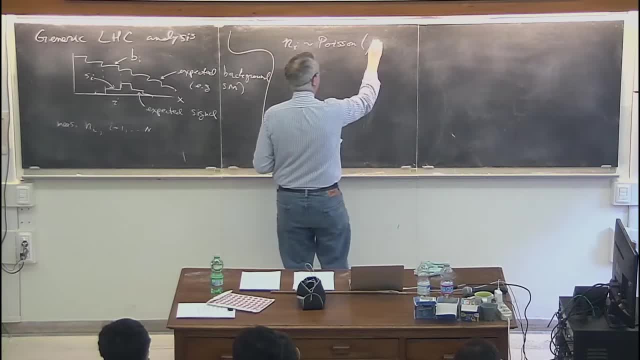 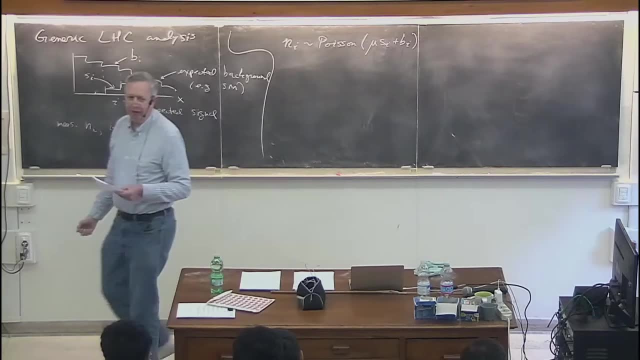 it's s? i plus b? i, And so I'll write this as a strength parameter: mu times s? i plus b? i, So mu becomes my parameter of interest. If I can reject the hypothesis that mu is equal to zero, I've made my discovery. 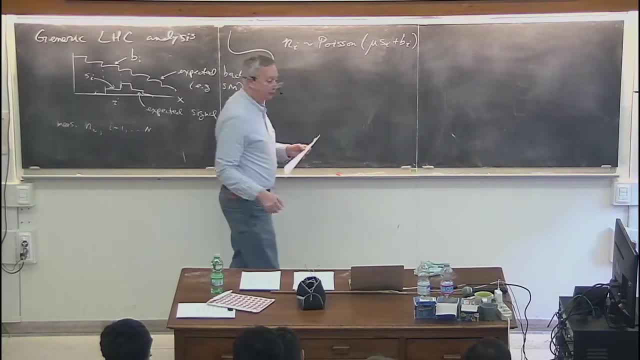 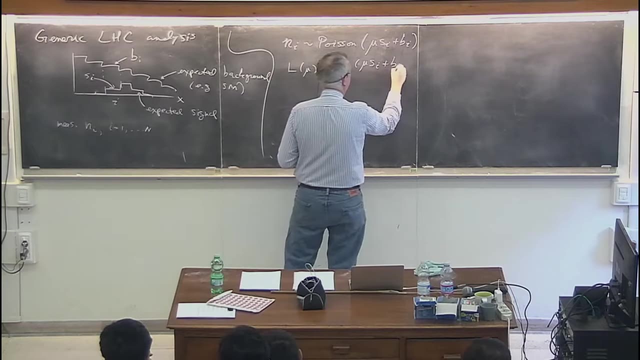 If I can't, I can set limits on mu, And so that means now that the likelihood function as a function of this parameter is just going to be: the product from i equals one to n of mu s i plus b i to the n i over n i factorial. 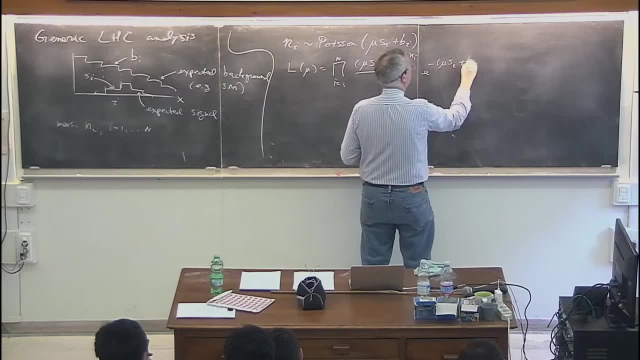 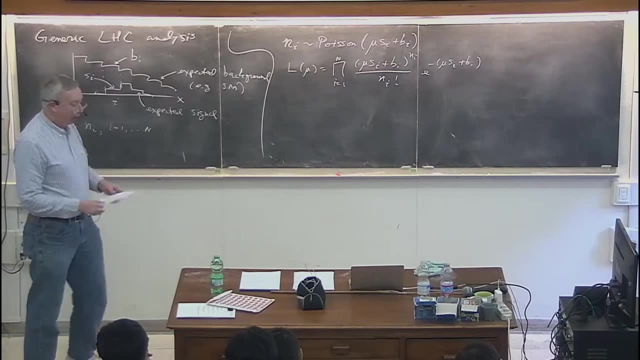 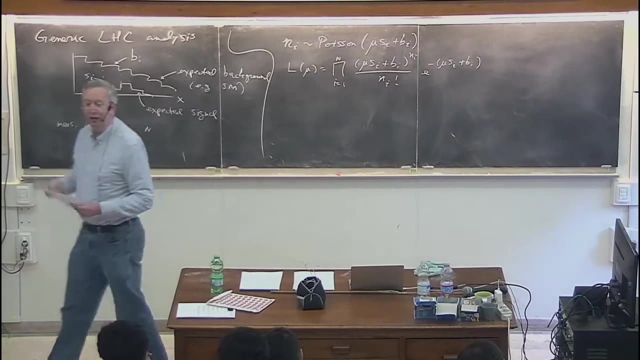 e to the mu s, i plus b i. So now I have my likelihood function. All right, mu equals zero. yeah, I said So. now I'm off and running Once I can write down that rule. I can go either down. 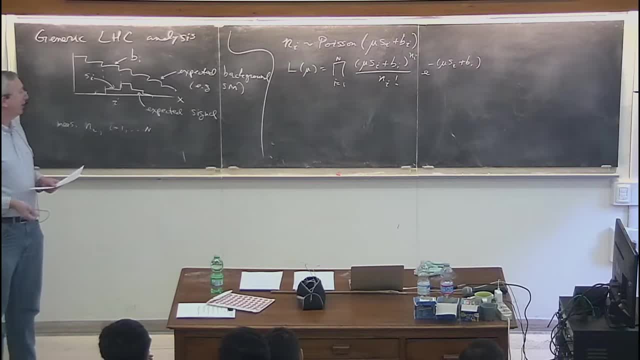 the frequentist route or the Bayesian route. But that's always the first step. in both cases You have to say what's the data and what is the probability for those data. So let's consider now still the frequentist approach, since that's what's by and large. 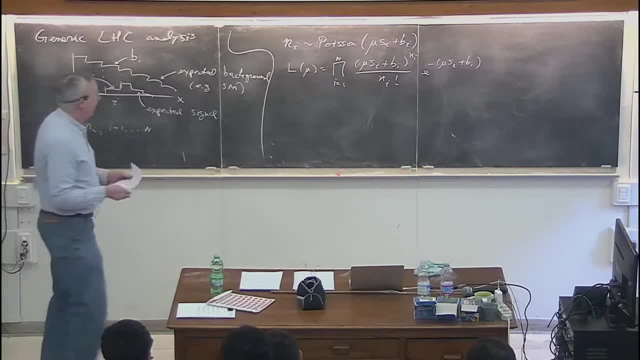 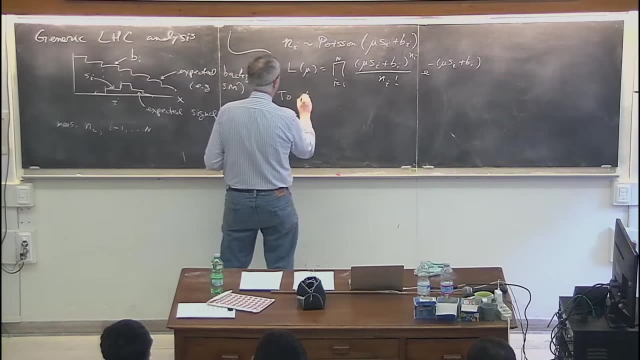 used in LHC analyses And I want to test different hypothesized values of mu. And so let's say, to test mu, what I need to do is I need some criterion according to which I'm going to say what for a given mu. 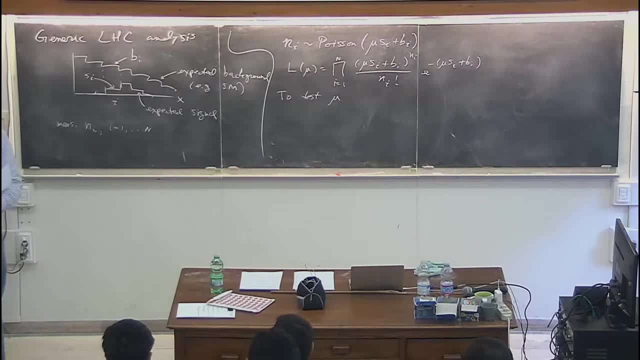 what data values would I put in the critical region? What data values would I say constitute lesser or equal compatibility for purposes of computing a p-value for mu? And to do that, remember that if you have some multivariate data space, it's not that obvious. 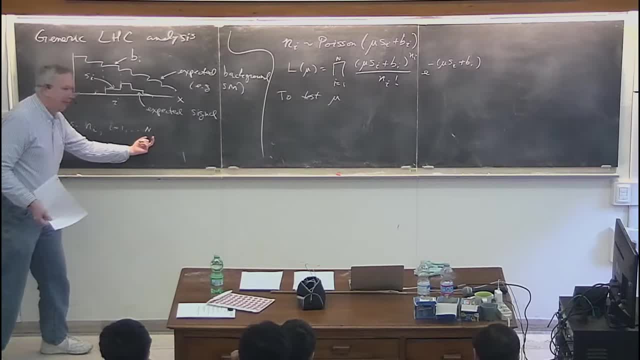 Here we have, you know, the n bins, capital N bins. So it's this complicated multivariate data space. What total, what region of that space am I going to use for my critical region? Well, the way to do that is to define a test statistic. 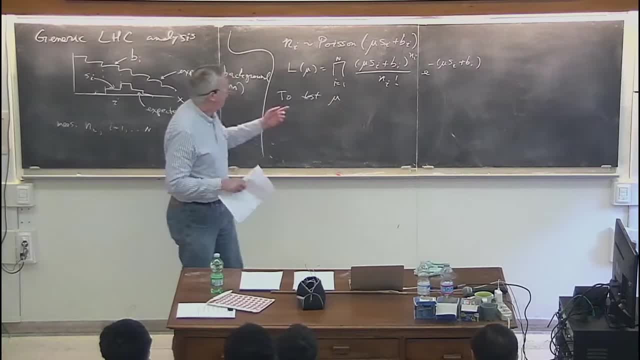 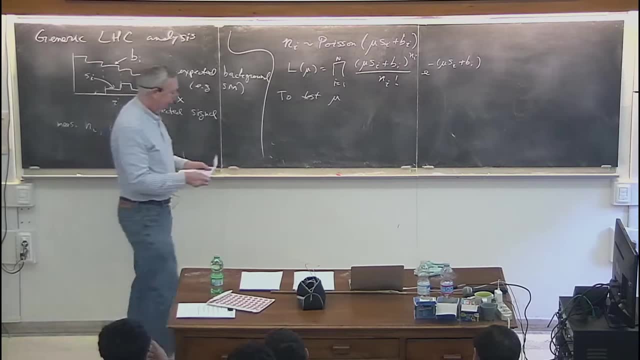 such that that test statistic, which is some function of the data, if I set that statistic equal to a constant, it will give me then the boundary of the critical region, And the test statistic that I'm going to use is what I'll call lambda of mu. 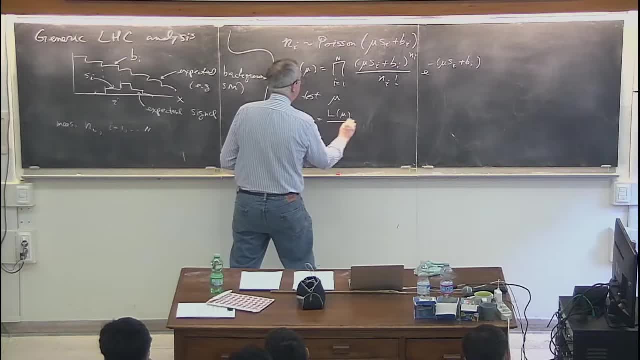 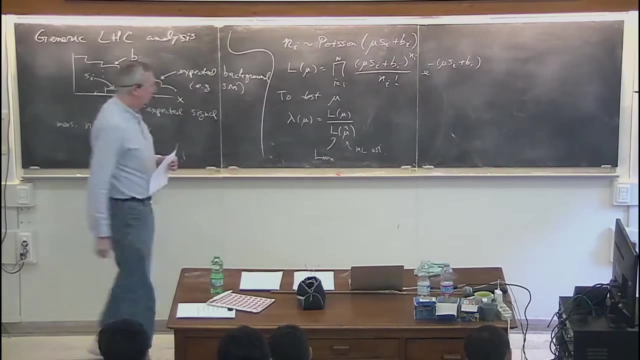 And that is going to be the likelihood of mu divided by the maximum of the likelihood, And I'm going to take mu hat here always to be the ML estimator. So that thing in the denominator is just L max. Okay, so that's a particular. 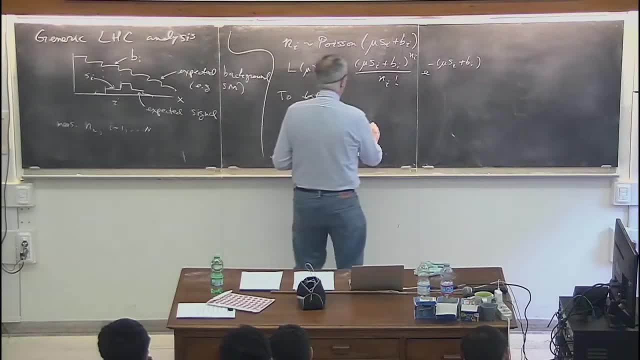 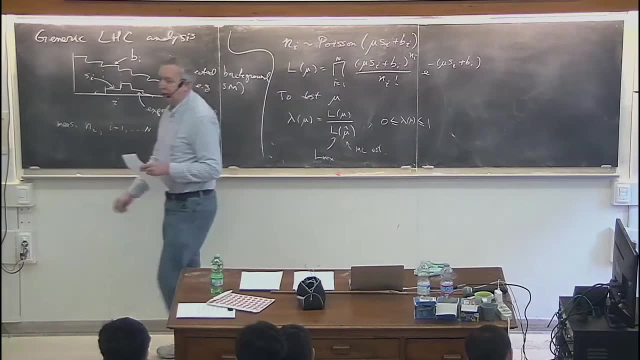 likelihood ratio, You can see that it lies between zero and one, And if the hypothesized value of mu is in good agreement with the data, that means that mu hat is going to come close to that value, And so, therefore, lambda is going to be close to one. 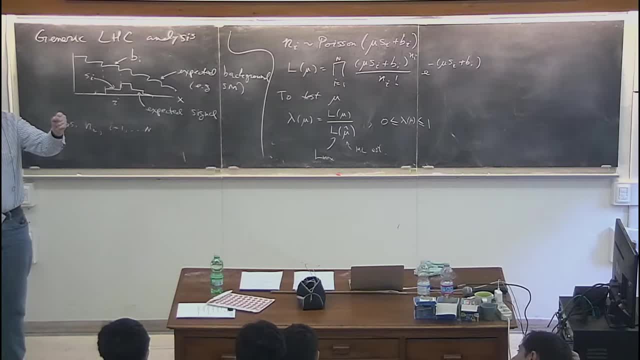 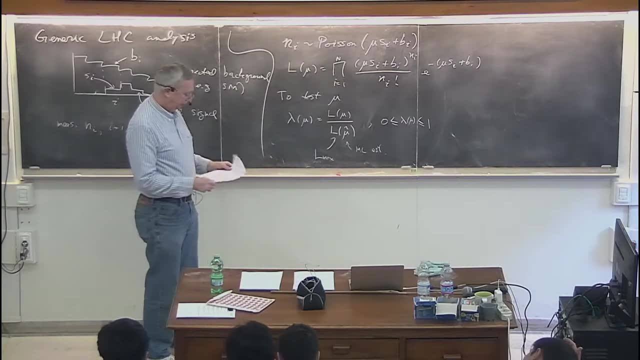 On the other hand, if you hypothesize a certain value of mu, but mu hat comes out miles away, then of course, then this likelihood ratio is going to be very low Right Now for sort of conventional- it's not just convention- 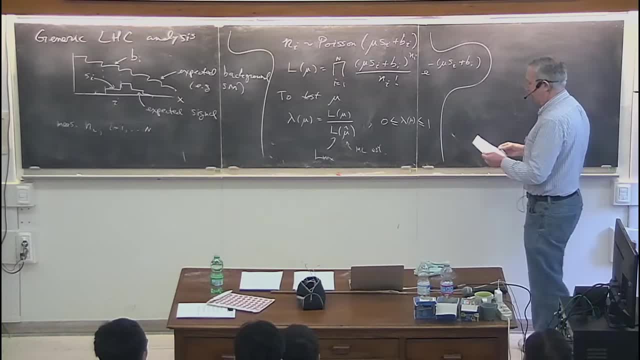 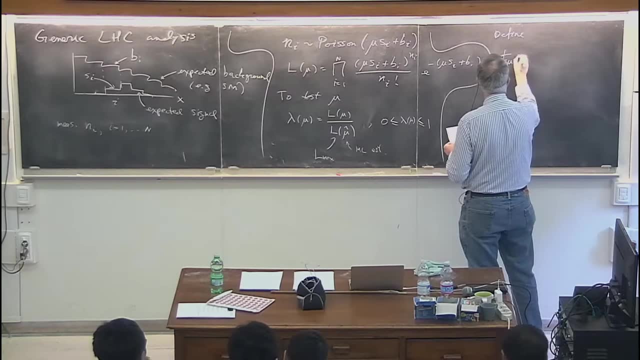 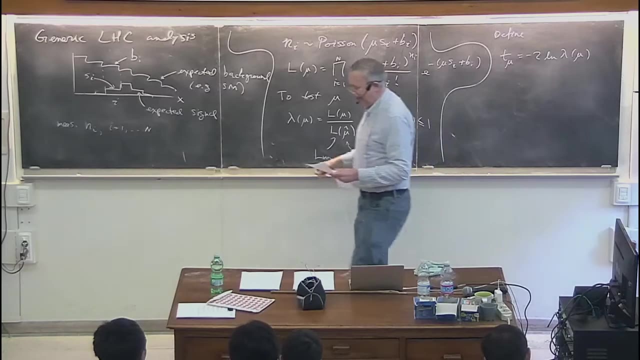 it's a little more than that. We could just work with lambda. but it turns out to be convenient to define T? mu, And T? mu is simply minus two times the log of lambda mu. And so now this notion of high means good and low means bad. 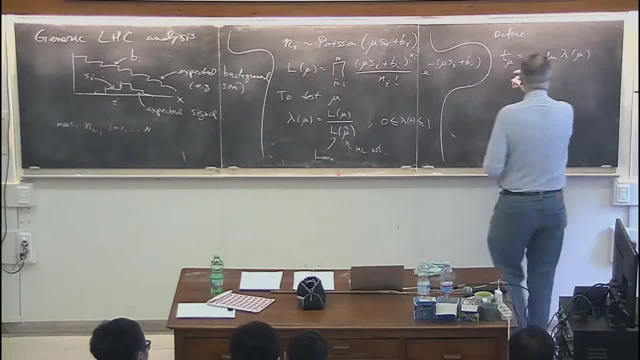 it gets reversed because of the negative logarithm. So now, if lambda is low, then T is going to come out high. If lambda is one, then T is zero. So you can think of this statistic T kind of like a chi squared variable. 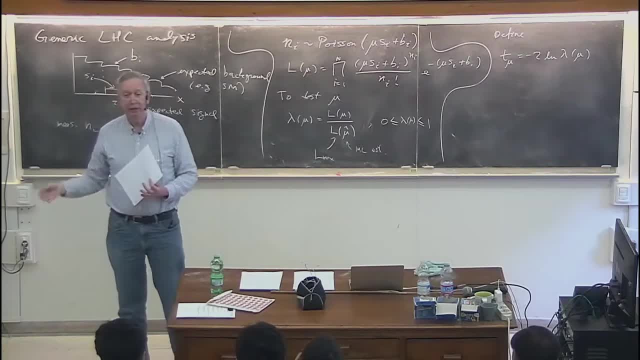 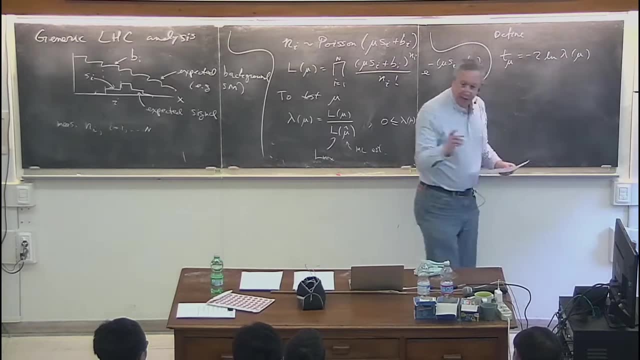 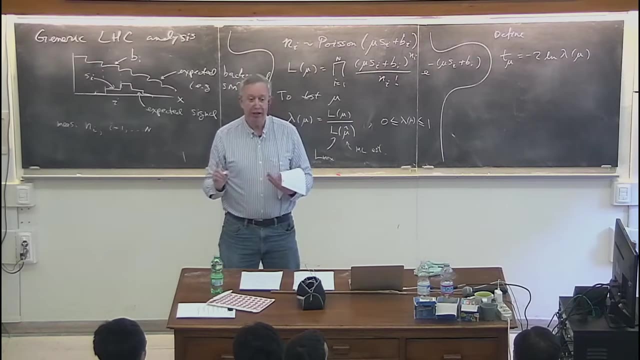 High values correspond to bad agreement between the hypothesized value of mu and the data, And so, given that statement, if I say now that high values of T correspond to lesser compatibility, that's the criterion I need to invoke to define the p-value. 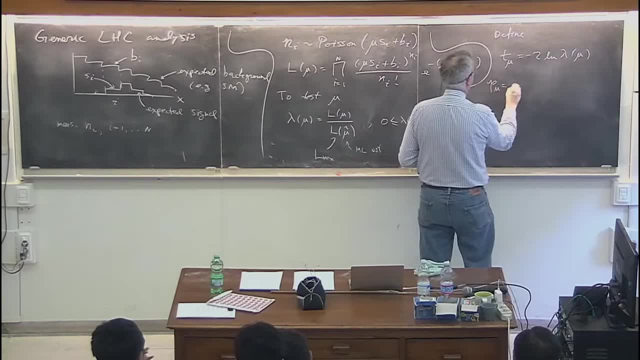 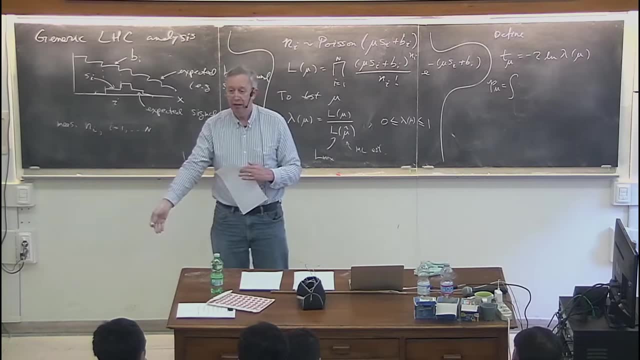 So now I can say that the p-value for a hypothesized value of mu is simply the probability to see T mu as high as the value I observed or higher. So that criterion now defines the region of data space that I will deem to have lesser or equal compatibility. 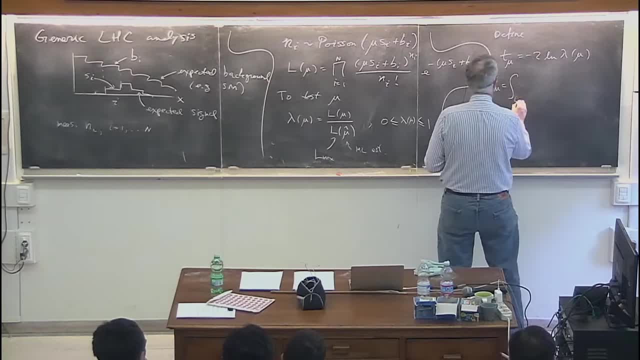 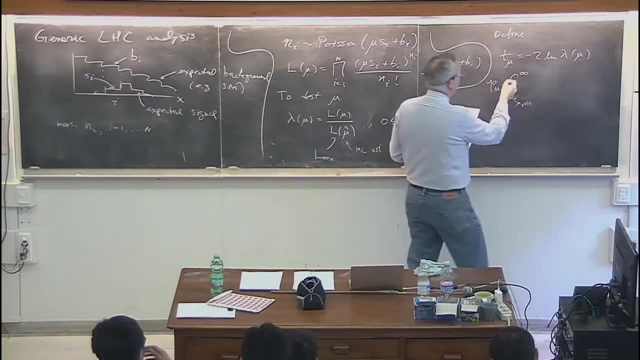 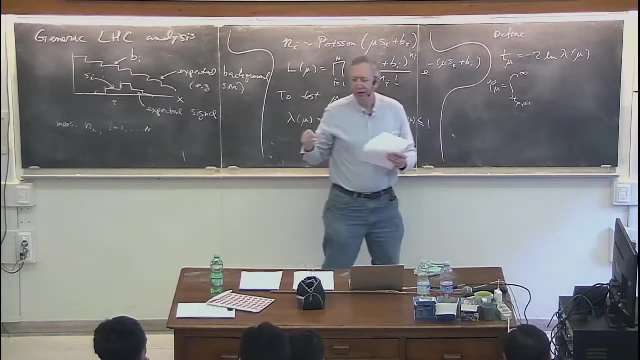 So this is then the integral of T mu observed to infinity. And now I need to know, under the assumption of a certain value of mu, if I were to repeat the experiment many times, how would the statistic T mu be distributed? I need to have some expression now. 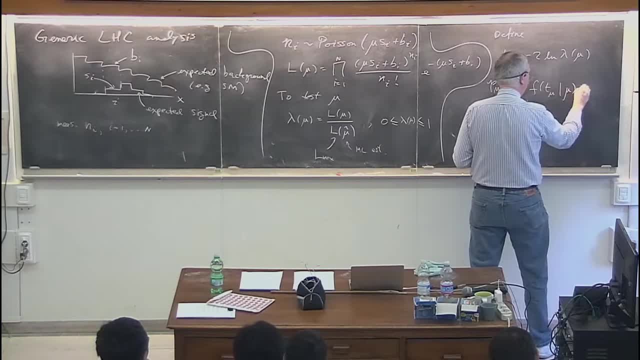 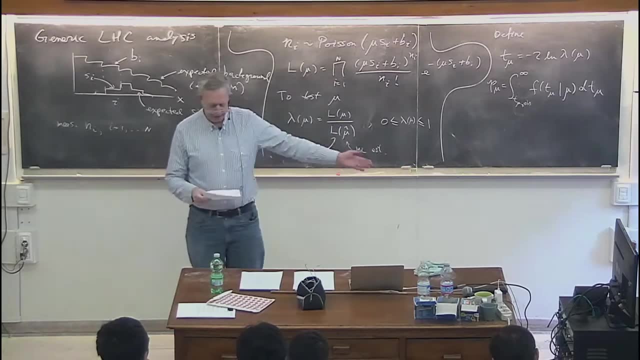 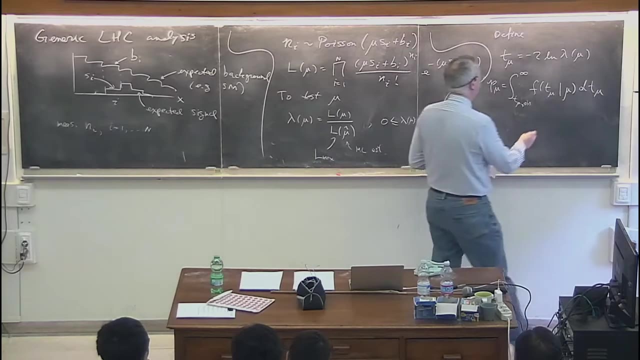 for the PDF of T mu under the assumption of mu. So that's going to be my p-value. If that p-value turns out to be less than some threshold alpha, I would reject the value of mu. But to do that I need this distribution. 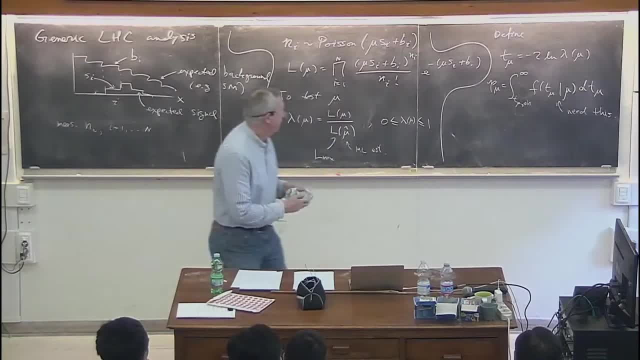 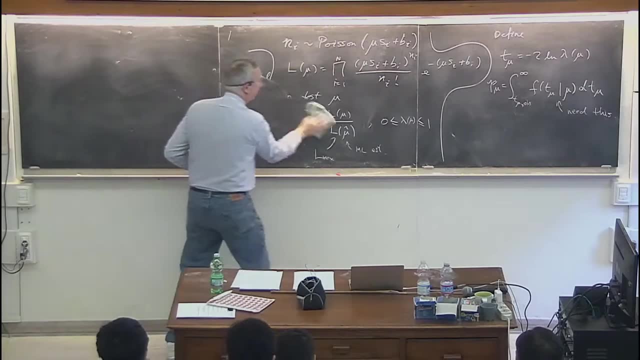 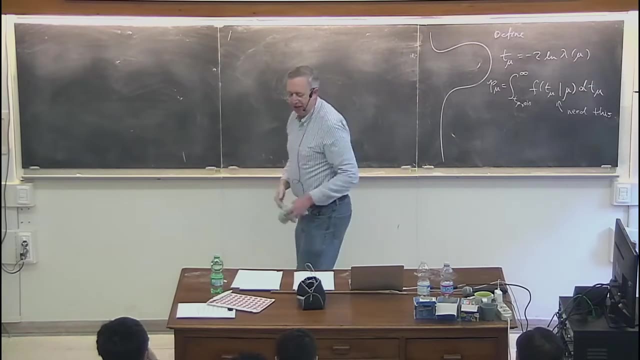 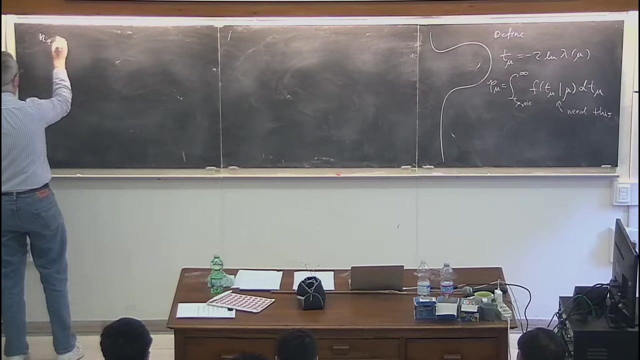 And, And that can either be easy or hard depending on the situation. Let's just think about that for a second. I shouldn't have erased that one equation, So remember that Here's the brute force way. Suppose that I remember that n sub i. 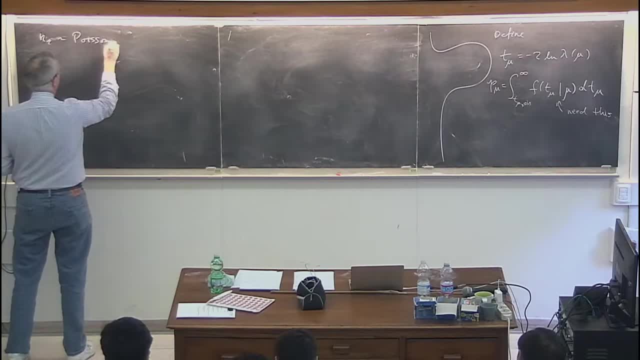 follows a Poisson distribution with a mean of mu s? i plus b? i, And the s? i's and the b? i's I've determined from Monte Carlo. Those are known constants now And I want to get a p-value for a given value of mu. 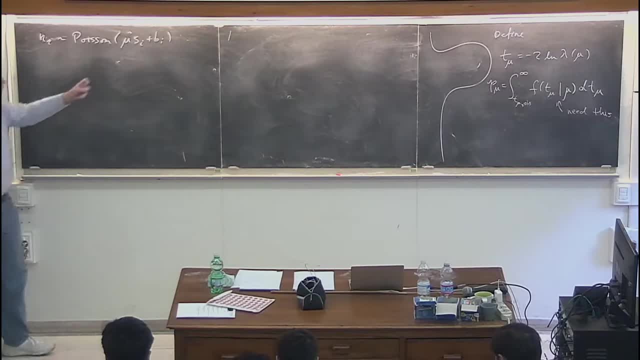 So you can imagine. one way of doing this is the following: Is put in the value of mu that you want to test. Generate a data sample, Generate the n? i's. But now you don't have to generate one number, You have to generate a number of n? i's. 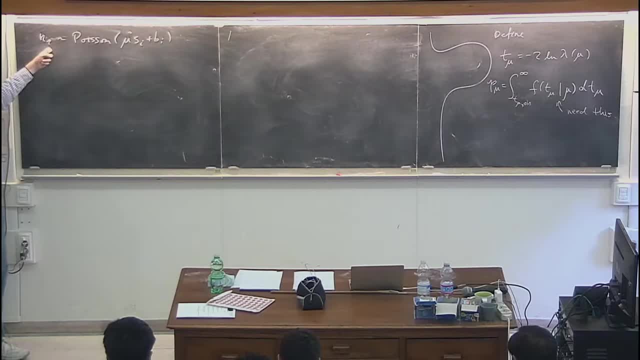 corresponding to each bin. So capital N of these n i's. Once you have that data set, you put it into the formula for T mu, You get a value for T mu And you plunk it into a histogram of T mu. 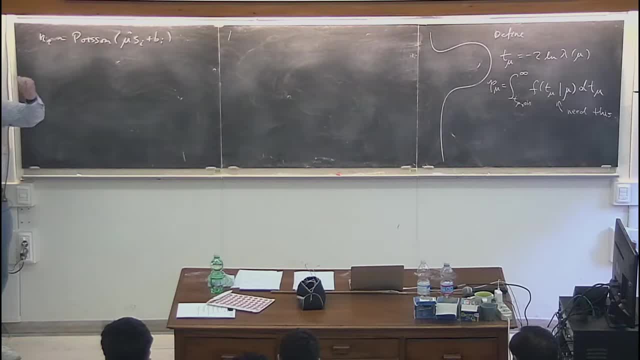 And then you go back and do it again. You do it a million times And in that way you get the distribution of T mu. So you get some sort of distribution that looks like this Right, And then you'd have the single T mu observed. 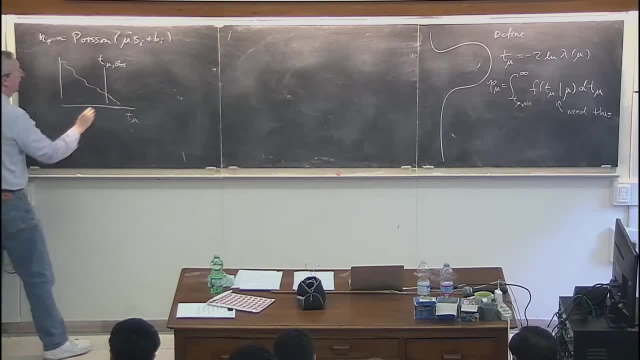 that you got from your real experiment, And then you'd simply calculate that probability. What's the probability to get T mu greater than or equal to the value that you found in your real experiment? Right, So this could be from Monte Carlo. We would typically call that toy Monte Carlo. 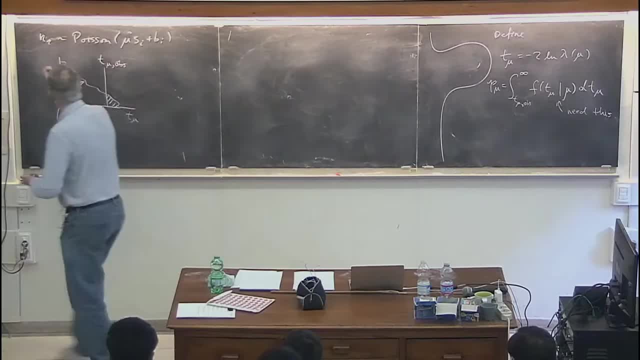 Right, Because I'm not simulating the entire experiment. I'm just simulating the data values n sub i. I don't have to go back and rerun some event generator or detector simulation That's already been done to determine the s? i's and the b? i's. 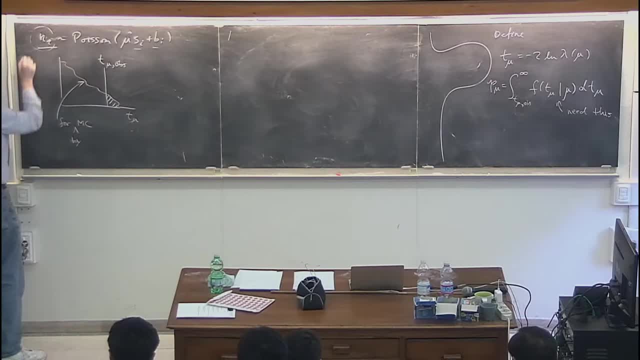 To determine one entry in this histogram, I just have to generate a set of n? i's And use those to get T mu Yes, So in the case of the first example, where we only had one value of n, I didn't bother to form a statistic. 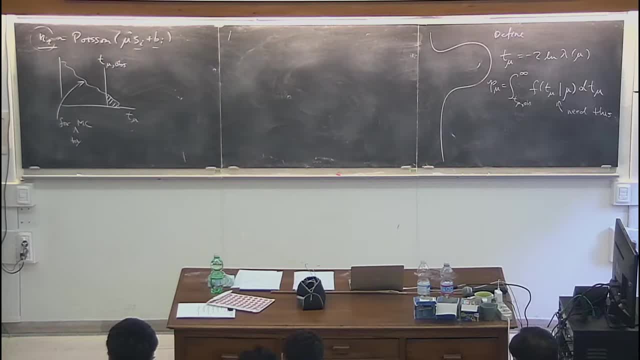 because the value of n itself could be used as that statistic. Okay, I could have, But here, once I have a multidimensional data space, then it's not obvious what to do. Should I say that in the case of the single n? 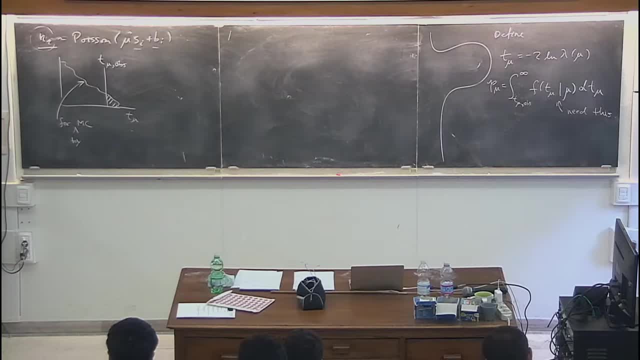 I said the region of lesser compatibility was n less than or equal to n. observed, Right. But then if I have n1, n2, n3, n4, well, how about? like, if n3 was a little low and n4 was a bit high? 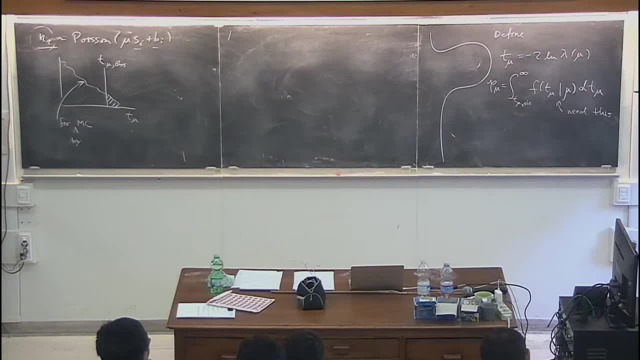 it becomes more difficult to establish the region of data values that you count as having lesser compatibility There, then I need some sort of a statistic like this Now to do this. I say it's toy, Monte Carlo, so it's pretty fast and you could do this. 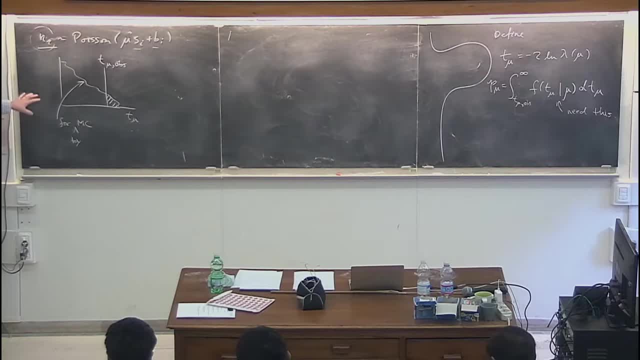 but it's still a bit of a pain in the neck that you have to write a Monte Carlo program and do this calculation. And it turns out that there's a wonderful theorem that will make this unnecessary in many cases of interest, and that's called Wilk's Theorem. 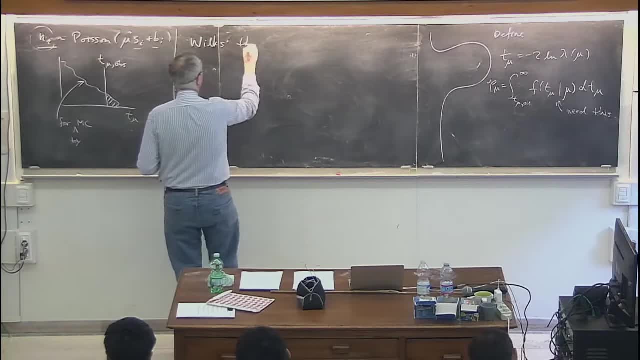 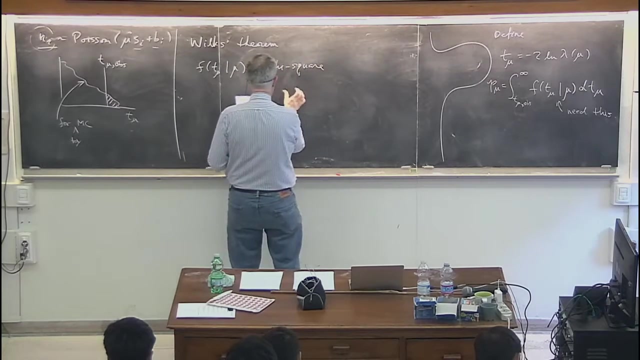 This is from the 1940s or something. There's a reference in the lecture notes, A very famous theorem which says that the PDF of T mu, under the assumption of mu, is a chi-square distribution. Chi-square distribution And the assumption of mu is a chi-square distribution. 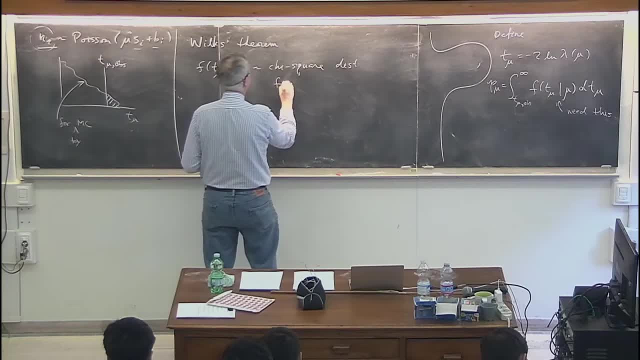 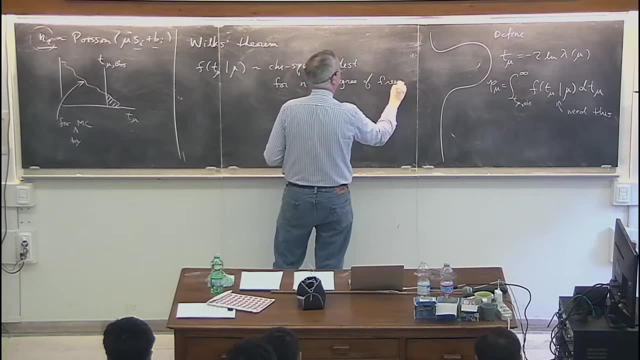 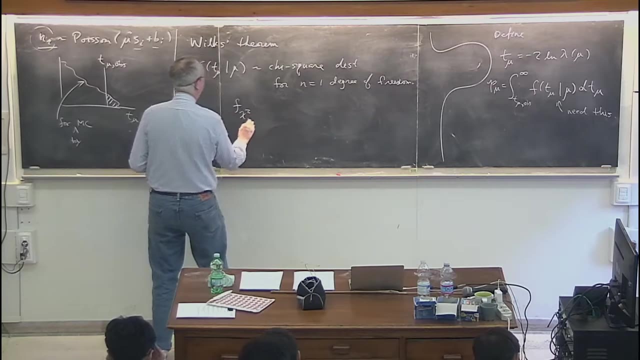 And the assumption of mu is a chi-square distribution For one degree of freedom, in this case Degree of freedom. I'll just remind you what this chi-square distribution looks like. So the chi-square distribution for n degrees of freedom. I'll always use this notation for a chi-square distribution. 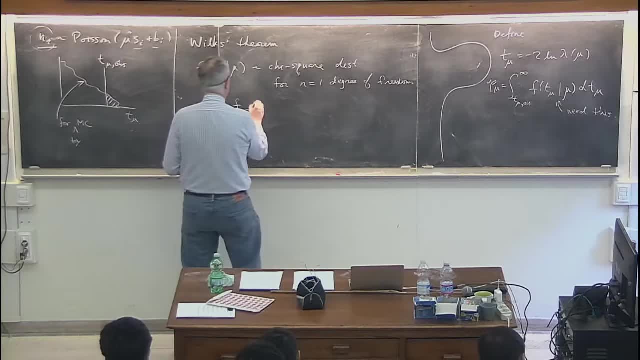 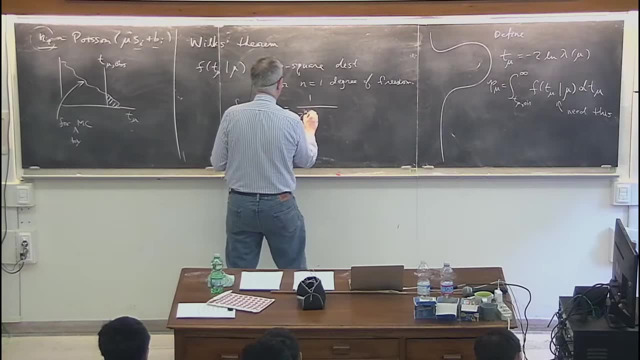 for n degrees of freedom. I'll write it down. I'll call the variable T mu. It's just the following: One over two, T mu to the n over two. Gamma of n over two. That's just a normalization factor. 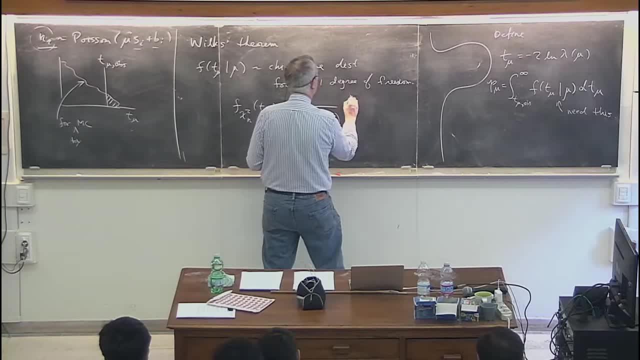 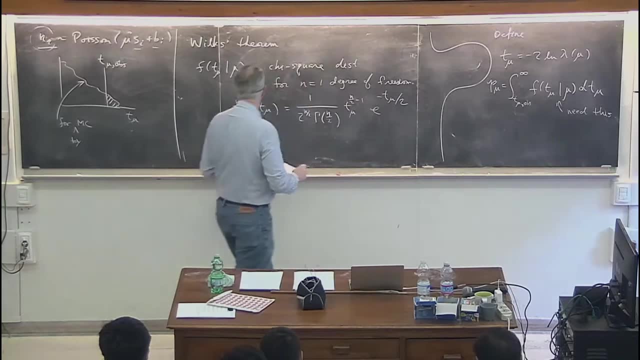 And then it's got a power law term, So T? mu to the n over two minus one, And then an exponential term, T to the minus T mu over two. And so what Wilk's Theorem says is that this distribution is a chi-square distribution, for n equals one. 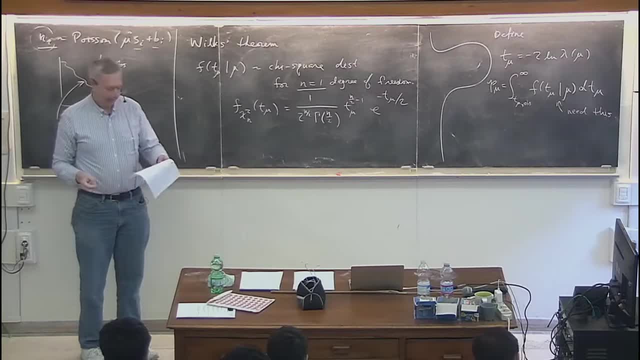 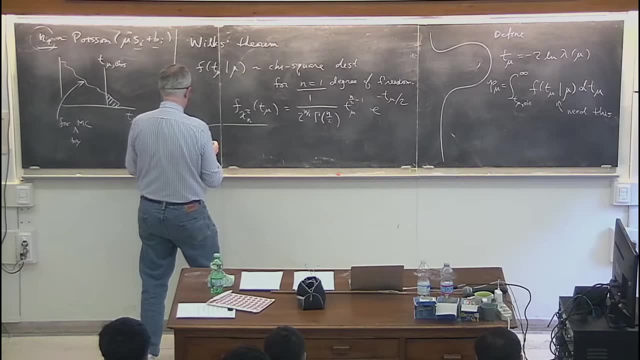 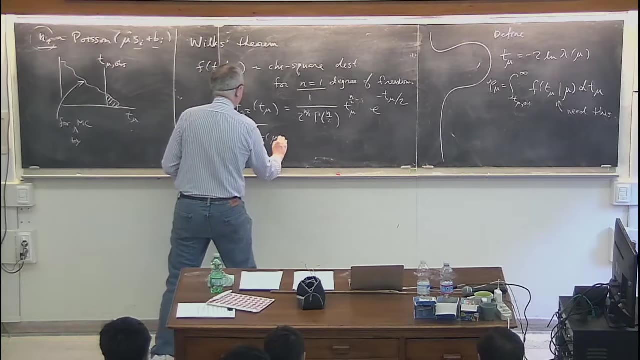 So you substitute in n equals one In the case. we're going to also deal with the case if you had more than one parameter of interest. So if instead of mu I had a vector of parameters, let's say mu, one through mu. 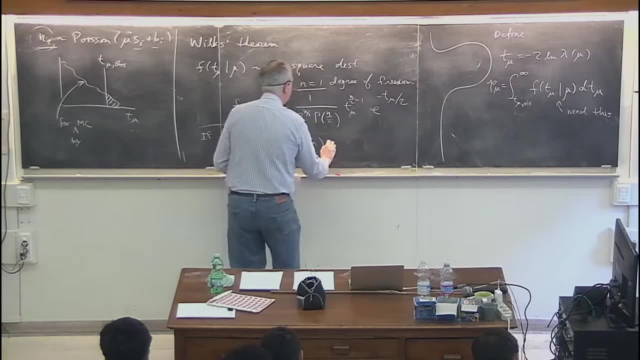 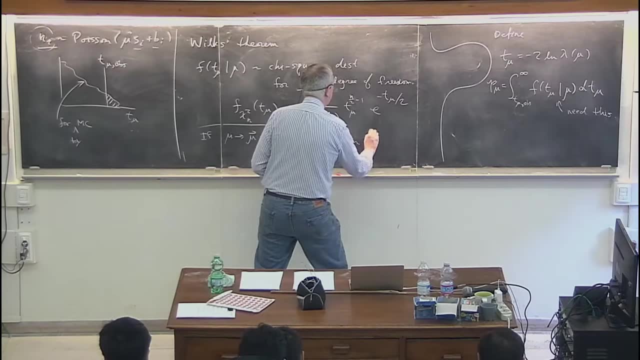 I've used n already here, so I better call it m. Then the corresponding statistic that I'll call T sub mu vector is going to follow a chi-square distribution for m degrees of freedom. So it's the number of parameters of interest gives you. 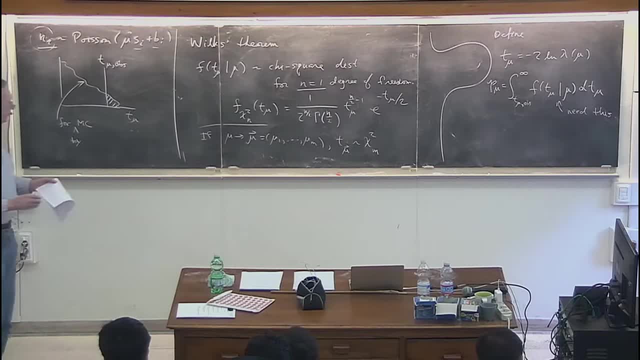 the number of degrees of freedom for the chi-square distribution. Okay, It's unfortunate that this term chi-squared gets overused. in statistics and data analysis. It is, I think, first and foremost the name of a particular distribution, But we've also used the term chi-squared to refer to that sum of squares. 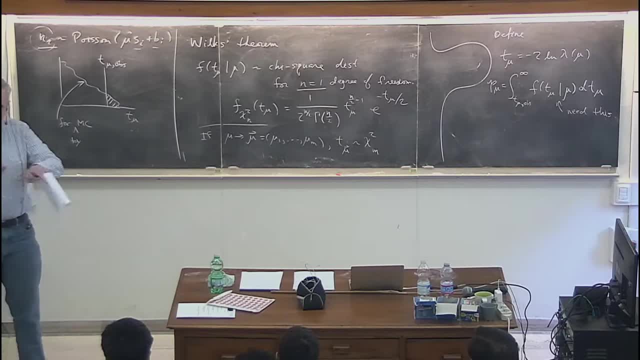 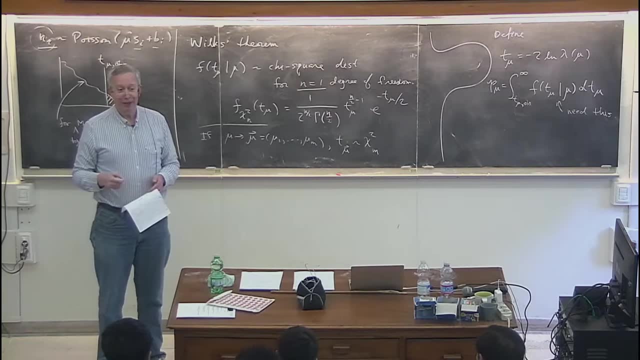 that you minimize, say, in the method of least squares, So don't get those confused. I mean, there's a reason for that and that is that the minimized chi-squared, if you're a chi-squared, if you were to repeat the experiment many times, 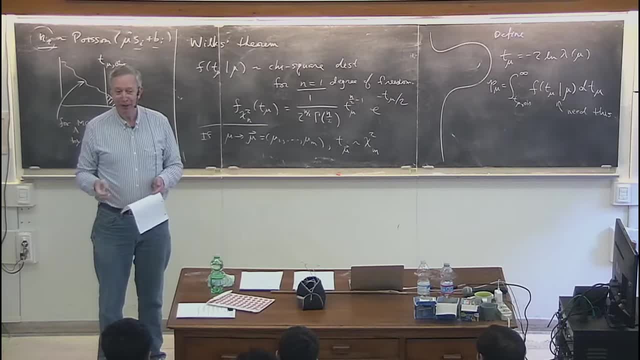 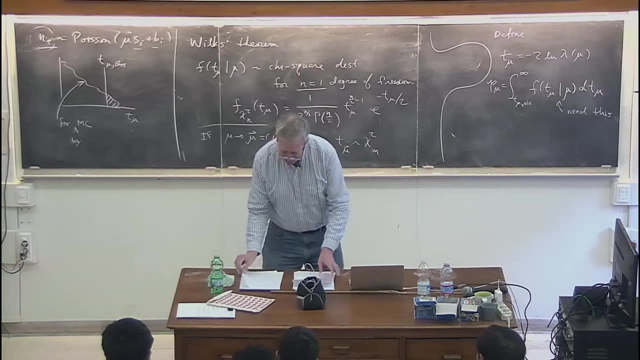 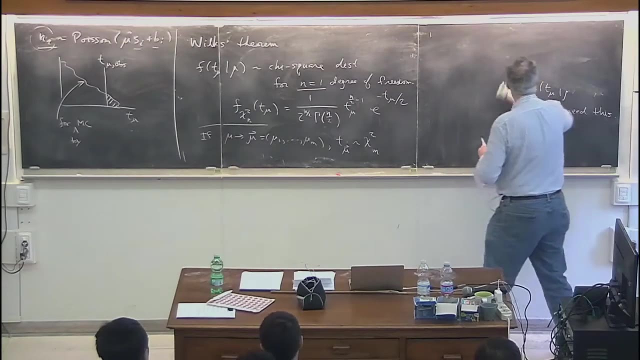 and get a minimized chi-squared every time. guess what distribution it follows: The chi-squared distribution. So that's the motivation of that. So back to this problem. I now assert that this statistic, T mu, follows a chi-squared distribution for one degree of freedom. 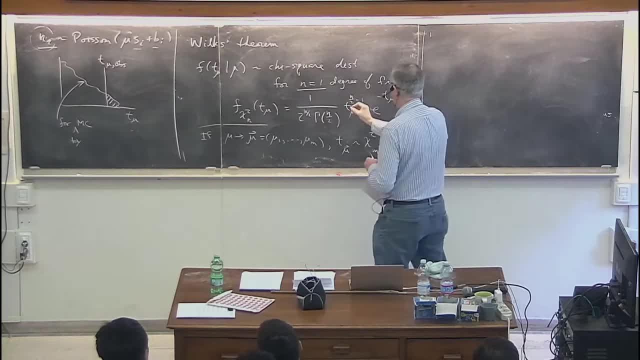 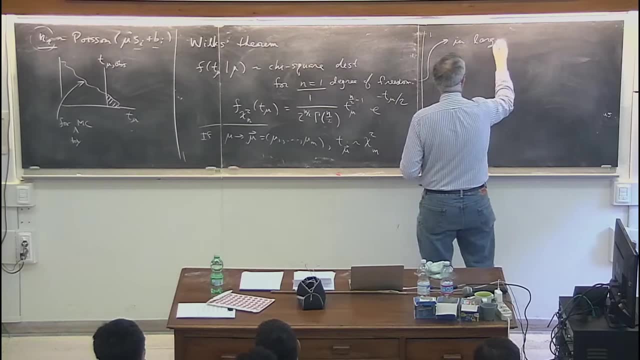 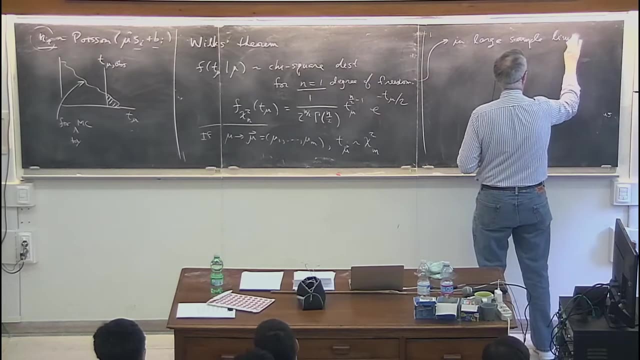 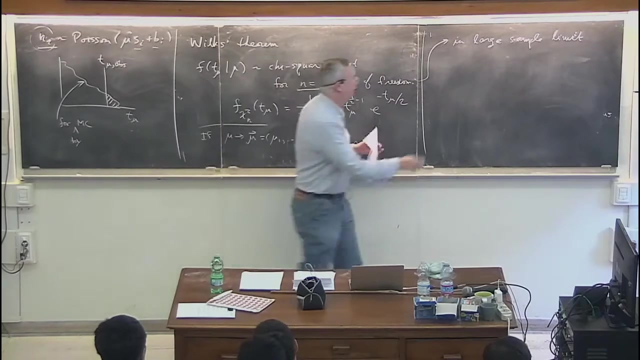 in a certain limiting case. So it follows chi-squared distribution for one degree of freedom in the large sample limit. So in this particular case that's going to mean when I have lots of data, Let's just leave it at that. 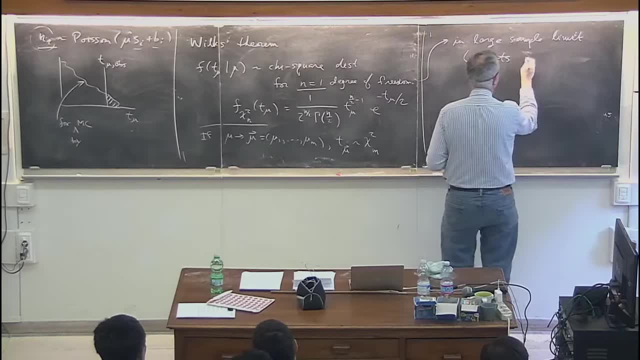 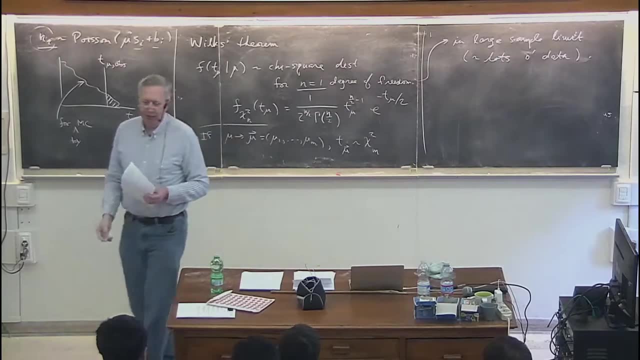 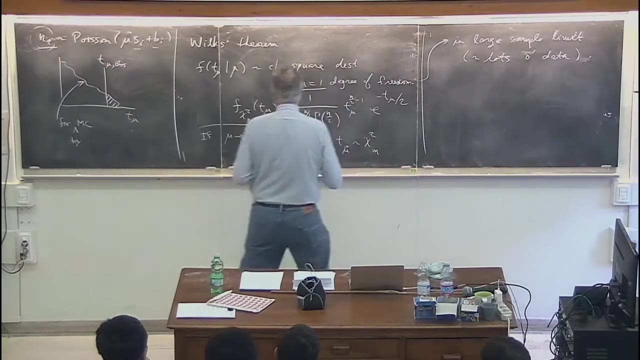 Lots of data. There are some other regularity conditions that have to be satisfied and it's all a bit complicated. In practice it's going to boil down to this: If I have a large data sample, then in that limiting case, 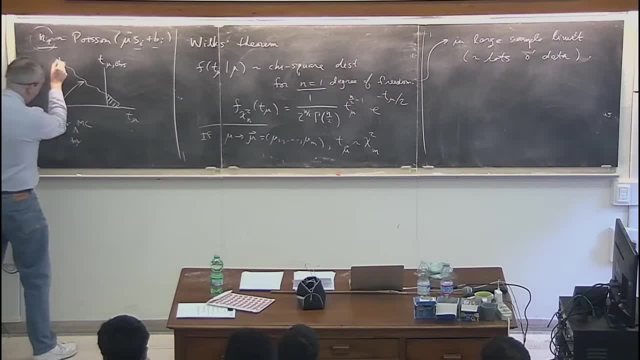 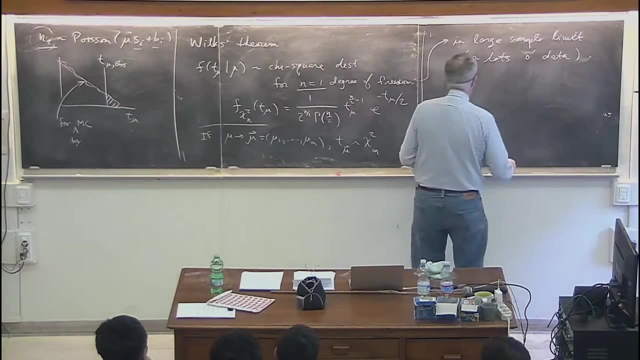 I don't have to do my toy Monte Carlo. I can just say: ah, it's a chi-squared distribution And that's much quicker, So let's suppose that that's the case. The p-value that I would need is: 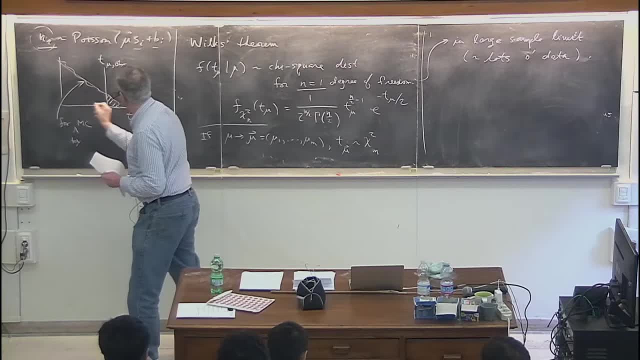 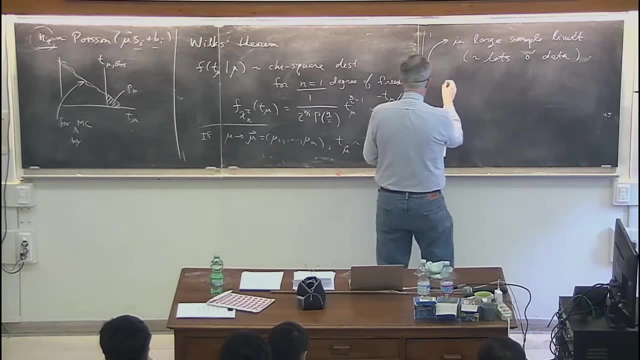 let's say the cumulative distribution is the integral from zero up to here. So the p-value is one minus the cumulative distribution. So the p-value is going to be one minus the cumulative distribution for a chi-squared distributed variable for one degree of freedom of t mu. 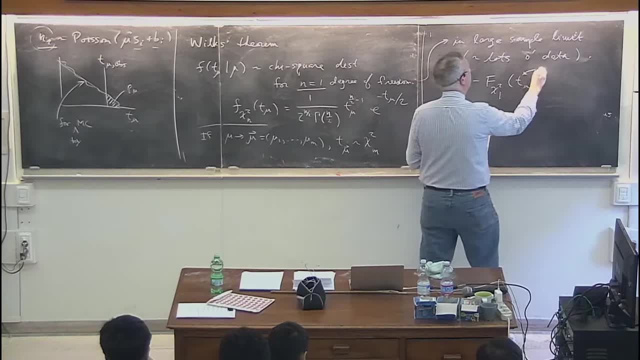 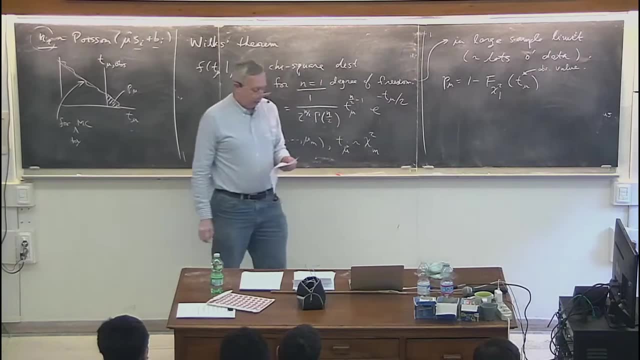 So I'm going to drop the subscript observed. When I now write t mu, I mean the observed value. All right, and I now want to find the value. I can do this for a given value of mu. I can repeat that for all values of mu. 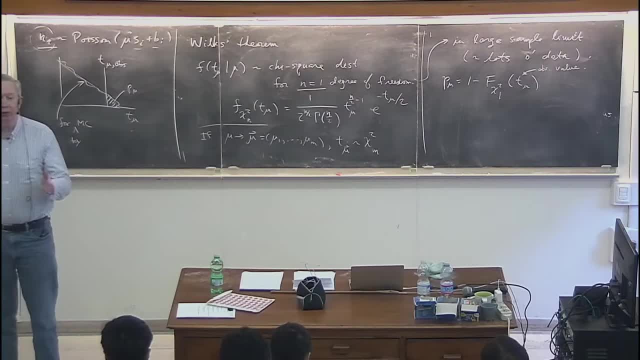 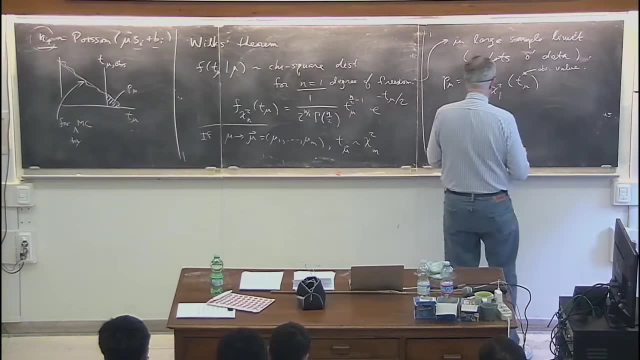 And I can find the value of mu that has a p-value just equal to 5%, just equal to alpha, And that would be the boundary of my confidence interval. So if I set this equal to alpha, set right, And I can then solve this equation for t mu. 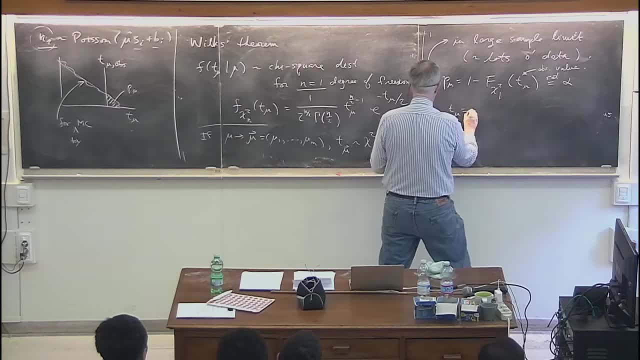 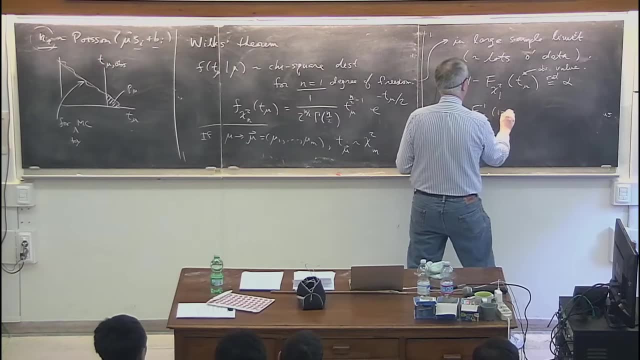 That's the first thing I could do. I can say, therefore: t? mu is equal to f inverse quantile of the chi-squared distribution of one minus alpha right. So that's easy, Assuming that I have access to some computer routine. 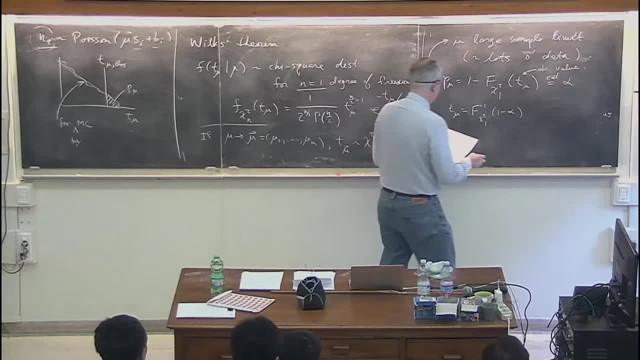 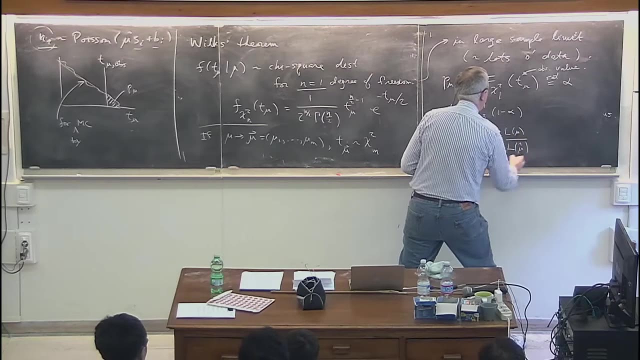 that gives me this quantile, which I do, But then also remember the way that I've defined. so I'll say also: the definition of t? mu was the following: This is equal to minus two times the log of l of mu divided by l of mu hat. 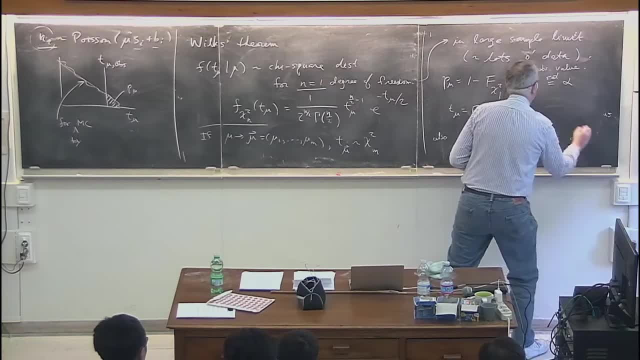 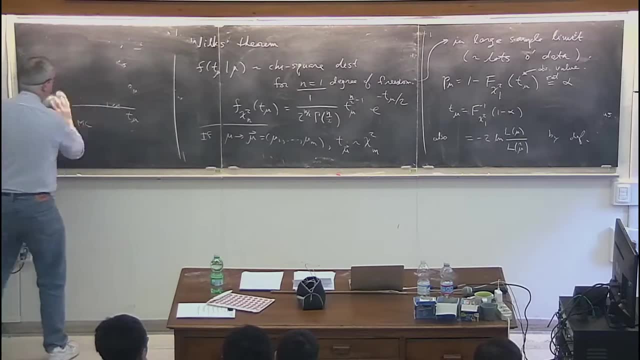 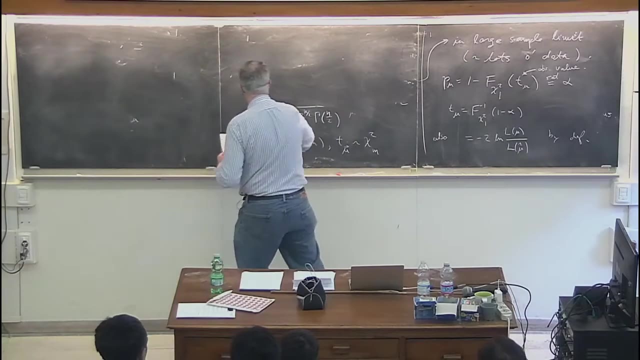 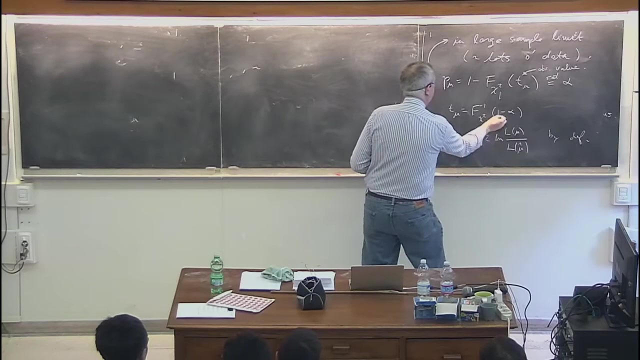 Okay, By definition, that was how I defined the statistic, And so if I want to know the value of mu that defines the boundary of that region, I can just take: let's see, this is equal to that And I'm going to solve for l of mu. 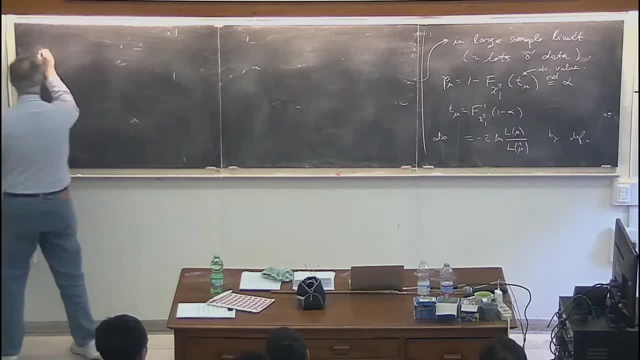 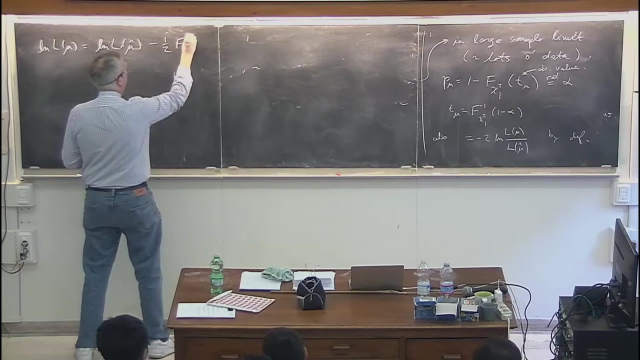 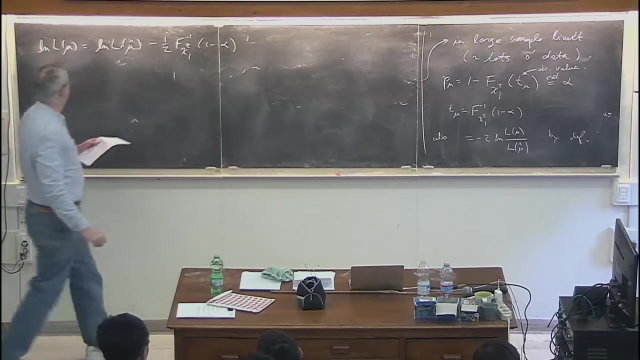 I'm going to solve for the log of l of mu. actually, The boundary is characterized by log l of mu, equal to log l of mu hat minus one half times the chi-squared quantile for one degree of freedom. one minus alpha. There we go. 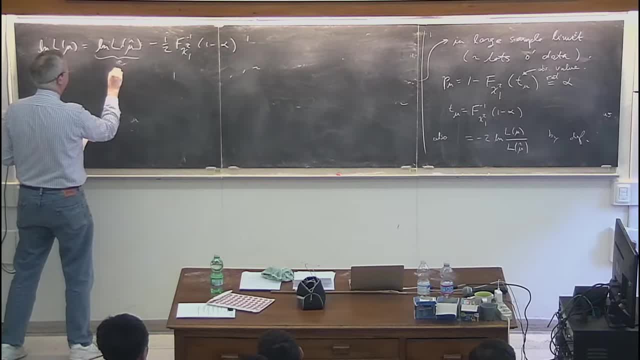 So this here, of course, you just recognize as the maximum of the log likelihood function, Right, And so what it says is to find the value of mu. that gives you a p-value of exactly alpha. What you do is you first, you find the place. 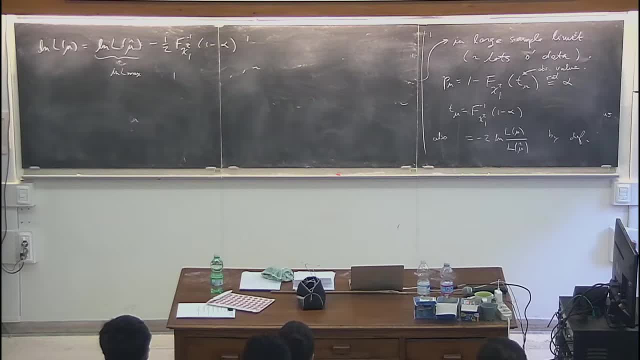 the value of mu, that maximizes your likelihood function, Right. And then you move away from that until the log likelihood function decreases from its maximum by a certain amount. So this you've decided on alpha It's five percent, And so this is just some number. 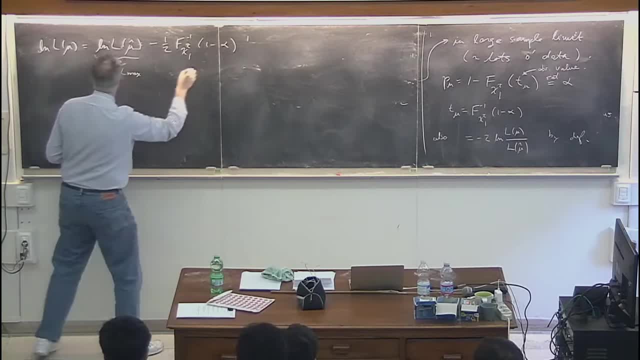 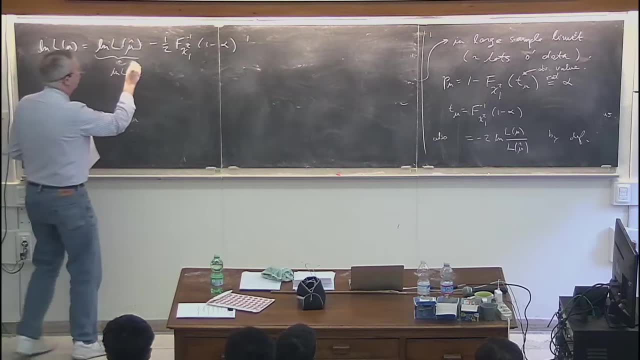 And for certain values of alpha. we'll see that this is a number of order units. This is a number of order unity. So the point is that there's just a given offset that you have to use. You move mu away from mu hat until log l decreases by that amount. 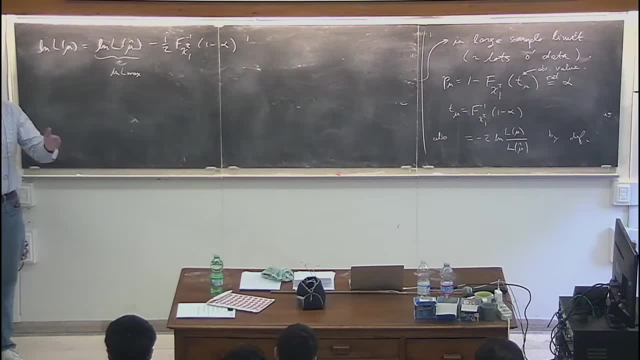 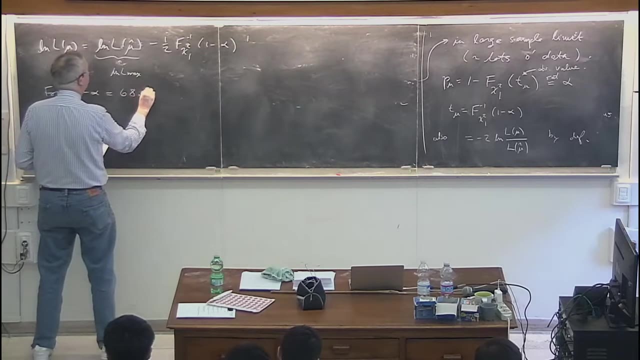 And so that's the recipe, That's a very simple recipe for giving you the bounds of this confidence interval. So, for example, there's an important example is that if I take one minus alpha to be 68.3 percent, then what you can show is the following: 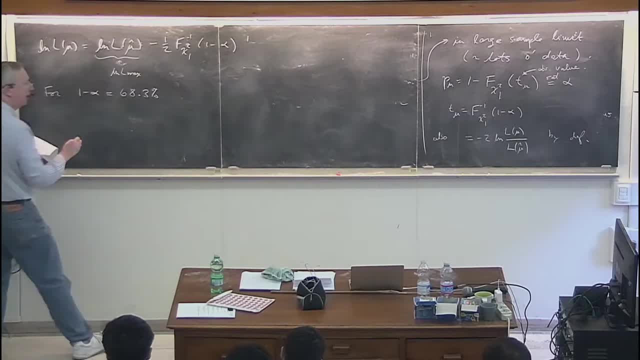 First of all, let me show the following. Let me define a number, a, to be the number of standard deviations, such that when I integrate a Gaussian between those limits, I get a certain one minus alpha. So I say that one minus alpha is equal to say: 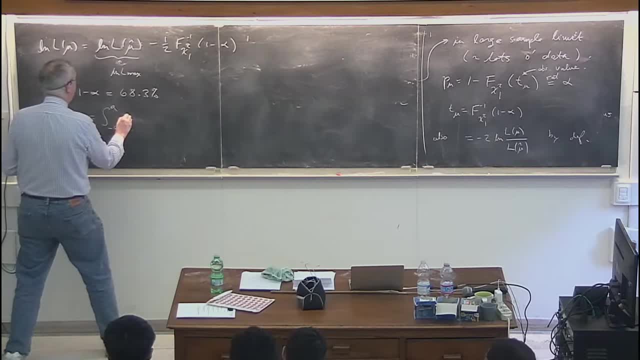 the integral from some quantity minus a to a of the standard Gaussian distribution. Let me call that little phi, as I've done before. So that defines the number of standard deviations of a Gaussian between which I contain an area one minus alpha. What you can show is that if x follows a Gaussian here, 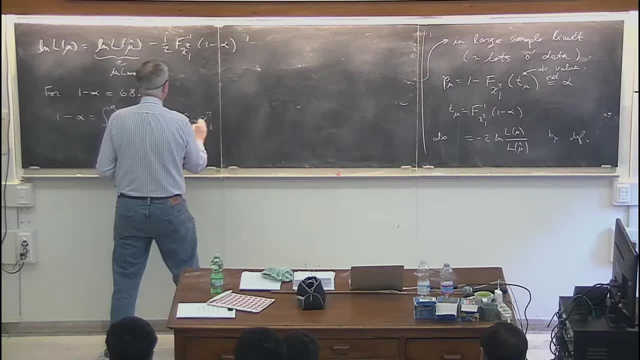 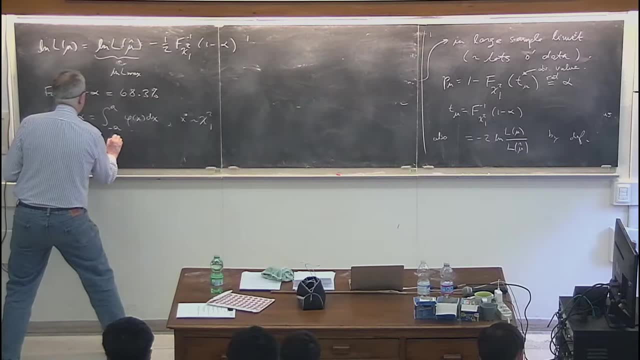 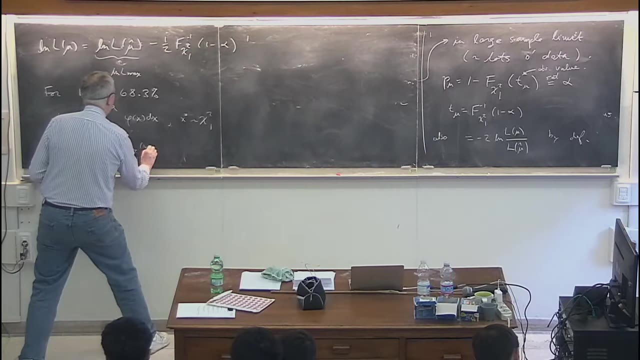 then x squared follows a chi-squared distribution for one degree of freedom, And what that means, then, is that this is equal to the integral, from zero to a, of the chi-squared distribution for one degree of freedom. Let me call that. call it y. 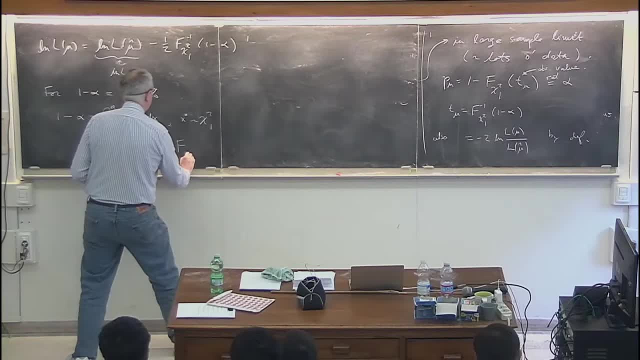 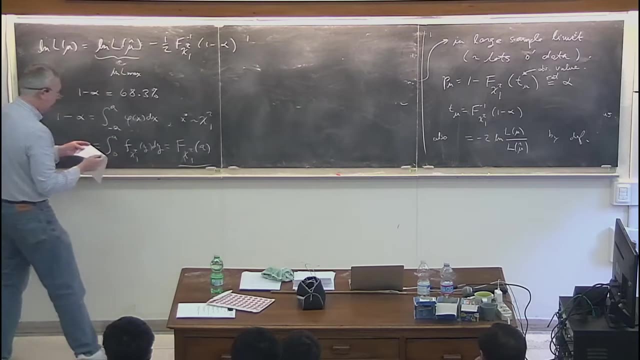 And so this is then just equal to the chi-squared cumulative distribution for one degree of freedom up to that value, a. So if I define a as the number of standard deviations between which I contain a certain area, then this equation also holds, And so what that means is that this one minus alpha, 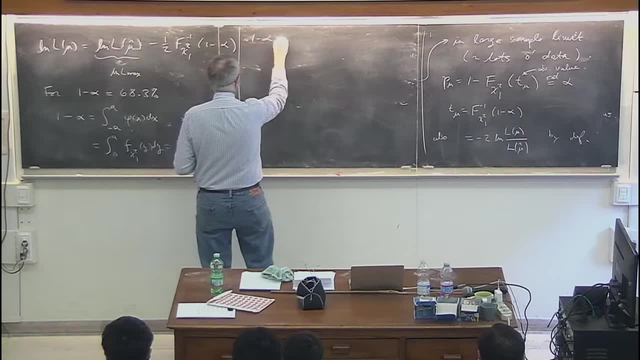 shall I write this now? the corresponding one minus alpha is just equal to the standard normal. sorry, the chi-squared quantile: Bah, Let me make sure I write this correctly. That's what I just said. Yes, sorry, let me say this right. 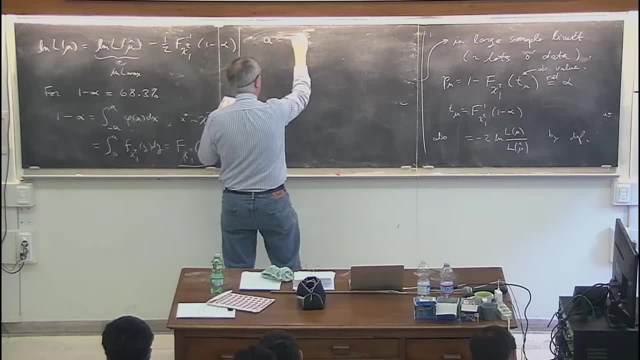 Therefore, that number of standard deviations is equal to the chi-squared quantile- that's what I wanted to say- of one minus alpha. There we go, Skipped a few steps in the derivation, but that's true, And the steps that I skipped are: 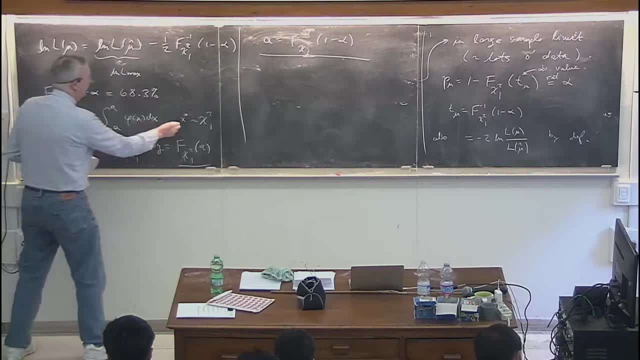 I've asserted that if x follows a Gaussian distribution, then x, squared, follows a chi-squared distribution. for one degree of freedom. That's a simple exercise that you can work out All right, and what that means is the following: is that if I take a to be one, 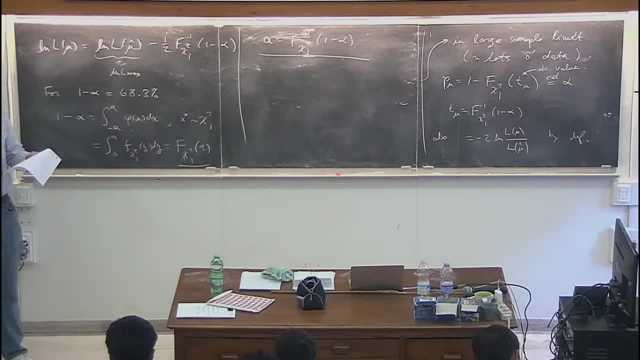 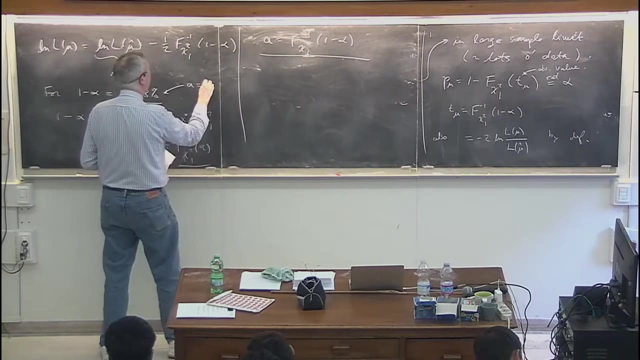 that is to say then the- I'm talking about the area between plus or minus one standard deviation. for a Gaussian that is 68.3%. So this course, this situation here corresponds to a equals one: the area between plus or minus one standard deviation. 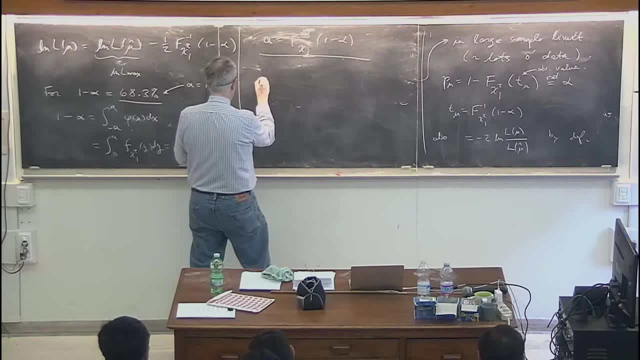 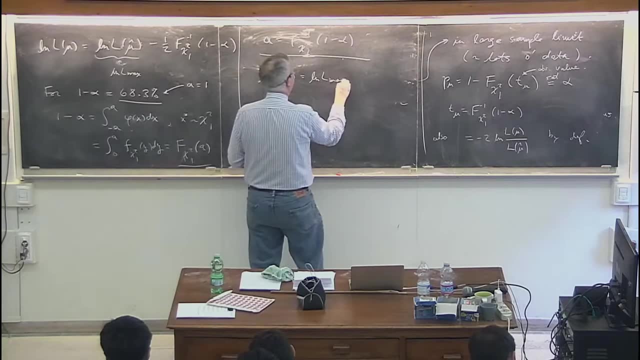 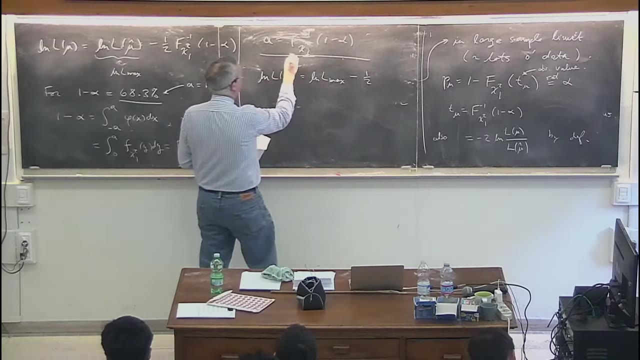 So therefore I get in that case that log L of mu is equal to log L, max minus one half times one right. So in that case that if that is equal to 68.3%, then this is equal to one. 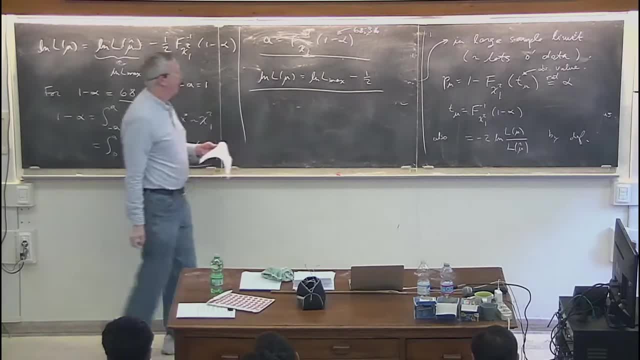 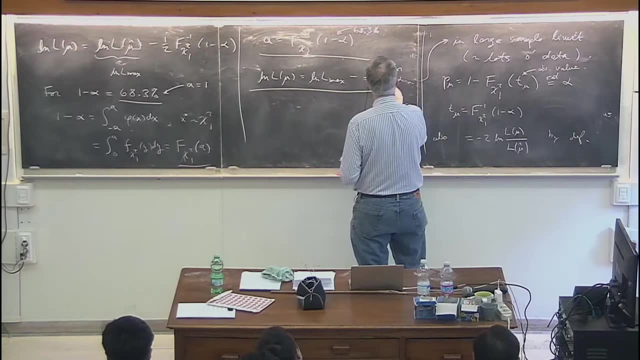 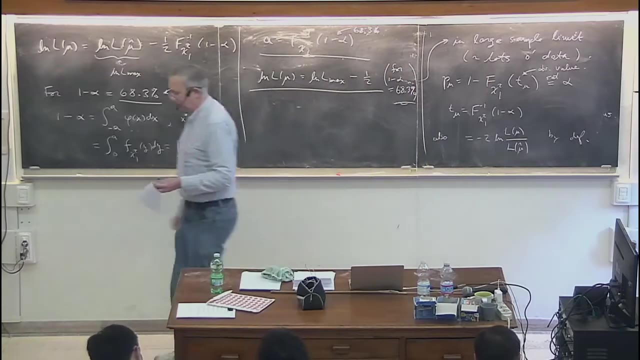 So times one, And that's then my recipe. Okay, So say four, Right, So to get the endpoints of the interval to correspond to a confidence level, a level of 68.3%, you move mu away from the maximum likelihood estimator. 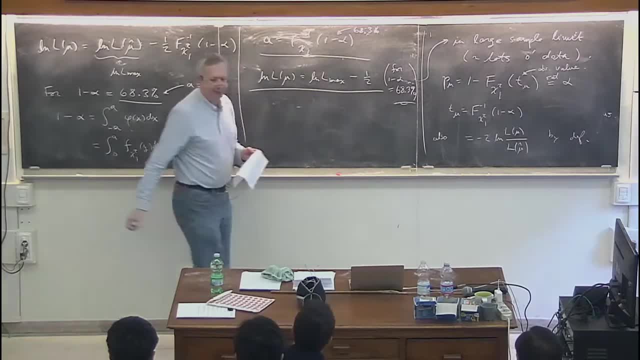 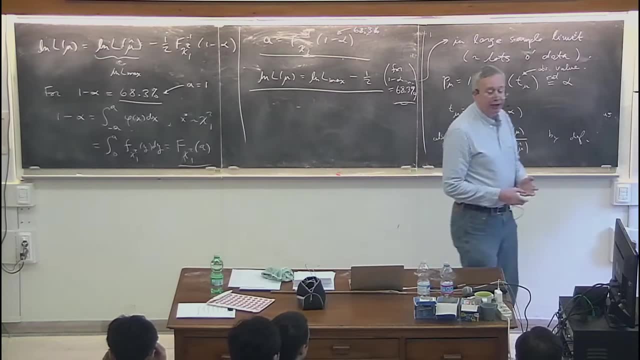 until the log likelihood goes down by one half. Okay, And that seems that should sound similar to the recipe that we talked about two days ago for finding the standard deviation of a maximum likelihood estimator. We said that that was the same recipe that you use. 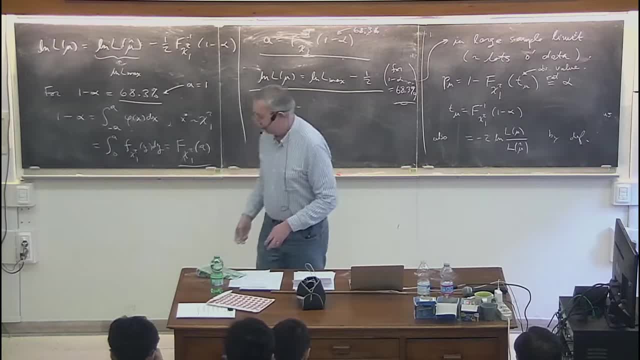 So the two things coincide in that limit That if you have a maximum likelihood estimator, say theta hat, and you have its standard deviation sigma theta hat, then what that tells you is that theta hat minus sigma theta hat, up to theta hat plus sigma theta hat. 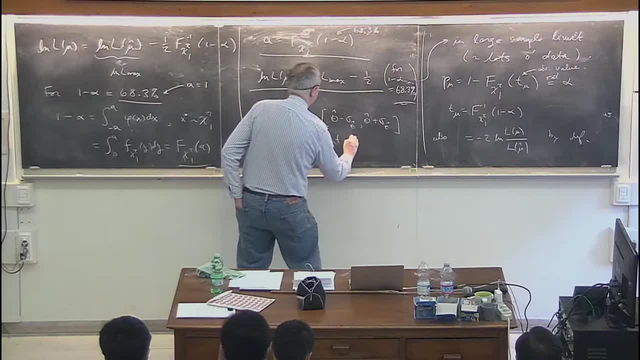 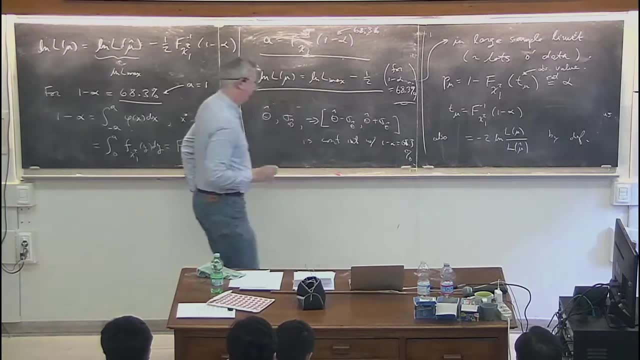 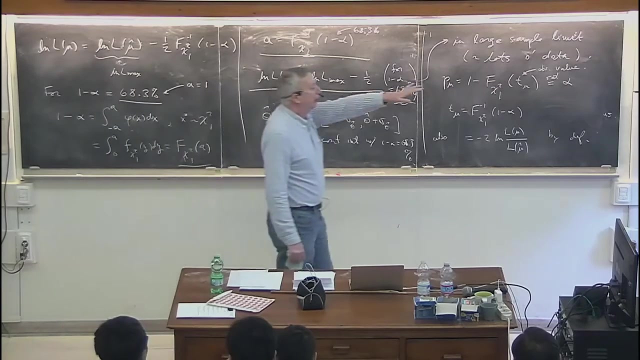 is a confidence interval. with one minus alpha equals 68.3%. Now, in the case where you have a fairly small data sample, this can still be used, but then the approximation of the chi-square distribution might not be exact, But this is what's very often done in practice. 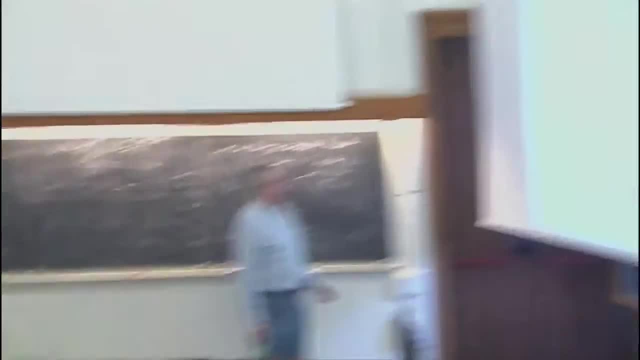 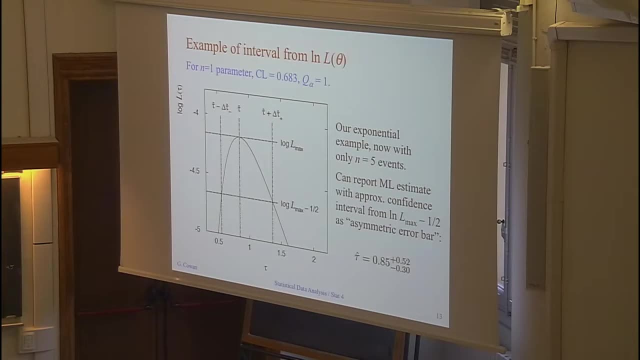 And so now, if you can see the example that we have here, this is the same example we worked out two days ago with the exponential distribution, And I said that the numbers I gave you in that example were with 50 events, And here what I've done is I've repeated it. 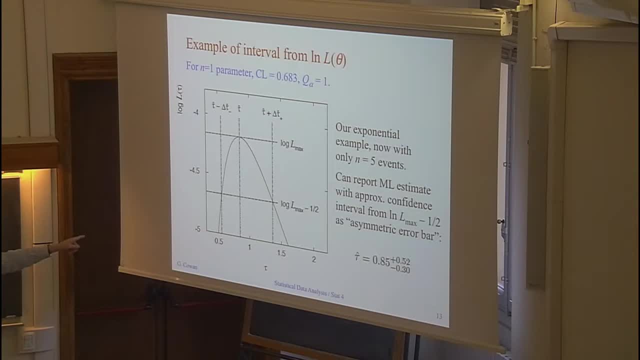 with only five events. And so here now is the log likelihood function as a function of the parameter. So remember we called it tau, which represented the mean lifetime of some particle, say. And so now you can see that this log likelihood function is noticeably asymmetric. 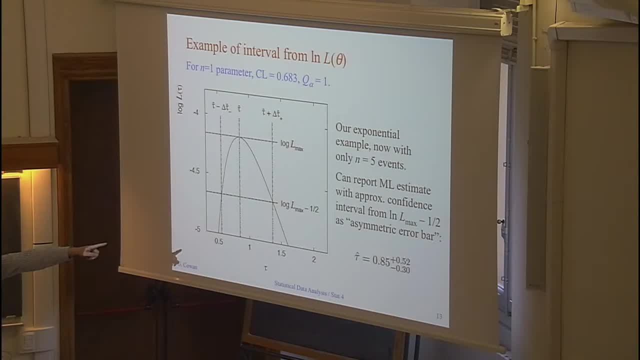 And so now there's what I call delta tau minus on the left and delta tau plus on the right. And now, because they're sufficiently different, you probably wouldn't want to just average the two numbers and report that as the standard deviation. What would make more sense in this case? 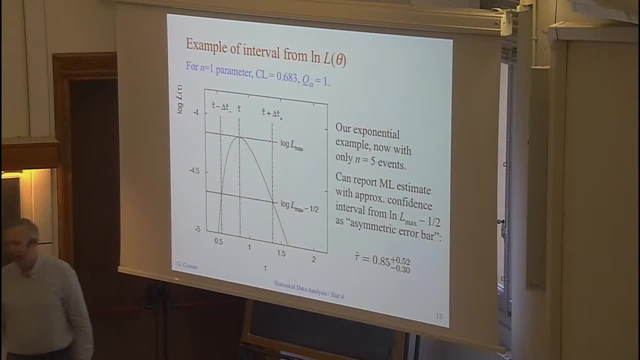 would be to actually report the full interval, say from here to here, and to assert that that is an approximate 68.3% confidence interval. And the way that's very often written is with these sort of asymmetric error bars You would give the central number. 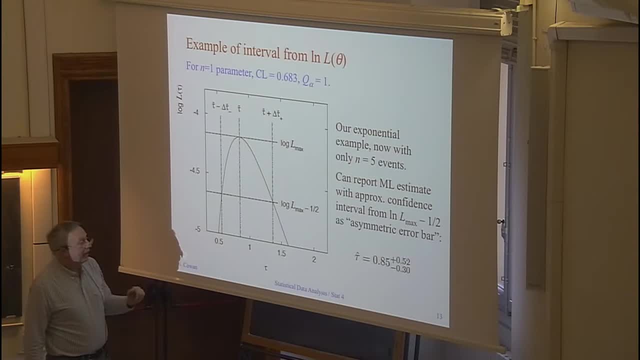 that corresponds to the maximum likelihood estimate, and then that plus 0.52 gives you this point and that minus 0.30 gives you this point, And so the way to interpret that is a 68.3% confidence interval. I need to remember to throw in the word approximate. 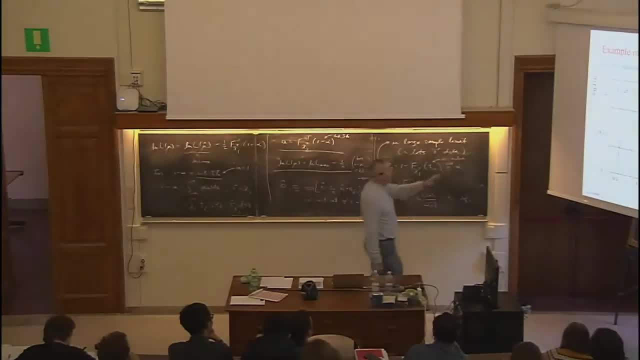 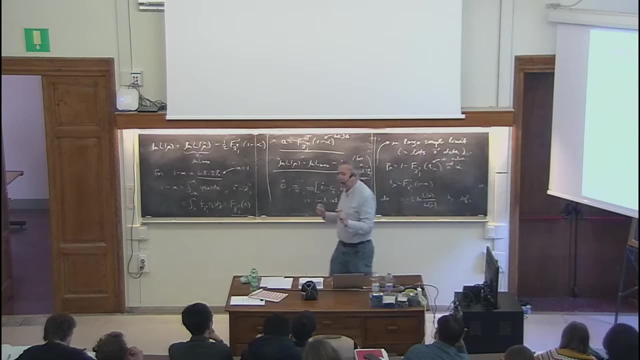 And the reason that it's approximate is because this is a function and this is a small data sample. The asymptotic form which you get from Wilk's theorem doesn't necessarily apply. So Wilk's theorem, this idea that the test statistic follows a chi-square distribution, 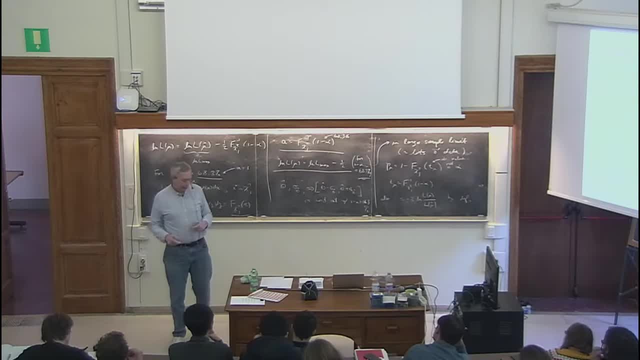 holds in the large sample limit, And here I have a small sample, And so the question is then: how good of an approximation would this be? And we've done many Monte Carlo studies to investigate this, and it's surprising how, for even a relatively small data sample. 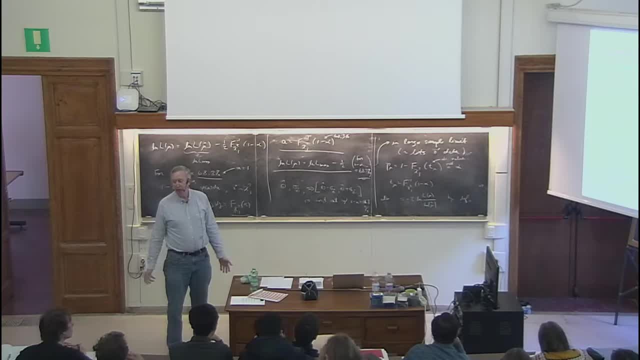 even say with five events, this would be a very good approximation to a 68.3% confidence interval. So in some sense that's. the miracle of Wilk's theorem is that even though the formula only holds in the infinite data sample limit, 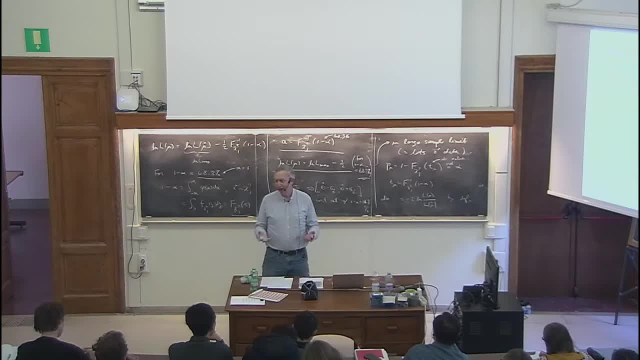 in practice, it's an excellent approximation for very moderate to small size data samples. Okay, let's keep going, Right, It's now 12.30.. When am I supposed to stop? Until they drop dead, or what? No, no, seriously. 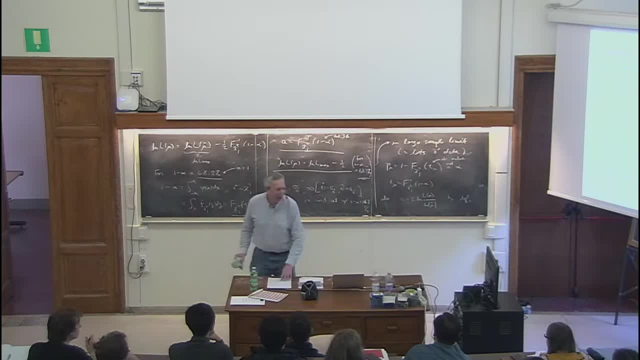 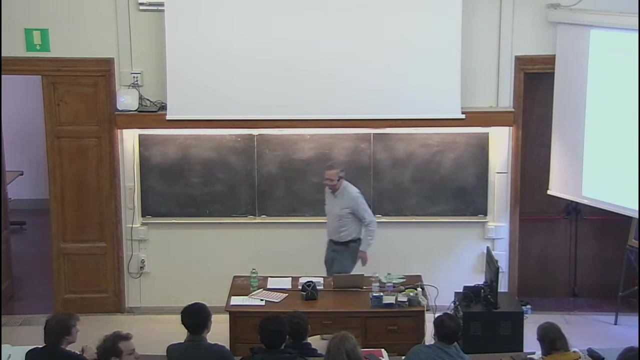 All right, Yeah, no, we're good, We're good, Okay, Okay. so what I can go over fairly quickly is the extension. Ah, no, sorry, Before I go there, I want to show a couple of tables while we're still on the projector. 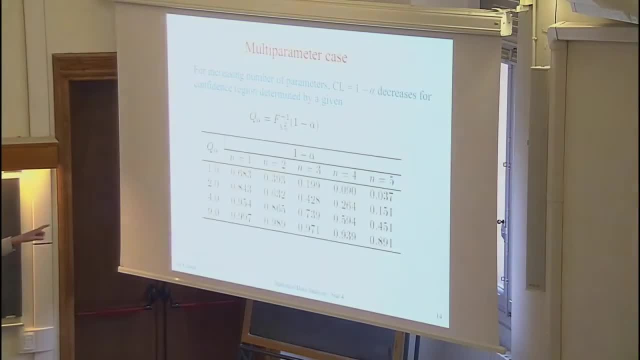 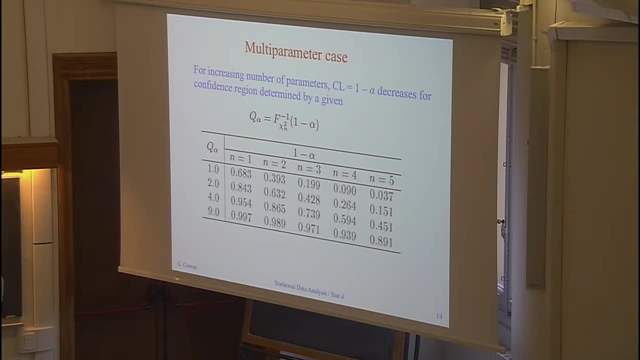 This number that I've put on the board, this chi-squared quantile for n degrees of freedom. that's the number that multiplies the one-half and it tells you how far you have to move the parameter away from the maximum in order to get the boundary of the confidence interval. 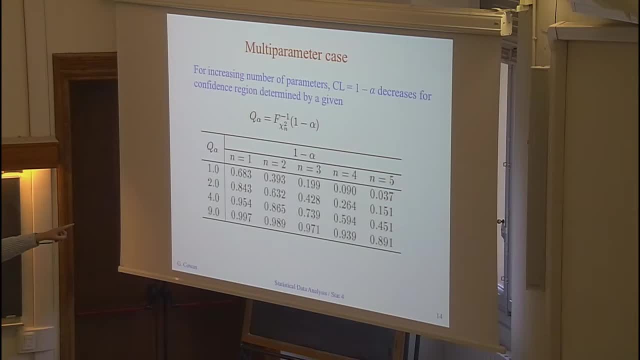 And what we just said was that for one parameter, and if you want a 68.3% value for one minus alpha, that corresponds to a value of this quantile of 1.0.. So it's important to know that value because it comes up very often. 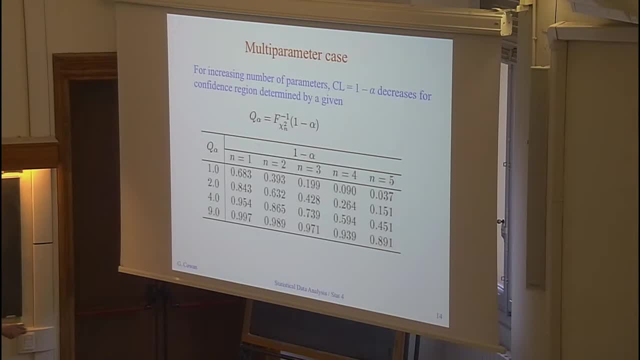 The one parameter case is in some sense the most important. If you had more parameters, say a two-parameter problem, a three-parameter, then what this tells you is that the corresponding quantile, if you set the corresponding quantile to one, always 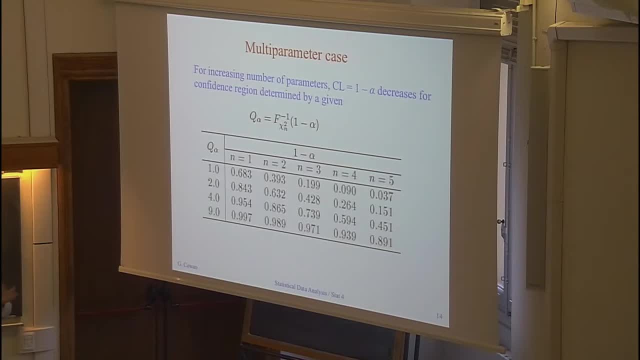 then the one minus alpha, which is the confidence level, gets smaller and smaller. If you form the region using log L equals log L max minus one-half, which corresponds to Q alpha of one, then the probability that such a region will actually bracket the true value of the parameter. 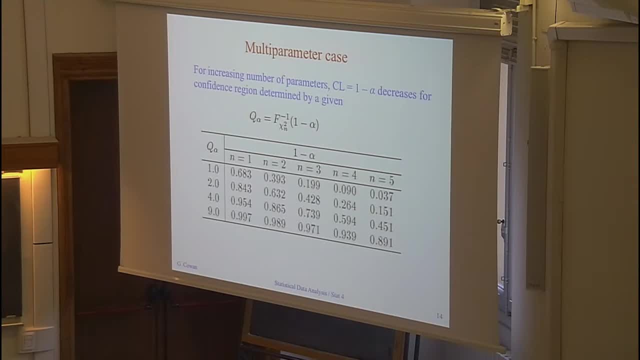 decreases as the dimensionality of the parameter space increases, And you can kind of imagine how that works, because, as you have a higher dimensional parameter space- and here's the point that I want to bracket- and here's this hyper-ellipsoid that I want to put around it- 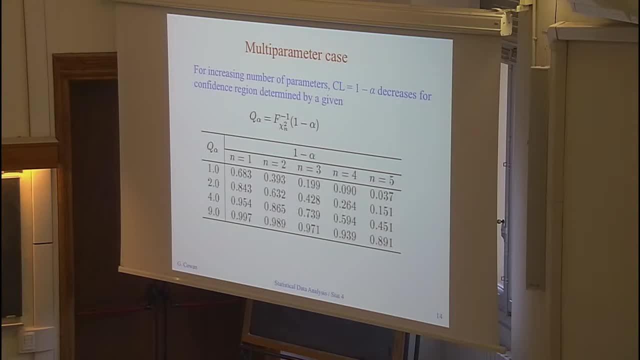 there are different ways that I can miss. I can be too high or too low, but maybe in height it's correct, but then I'm off by being too far to the left or too far to the right, And as you increase the dimensionality of the parameter space. 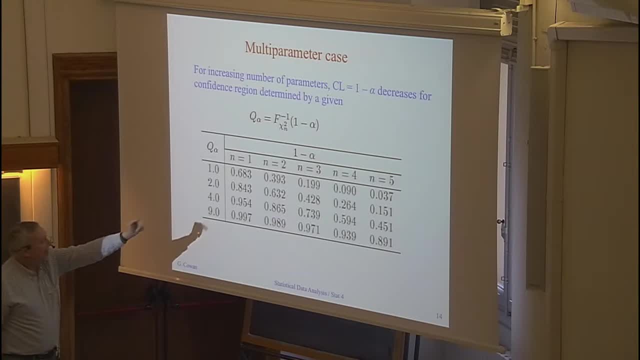 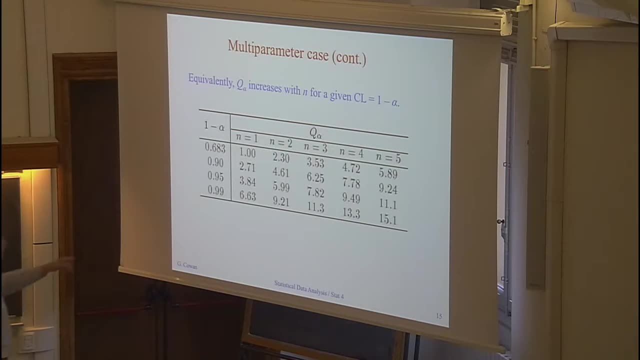 there are more ways to miss, And that's what's reflected here. So that table gives you the values. Very often what we want to do is we want to set one minus alpha- the confidence level to some convenient value like 90% or 95%. 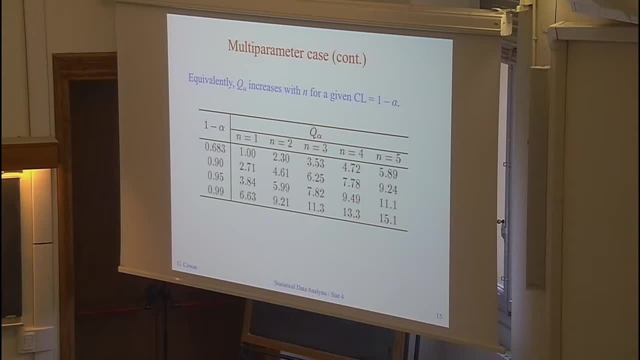 And then we would like to know: well, all right, how far do you have to move the parameter, How far do you have to get the log likelihood to decrease, And this tells you then, in this table, what the corresponding value of that quantile would have to be. 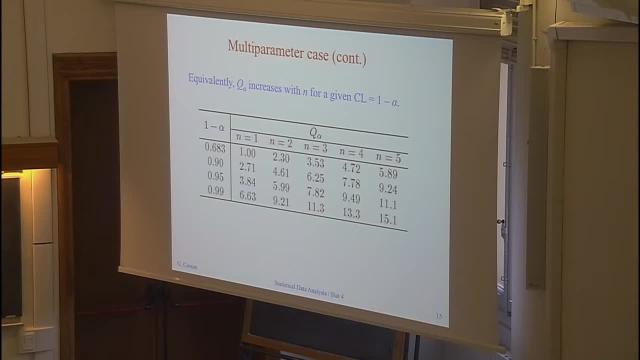 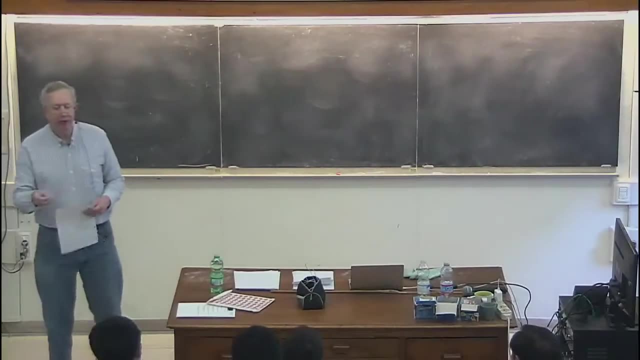 All right, so that's that table. Now I want to go on and just generalize this procedure to the case where we have some number of parameters that I want to set limits on, but the model also contains additional parameters that I don't care about. 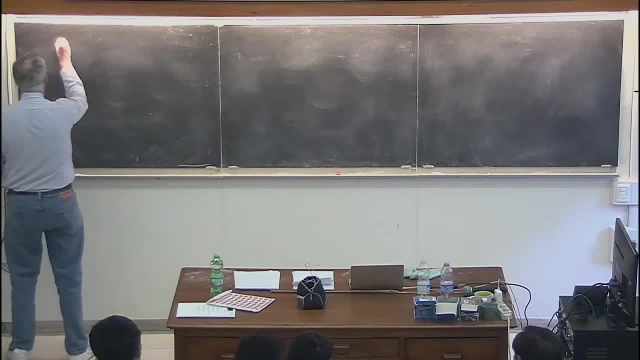 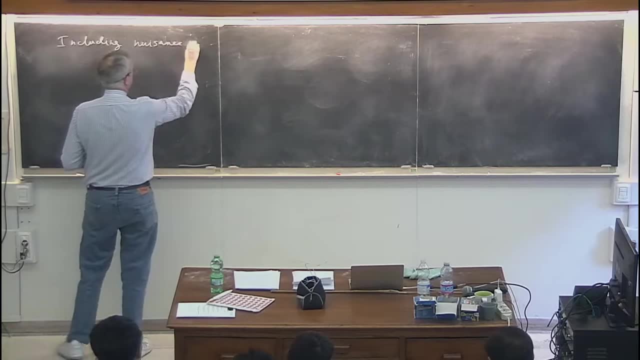 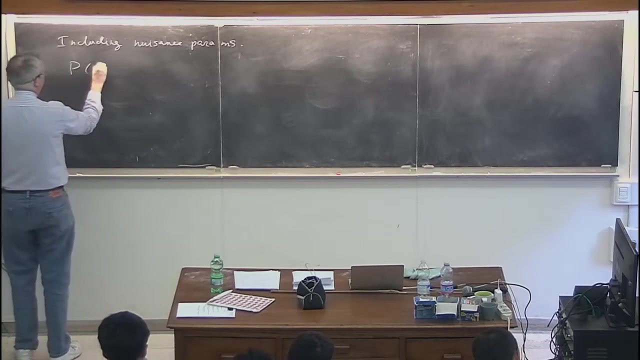 these so-called nuisance parameters, including nuisance parameters, And it's easy. It turns out to be surprisingly easy to do this, So let's suppose that I have. I start out, as always, by trying to write down the rule for the probability of the data. 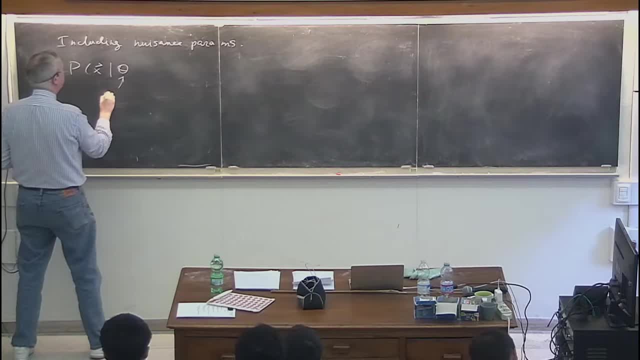 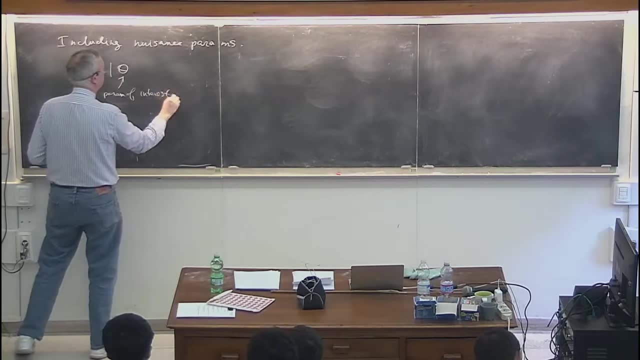 It will contain some parameters of that, some parameters of interest, theta, and also some other parameters that I don't care about but which I need to put into the model to make it correct. All right, so I've got nuisance parameters- new. 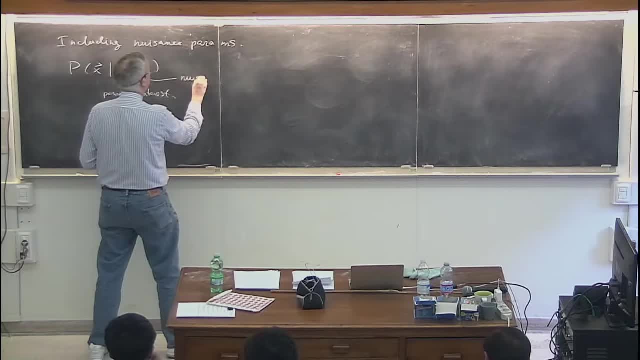 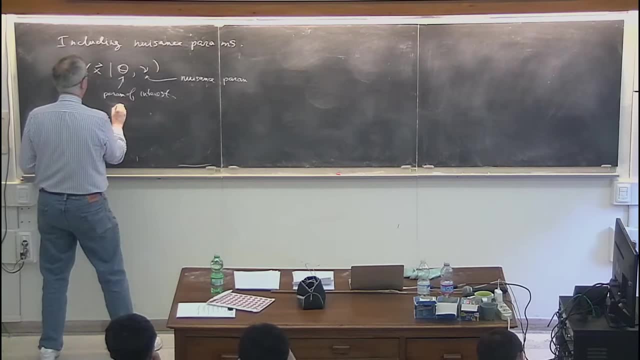 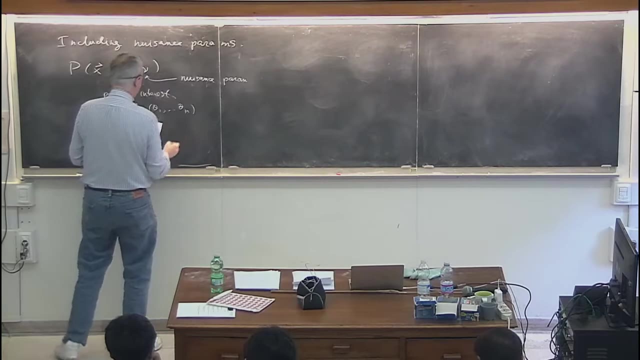 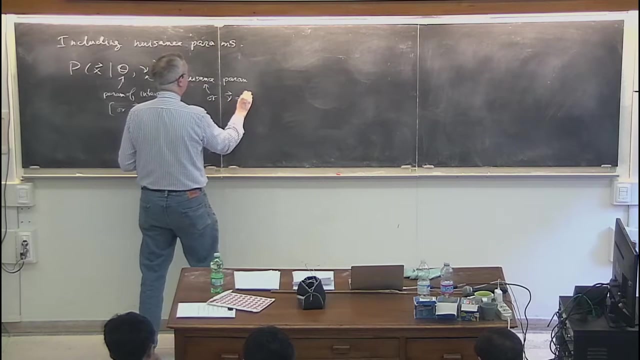 I could also talk about the case where I have more than one parameter of interest. So let me just generalize this from the very beginning. For instance, I could have a vector with n parameters of interest and I can have more than one nuisance parameter. 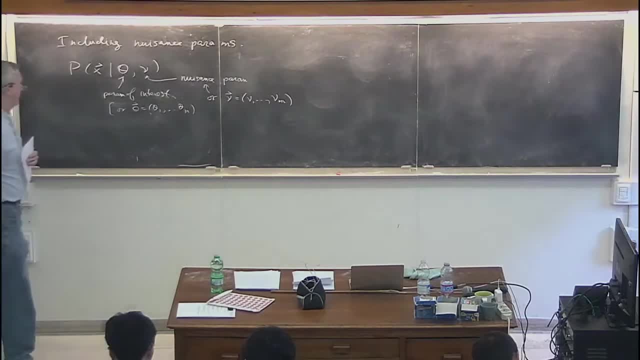 with some number of components. Let me call that m. So to begin with I'm just going to consider the one parameter case, but it's very easy to generalize this to the case where I have a vector of parameters of interest and a vector of nuisance parameters. 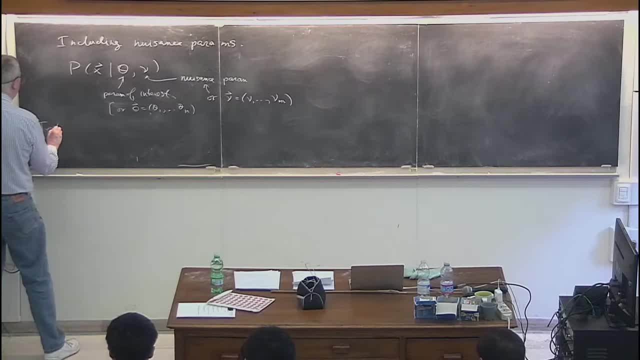 And so what I want to do is I want to test a point in the space of this parameter of interest. I want to test a value of theta. So I will test theta using the following quantity: lambda of theta. So this is going to be kind of like the lambda of mu. 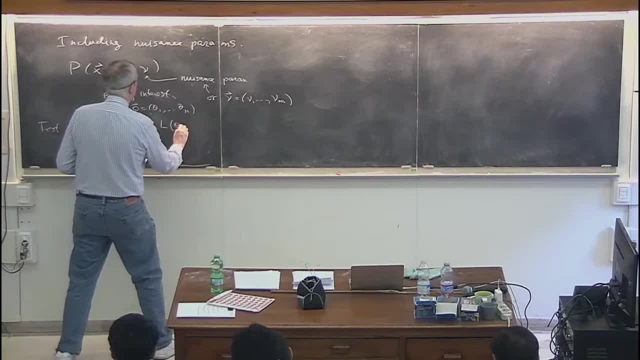 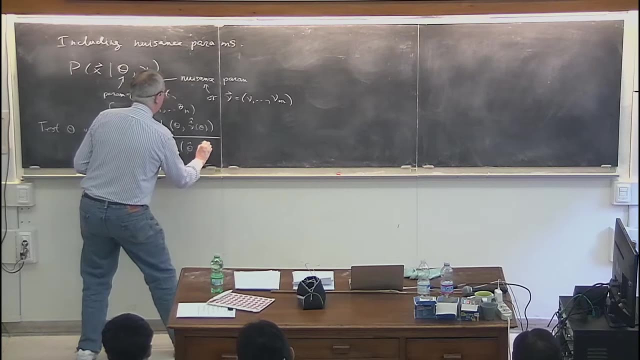 And this is going to be equal to the following: the likelihood of L of theta and nu double hat of theta. I'll have to define what that is Divided by. L of. sorry, not mu theta hat nu hat. Okay. 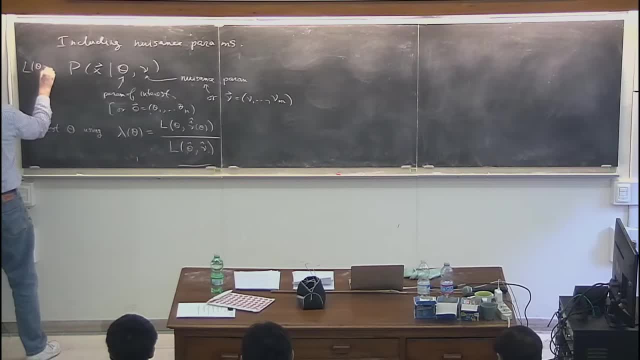 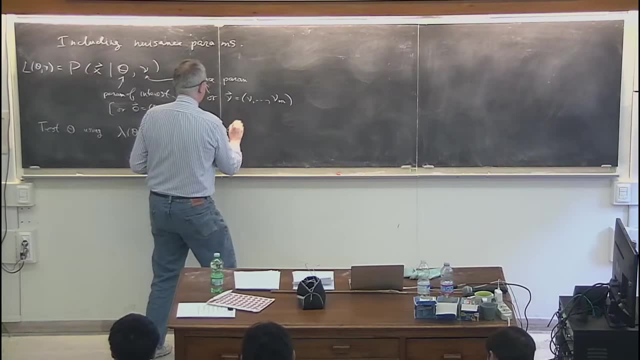 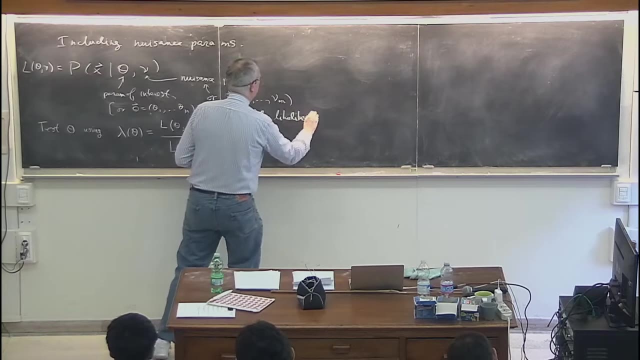 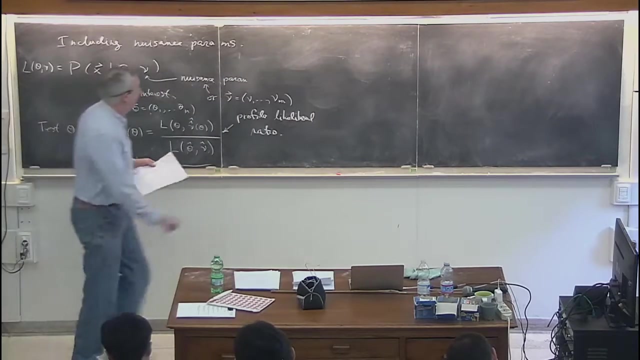 So remember this expression here: that is the likelihood, right, And so I'm going to test a value of theta with this quantity here and I will call that the profile likelihood ratio, Right? So this contains some things I haven't defined yet. 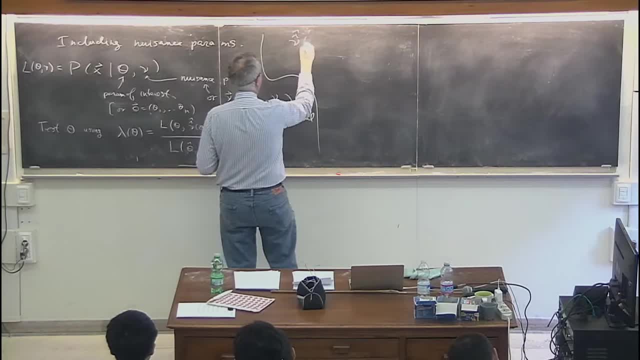 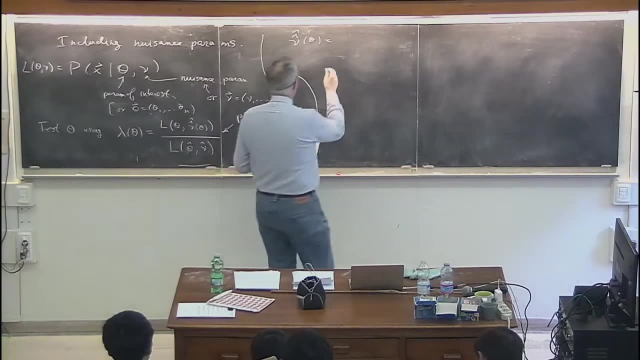 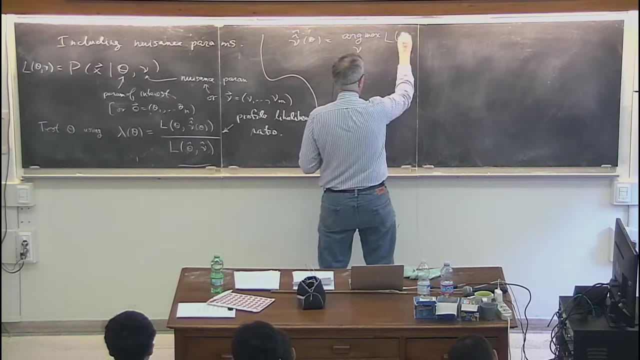 So let me say that nu double hat of theta. what is that? That is what's called the profiled value of the nuisance parameter, And that means it's the. I'll write it formally first: arg max nu of L of theta and nu. 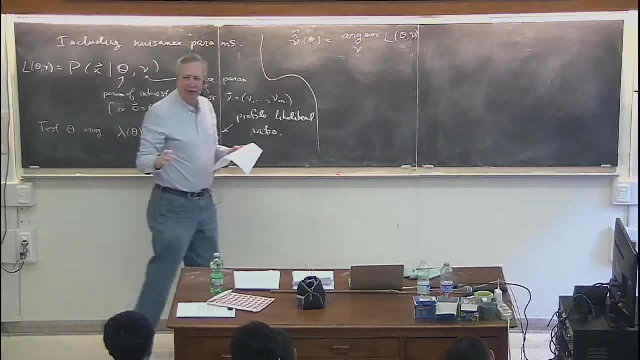 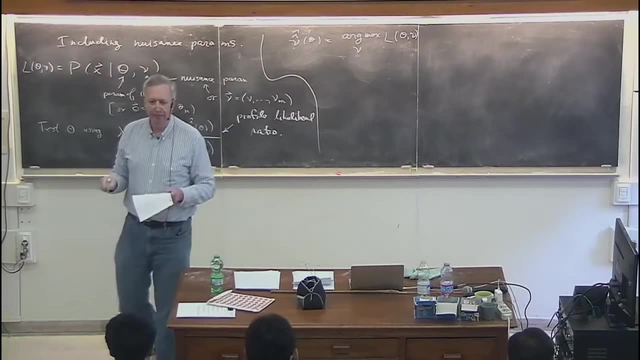 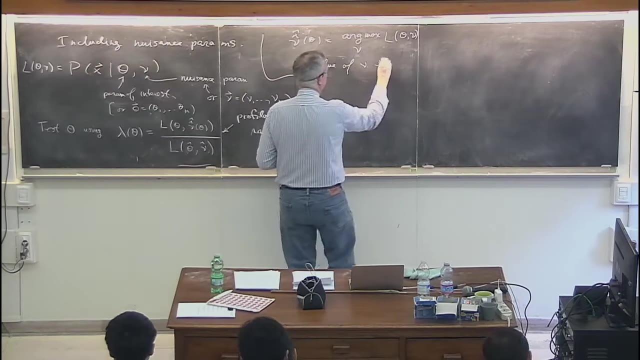 And that means that I specify the theta that I want to test, And nu double hat is then the value of nu that maximizes the likelihood for that value of theta. All right, All right, And so that's what's called the profiled value. 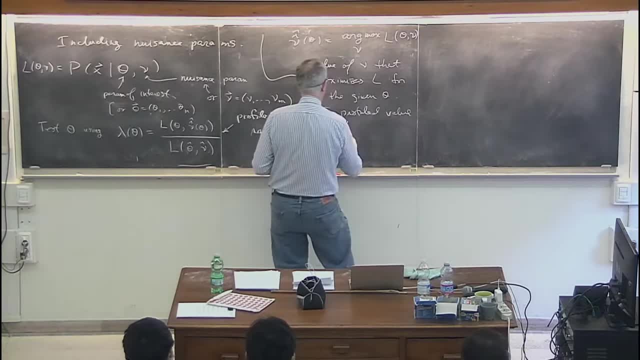 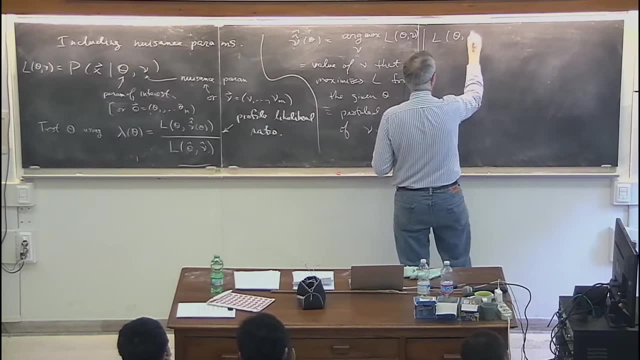 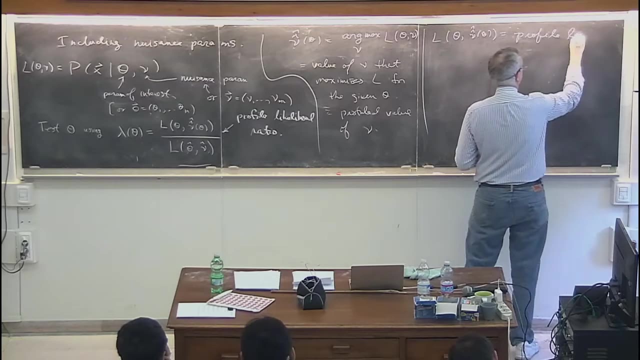 Of nu. All right, And so then, this quantity here, L of theta, nu double hat of theta. this is called the profile likelihood. I'll sometimes write that Lp and it is, you will notice, only a function of the parameter of interest. 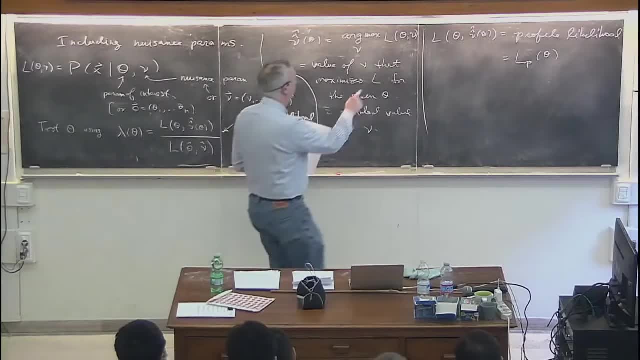 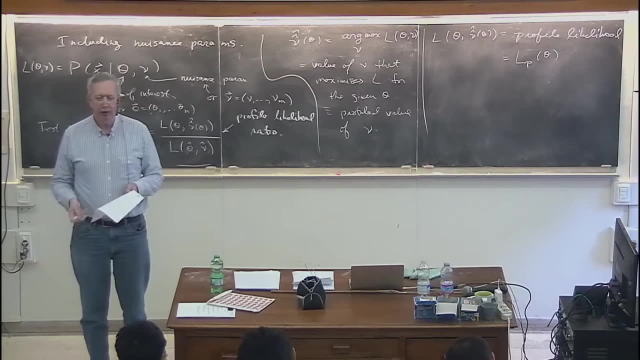 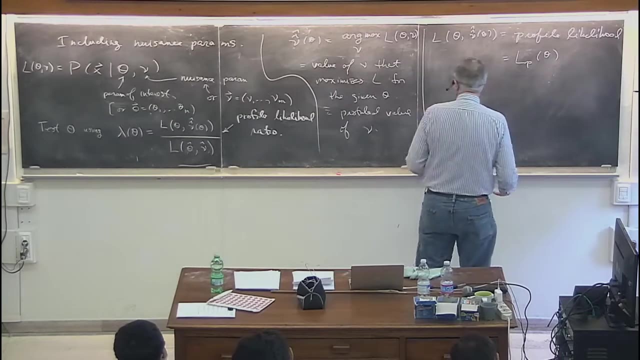 I've eliminated the nu substance, the nuisance parameter, by evaluating it with the nuisance parameter that maximizes L for the given value of theta. So that's the important point is the profile. likelihood only depends on the parameters of interest. All right, And now I just proceed kind of as before. 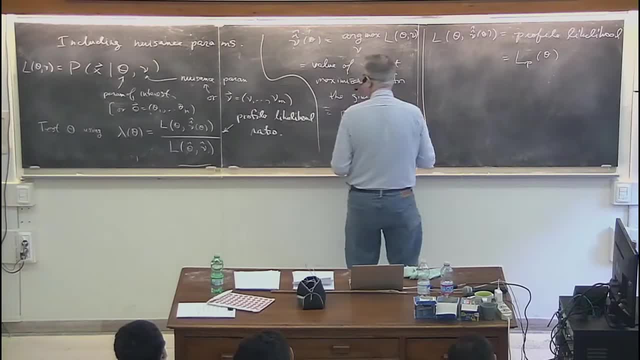 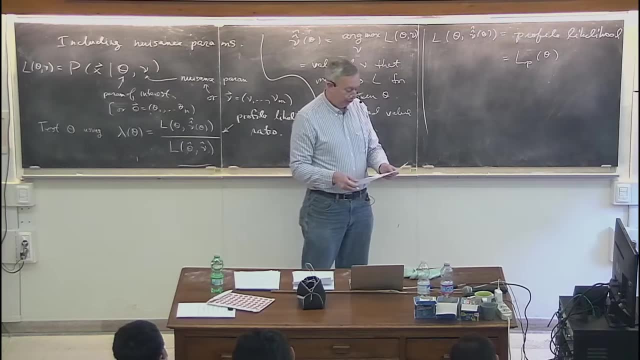 I have this profile likelihood ratio, and so what I can do is I can use it like the likelihood ratio that I had on the board just a half hour ago, which is to say that if this likelihood ratio turns out to be close to one, 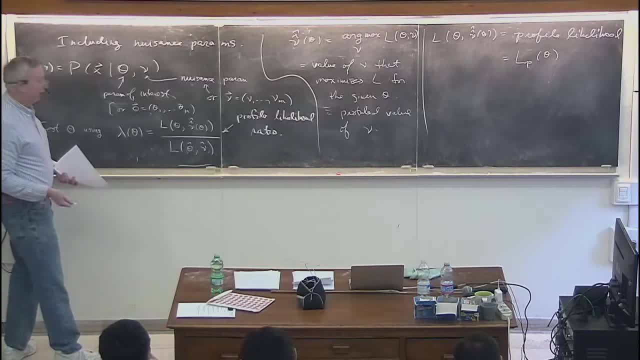 well, that means that the value of theta is in good agreement with the data. If I get a small value of theta, it is in bad agreement with the data, And so I can use this quantity as the criterion by which I establish the critical region of a test. 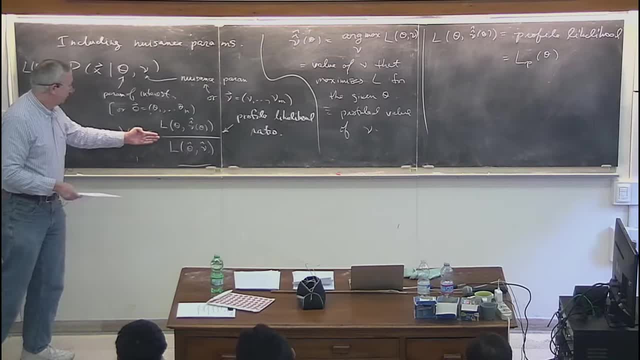 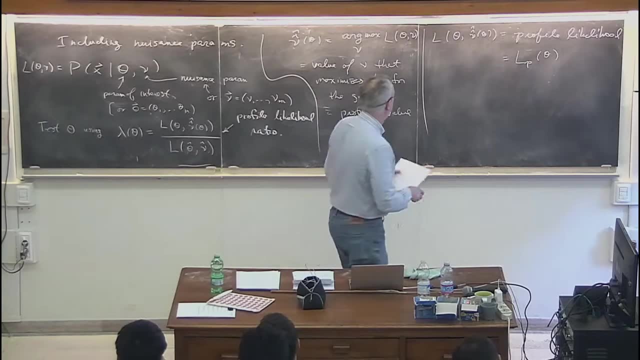 or the criterion by which I determine a p-value. All right, And so let's just see how that works. So, for example, to test theta, I'm going to define this quantity, t sub theta, which is minus two times log of lambda of theta. 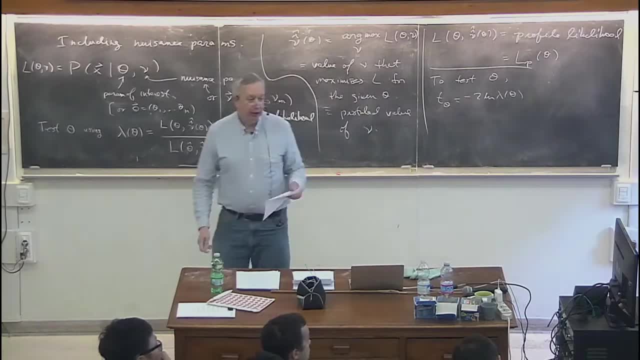 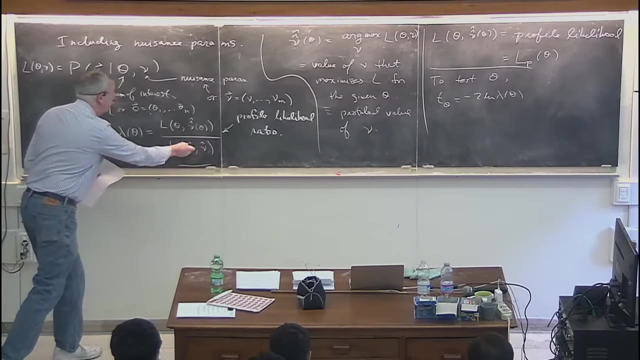 just like before. And yes, No, no, it's still bounded between zero and one Right, Because in a denominator I have the maximum of the likelihood. The single hats denote the ordinary maximum likelihood estimators. Sorry, I should have repeated. 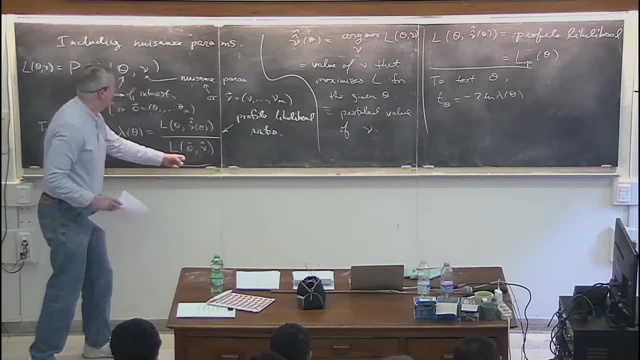 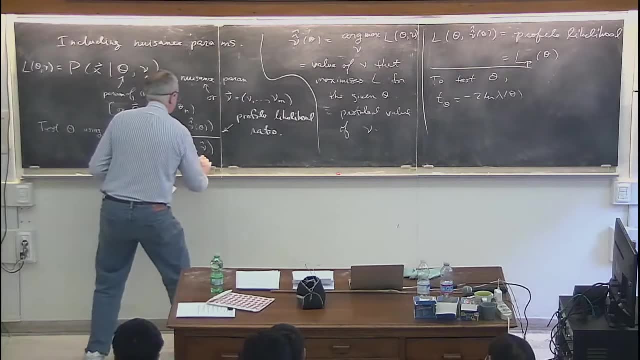 Yes, the global maximum. So when I write L of theta, hat, nu hat, I mean the values of theta and nu that maximize the likelihood. So that's no good point. This denominator is the global maximum of the likelihood And this lambda is like the other one. 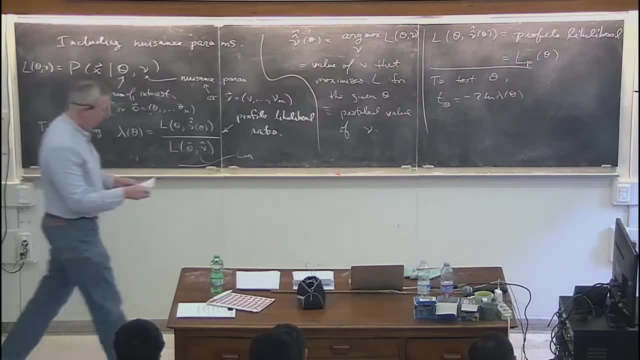 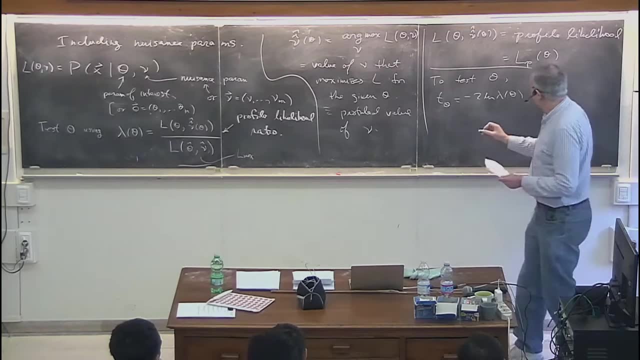 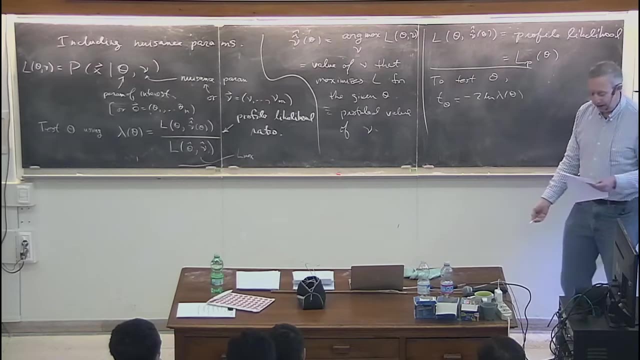 bounded between zero and one. Yes, And I'm going to say that high values constitute good agreement, low values constitute bad agreement. Or, if I define the statistic t theta in this way, high values of t? theta correspond to lesser compatibility, And so, therefore, my p-value. 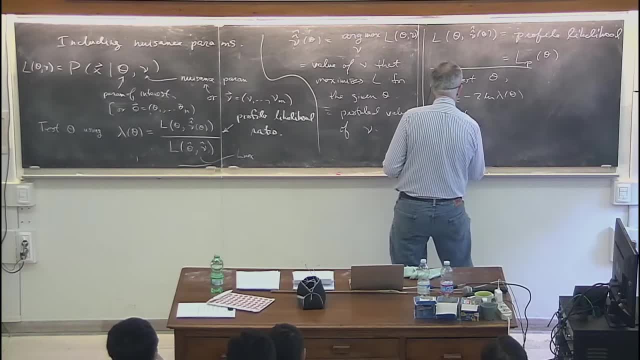 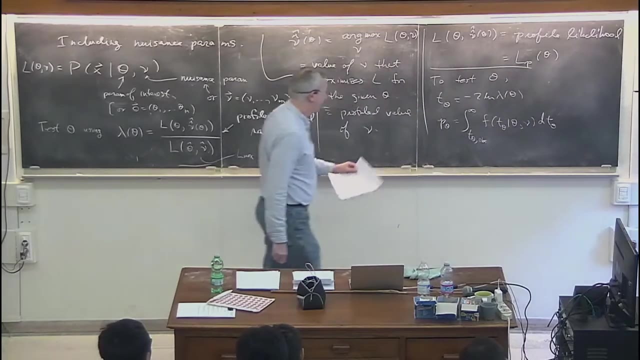 of a hypothesized value of theta is just going to be just like before. It's the probability to find t theta as high as the value I observed or higher, But now a subtle difference. Right, That's the p-value I need to compute. 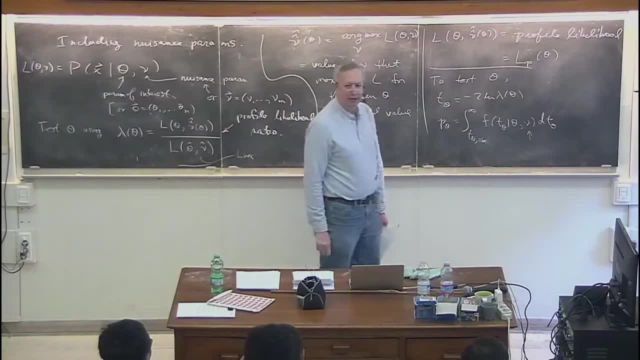 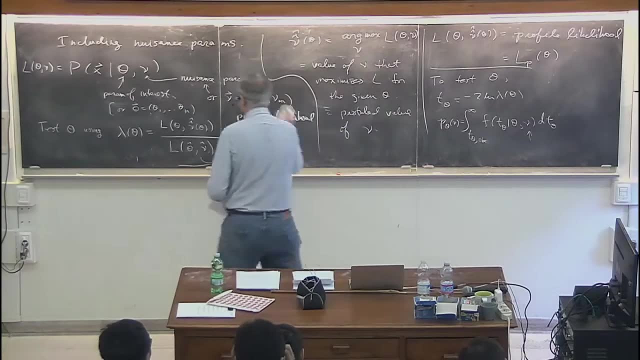 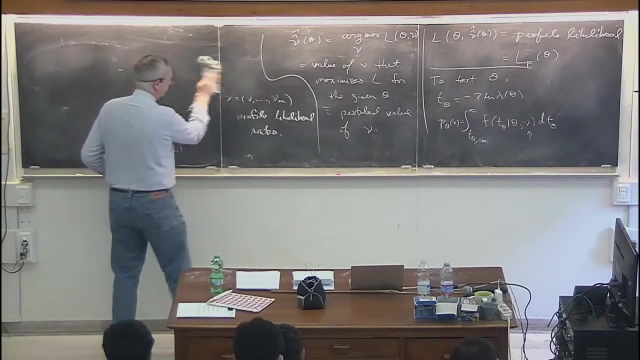 But you notice it contains the nuisance parameter, So this p-value becomes a function of the nuisance parameter. So I think that we discussed this partially in the discussion sessions yesterday. so let me just say review briefly how this works. I'm not sure I said it in both sessions. 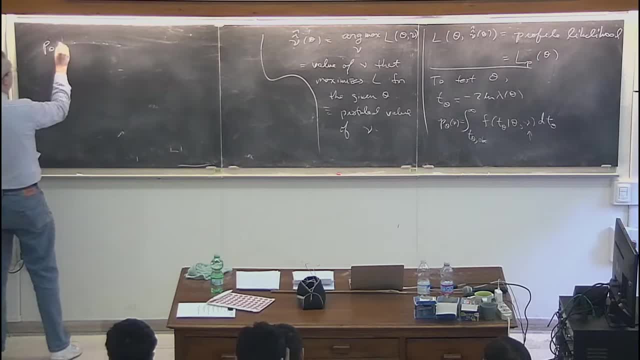 But what you're going to get then is a p-value that depends on this nuisance parameter, So I could plot it as a function of the nuisance parameter, if you want, And I could say alright. so here's alpha, the threshold below which I'll reject the value of theta. 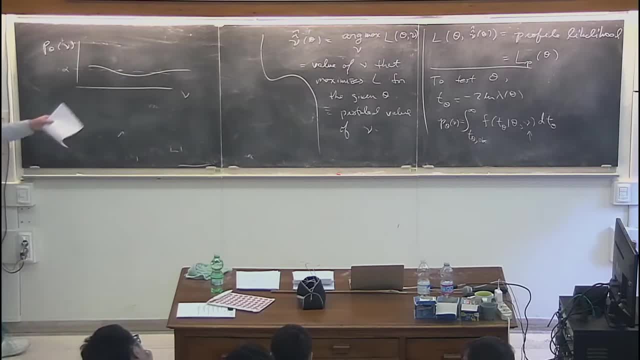 And I could compute this p-value and it might look like that: Maybe sometimes the p-value is below my threshold, sometimes it's above, And the question is: would I reject this value of theta? And the answer is, in this case, no. 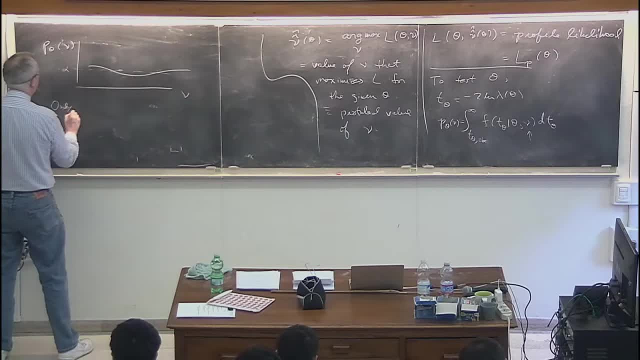 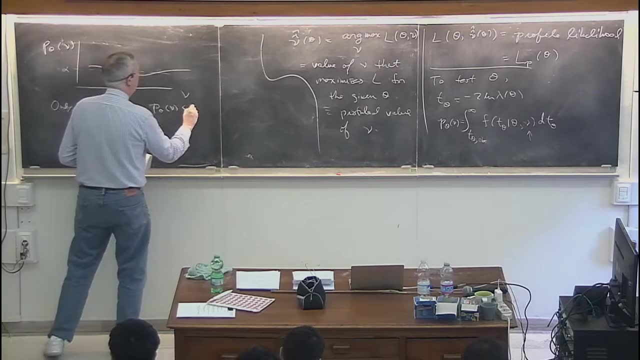 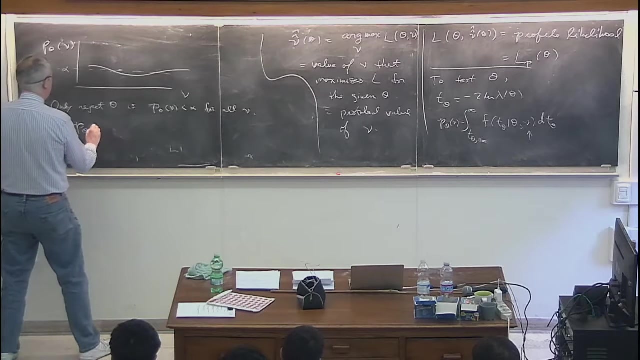 So we would basically only reject theta if the p-value is less than alpha for all values of the nuisance parameter. So that is effectively saying that I'm going to say that the p-value, or should I write this? I don't have a notation. 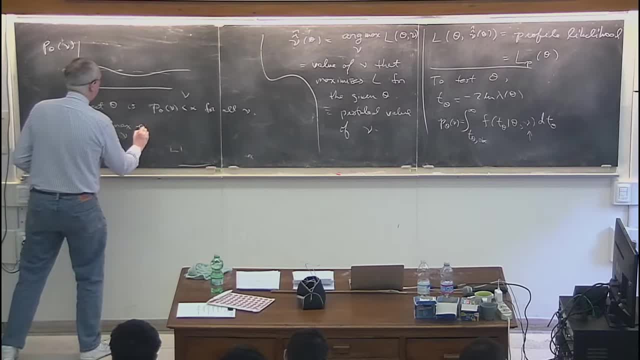 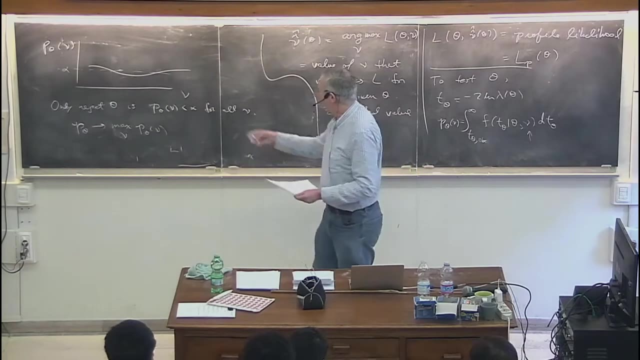 is going to be replaced by the maximum of the p-value. when I vary the nuisance parameter, I'm going to take effectively the maximum and require that it be less than alpha, And in some cases that can be problematic. We discussed this in the discussion session. 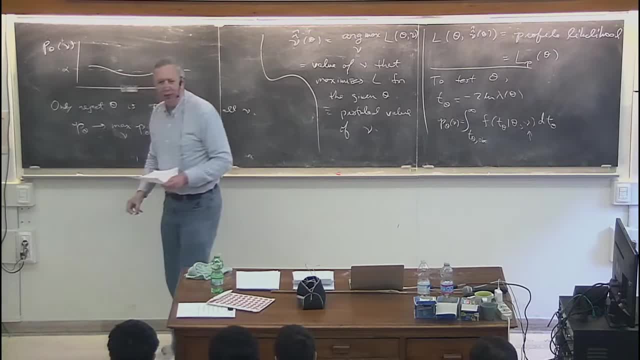 that maybe I really believe that the nuisance parameter should only be over here and that somehow the fact that it's given me a p-value greater than alpha over here prevents me from excluding that value of theta. And the way to deal with that is to build into the analysis. 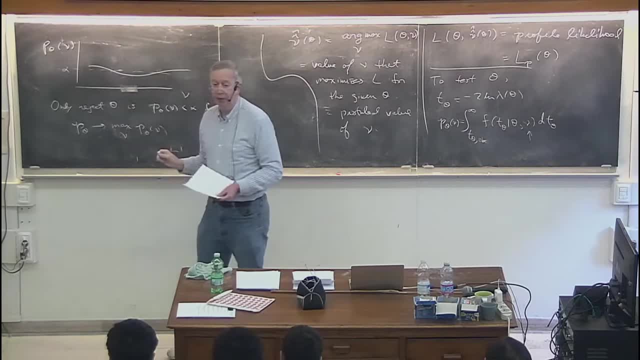 the information which you believe constrains the nuisance parameter. But that's another story and we're not going to go into that now. What I want to point out now is another miracle of Wilk's theorem that actually obviates that entire discussion. 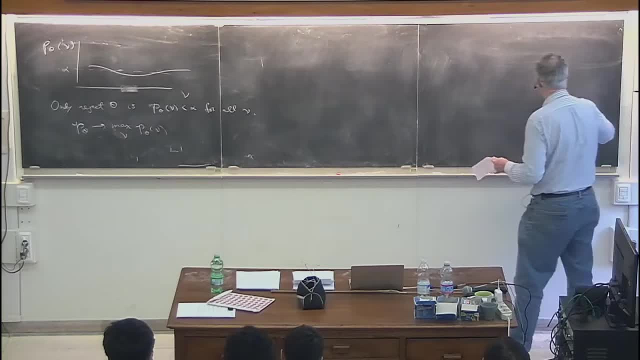 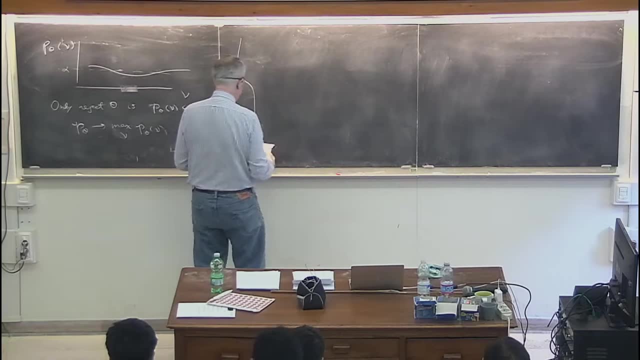 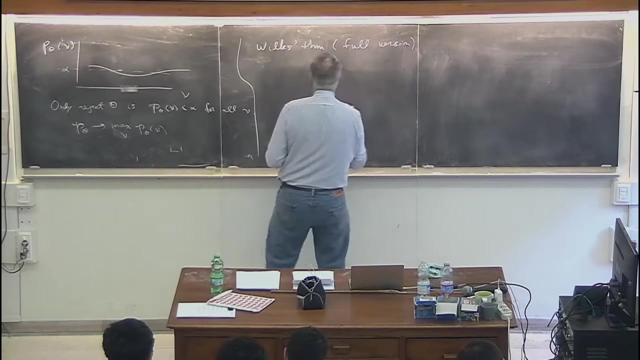 The first version of Wilk's theorem that I gave you was for the case when there is no nuisance parameters. But what Wilk's theorem also says is the following: So what I call this full version, not the simple version, says that t sub theta. 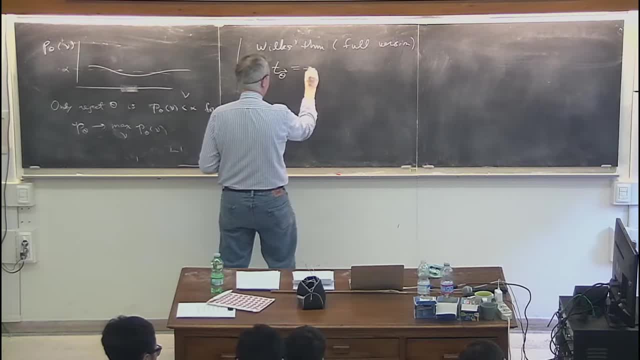 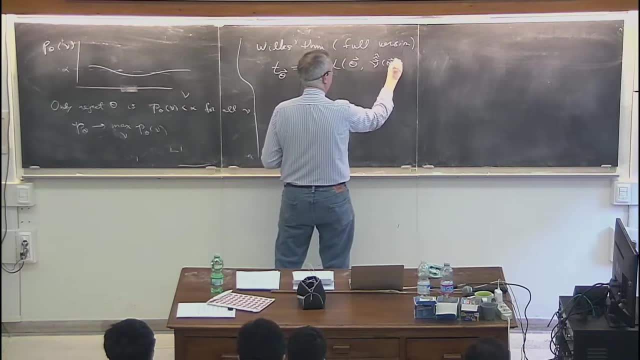 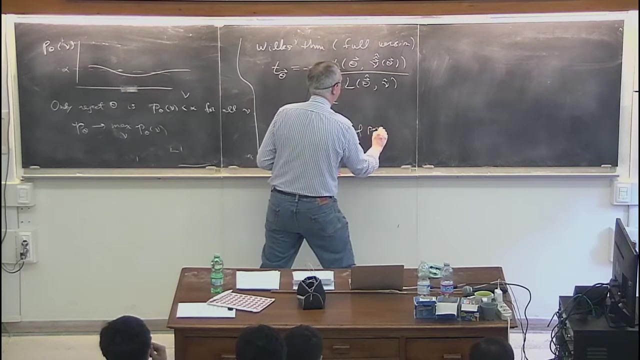 I'll call this a vector theta, which is minus two times log of say vector theta, vector nu. all right, is the radian. Let's suppose that this thing follows a chi-squared distribution for n degrees of freedom, where n is the number of parameters of interest. 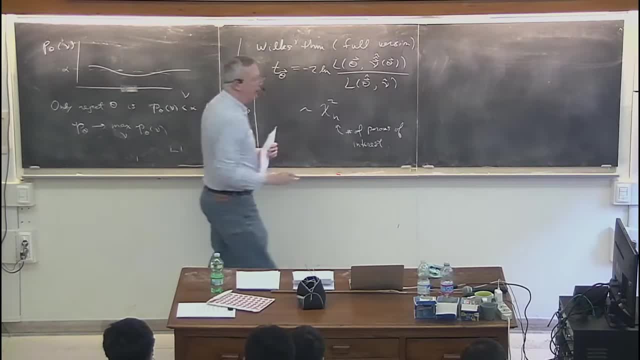 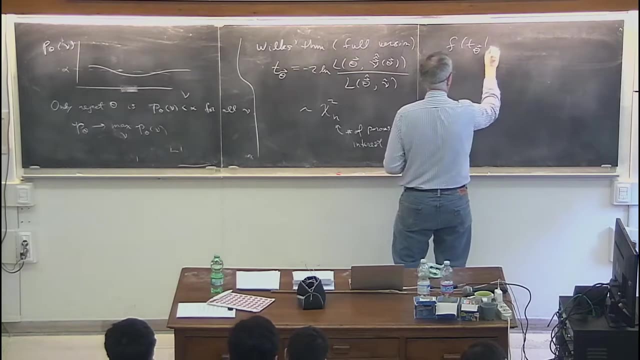 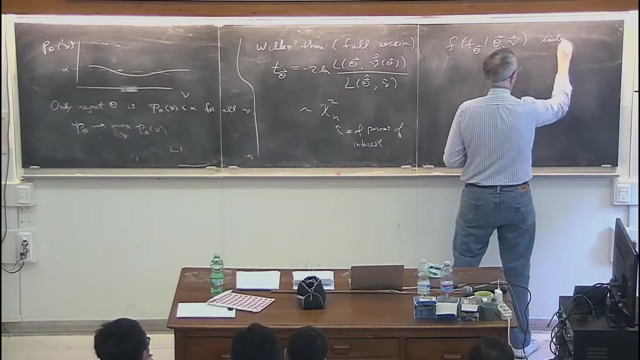 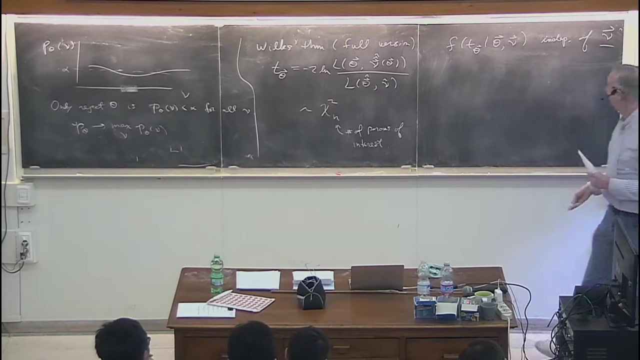 It's the number of parameters in the likelihood that don't get hats. And this is true, for that is to say that this distribution, given theta and nu, is now independent of the nuisance parameters. That's crucial. So that means that if I exclude, if I can assume that this distribution is correct, 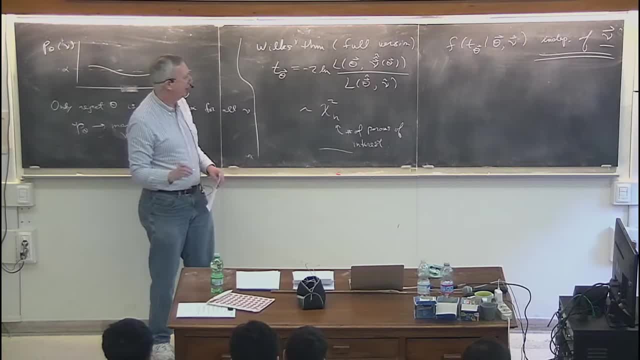 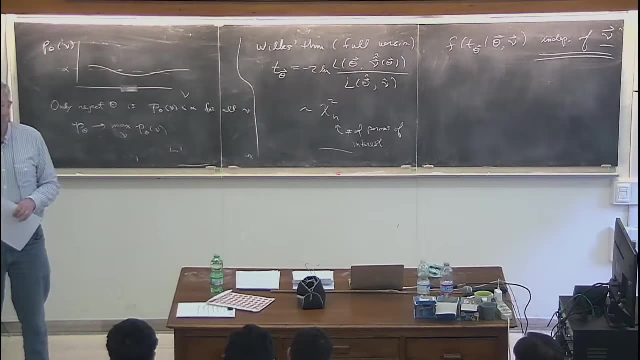 which it will be in the large sample limit right for a sufficiently large data sample. and if I get a p-value for theta which is less than alpha, then it's going to have to be less than alpha for all values of the nuisance parameters. 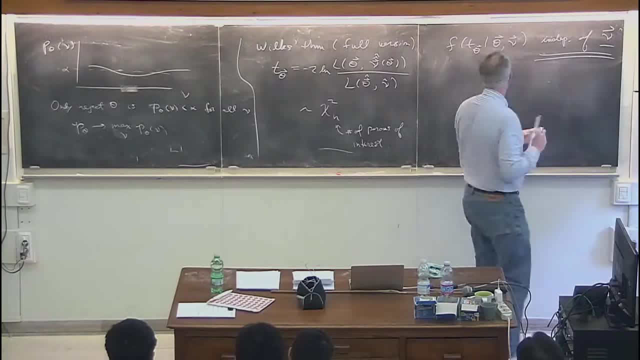 Because this distribution becomes independent of the nuisance parameters. It's just a chi-squared distribution. It's just that formula that I had written down: No nuisance parameters in that. So that's the really handy miracle of Wilk's theorem that we exploit. 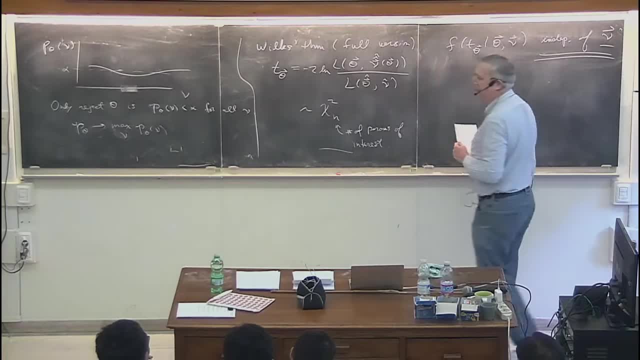 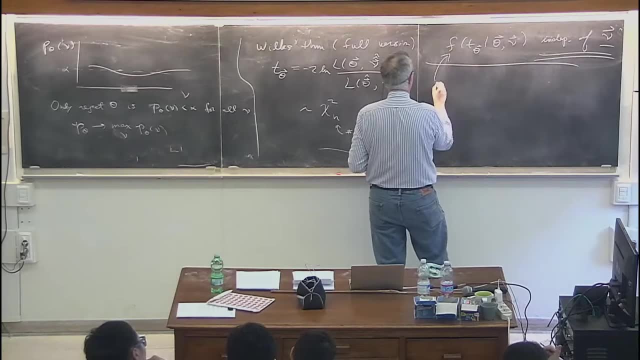 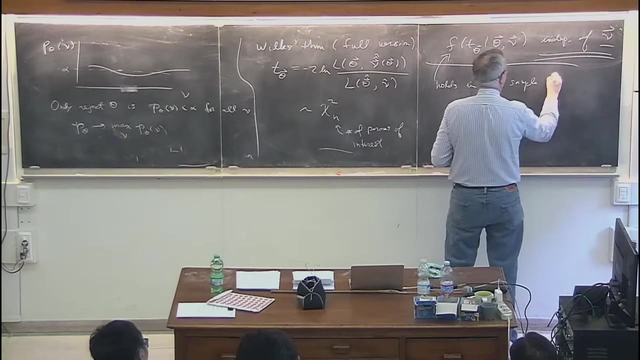 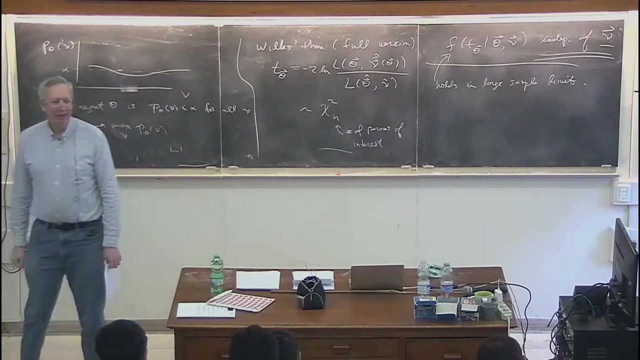 Now that holds in the large sample limit. So this is holds in large sample. This is the large sample limit If you have a finite data sample. I mean if, of course, you have a finite data sample, but if you're worried that the size of your data sample is small enough that that approximation 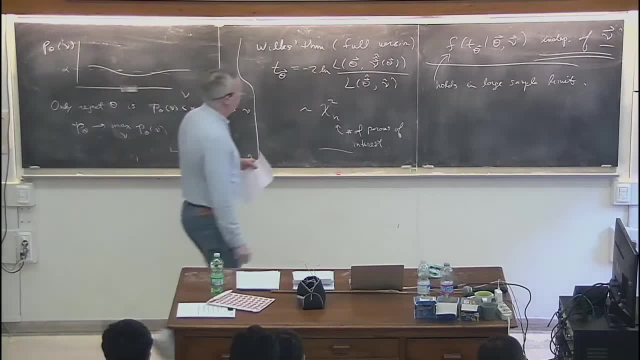 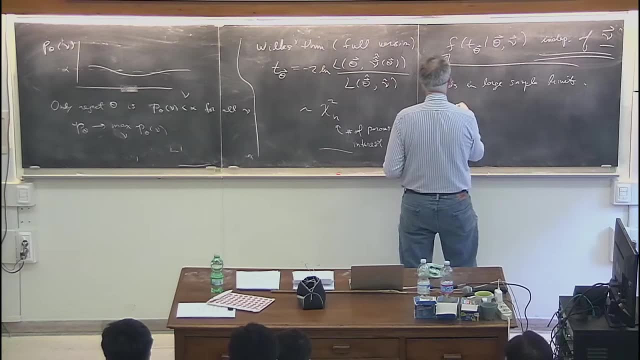 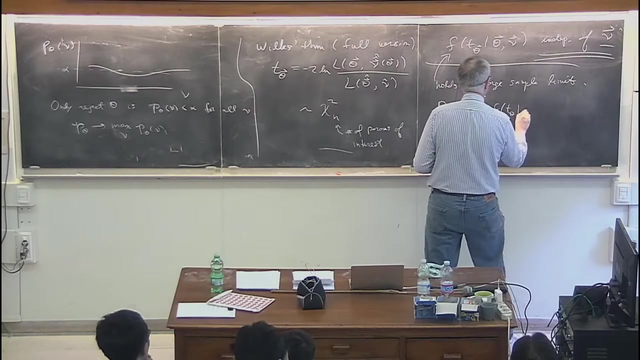 might not be valid. you can construct an approximate p-value in the following way: You can construct it as the integral from t observed to infinity, sorry, t theta observed to infinity f of t theta, given theta. And so if you need to put in the nu dependence and so you're not allowed to use Wilk's theorem, 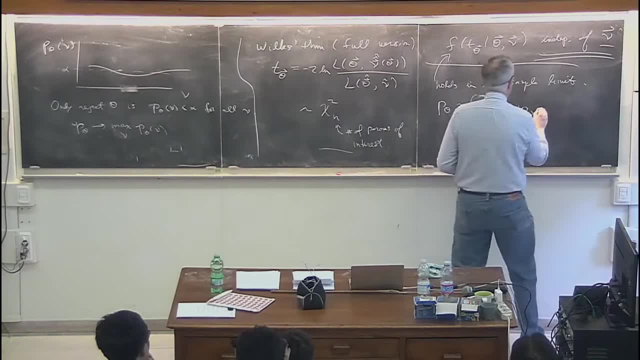 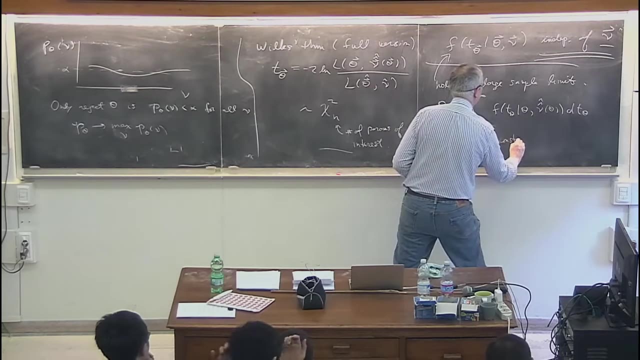 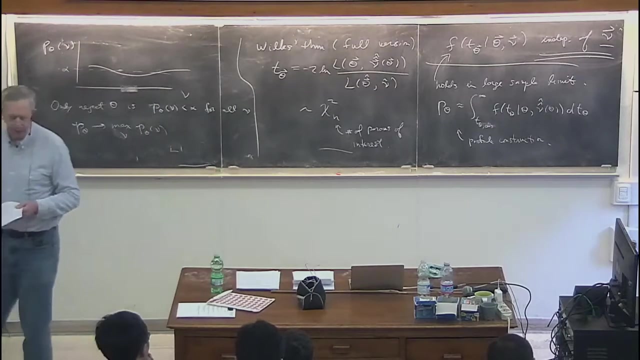 instead of scanning the entire space of nu, what you can do is you can evaluate it just with the profiled value of nu, And this use of this p-value is what's called profile construction, at least in particle physics And in cases when the data sample is not large enough for us to exploit Wilk's theorem. 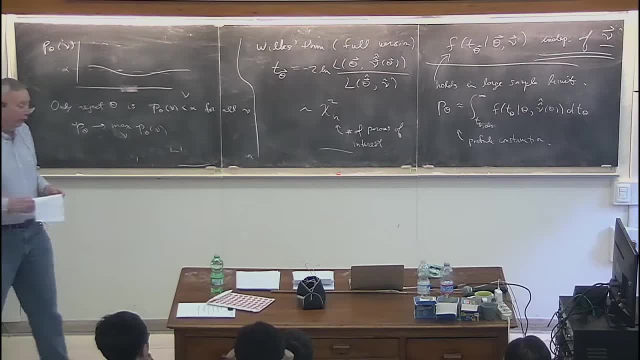 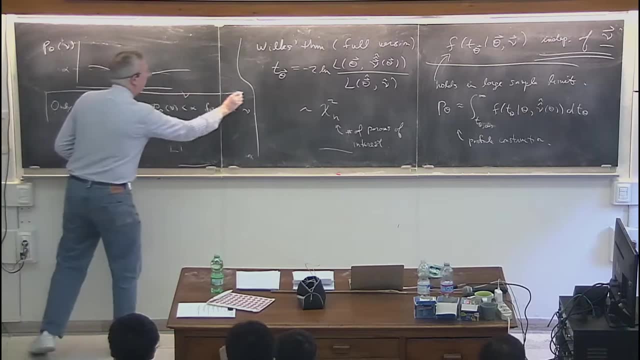 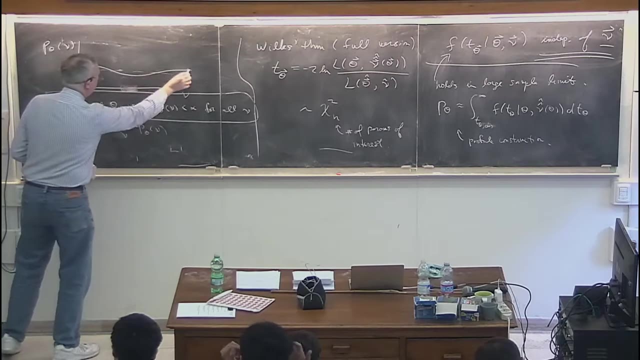 this is very often the approximation that we use, So we will not go back on this fundamental statement here. It's not that we will only reject theta if its p-value is less than alpha for all nu, because to actually compute this, this curve, could be a very laborious process. 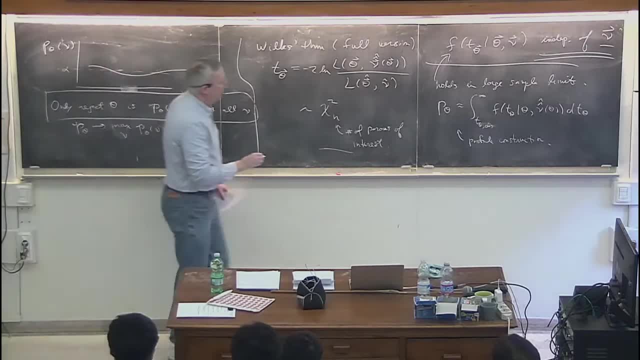 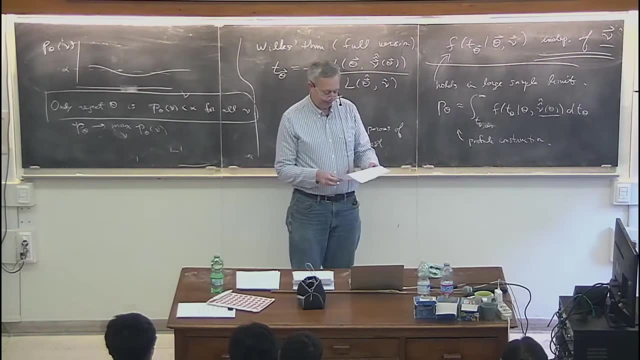 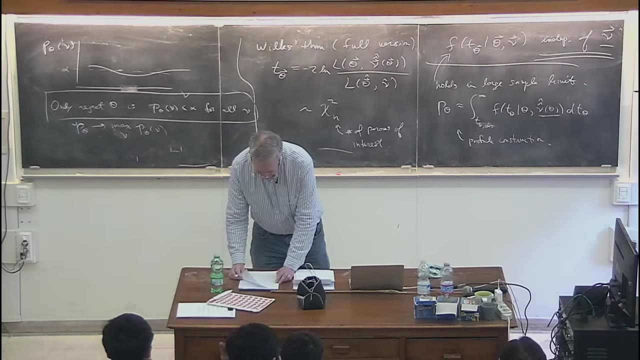 What we would do instead is we would only go to the value of nu that corresponds to the profiled value, and we would compute the p-value using that. That's an approximation, Okay. So from there, basically, it says that we can proceed as before. 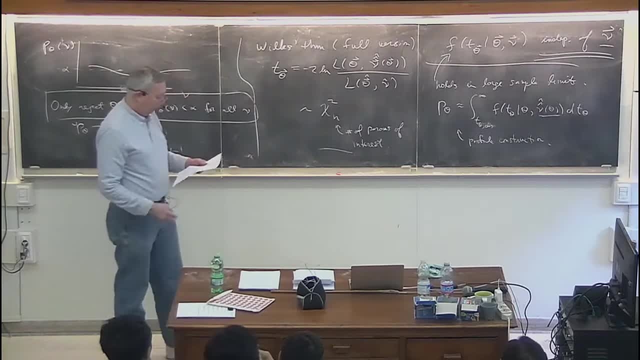 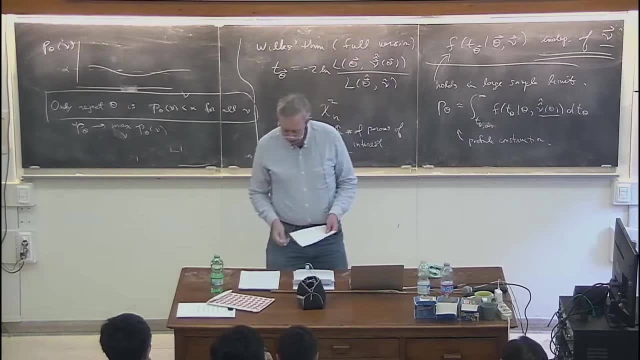 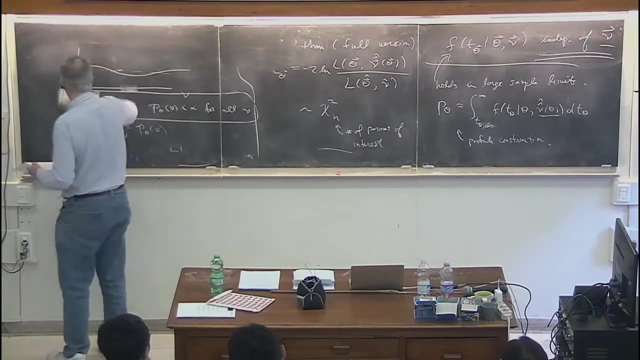 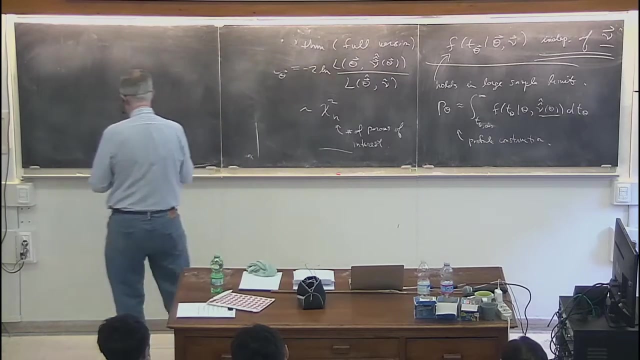 because this is exactly the same distribution that we had before, And so the uh uh, same formulas that we talked about earlier are still valid. That is to say that you will get- I'll just write it on the board- The region of theta space that you want to look at then. 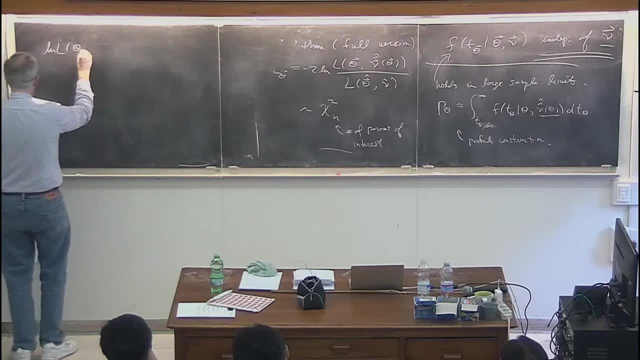 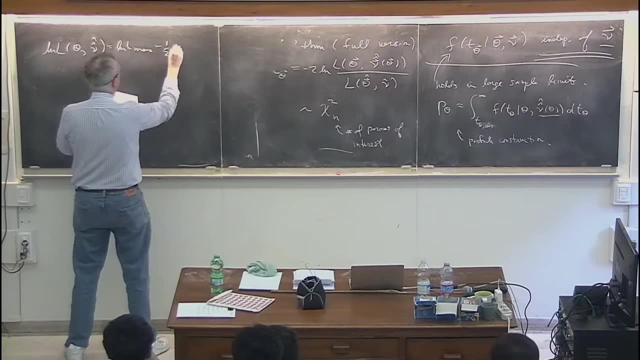 is the region that corresponds to log L of theta, and nu double hat equals log L max minus one half times the chi-squared quantile for n degrees of freedom, where n now refers to the dimensionality of the vector of theta of one minus alpha. 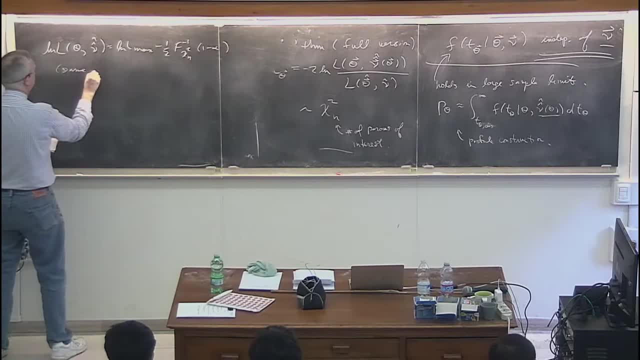 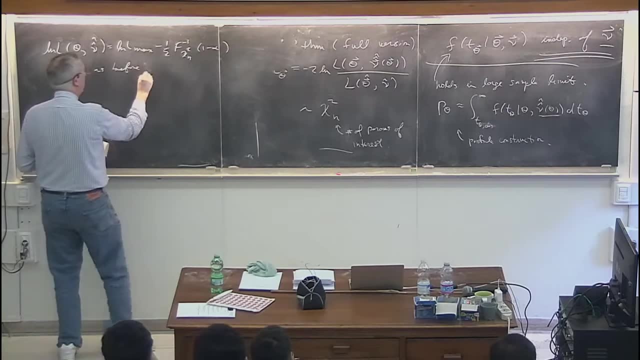 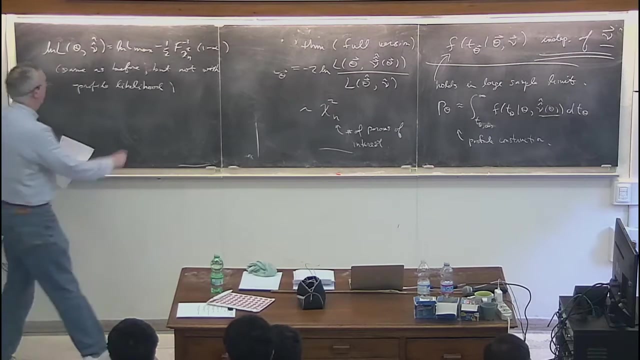 So it's the same as before, But now, instead of having the likelihood, so same as before, but now with the profile likelihood, Voila. So L max is going to be log L of theta hat nu hat. It's the global maximum. 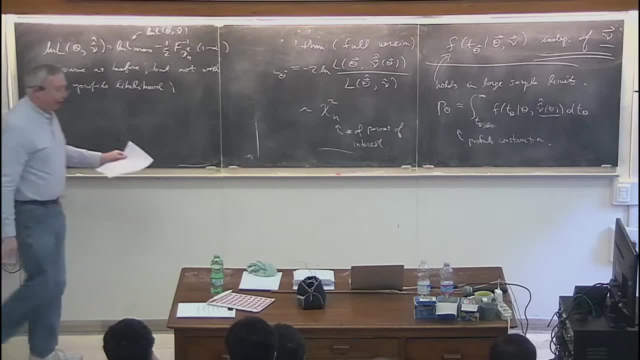 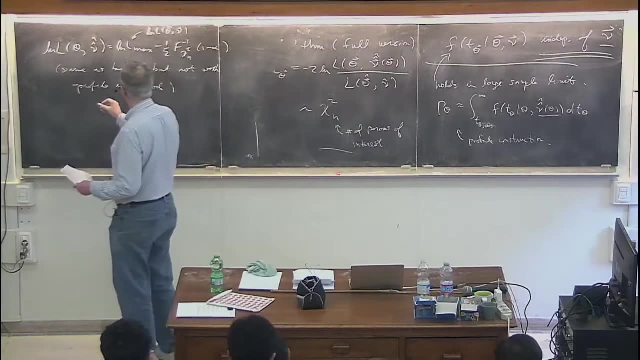 So that's an amazingly simple recipe. It simply says that if you have nuisance parameters, you do it the same way as you did before, and you simply use the profile likelihood instead, And we can see how that works graphically. So I'll try to finish this up. 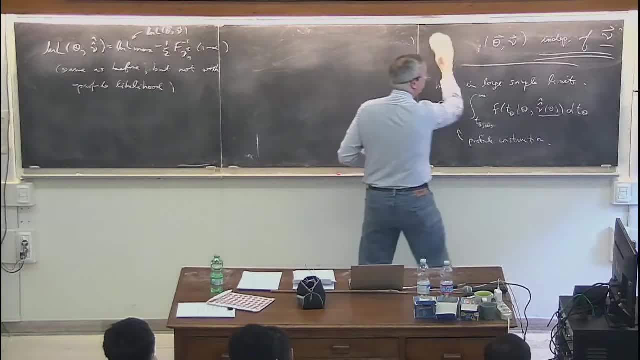 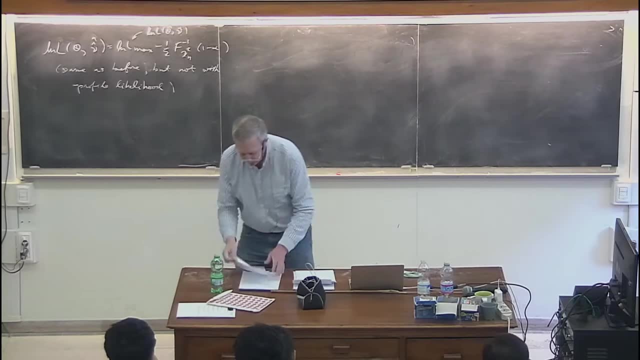 There's one more thing I want to talk about before we finish. get through this. So, for example, suppose you had a single nuisance parameter, nu, and a single parameter of interest, theta. So there would be some point here where you have the maximum right. 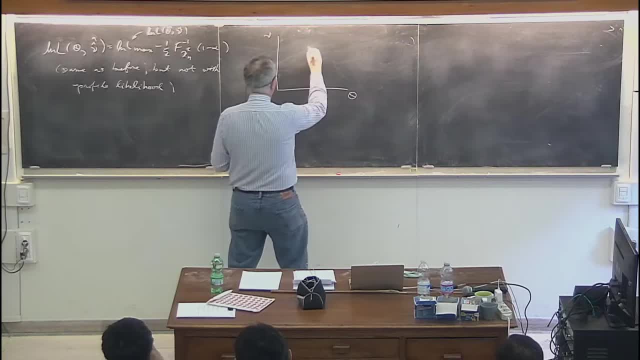 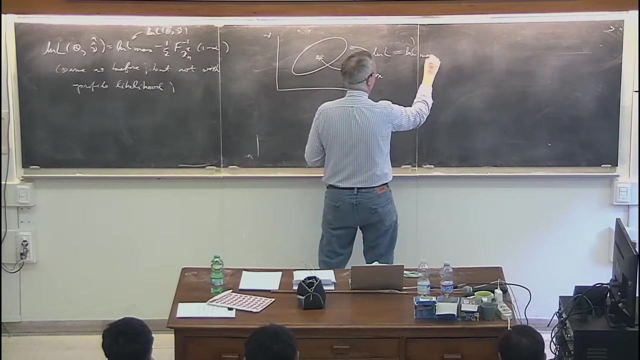 And so there will be some curve, say here, that corresponds to: that's log L max, And this curve corresponds to: log L equals log L max minus one half. So that's not the profile likelihood, that's the full likelihood, right. 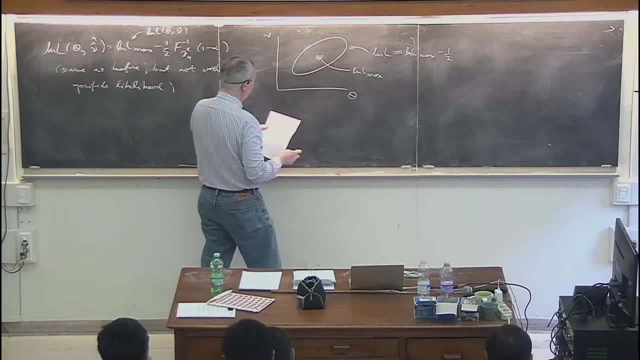 And so the rule says now the following: It says that I should find the values of this log likelihood such that, let's say, the log likelihood decreases by this amount, And that gives me an interval, say A, and, And so there would be theta hat. 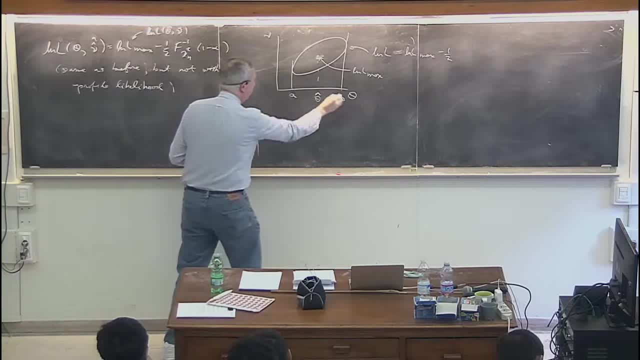 And so why is it this A and this B? Well, that's because, if you imagine this contour of likelihood as being some sort of bulge that comes out of the board, the maximum is going to be this point here, So that bulges the furthest out of the board. 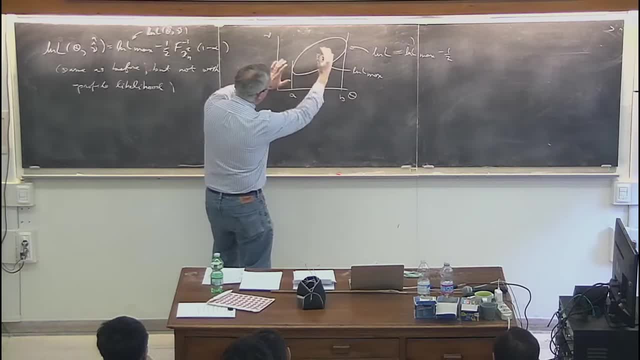 And then I have some sort of a shape, a smooth shape, a mountain that recedes back into the board. And so if I consider this value of theta here and I say what is the value of nu? that maximizes the likelihood. 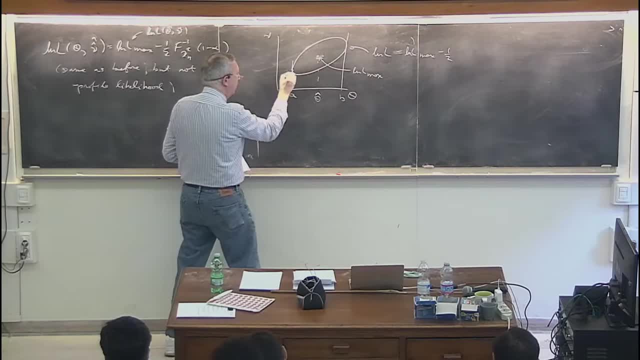 Well, as I go in this direction, it's when I get to that point right there, that's going to give me the maximum of the likelihood for this value of theta. So that value there is going to correspond to nu double hat of A. 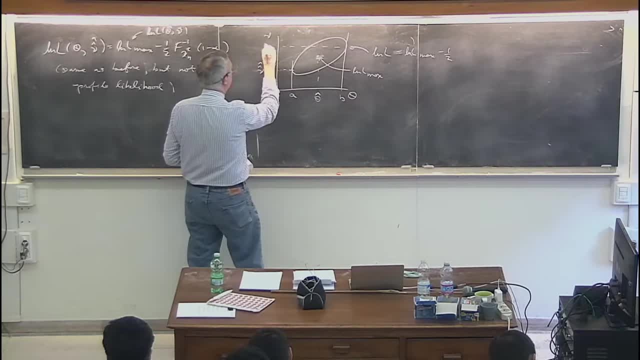 And similarly this value here is going to correspond to nu double hat of B. And as I go along in theta, if I did the same game I would find some trajectory. It's going to have to go through like that, Nope. 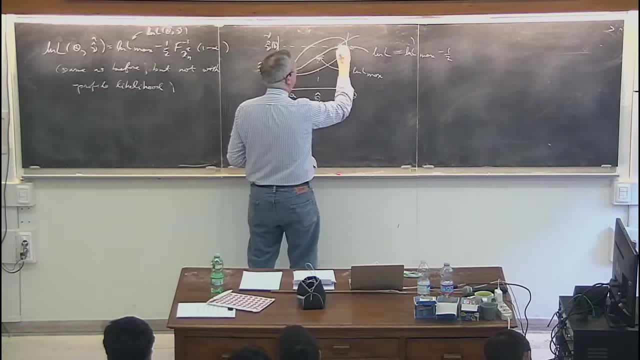 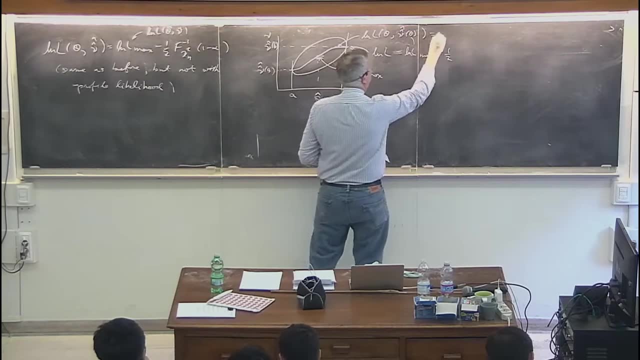 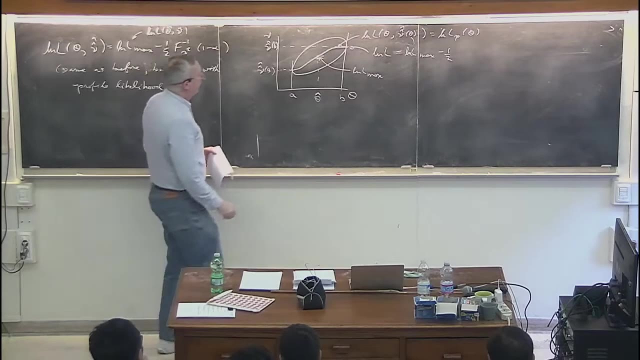 Sorry And so that path there is going to give me log L of theta, nu double hat of theta. So that's the profile likelihood, the log of the profile likelihood. So you can see that if I use this procedure, this is going to be then the same procedure that I would get. 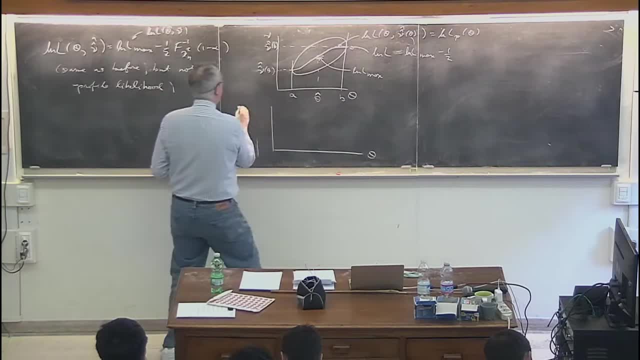 if I just look as a function of theta And over here I look at the log of the profile likelihood, So theta nu double hat of theta right, So that's going to give me, then this is just a function of theta. 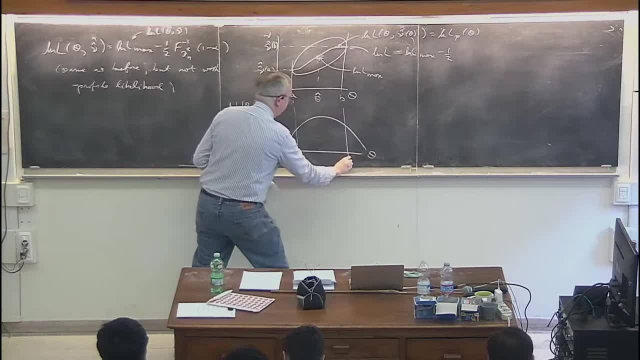 but that's going to give me the value A and the value B right, So that decrease will correspond to the same situation that I would wind here, because it's just looking at the profile. likelihood as a function of theta is the same as going along this trajectory here. 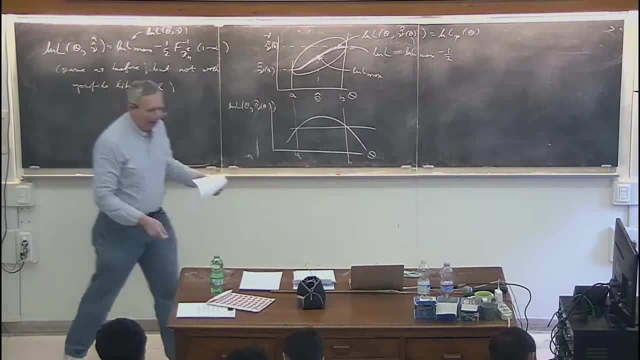 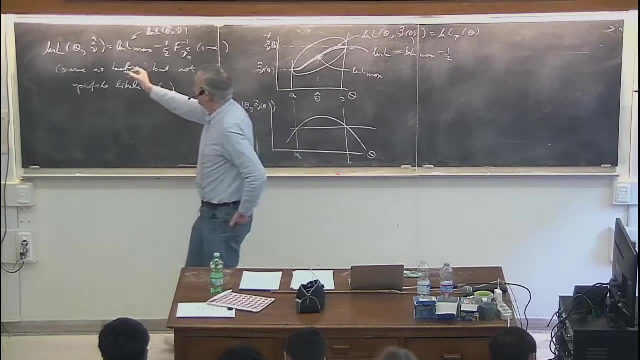 Okay, Wow, Sorry, that was a bit of a rushed explanation, but I think that The end message is simple, And the end message is that you do the same thing as you did before, but you use the profile likelihood. Okay, 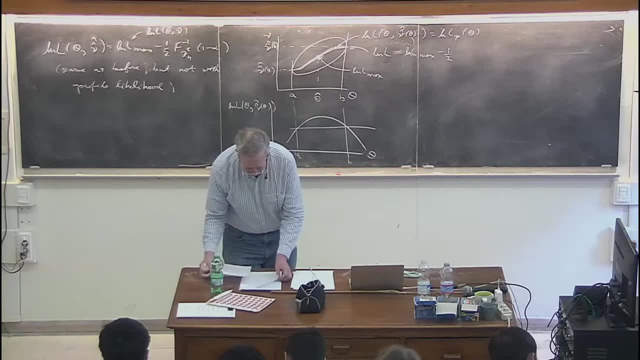 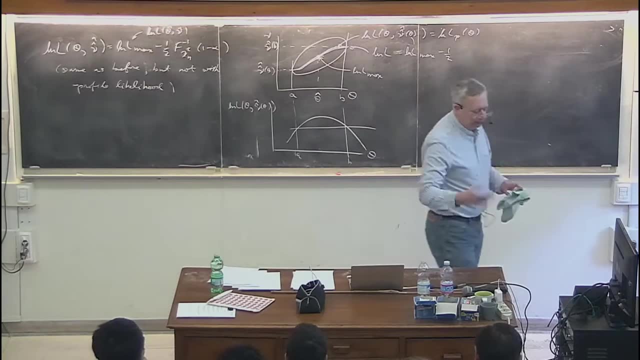 Now I only have some 10 minutes or so left, And so I want to go on and show you something which I think is really interesting and useful, And it's the kind of thing that you will hear lots of people talk about, certainly in experiment. 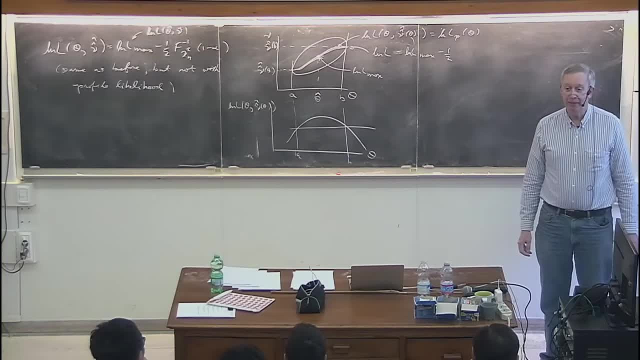 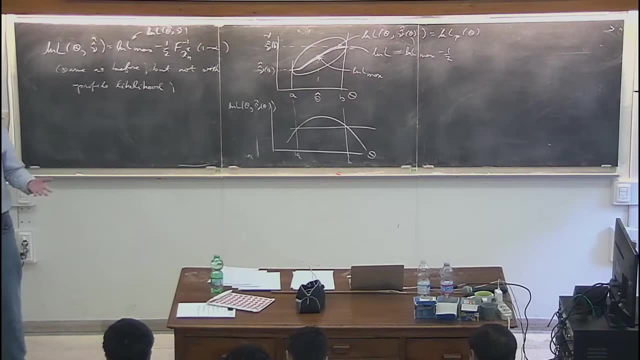 And that is a way to quantify the experimental sensitivity. This has to do with the thing that we were talking about earlier, where you would give the mean upper limit in a parameter under the assumption of no signal. So it's the kind of number that you would report. 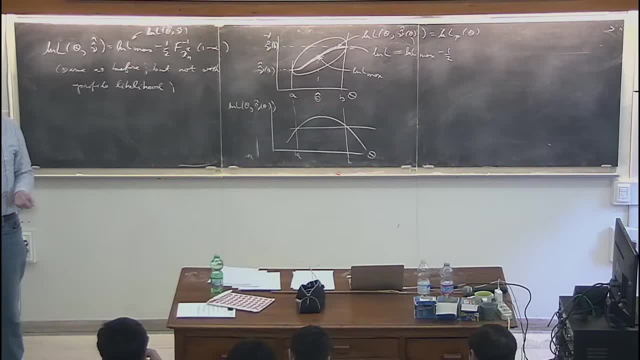 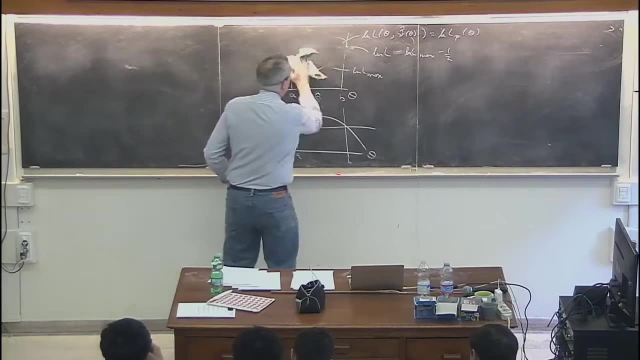 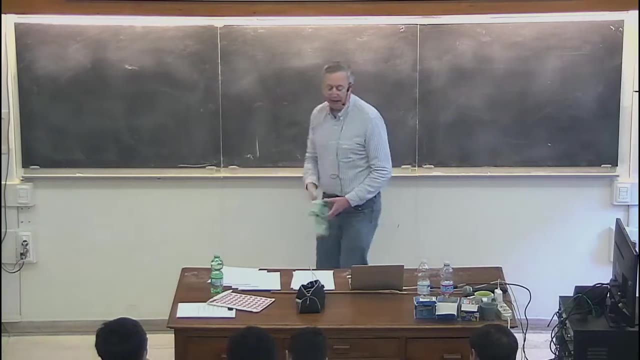 before you get the funding for an experiment, to say how sensitive it is. So I want to just run through that quickly. When you want to say how good an experiment is going to be, what its sensitivity is, there's a couple of ways of doing that. 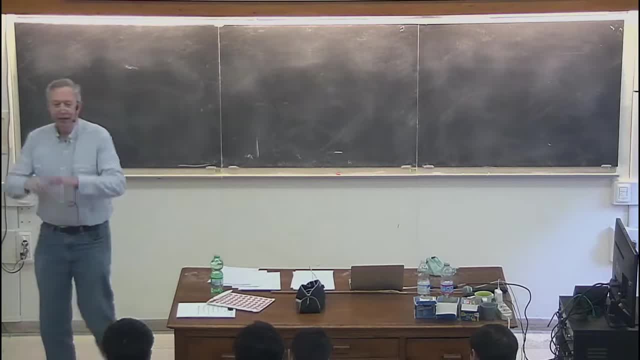 One way would be to say: well, if the signal is absent, this is, this is how the limit that I expect to set on some parameter. But that's a bit defeatist, right? We don't do experiments just to set limits. 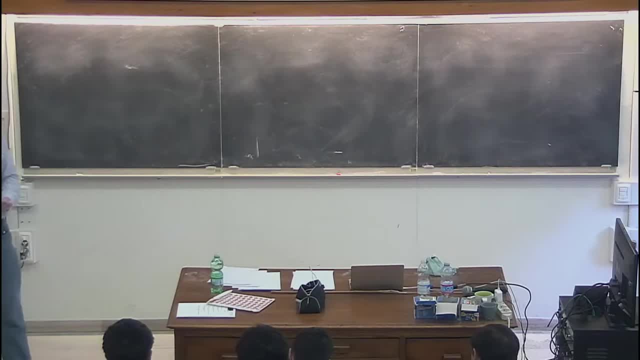 We do experiments to discover new phenomena. So really, what we would like to know is the following: We would say: if the signal is actually there, what are my prospects for discovering it? And to discover the new signal process, what you need to do is to reject the background-only hypothesis. 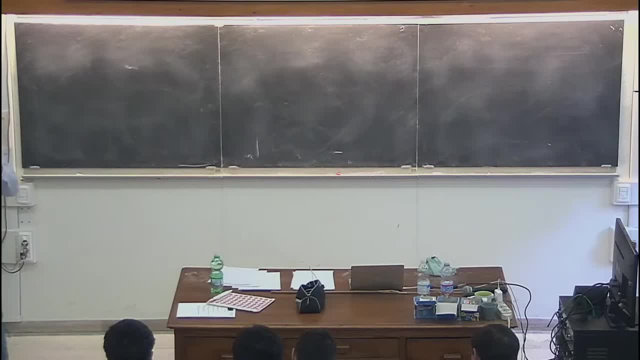 And so what's the corresponding measure of sensitivity? It would be to say what's the mean or median significance with which I would reject the background-only hypothesis. if the signal is actually present at some nominal rate- And that's the number you would tell your funding agency to say. 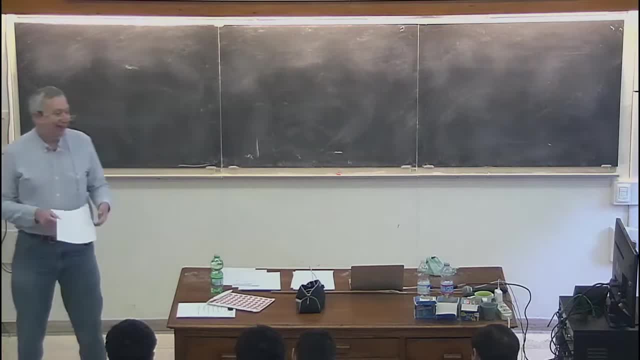 look, if you give me so-and-so million dollars, then I will build an experiment that will give you expected five sigma discovery significance if the particle is really there to be discovered. You don't know if it's really there, And so you can't promise the funding agency. 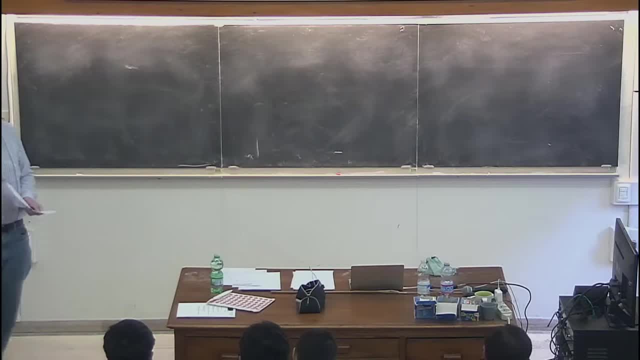 that you're going to make the discovery. But what you can say is: look, the experiment will be. it will have such a quality that if it's there, I will get you five sigma, or so-and-so many sigma, discovery significance. So first of all, we need to say a little bit more. 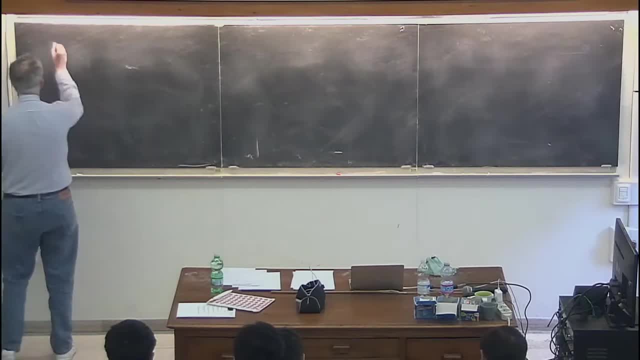 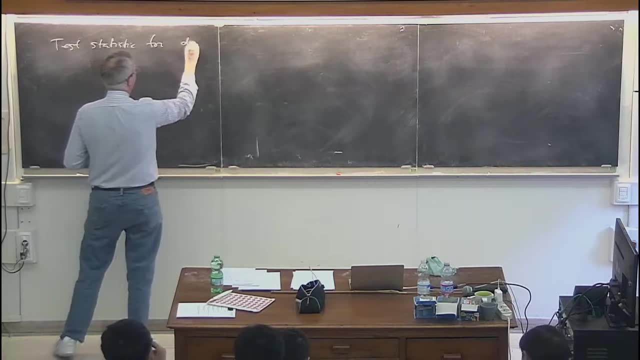 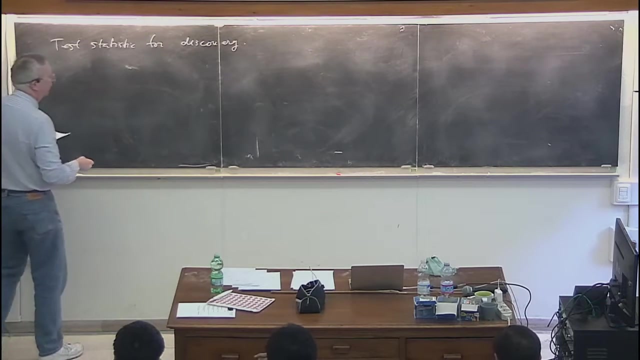 about how to quantify the significance of a discovery. So here's something about the test statistic that you would use for discovery, And it's going to be very similar to the profile likelihood ratio that I just showed you, So I'm going to use this strength parameter mu. 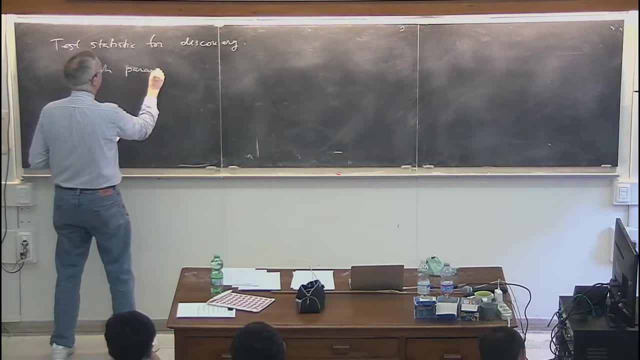 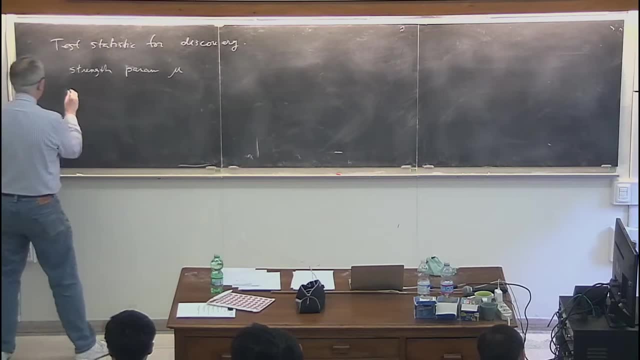 like I defined before. So mu equals zero, corresponds to the background-only hypothesis, And so what I want to do is to test the hypothesis that mu is equal to zero. So I'll call the statistic q0. And I'm going to take it to be the following: 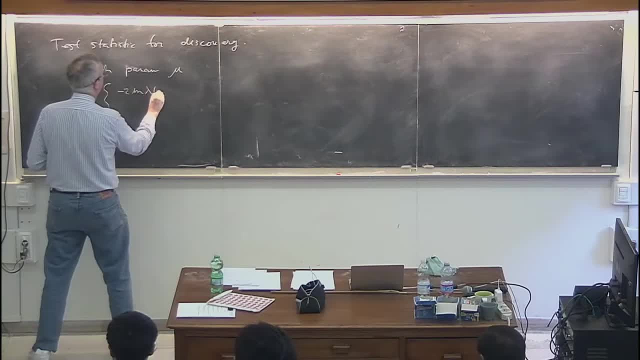 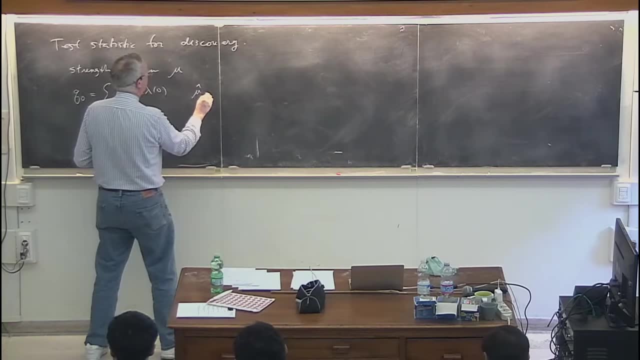 I'm going to take it to be equal to minus 2 log lambda of zero, where it's the same lambda that I had before. All right, So I'm only going to take it to be that if the observed signal strength fluctuates positive. 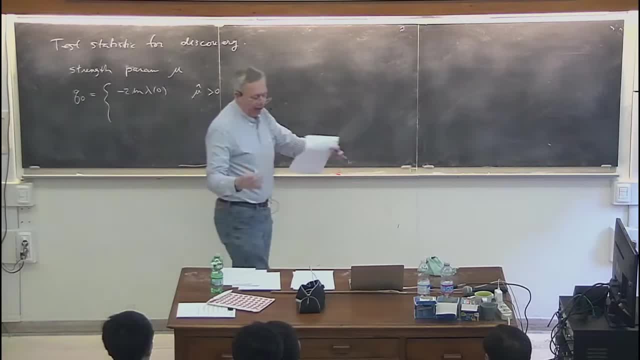 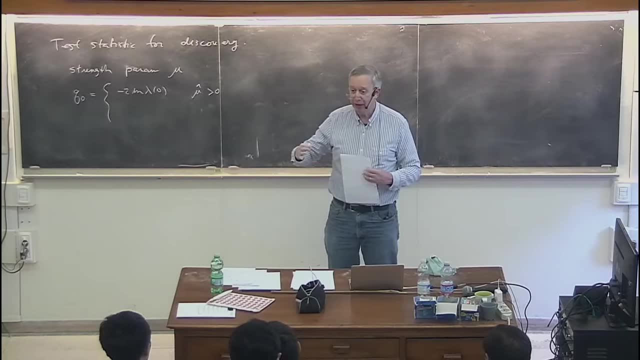 If the signal is actually absent. so I only have background and I try to fit the observed signal rate. that could fluctuate negative, because I might see actually fewer events than what is expected from background alone. If that happens, though, I don't want to exploit that happening. 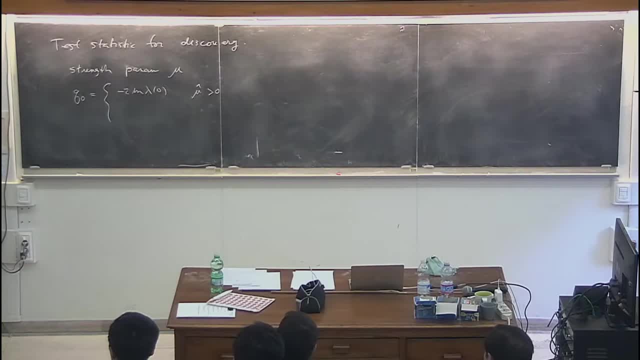 to claim that I've discovered a new phenomenon. If I expect 100 events and I see 62, then that is a discrepancy, But it's not the sort of discrepancy that I would exploit to write a paper saying I've discovered a new signal. 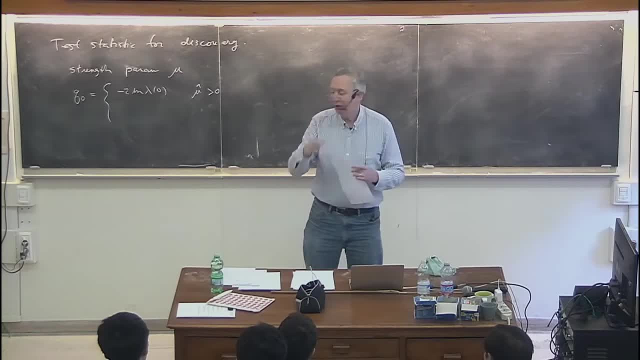 if I think that signal should only add events. So I'm going to simply assign a value to the statistic of zero Because, remember, it's high values of this statistic correspond to incompatibility with the hypothesis. I'll say if mu hat fluctuates negative. 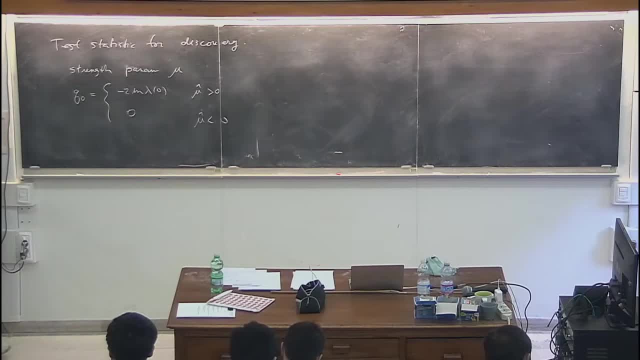 I'm not going to count that as representing any event. It's going to be incompatibility. So if I take that definition that's a little bit different from the formula I had before. But I assume that the large sample asymptotic form 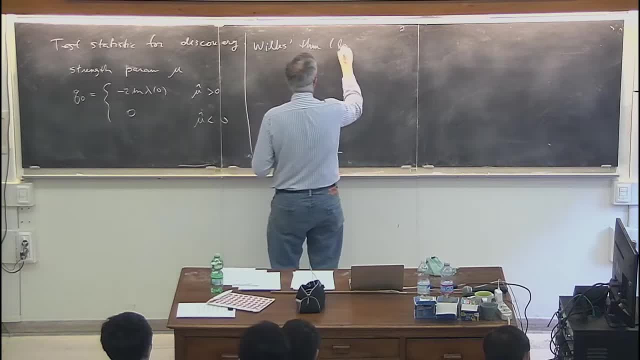 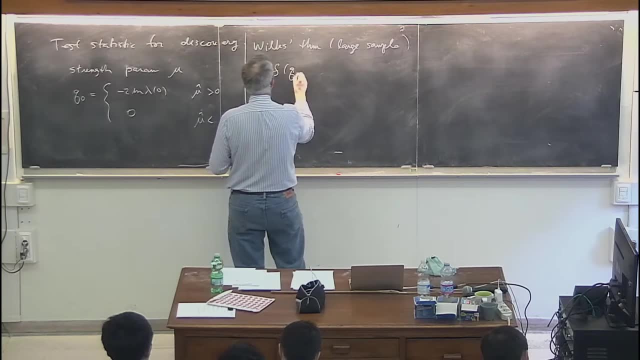 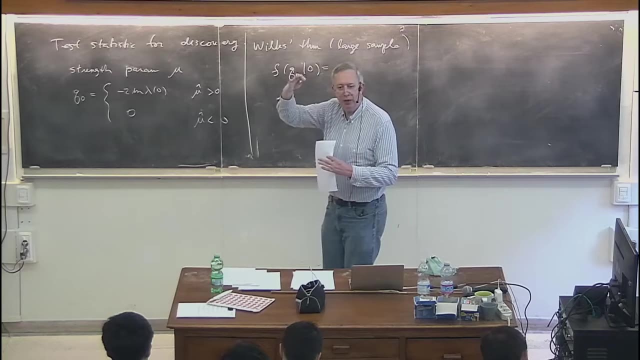 is valid from Wilk's theorem, So the large sample limit. It's going to give me the following PDF for the statistic: The distribution of Q zero, assuming mu equals zero if the data fluctuates low. so I get fewer events than expected from background alone. 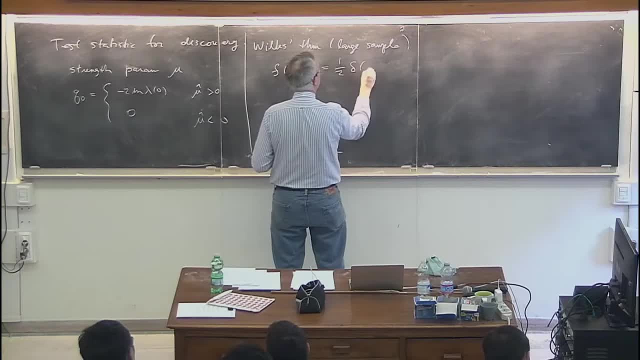 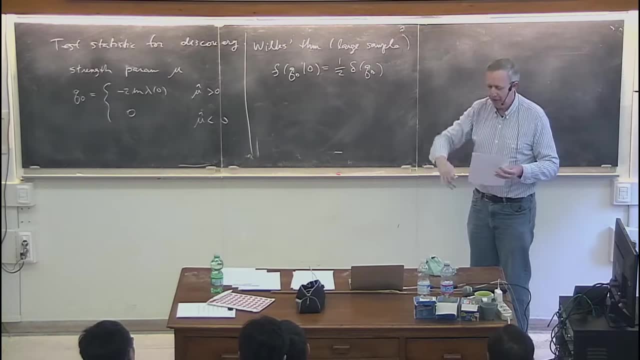 I get zero, And so this is going to give me a delta function at zero, And that'll have a probability of one half If I have no signal. half the time it'll fluctuate up, half the time it'll fluctuate down. 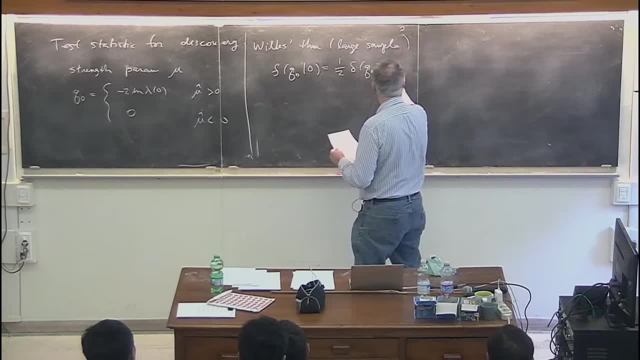 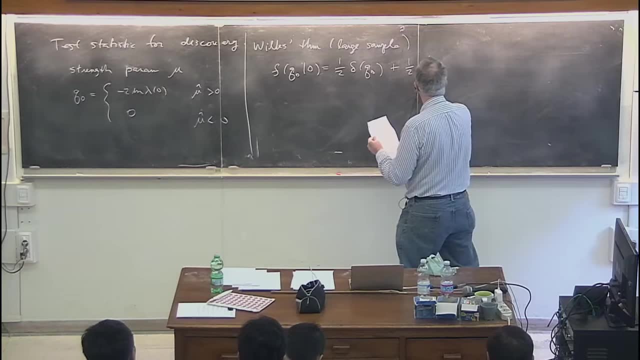 If it fluctuates up. so I get mu hat greater than zero, then what I get is a chi-square distribution for one degree of freedom, also with a weight of one half, And I'll just write the formula for the chi-square distribution. 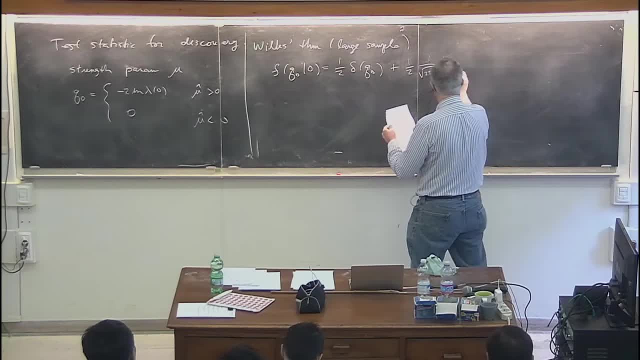 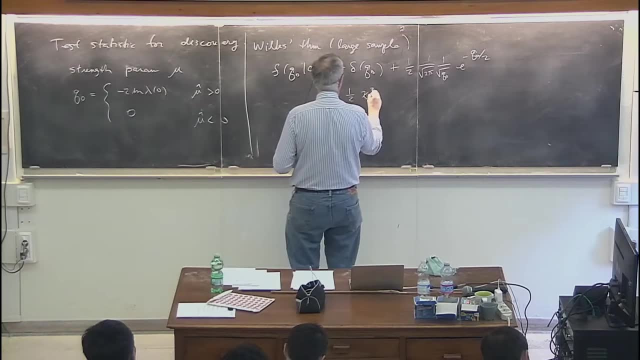 It's one over root two, pi, one over root Q zero, e to the minus Q zero over two. So sometimes we call this a half chi-square distribution. That's just our own particle physics name for this, because that's a chi-square distribution. 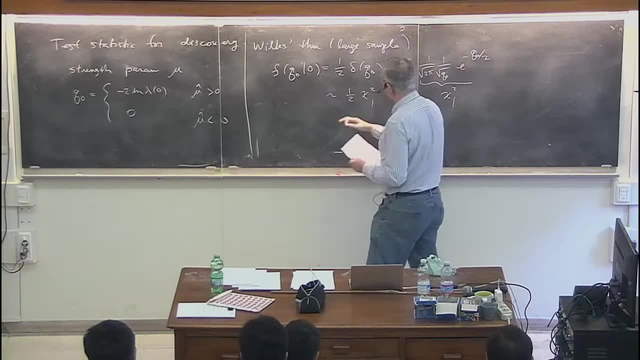 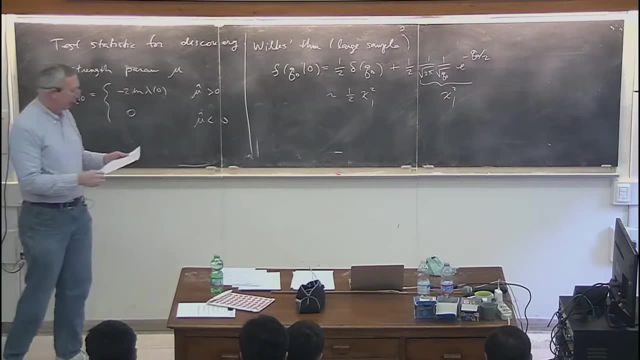 this much of it, chi-square for one degree of freedom, And so it's a delta function at zero with a weight of a half, and a chi-square distribution for one degree of freedom with a weight of one half. Once I have that distribution. 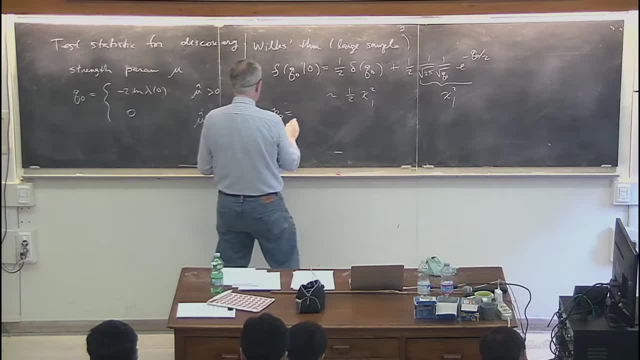 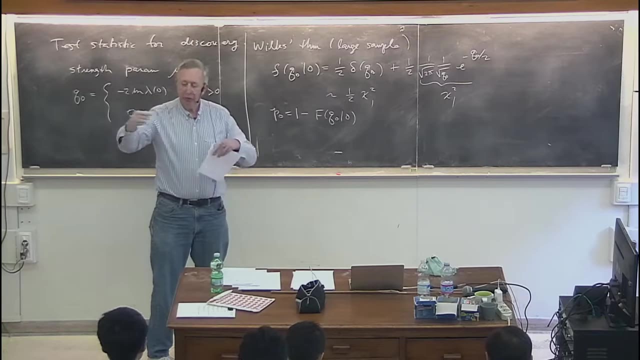 of course I can find my p-value, And that is just one minus the cumulative distribution of that statistic, And what you can show is that this cumulative distribution for a chi-square distribution is related to the. I told you that the chi-square distribution and Gaussian distributions are related. 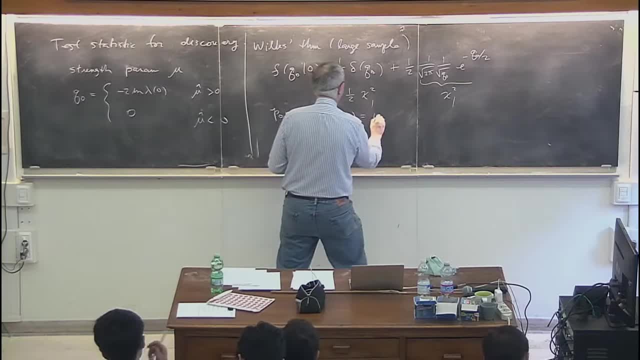 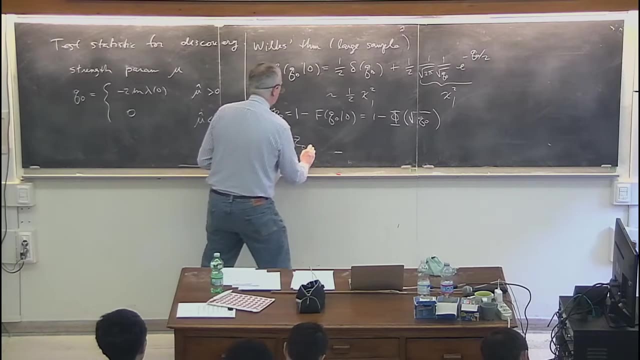 This turns out to be equal to one minus the cumulative Gaussian distribution of the square root of Q, zero. All right, And that means that the discovery significance, once I have the p-value, the corresponding discovery significance is capital phi inverse, the standard normal quantile. 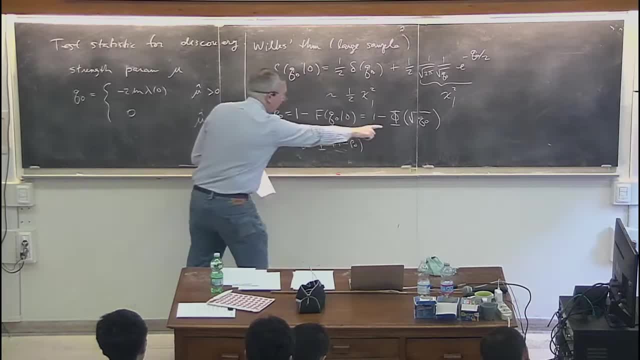 of one minus p zero. Ah, but notice that p zero now includes a standard, normal cumulative distribution And the phi inverse hits the phi and they annihilate. And I get a very simple formula: Square root of Q zero. All right, Really easy answer. 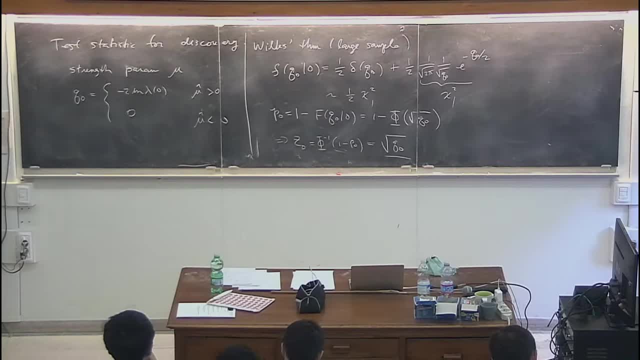 So if I just follow this procedure, I compute my Q zero from the data, I take its square root. If I get a number here of 25, say: and so my square root is five, voila, I have five sigma significance. 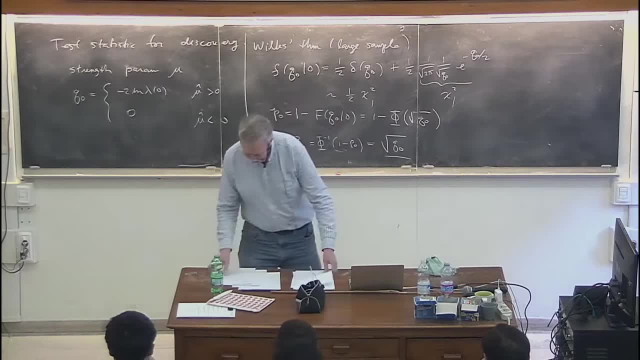 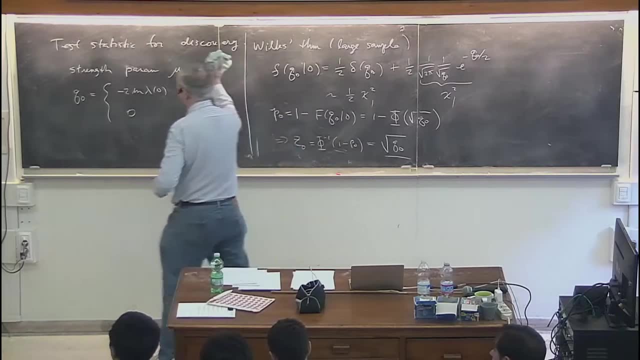 with which I reject the standard model hypothesis, The background only hypothesis. Now I want to get on. I realize I'm running out of time. I'm trying not to rush this too much, But I want to use this now to show you something. 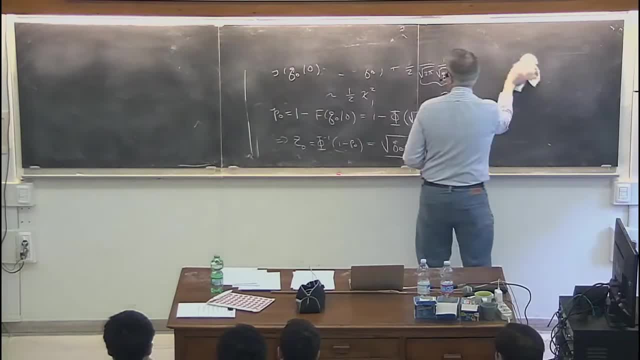 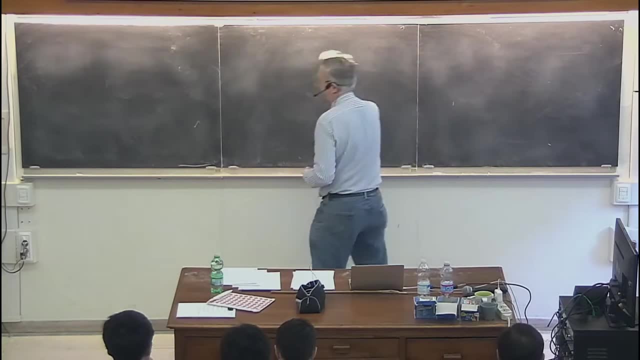 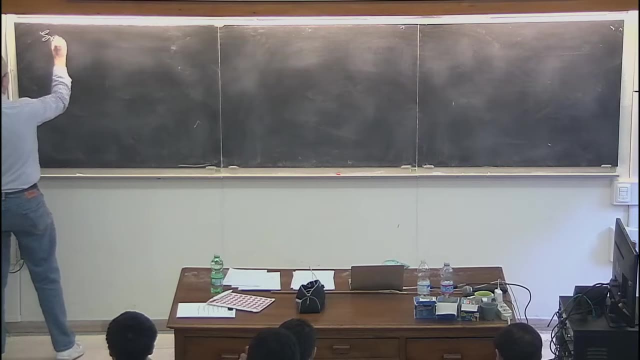 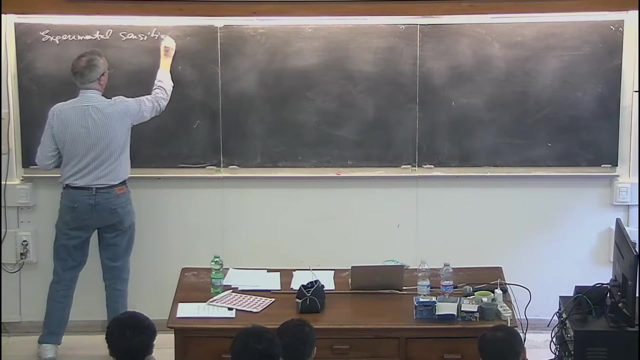 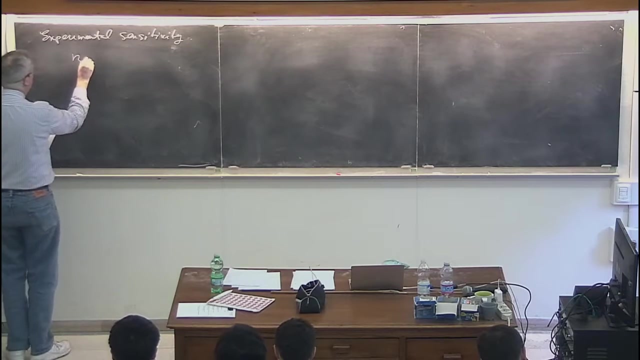 which I think is really useful, And I can kind of do it in five minutes, And so this is now back to this point of experimental sensitivity. So let's go back to the one-bin Poisson equation. This is a Poisson counting experiment. 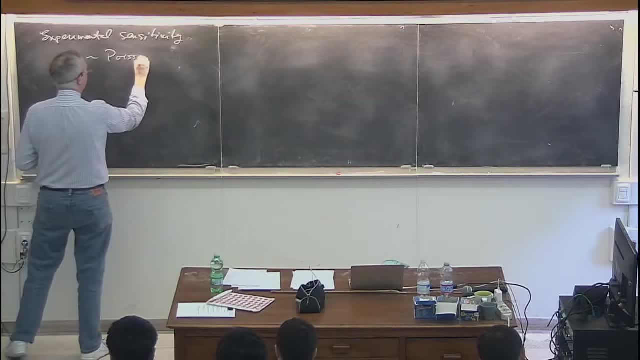 So I count as my data a single number, n, which is Poisson distributed, with a mean of s plus b, And one of the things that you probably know about the Poisson distribution is that when its mean gets very large, the Poisson distribution starts to look like: 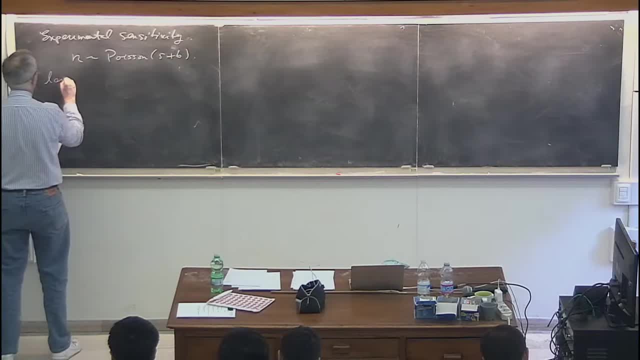 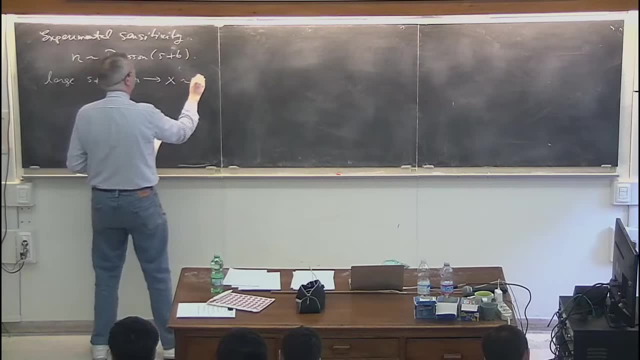 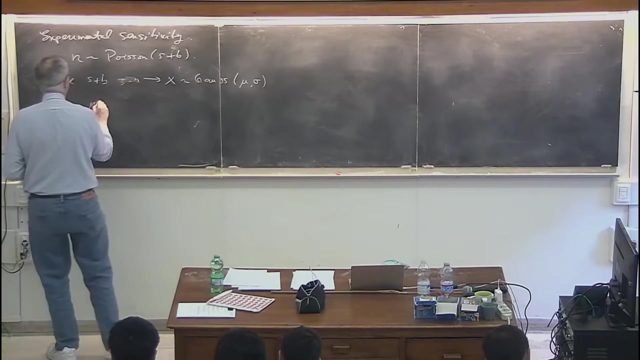 a Gaussian distribution, All right. So for large s plus b, n acts like a continuous variable Following a Gaussian distribution, And the mean and standard deviation would be. Well, the mean, of course, is the same as the mean of the Poisson distribution. 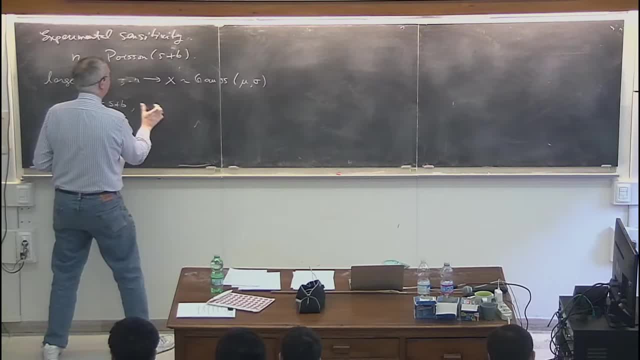 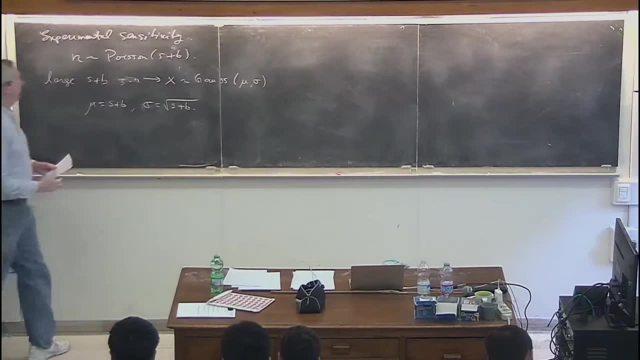 s plus b And the corresponding standard deviation is the square root of the mean, Because that's what you get for the Poisson distribution. So for a sufficiently large mean I can replace my Poisson distribution by a continuously distributed Gaussian variate x. 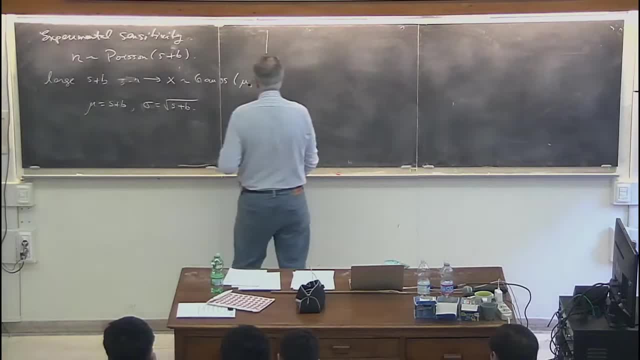 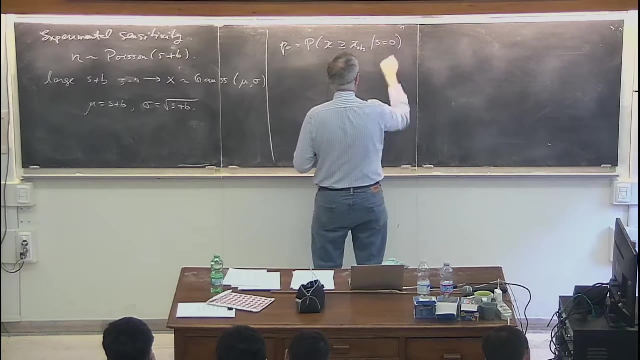 And the corresponding p-value that I would get for the hypothesis of s equals zero and p zero is just going to be the probability that x now is greater than or equal to x observed under the assumption of s equals zero. All right, 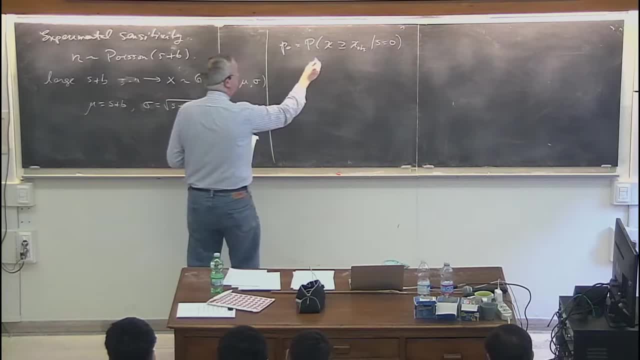 But that's I can write down just in terms of the cumulative distribution of a Gaussian. So this is now one minus the cumulative distribution of a Gaussian, And, if I use the fact that this is supposed to be with the assumption of s equals zero. 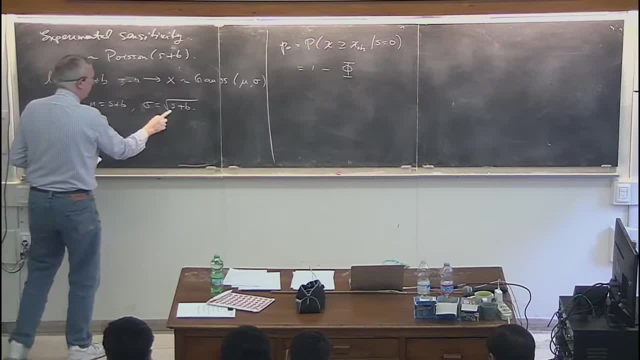 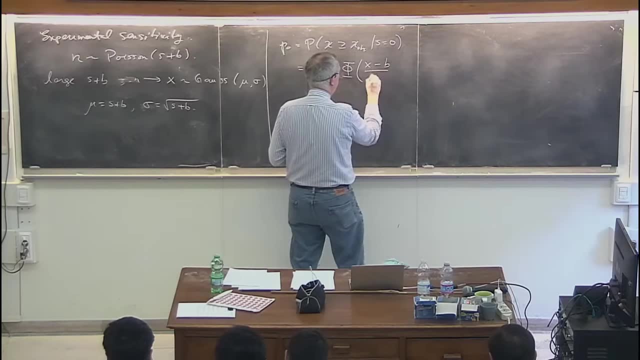 so I have a mean of b and a sigma of root b, so this is going to be phi of x minus b over root b, Right, Where that x now refers to the observed value. Okay, so once I have the p-value. 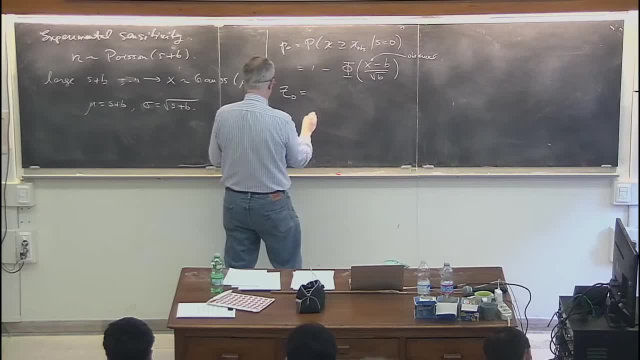 I would then say that the corresponding significance is phi inverse of one minus p. But here again I've got the phi inverse and I've got the phi, And they, The two, cancel each other, so to speak. And that gives me then: 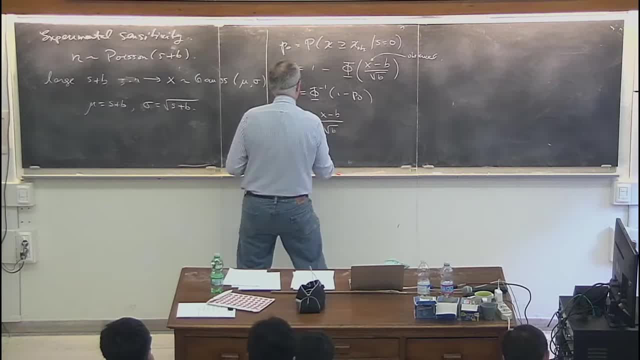 x minus b over root b. So if I actually observed a number of events, n, or I call it x, that's then the formula that I would use to give the significance. All right, And we've actually, in some of the hand-wavy arguments, 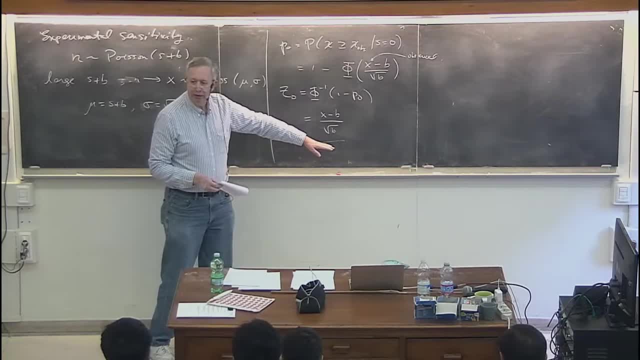 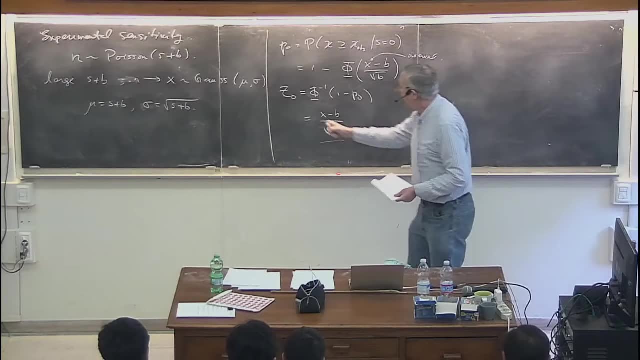 that we were talking about yesterday. that's implicitly what we were doing. All right, But now that's not the number that I want to tell the funding agency before I get the money for the experiment. I want to tell them what I expect this value to be. 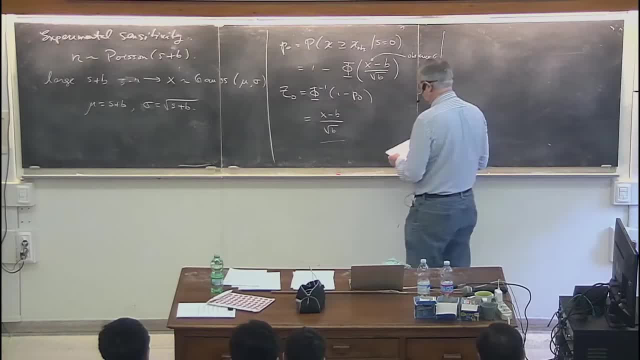 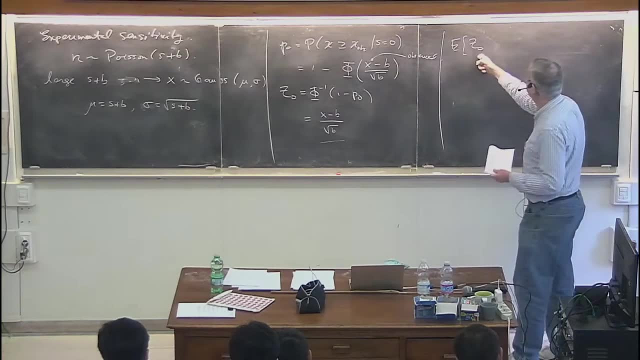 if the signal is really present, And so what I want to give is the expectation value of the discovery significance. So I'm testing: s equals 0, but I want this expectation value to pertain to a non-zero value of s. All right, 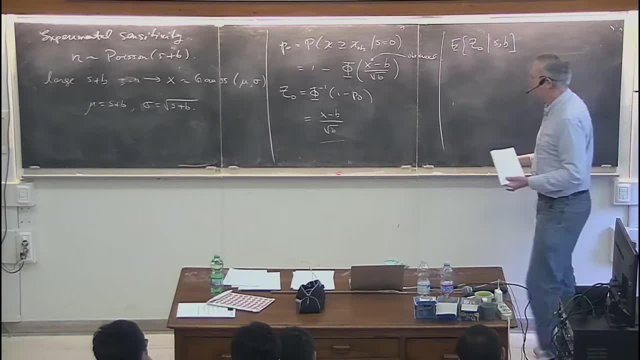 Namely the value of s. that corresponds to my nominal signal model. So if I take the expectation value of x, assuming a mean of s plus b, this is going to give me s plus b minus b over root b, which is s over the square root of b. 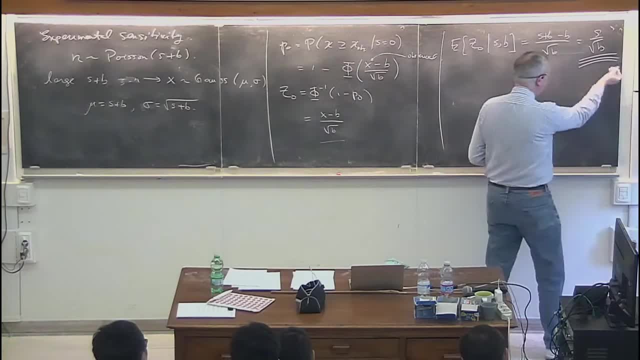 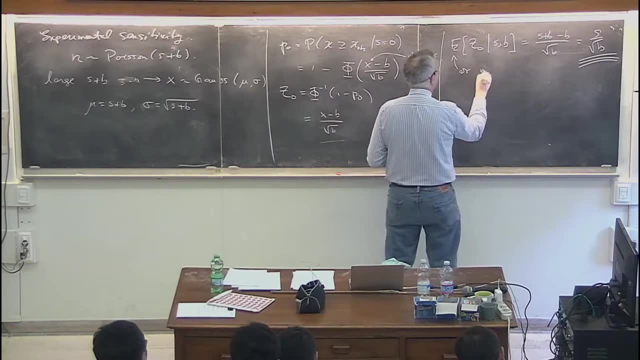 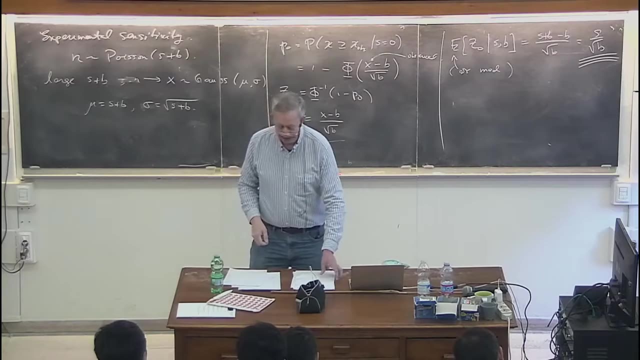 All right, And so that's the expected discovering significance And that's the number that you would report to get your money. For technical reasons, we don't use the expectation value. Sometimes we use the median, But that's a point we don't need to get into. 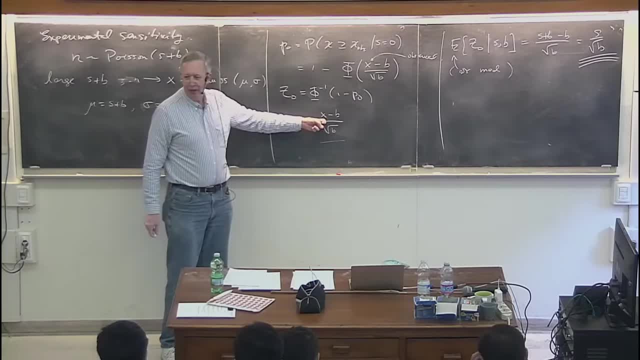 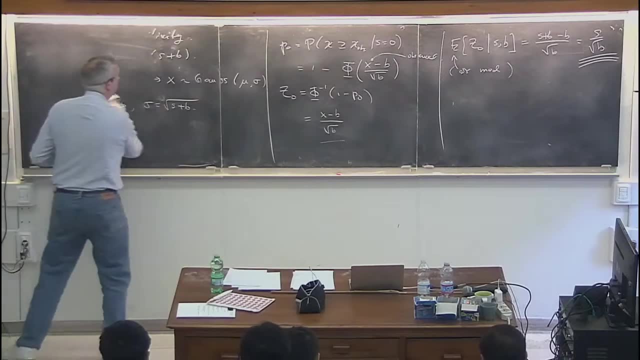 In this case, no, No, because x is going to be Gaussian distributed and the median is equal to the mean. Now, final thing is the following: is that people use that all the time, and I'm sure that you've heard. 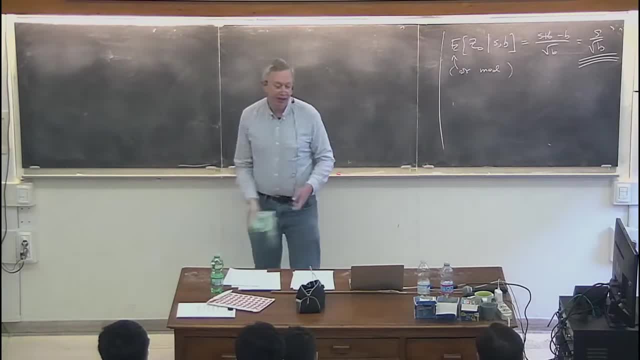 of s over root b. It's the kind of thing if you just walk around the canteen at CERN at lunchtime you'll hear oh s over root b, this s over root b, that It's always being referred to. 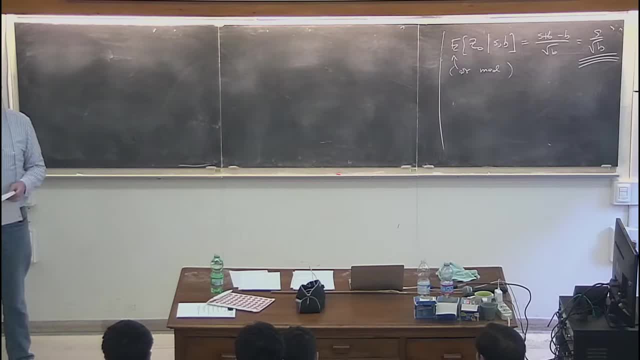 But in fact it only holds in this limit where the Poisson distribution looks like a Gaussian distribution And that's not necessarily a very good approximation. We said originally that the data were Poisson distributed, So let's go back to that right. 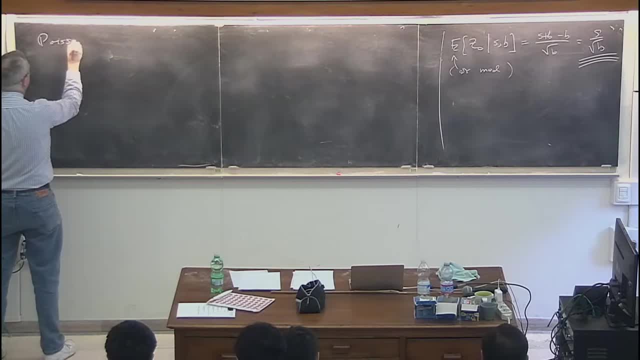 Let's write down the Poisson likelihood. what we have here is the Poisson likelihood. The Poisson likelihood is that the Poisson coefficient is equal to the L of s, that's s plus b to the n over n factorial e to the minus s plus b. 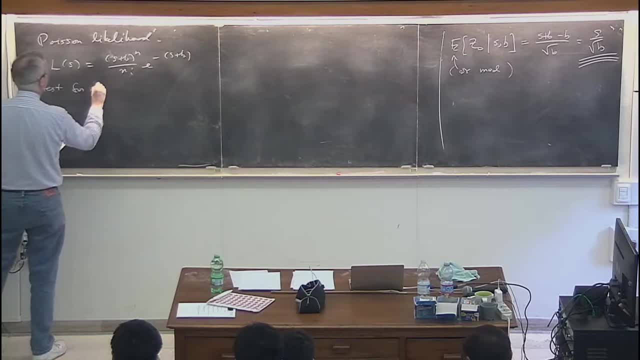 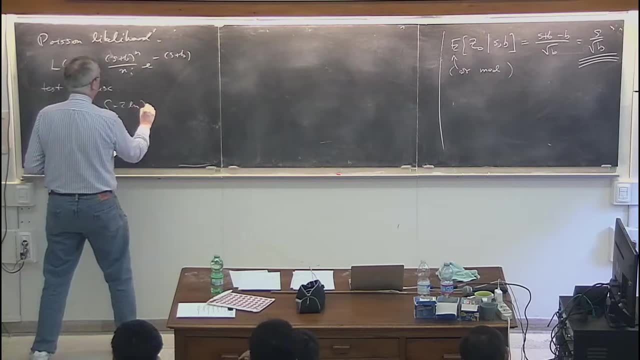 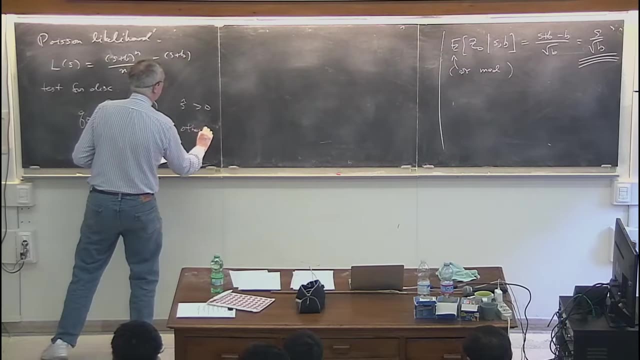 So there's the likelihood, And I want to test for discovery, And I will use the same statistic that I defined before. I'll say that this is minus two log lambda of zero for s hat greater than zero and zero otherwise. So s is playing the role of mu before. 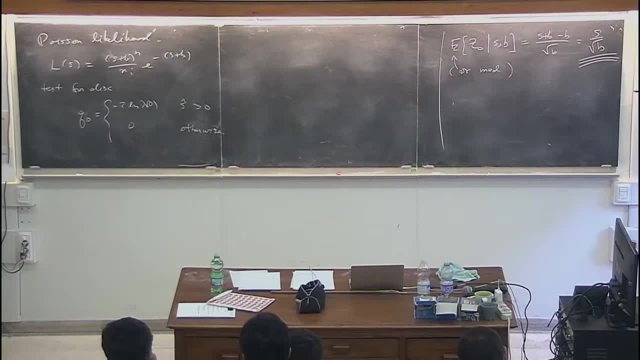 because I only have one measurement. All right, so that's the statistic. And if you plug in that likelihood into this thing, what you get is 2n. log n over b plus b minus n. That's what you get if n is greater than b. 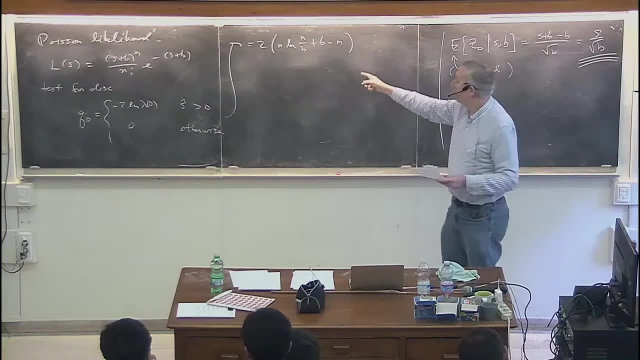 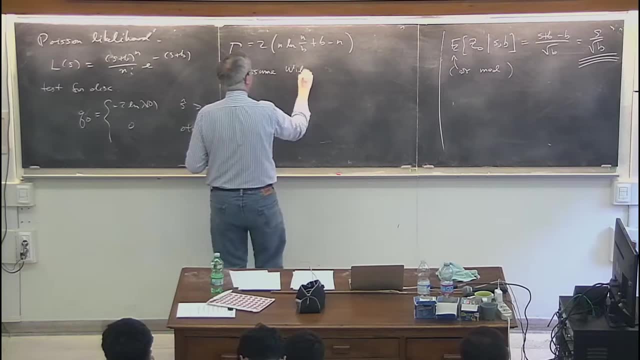 and it's zero otherwise. Okay. so that's the. let's see, that's Q0.. And now I said I'm going to assume Wilkes. Strictly speaking, Wilkes theorem is also only valid in the very large sample limit. 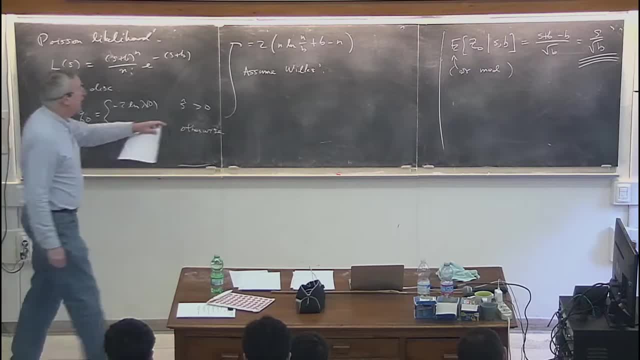 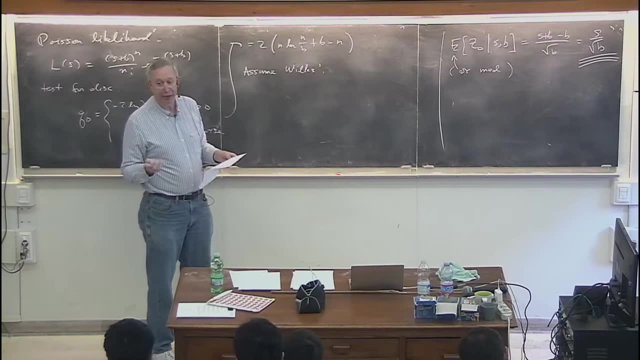 And then you might say: well then, your Poisson's like a Gaussian, But the validity of these asymptotic forms from Wilkes theorem kicks in much earlier. All right, it's still valid, even for just a few events. So I'm going to say I'm going to use s sorry. 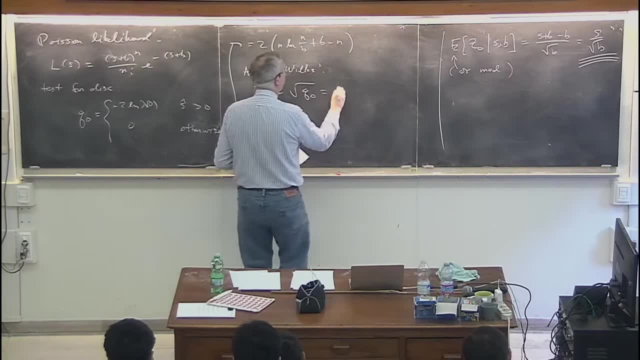 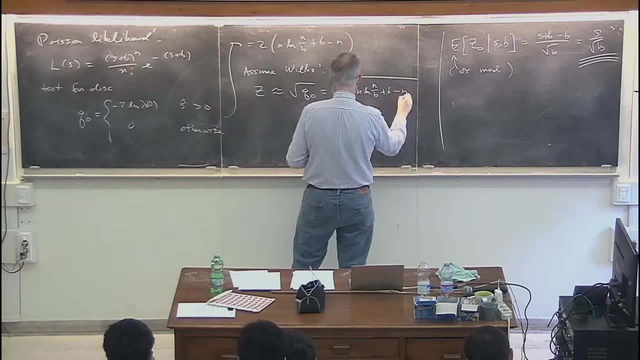 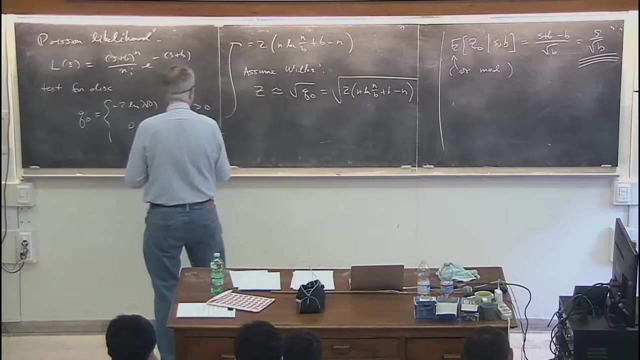 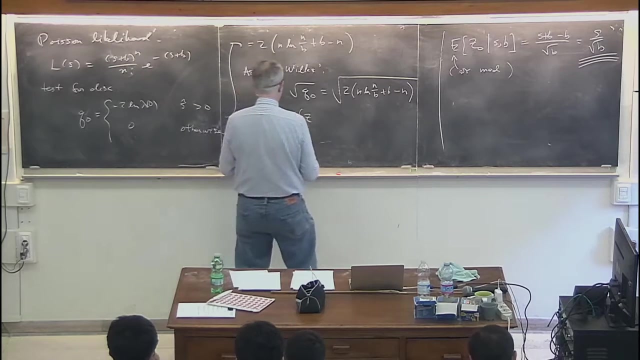 the significance is approximately equal to the square root of that, So square root of 2n. log n over b plus b minus n, voila. And so now what I want to do is to find the expectation, or median. I'm going to use the median now, z all right. 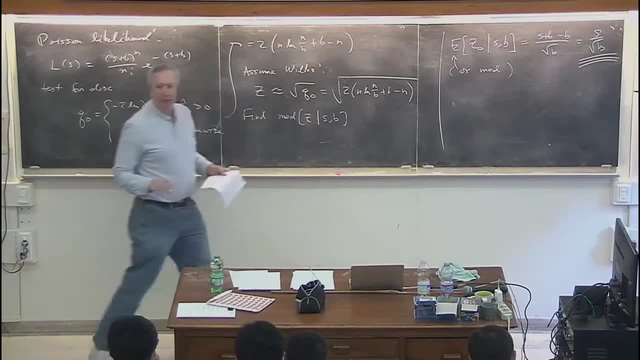 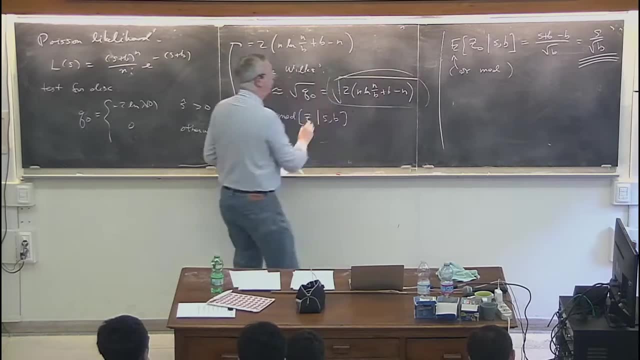 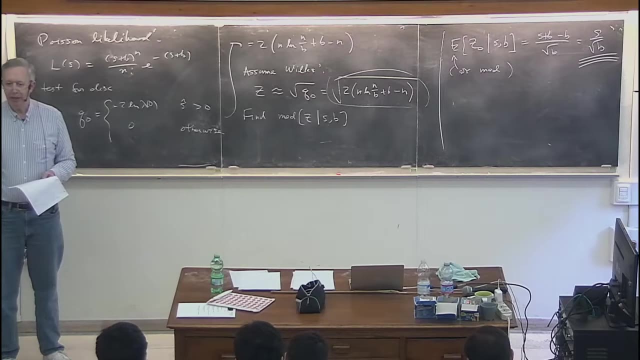 assuming I have signal, all right, and that's the number that I would use. And so the question is: how do you find the mean or median of that quantity? assuming that n follows a Poisson distribution with a mean of s plus b, That would be a difficult. you can't do that in closed form. 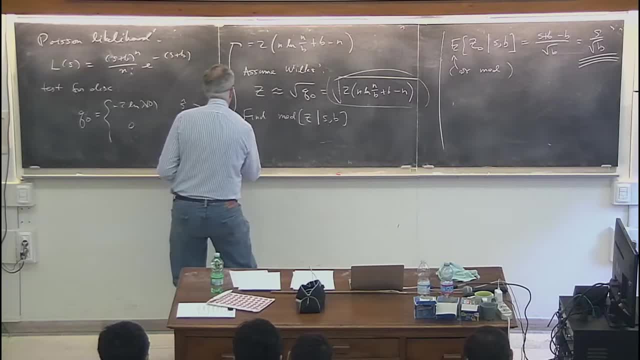 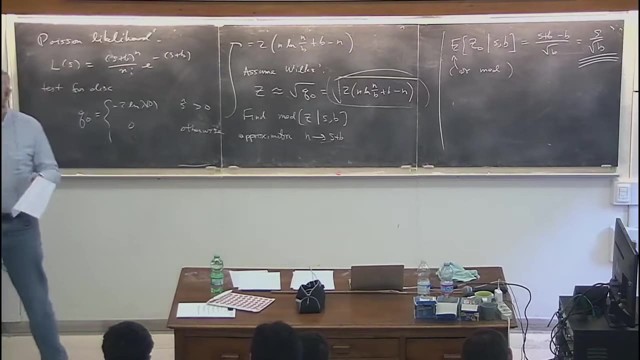 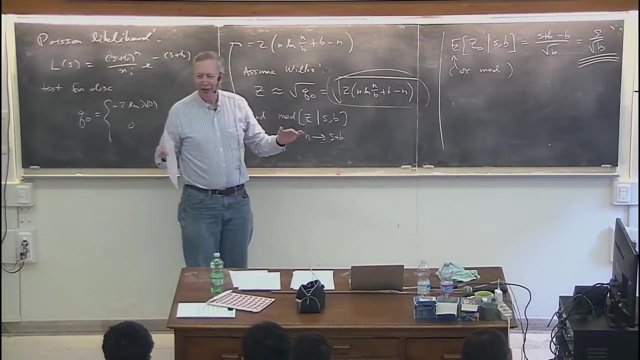 But there's a simple approximation, and that's the following. You see, you simply ah approximation. you simply replace n by s plus b. So instead of somehow generating an ensemble of experiments according to a Poisson distribution, evaluating z for each one and then computing the average, what I'm going to do is I'm going to just take. 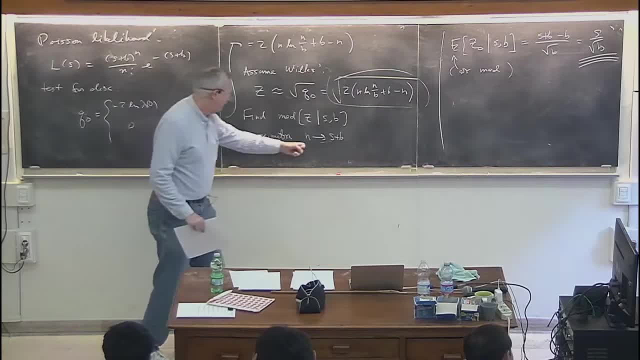 one data set that I consider to be representative, namely, I'm going to replace n by s plus b, even though that's an integer, and this isn't Plug it into that formula, and what Monte Carlo studies show us is that that, in fact, is a very good approximation, And so that's going to give. 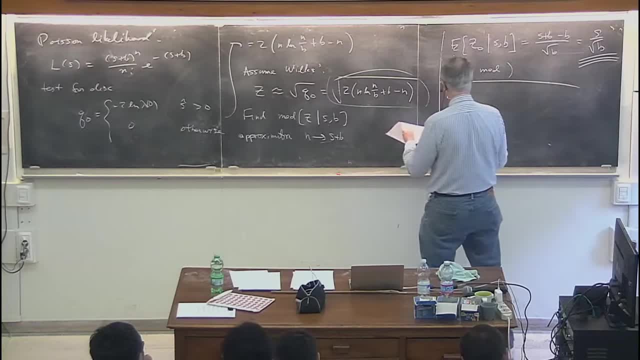 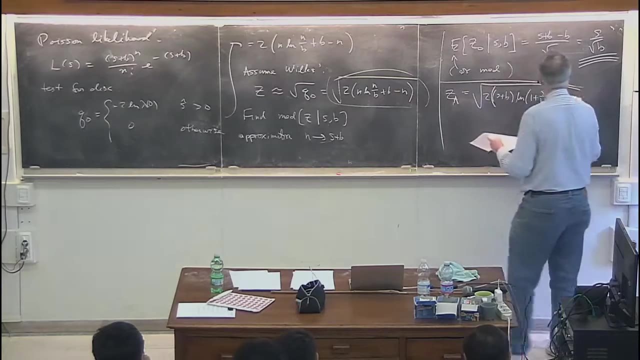 me this formula, which I'll call z sub a. I'll explain the a in just a second, And that's the last formula that I'm going to show you. Sorry, one more parenthesis: Log of 1 plus s over b minus s, Voila. So that's, then, the formula that we very often use as a replacement for s over root. 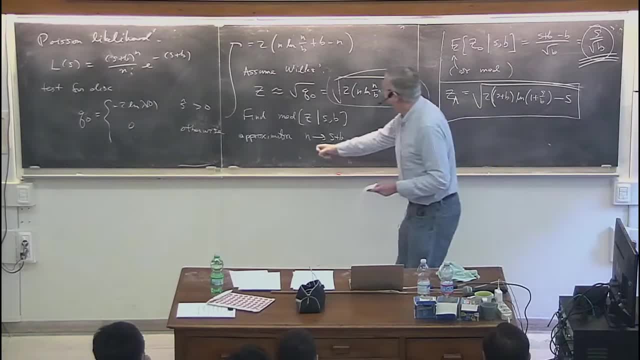 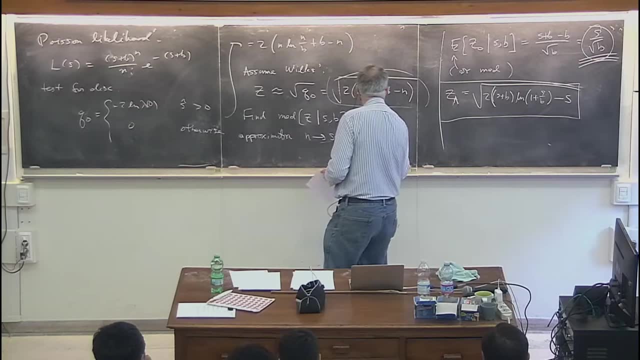 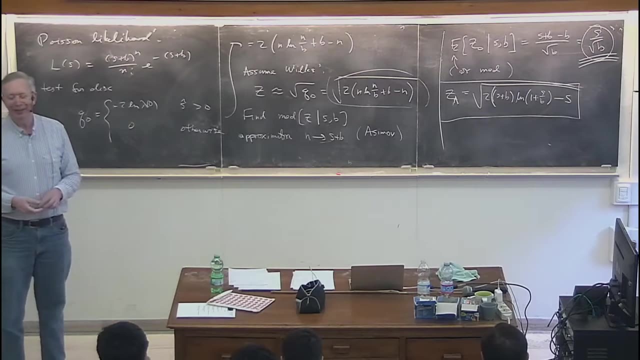 b. So this thing about using what I call a representative data set is what we call sometimes the Asimov data set, And that's a term that's almost caught on and I feel a little bit guilty about that, Having pushed it early. So I'm going to explain the Asimov jargon behind this And Isaac Asimov. 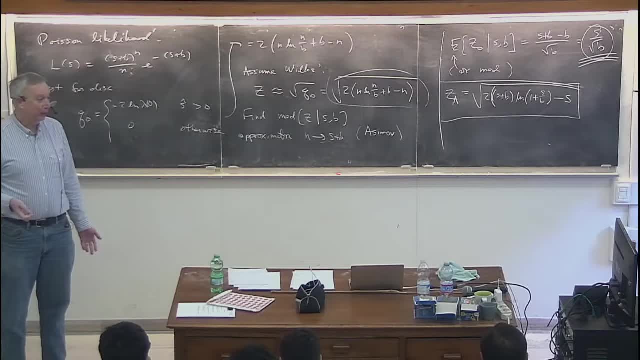 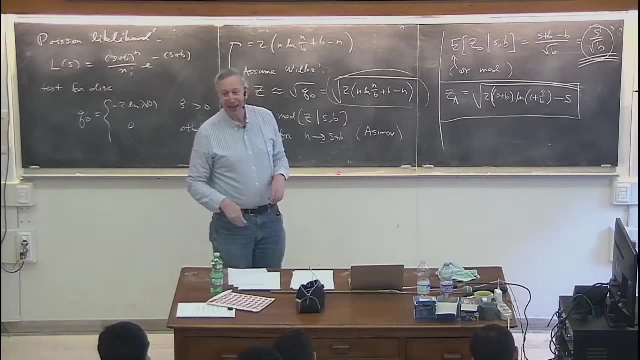 the science fiction writer in the 1940s wrote a short story called Franchise, And this was describing the far-flung future of 2008.. And in 2008, in America, presidential elections had gotten too expensive. They couldn't hold them anymore, And so what they did instead is they. 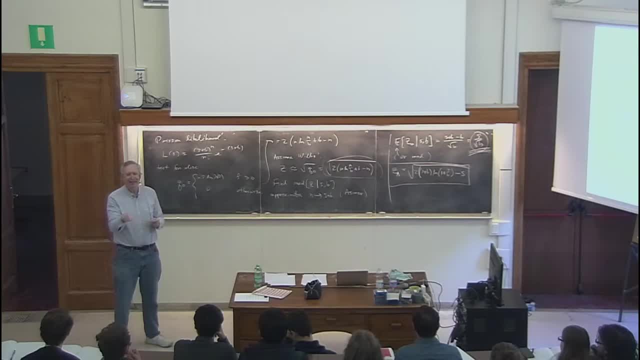 had this super-duper computer And the computer was smart enough to identify the guy, who was like the most average boring, typical person in the country, And once they find him they sit him down in a chair and say: what are your? 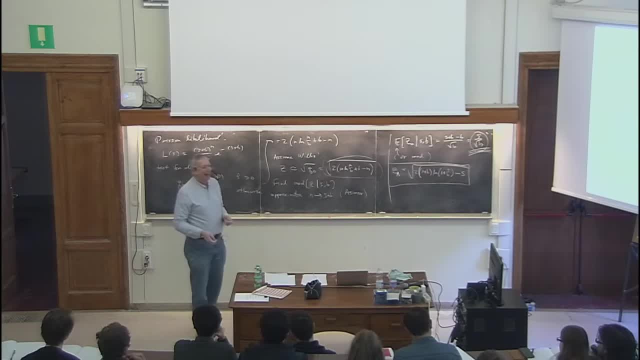 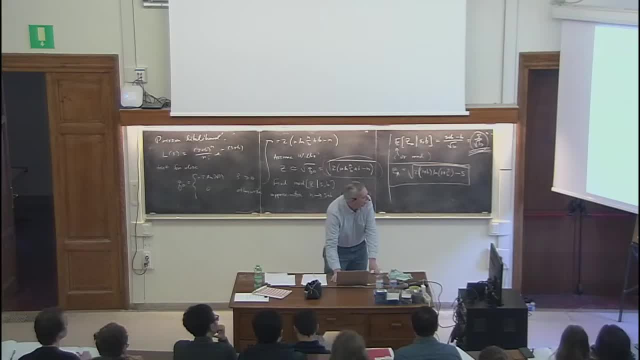 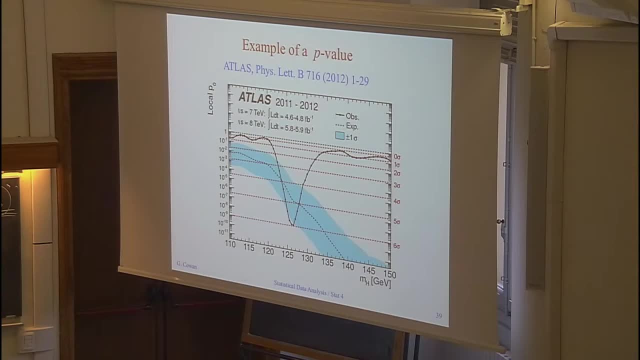 And that's about where I'm going to stop. I'm just going to show you really quickly. Say again: The median. yes, So I could just use the expectation instead. I don't want to dwell on why I use the median instead of the mean the expectation, but they're very close. We find it's a better. 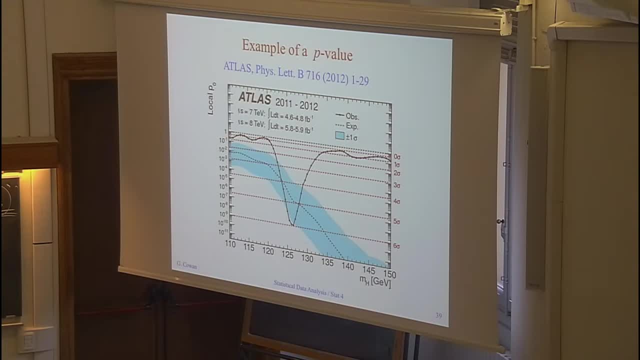 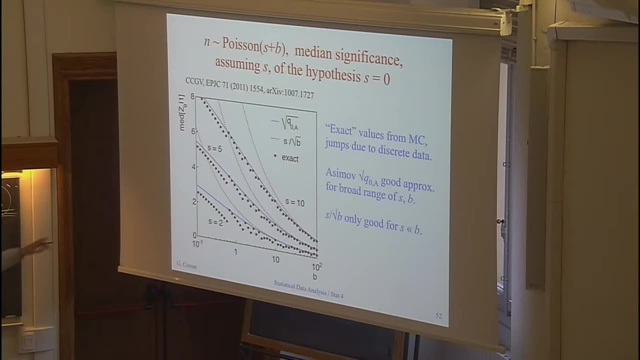 approximation for the median. I'm going to show you and just if I can get. I realize it's lunchtime and I want to stop, but so here's the median discovery significance as a function of b for several different values of s. 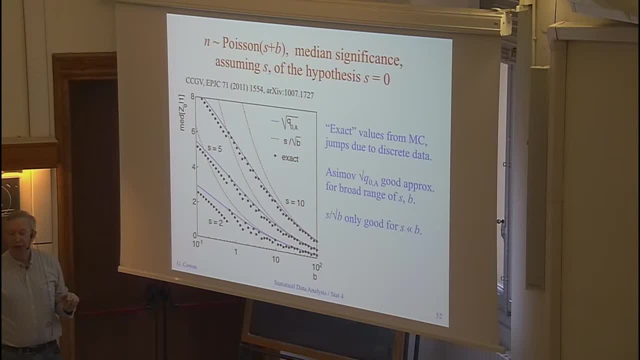 all right. the dots were computed with Monte Carlo, so by construction they are exactly correct. they make no approximation right. the red curve is the s over root b curve and you can notice that everything agrees if I have sufficiently large b. but this Asimov curve is the blue curve. 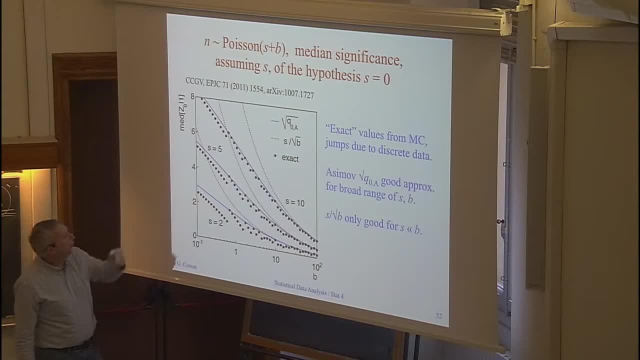 and you'll notice that if I go down towards smaller b, the blue curves continue to approximate quite well the exact dots, whereas the red curves overestimate substantially. so if somebody tells you I'm planning this experiment and it's got a very low background, b is equal to one and I expect. 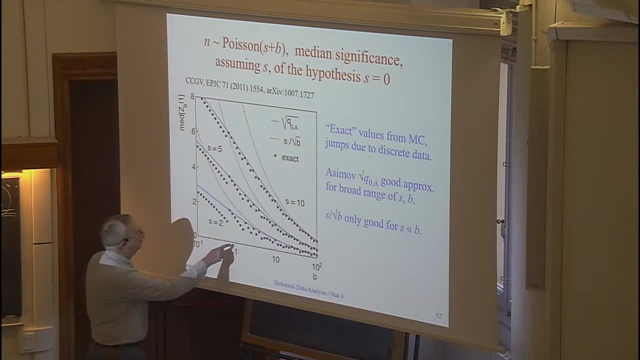 you know an s of five, and so I'm going to tell the funding agency that I expect to get a five sigma discovery significance. and I'm going to tell the funding agency that I expect to get a five sigma discovery significance and I'm going to tell the funding agency that I expect to get a five. 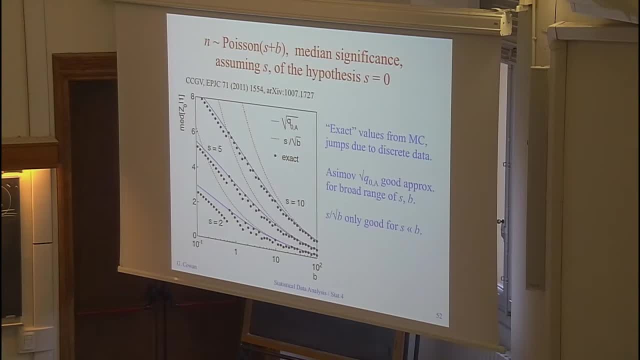 sigma discovery significance. they might get funded, but they shouldn't. that's unfair, because really they should be using the blue curve here and that's less than four sigma. okay, so it's important. I've gone over, so I'm going to stop now.